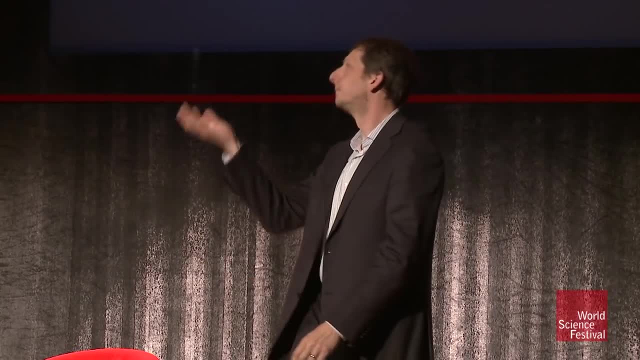 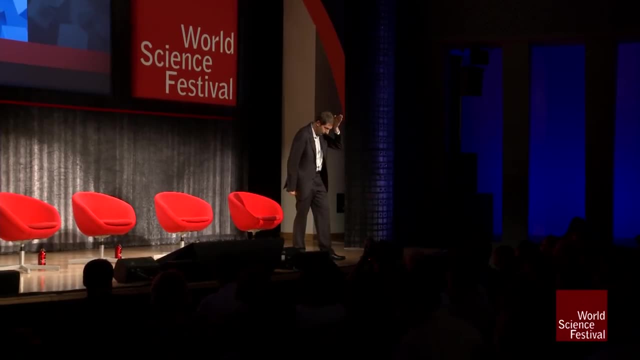 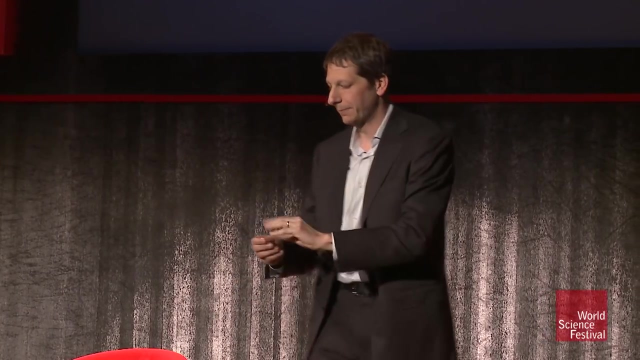 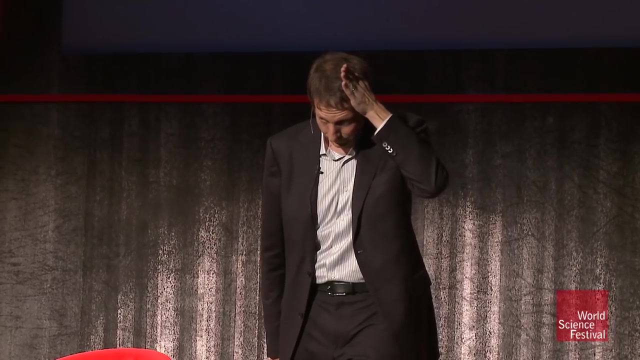 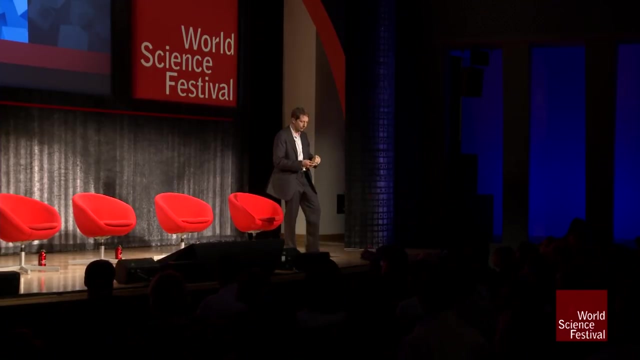 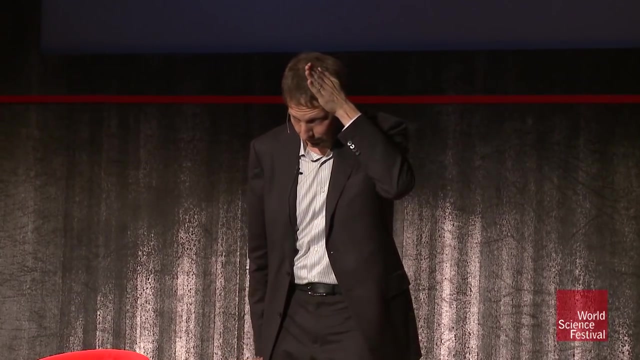 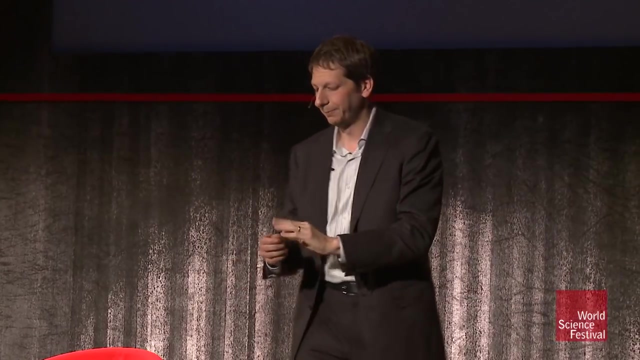 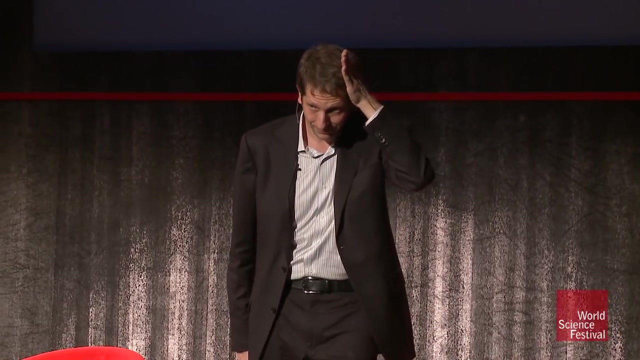 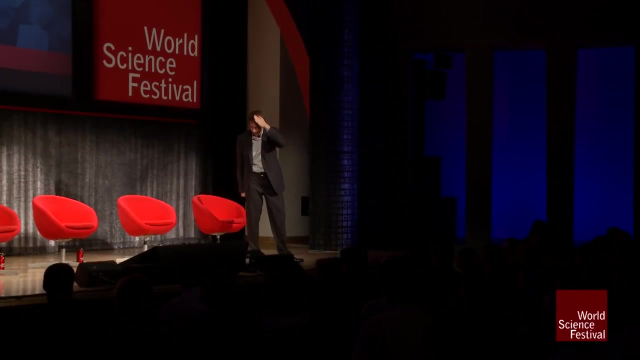 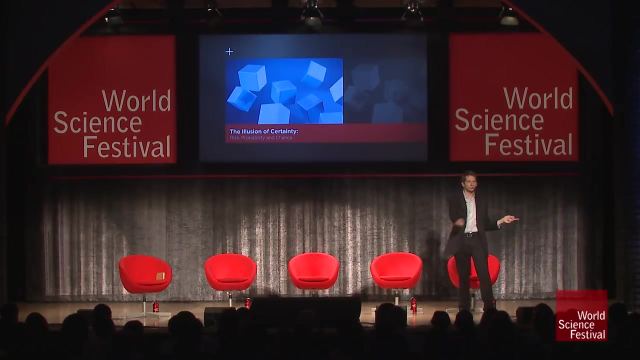 Second flip: All right. Number three, Four: Okay, Last one, Last one, Okay, Very good. Now some volunteers are going to come down both aisles and we'd just like you to pass your card to the nearest aisle and they'll collect them. You may be wondering. 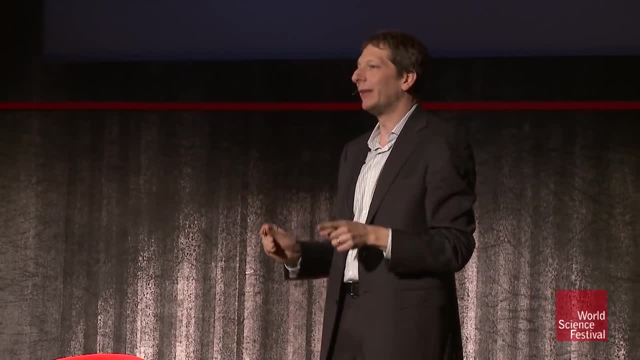 whether you got it right or not. Hold that thought. Don't hold the card, but hold that thought and we'll come back to it later in the show. All right, Please pass in your cards and I will see you in a minute. 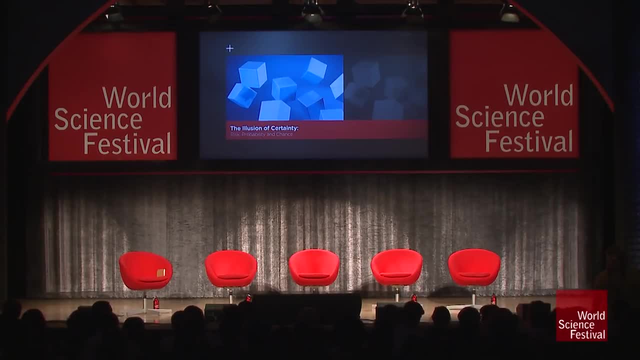 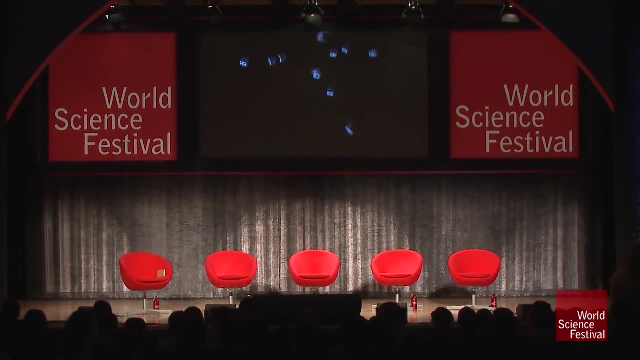 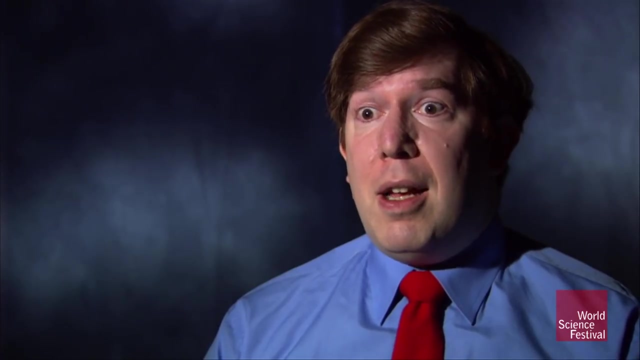 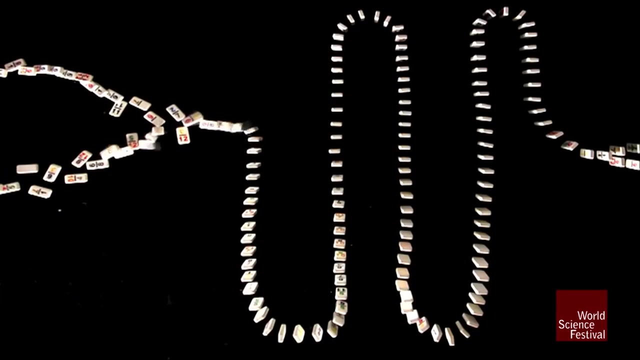 We like to think of numbers as being absolutely true, absolute truth incarnate that numbers in some sense are Truth handed down from a platonic realm above us. One plus one is always two. It's never going to change itself and become three. But every number comes from a measurement of some. 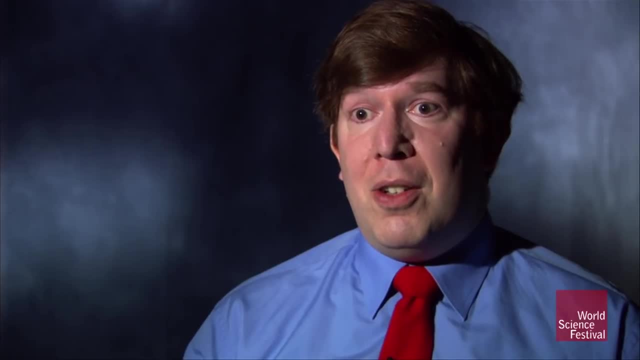 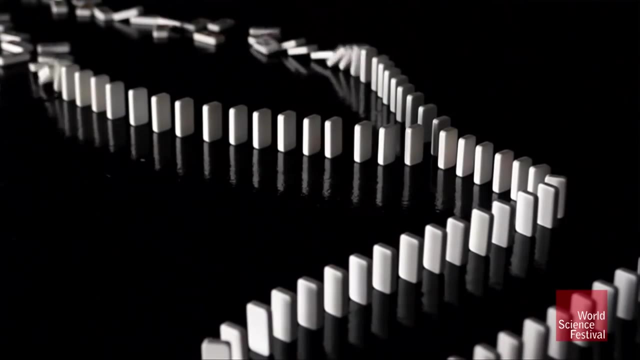 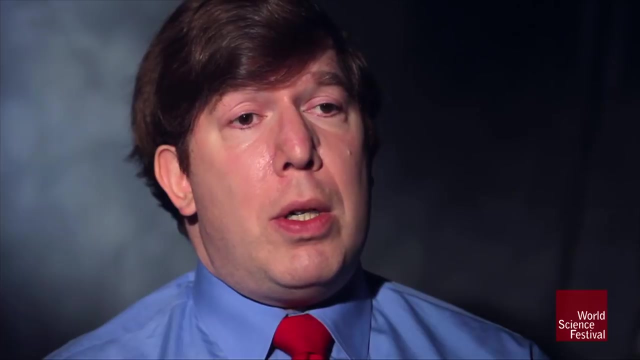 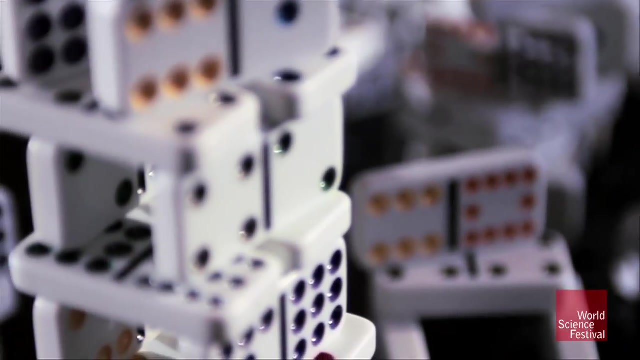 sort And because we humans are doing the measurements, they're not entirely true. A good example of this occurred in Britain. Three women had two children die of SIDS And there was an expert witness, a very famous pediatrician, Who testified that the probability of having two children die of SIDS was infinitesimal. 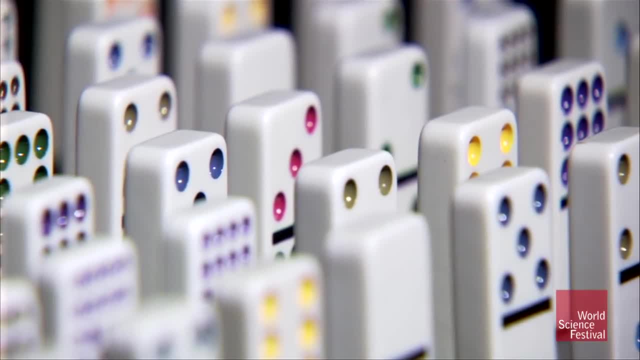 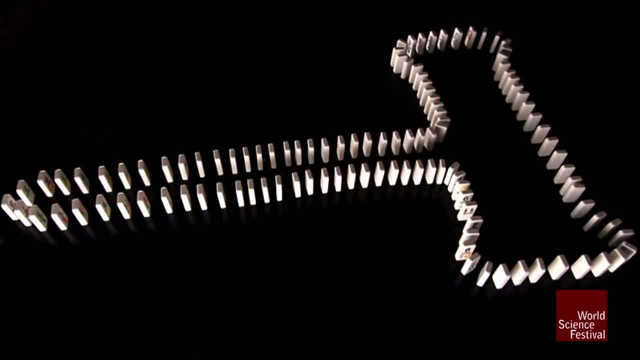 One in 73 million. So, he argued, such a small probability means that it's much more likely that the women were murderers. The probability that a child will die of SIDS is actually not a straightforward calculation. It could be that there's something genetic, or there's something even in the environment. So if, in fact, your first child died of SIDS, your two children are probably so much more likely to die of SIDS than you would, And it could be that you have a very special relationship with someone who died of SIDS. One of the reasons that we think this is so important is because 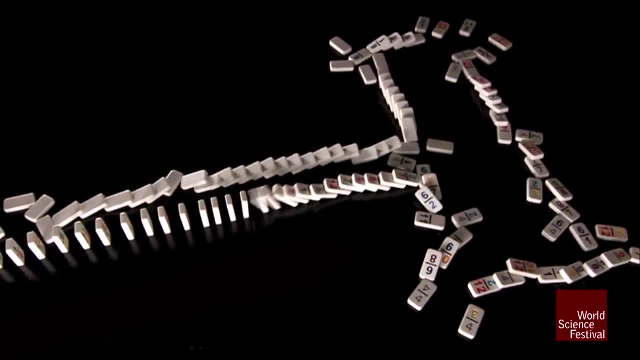 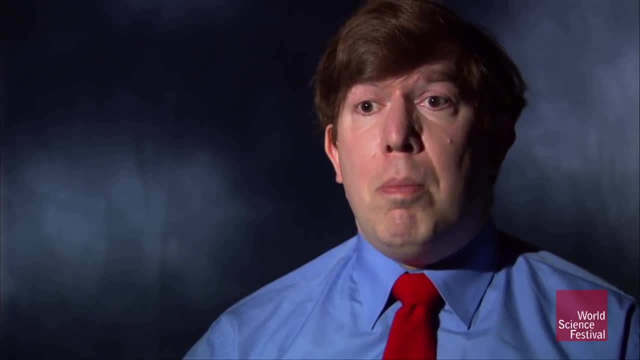 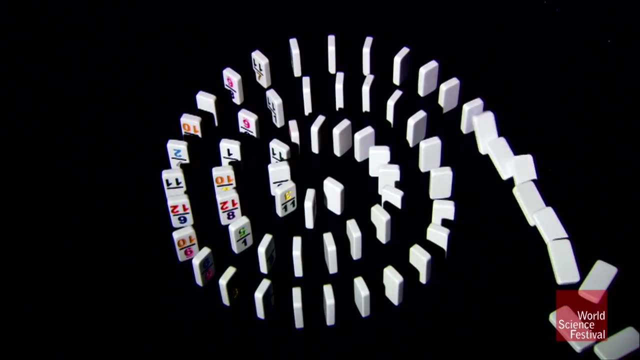 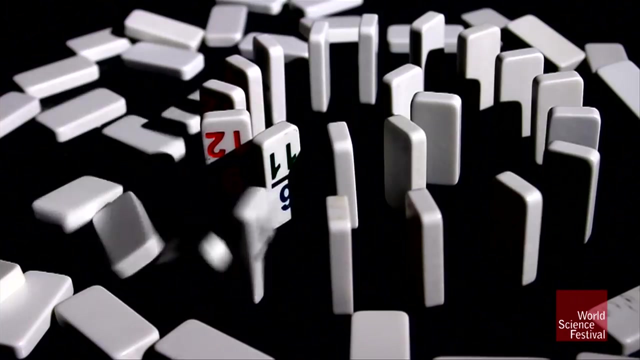 your first child dies of SIDS, the chances of your second child dying of SIDS are much greater. Three women were convicted of murdering their children based upon testimony like this. In the mid-1990s, people suddenly got very scared that NutraSweet aspartame, the sweetener in Diet Coke, was causing brain cancer. 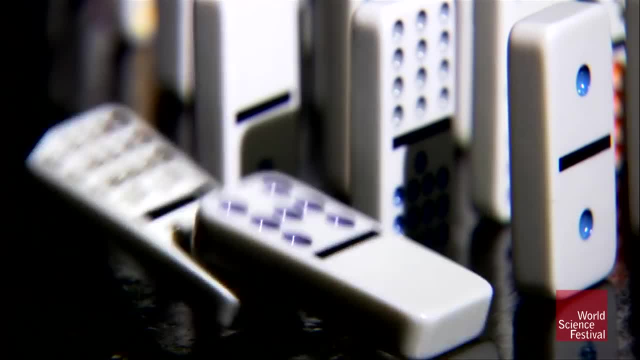 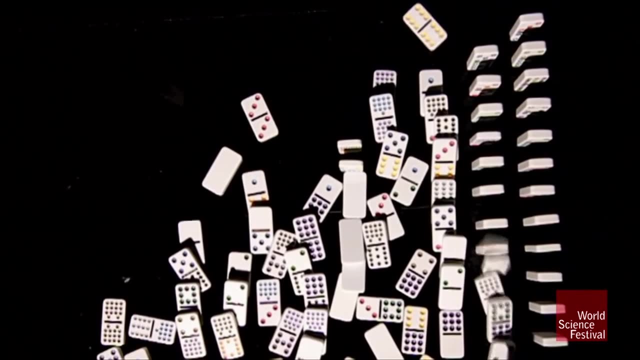 And one of the main lines of evidence was that you had this rise in NutraSweet and the rise in brain cancers from mid-1975 on. So, aha, there must be some connection. Well, in fact, there were a lot of things that tracked at the same time. 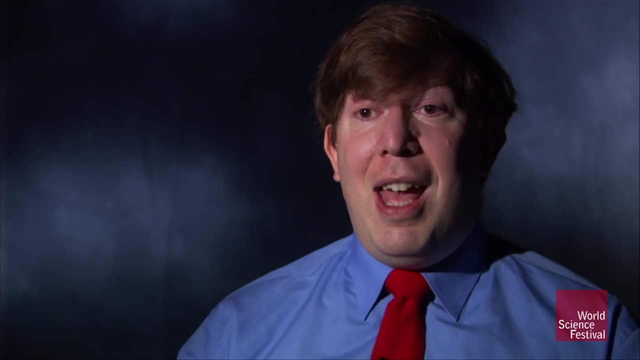 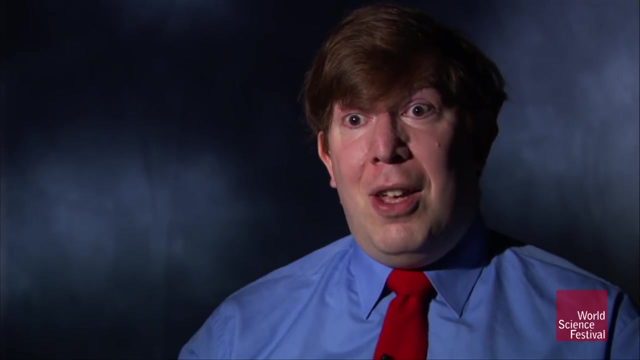 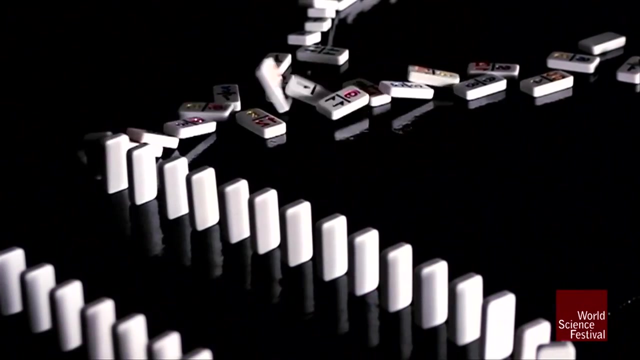 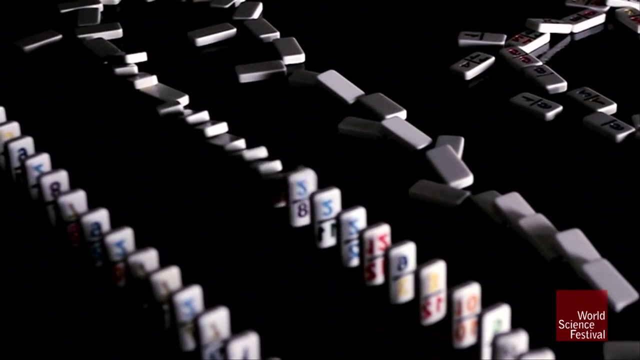 If you look at the budget deficit and how much more we were spending in government than we were taking in on taxes, you saw that brain cancers tracked extremely well With the budget deficit. in fact, the correlation was almost perfect. So just because you see a rise in something associated with a rise in something else, it doesn't mean that the two are related. 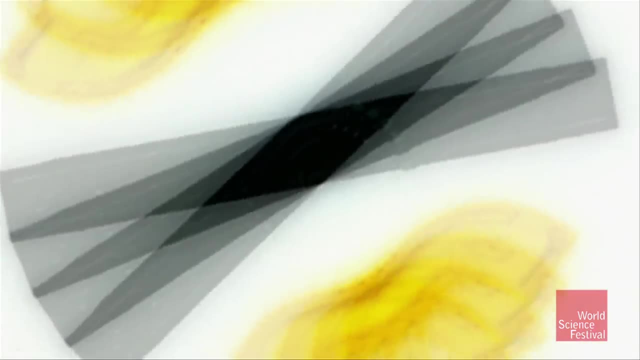 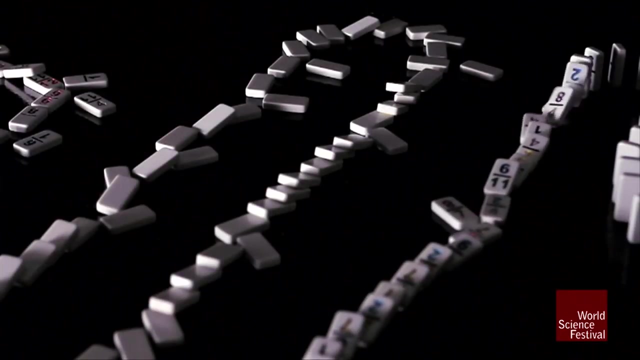 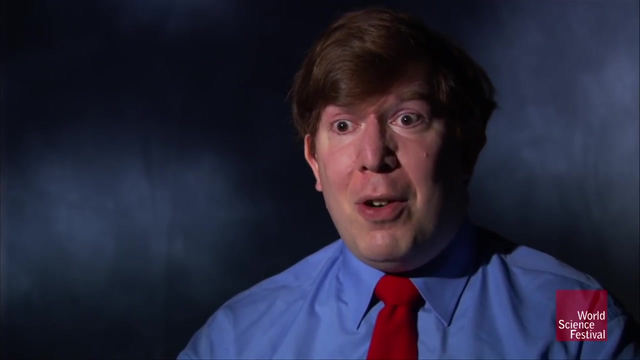 In fact, often it's not the case. If you've got a prosecutor who's looking at fingerprint evidence and saying there's only a one in a million chance that this fingerprint didn't come from the person I want to convict, well, if you're in a city of eight million people, that means on average, 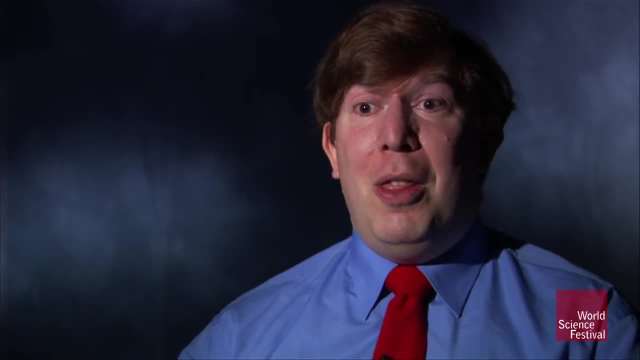 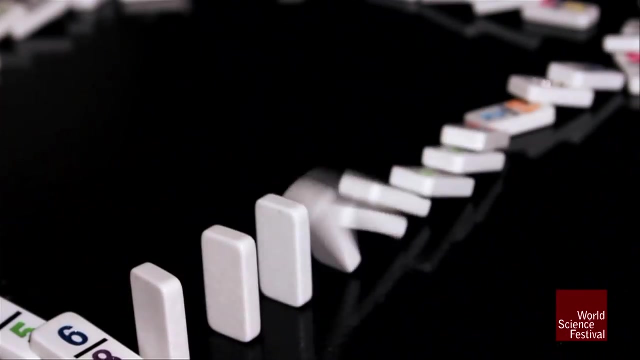 there's eight other people running around the city who the prosecutor could say exactly the same thing about. We do feel safe when there's a number there. It gives us something to grab onto and believe is absolutely true, even if that number has no foundation whatsoever. 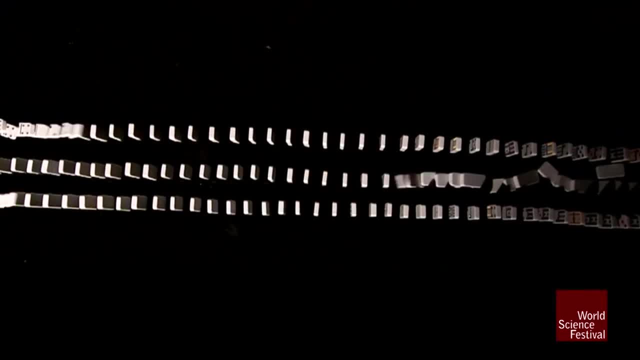 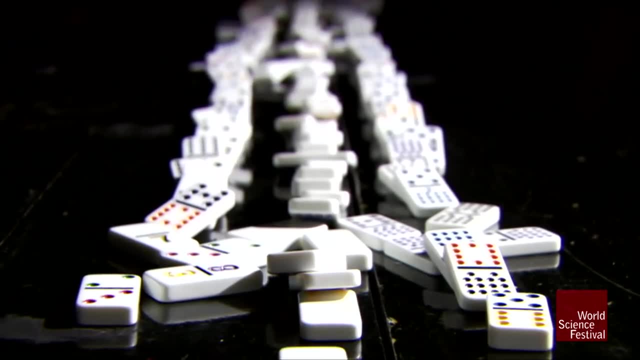 Advertisers know this. This is why four out of five dentists prefer Trident. It's why L'Oreal's Extra Impact Mascara has 12 times more impact. Think about that. Think about that for a second. How do you measure impact? 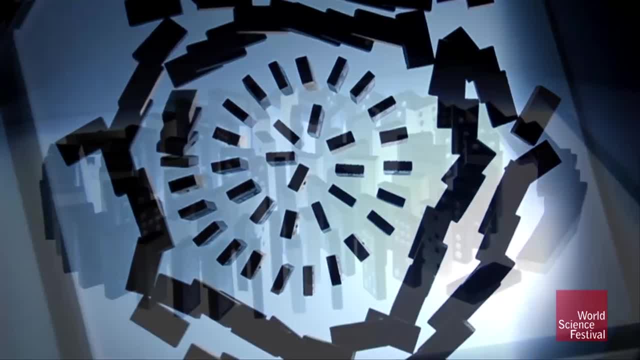 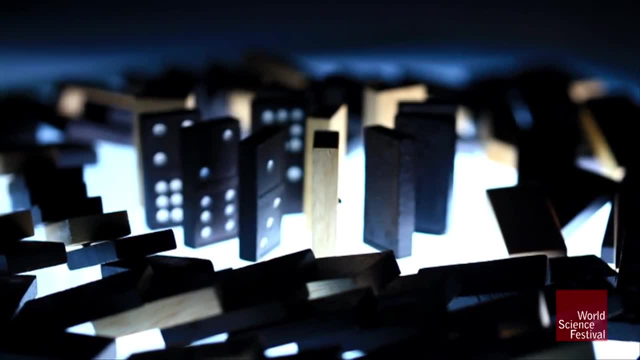 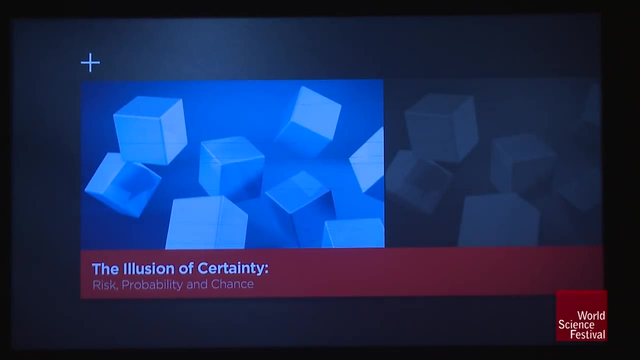 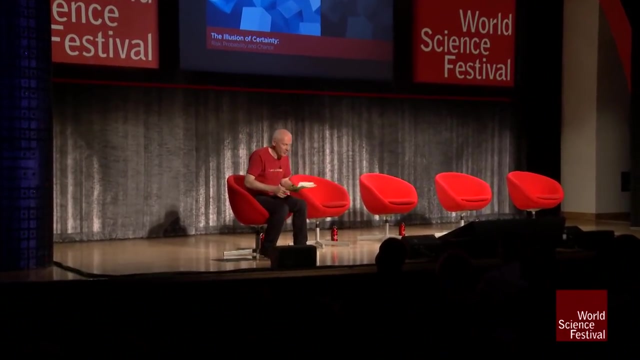 Anytime someone presents something in quantitative form, people will believe you. even though numbers themselves may be perfect, because we are faulty In our hands, numbers can lie. Thank you, Hello, and welcome to this session. The Illusion of Certainty, Risk, Probability and Chance. 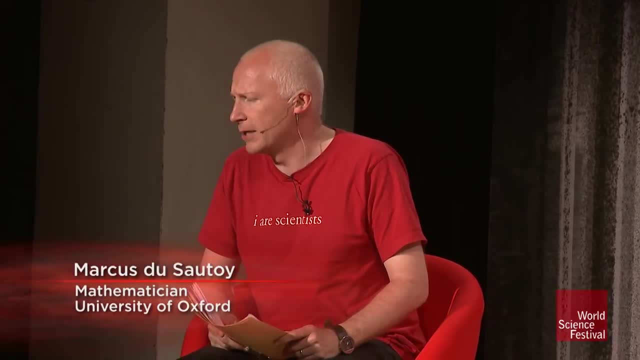 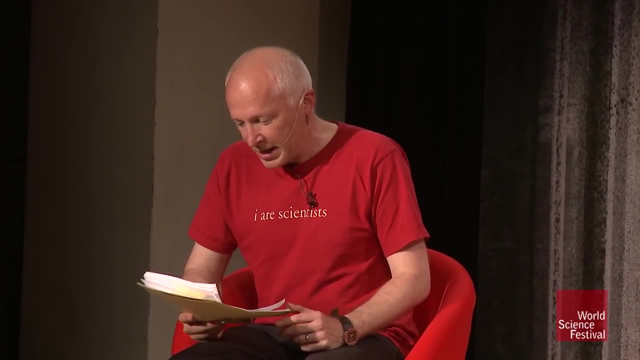 My name's Max de Sautoy and I'm a professor of mathematics, and I succeeded Richard Dawkins as the professor for the public understanding of science at the University of Oxford. To quote the philosopher Ian Hacking, we live in an avalanche of printed numbers. 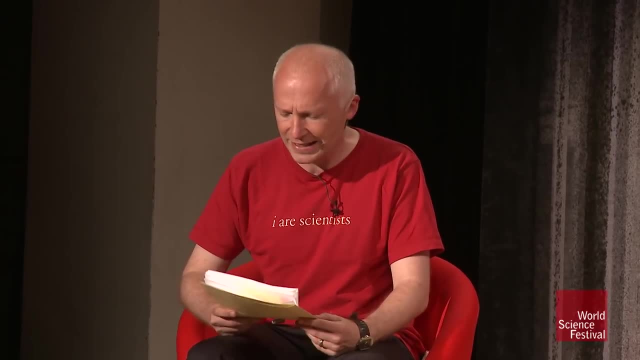 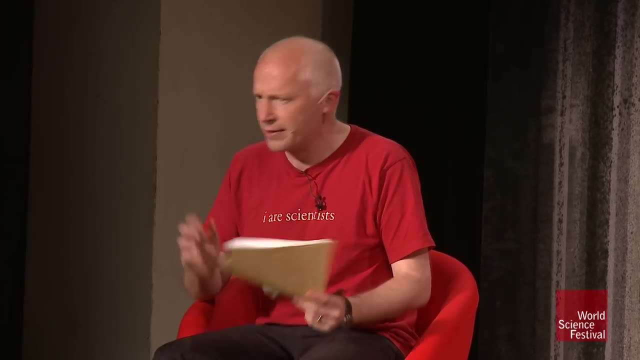 But how can we interpret all the data that we get onslaughted with every day? Tonight, we're going to consider our inner statistician. How good are we at this? How good are we at understanding things like percentages? What is coincidence? Does it really exist? 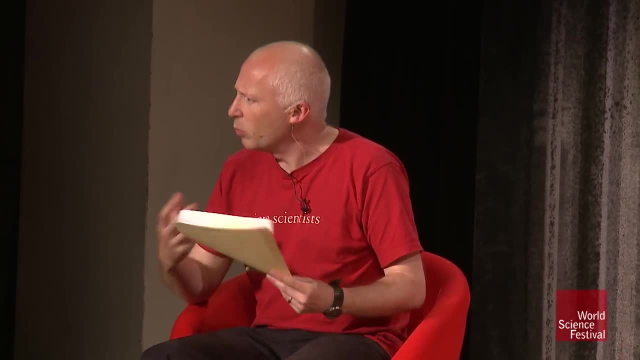 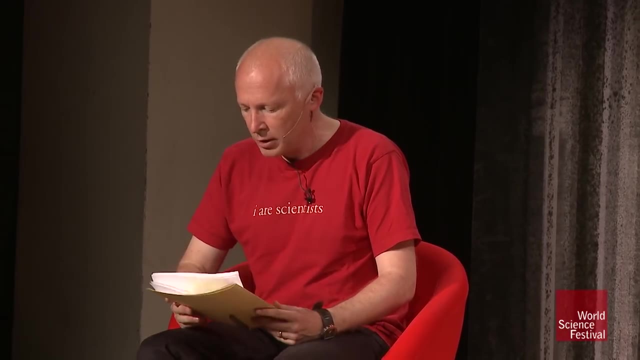 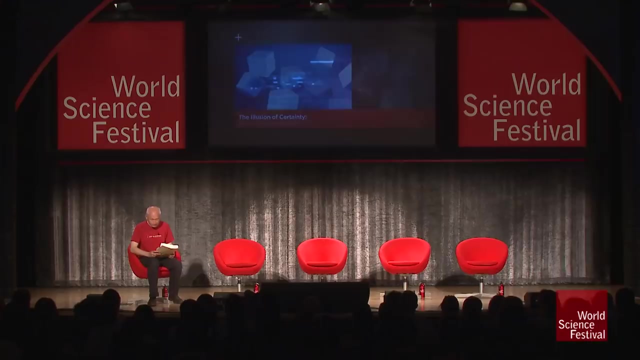 And what sort of numerical information is our brain quite well attuned to understand? And, of course, how trustworthy of a compass is our gut feeling? Well, tonight we've got a fantastic collection of panelists for you, and I'd like to start by introducing Gert Gigerenzer. 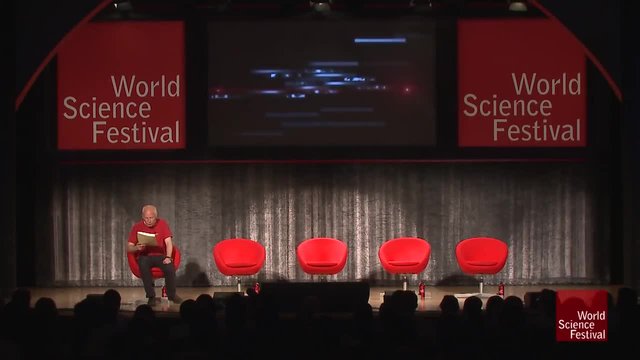 Gert Gigerenzer is a director of the Max Planck Institute for Human Development in Berlin. He's trained US federal judges and physicians in decision-making and understanding risks and uncertainties. He's written the award-winning popular books Calculated Risks. 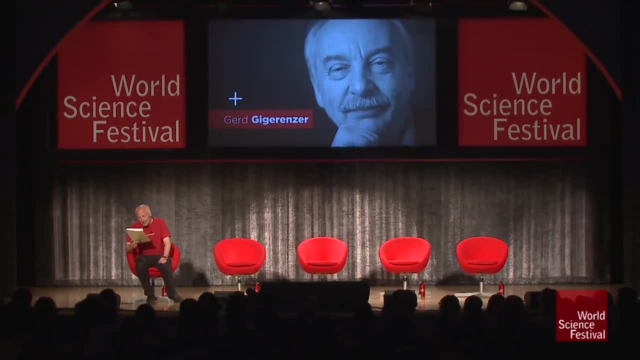 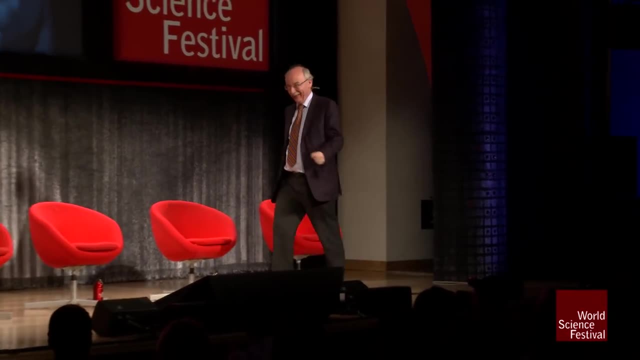 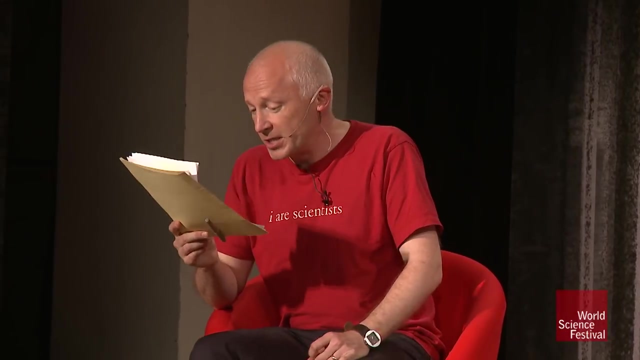 How to Know When Numbers Deceive You and Gut Feelings: The Intelligence of the Unconscious. Gert Gigerenzer, How are you doing? Hi, Welcome. Gert Leonard Mlodinow is a physicist and author. 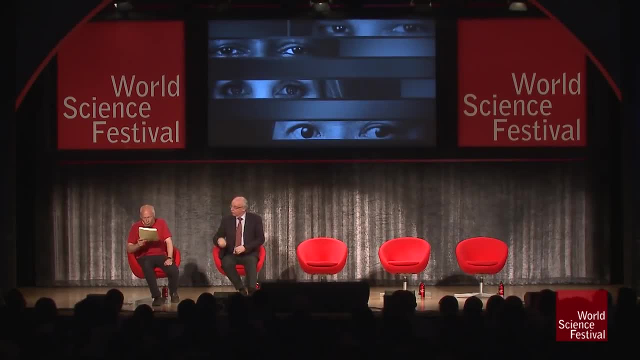 His best-selling book The Drunkard's Walk- How Randomness Rules Our Lives was described as a readable crash course in randomness and statistics, And his upcoming book War of the World Views: Science vs Spirituality will be co-authored with Deepak Chopra. 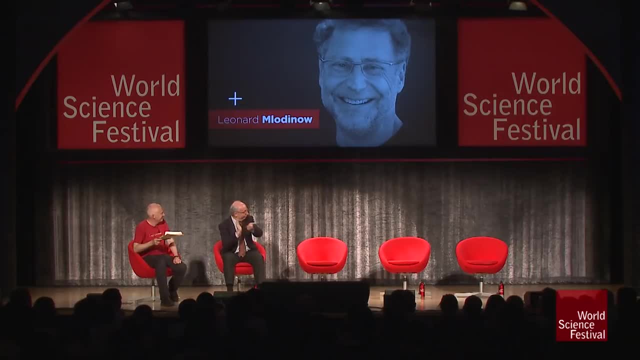 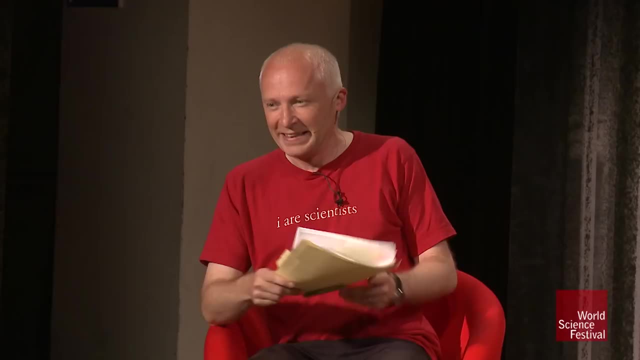 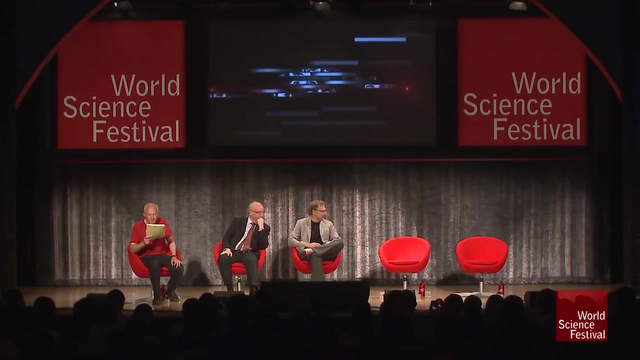 Please welcome Leonard. Now you've already met our third panelist, Josh Tenenbaum. He's a professor of computational cognitive science in the Department of Brain and Cognitive Sciences at MIT. His current work focuses on the nature and origin of people's intuition about the world. 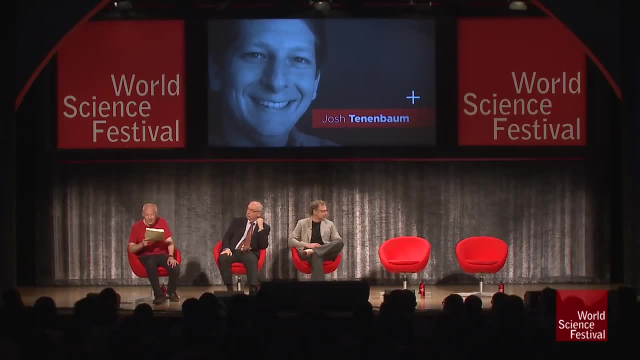 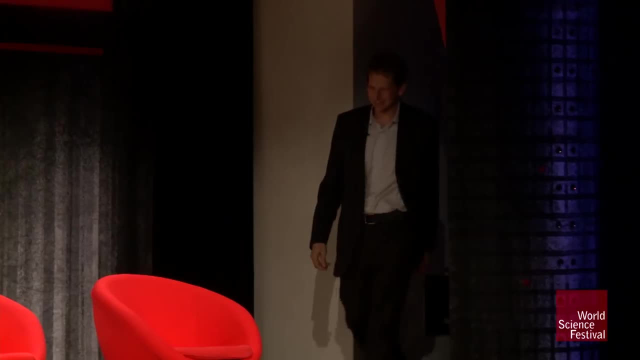 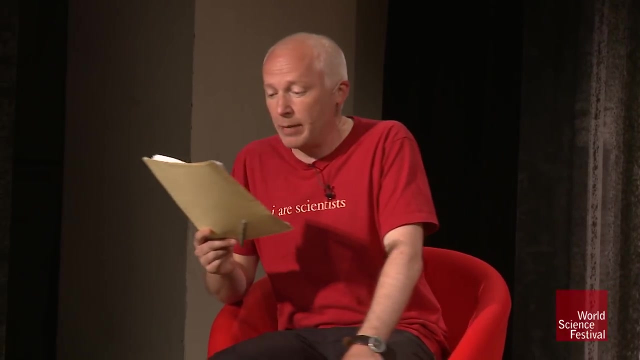 He worries that too much attention is paid to how our minds get things wrong and not enough to how much they get it right. Please welcome back Josh Tenenbaum. And finally, our last panelist, Amir Axel. He's a mathematician and science writer. 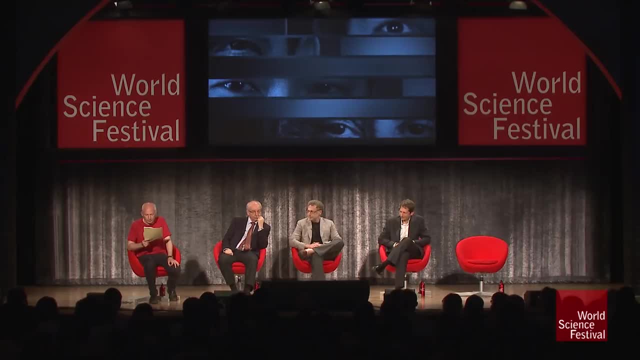 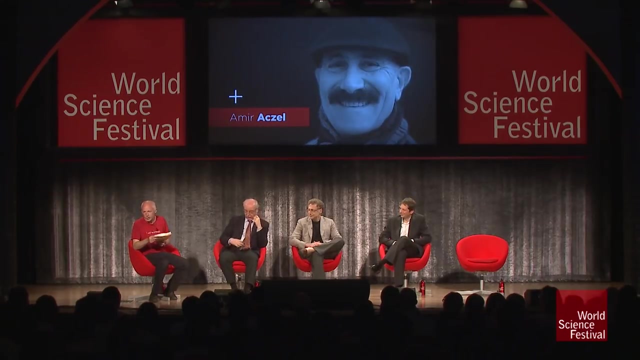 as well as a recently named Guggenheim Fellow. Axel is the author of numerous books, including Chance, described by the New York Times as an edifying and amusing guide to the basic elements of probability theory, And his upcoming book is called A Strange Wilderness: The Lives of the Greatest Mathematicians. 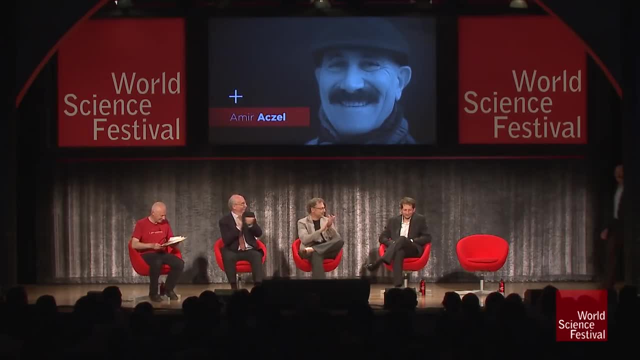 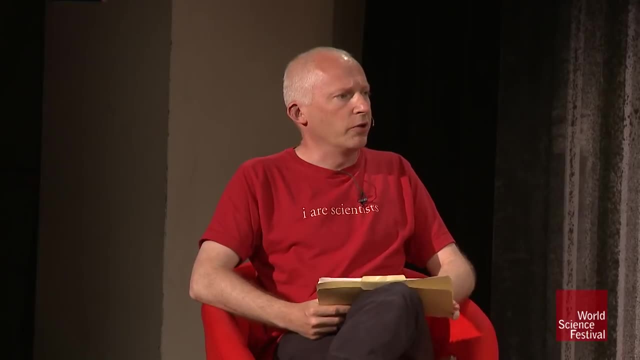 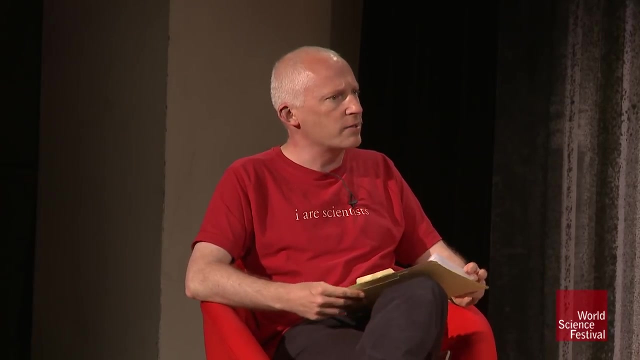 Please welcome Amir Axel. Now I'd like to get us going just with a sort of gut reaction to whether you think that the general public people are good or bad at interpreting data and numbers. Gerd, what's your feeling? Are we good at it or bad? 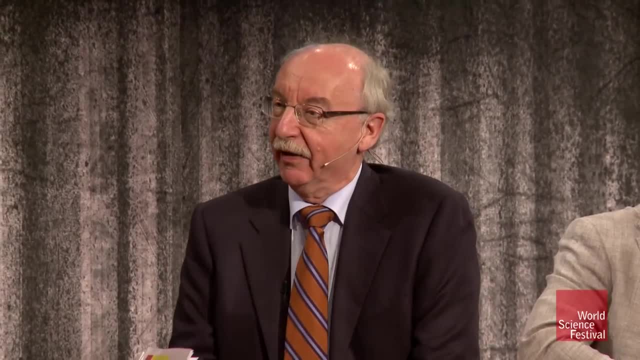 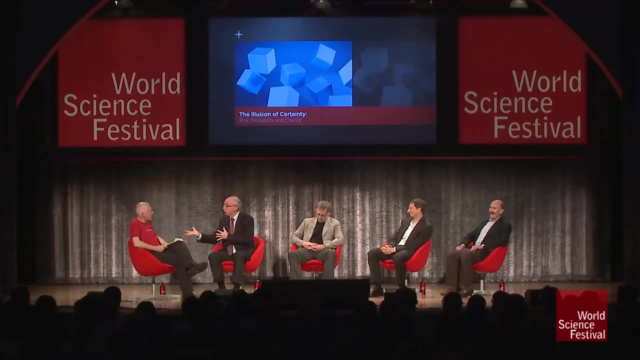 Let me try with you. Do you know what a probability of rain means? So if you hear tomorrow is a 30-day forecast, 30% chance of rain, Do you know 30% of what? Well, exactly Does it mean it's going to rain 30% of the 24 hours. 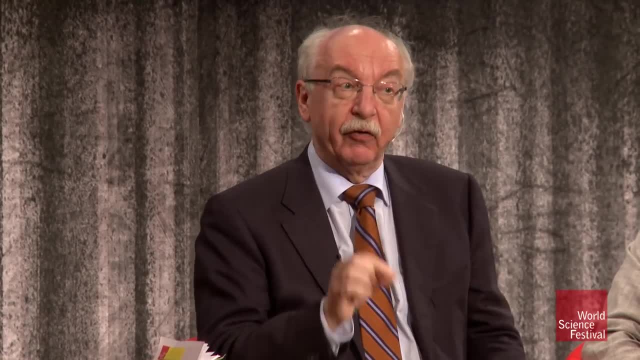 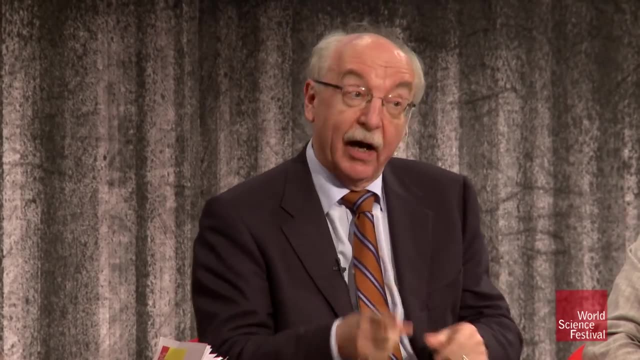 Or does it mean So? I live in Berlin. Most Berliners think it means that it will rain tomorrow in 30% of the time, So seven to eight hours. Others believe it will rain tomorrow in 30% of the region. 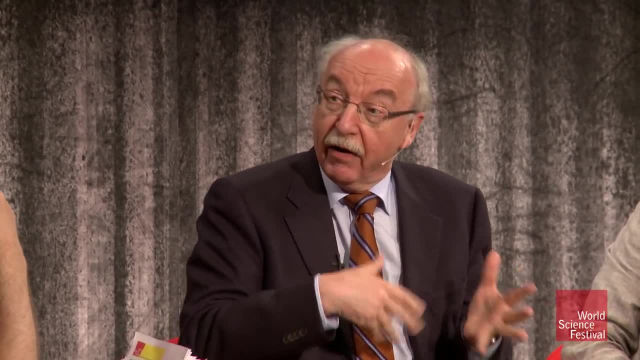 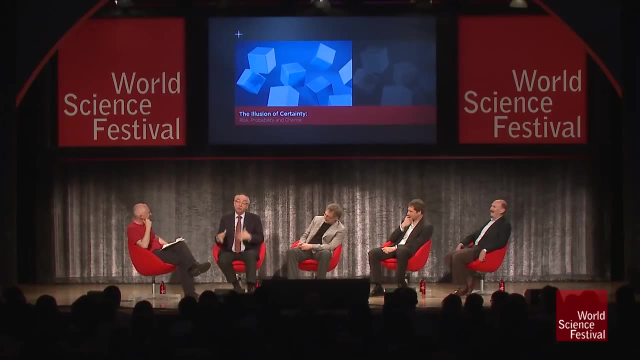 So most likely not where I live. Others believe it will rain in 30% of the days. Most likely not at all. So that illustrates that there's a high variety. But also the problem is not in the people's mind. 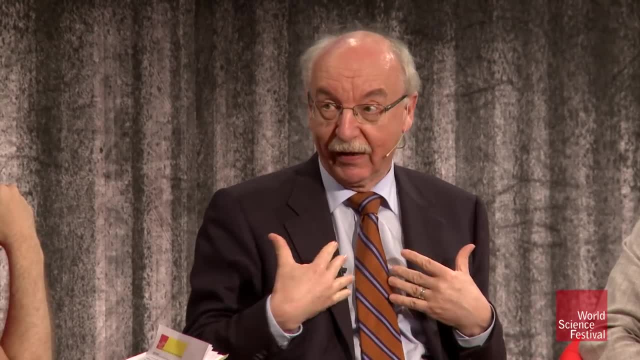 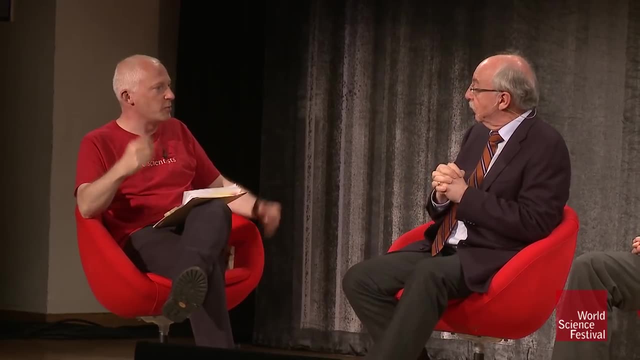 as many psychologists believe, It's in the meteorologists. They don't know how to communicate with it. Yeah, yeah, Well, we don't have this problem in England, because it rains all the time. It's 100%. We all know what that means. 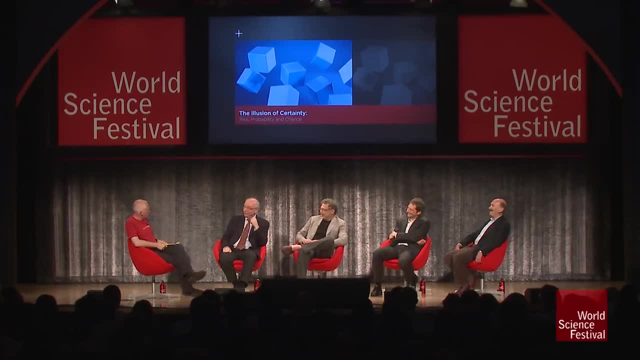 So, Leonard, what's your feeling? Do people? Are we good or bad at data? Well, in Los Angeles, it's very easy to predict the weather. Just say it's going to rain. tomorrow, The weather Just say it's going to be sunny. 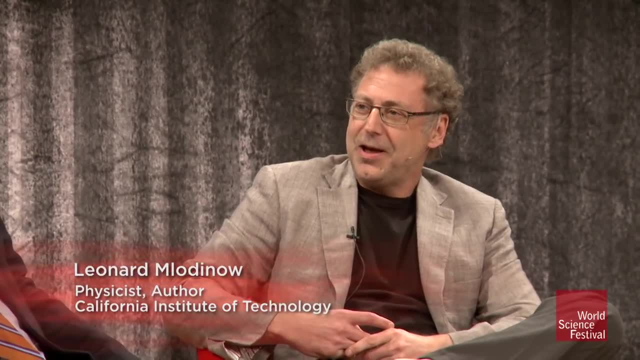 No, no, I went and filmed there recently and we had the only week of rain. It was hopeless. Well, you know. so, when I was a kid, I was interested in meteorology And what turned me off and maybe moved me a little bit more towards physics. 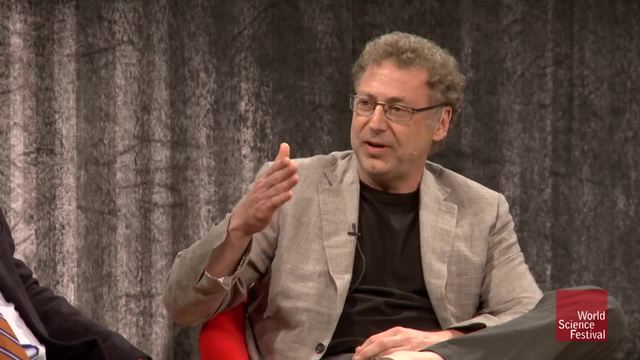 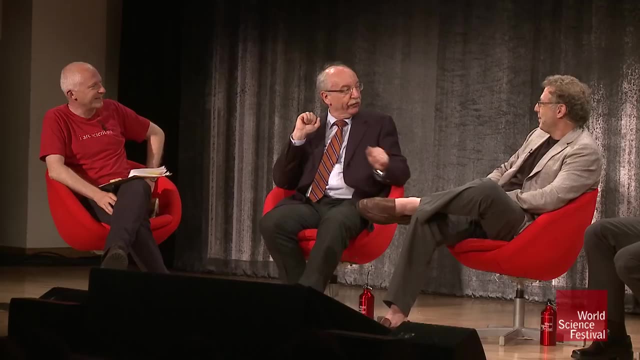 was that I learned that if you predict in Los Angeles that tomorrow will be just like today, you do much better than the meteorologists who are trying to guess what the anomalies are going to be. That's called a heuristic Yes, And that's exactly the point. 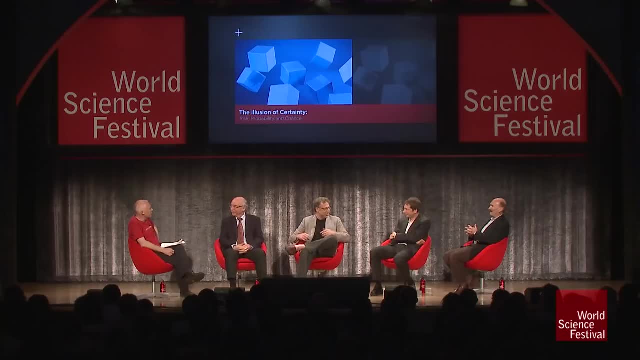 And so people are both good and bad, And I know Josh is going to get on it. Yeah, Josh, what do you think Josh will get on the good part? Yeah, We can talk about the bad part. Yeah, yeah, yeah. 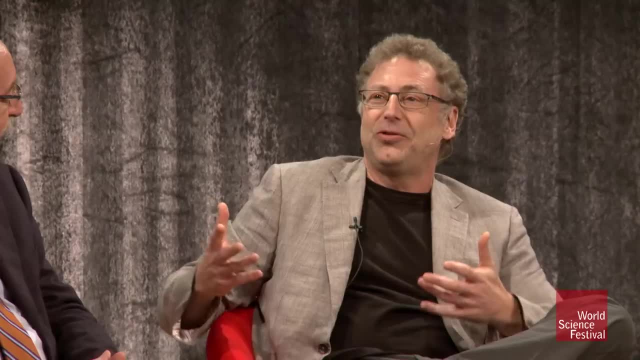 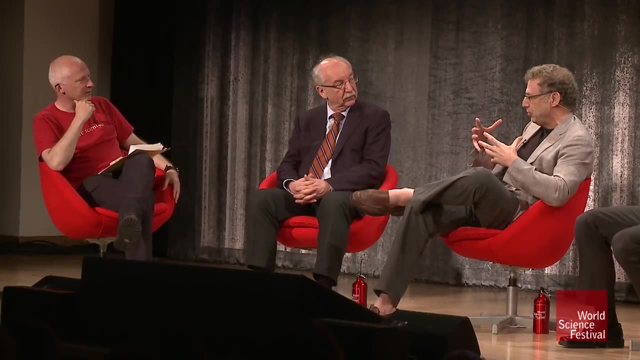 But I just want your gut reactions, because we'll explore it a bit more, you know Right. so So we've got a bad, bad, A bad and good, because what we do is our minds have evolved to treat the world in a certain way. 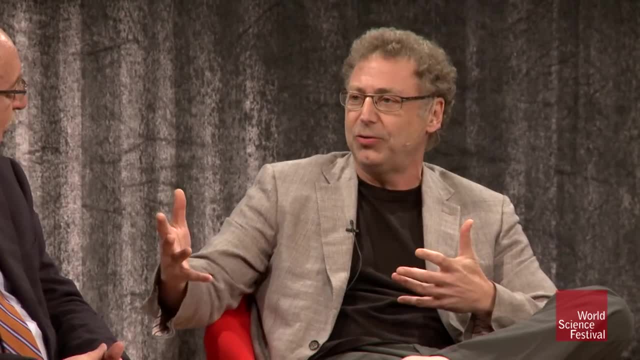 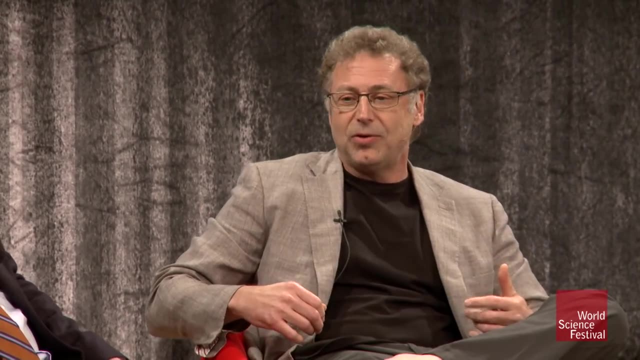 to have certain understanding, certain heuristics where we Shortcuts right. We can't sit down every time we walk outside and go do a probabilistic calculation, We just have to get out of the way of the bus, right. So we have these rules and these heuristics that we live by. 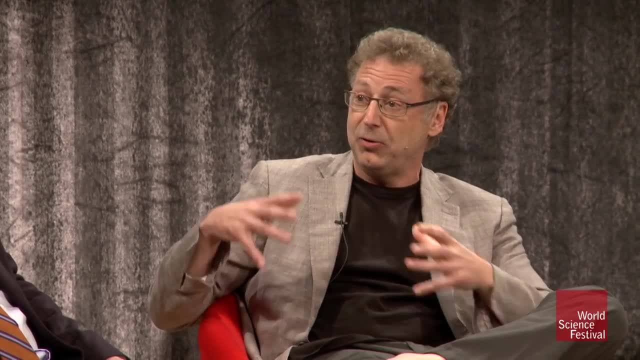 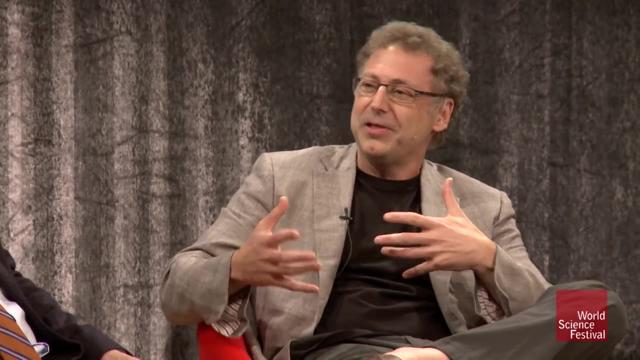 and that we instinctually follow, And, And they're very good in most cases, and sometimes you buy Enron and you're wrong. So So they work and they don't work, and that's why it's interesting. Yeah, Yeah, I would go with good and bad. 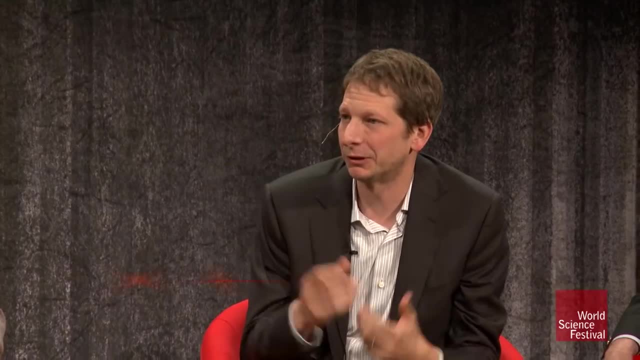 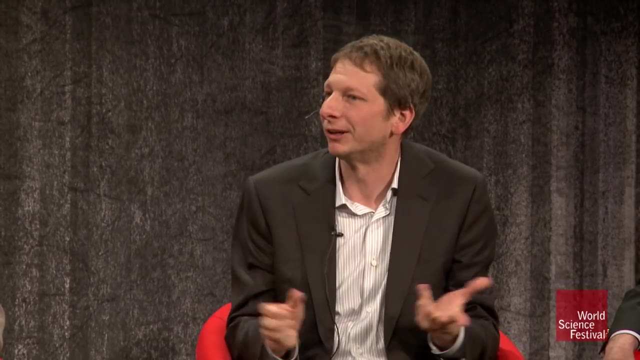 I would say bad or not so good with numbers, but good with data, when you take into account the kind of data our brains are designed for. So my job as a scientist is to figure out how the mind works. I want to understand what makes us smart. 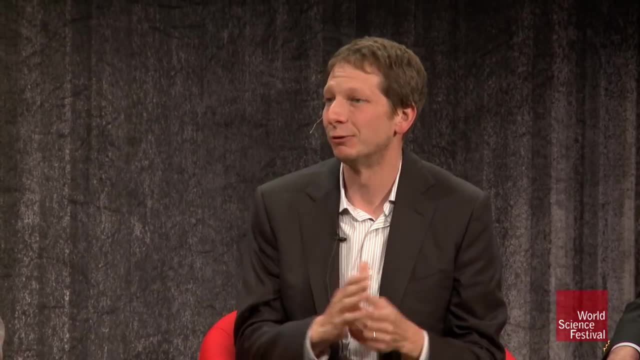 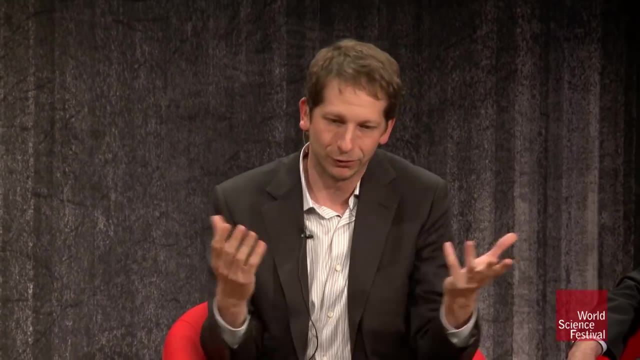 I want to understand why a machine, an artificial intelligence system, has never been built that comes anywhere close to the kind of real intelligence, just common sense understanding of the world that the human mind has, And we think that there's something about how the mind takes data coming in through our senses. 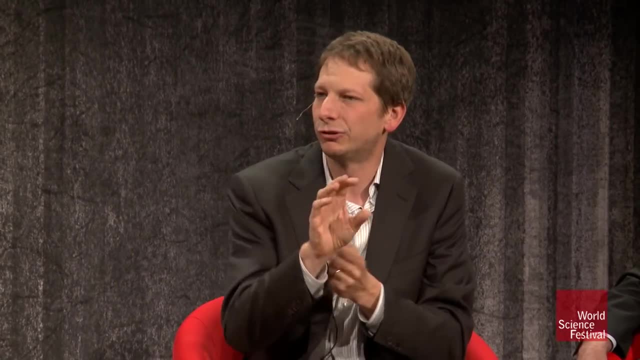 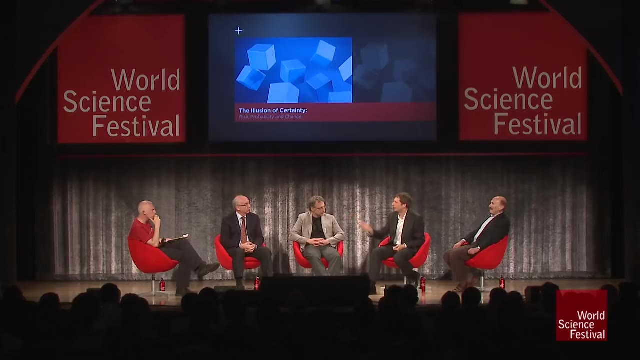 you know our eyes, our ears and so on and finds patterns, finds structure about what's out there in the world. that follows actually some pretty sophisticated statistical inference. you know what you call the kind of statistics in our mind, or probabilistic reasoning. 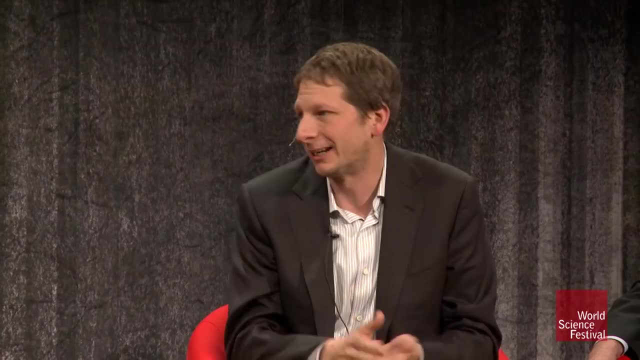 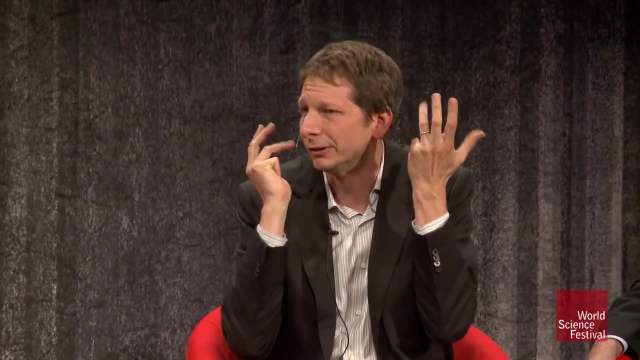 And we want to understand that way that you know, maybe not from the kind of data that you'd read off the stock market tables, but the kind of data that comes in through our visual systems, through our ears, And there I think we're pretty good. 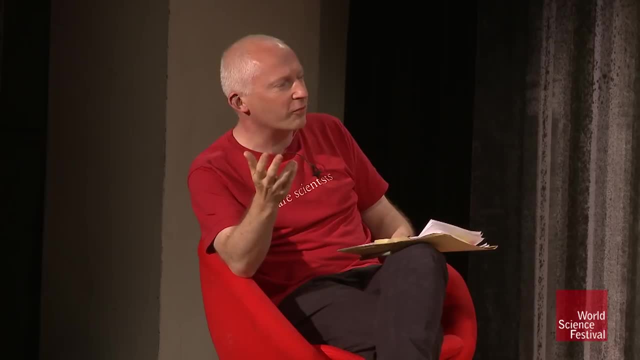 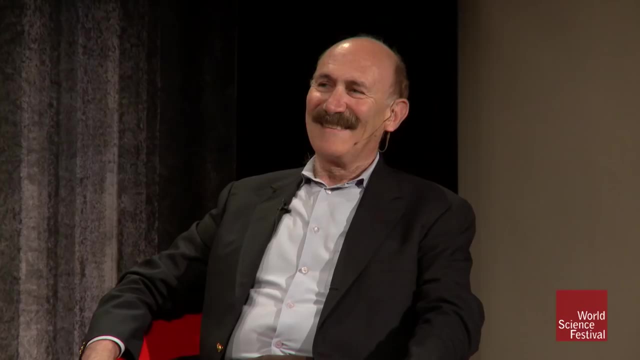 All right, Amir, as a mathematician, you must have that sort of feeling when you go to a party and you say you're a mathematician and everyone always says I'm terrible at maths. I mean, I get so bored of this. 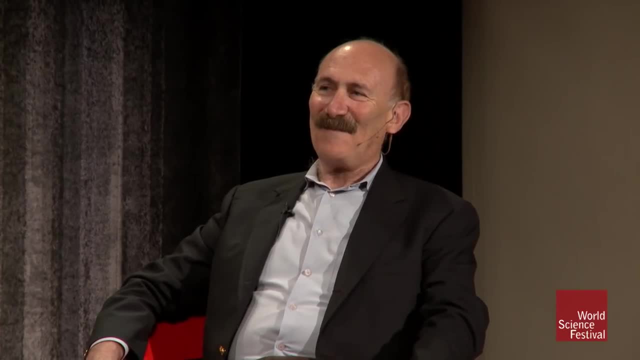 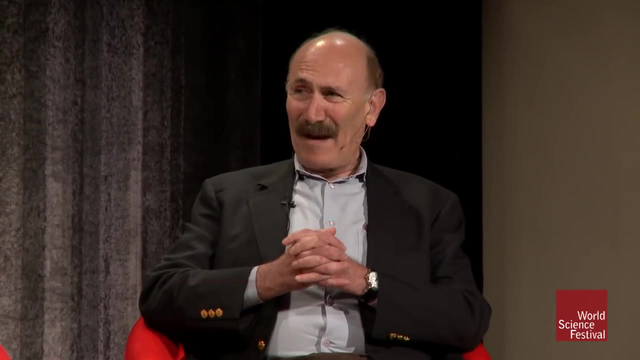 you know, almost being proud, this badge of honor. So do you think that people are really bad at maths and numbers and data? I don't think people are bad with math, but I think we're not hardwired to understand probability for some reason. 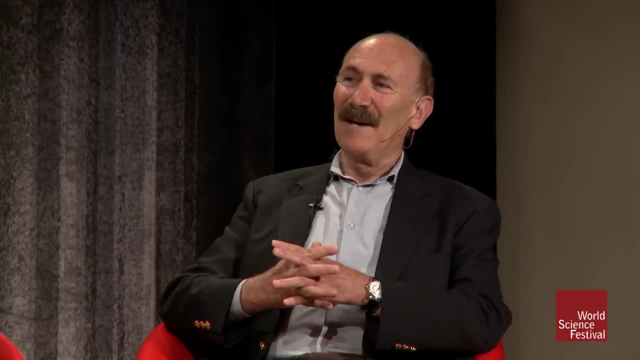 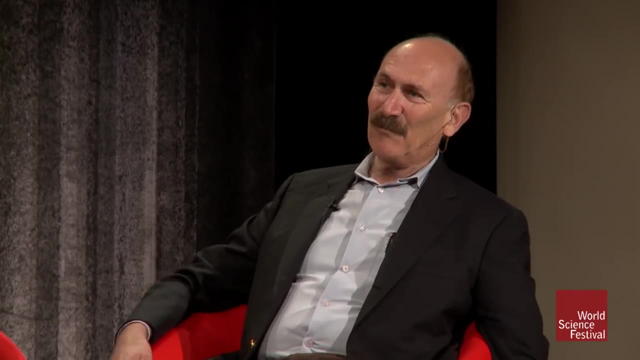 And there have been cases where people with PhDs in mathematics got a probability problem wrong. and that's actually a particular problem that Gerd and I were talking about just a few minutes ago- the famous Monty Hall problem. We have three doors. 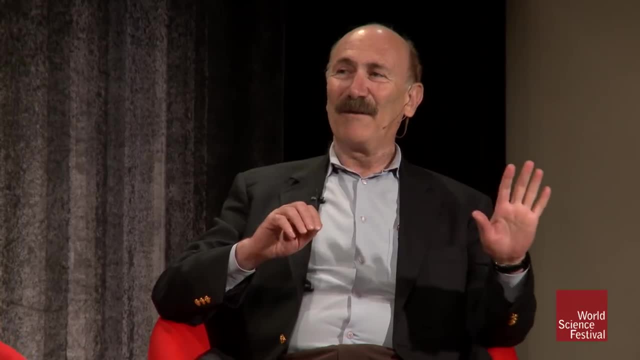 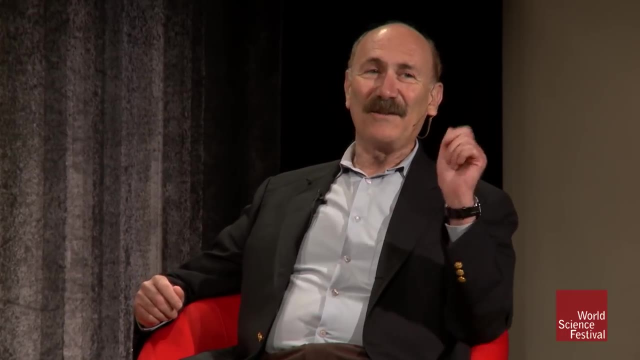 This is an old game on television. Behind one of them there is a car, a goat, behind another one, and the third door, I think, has nothing. The question is, you choose a door and then you know Monty Hall who runs this show. 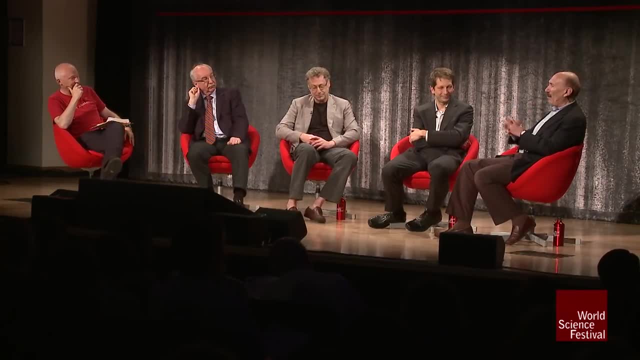 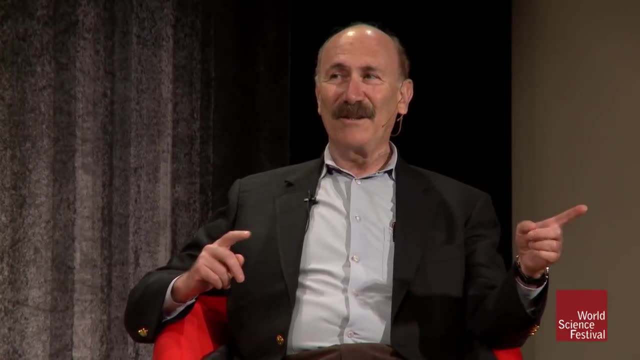 and it was a real show, wasn't it? A real show on television opens one of the other two doors and shows you a goat, And then the question is: do you stick with your answer or do you switch? Well, let's ask the audience that. 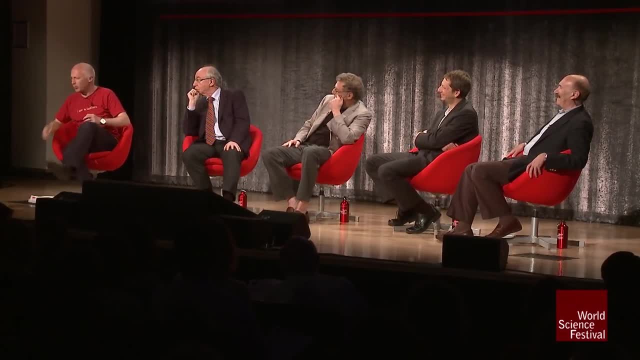 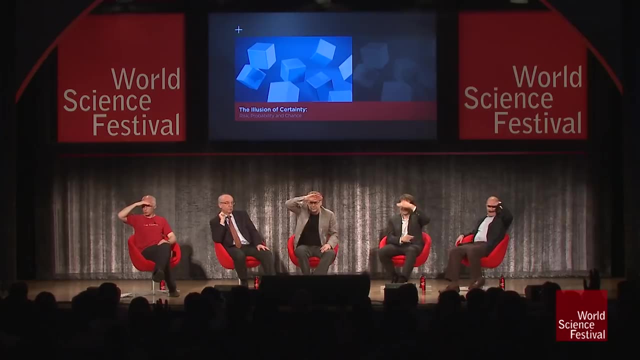 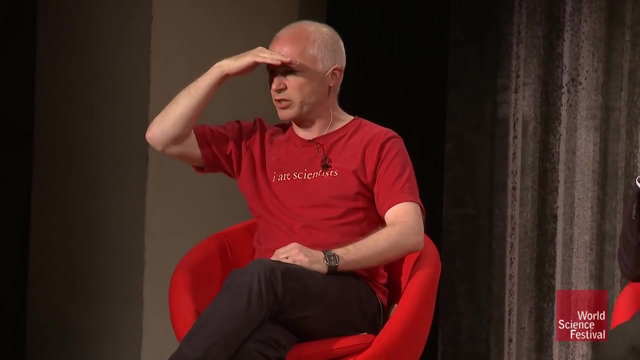 So maybe you're all too well-informed, but perhaps put your hand up if you actually would stick with your first choice. So we've got quite a few hands up. How many people think it doesn't really matter, Perhaps you know. 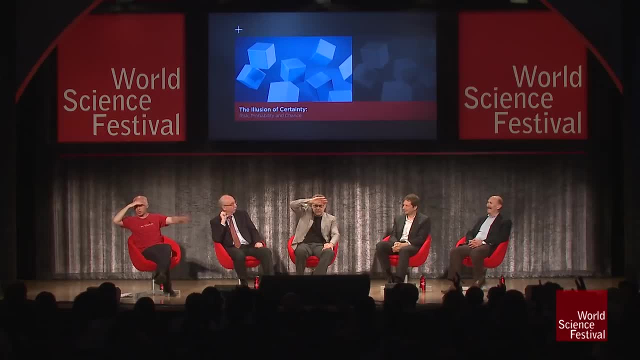 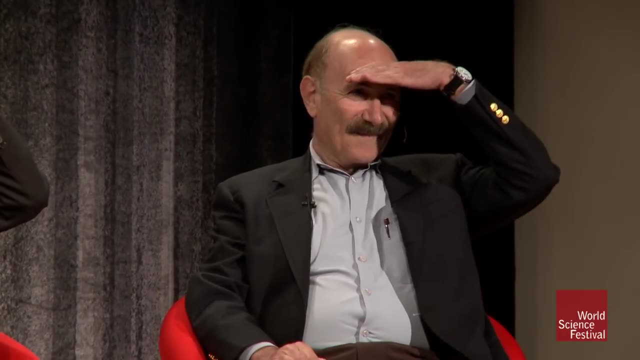 it's now 50-50.. You've got two doors. One's got a car. How many people think it'd actually be better to swap to the other door? Yeah, we've got a too well-informed audience, So most people's intuition. 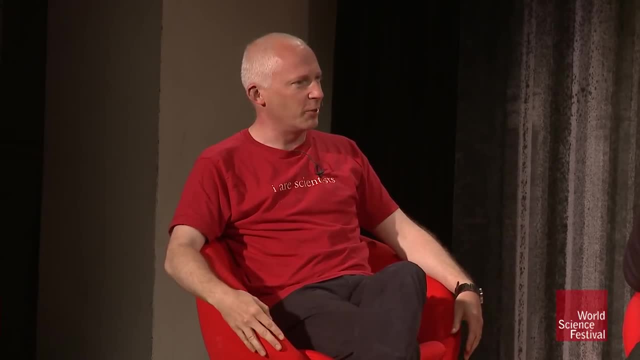 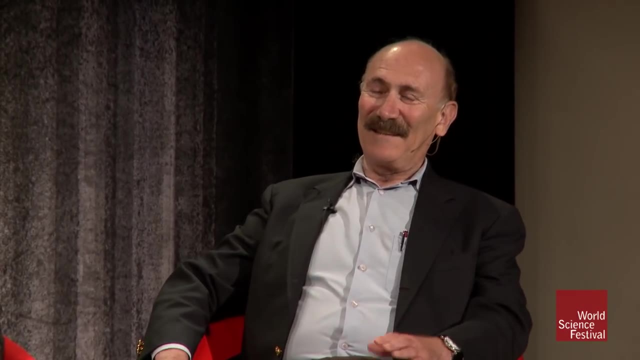 is that it's a 50-50.. It doesn't really matter. I'll kick myself if I swap to the other door. So I'll stick with my first choice. But that's wrong, Right. This appeared in Parade magazine two years ago. 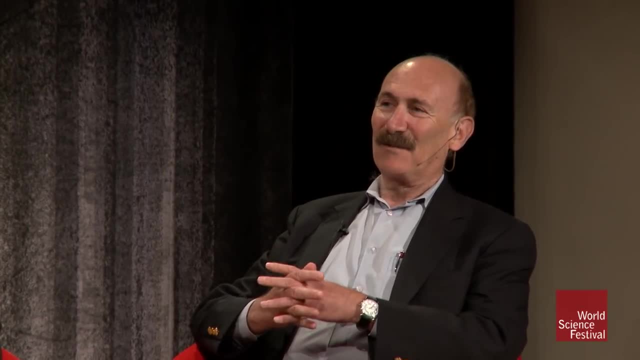 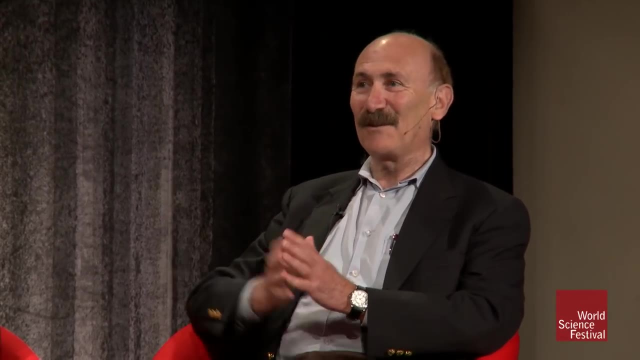 10, 15 years ago And people with PhDs in mathematics wrote complaining about the answer that was published in the paper And of course they had to be very embarrassed because you should switch. Are you going to tell Paul Erdos' story? 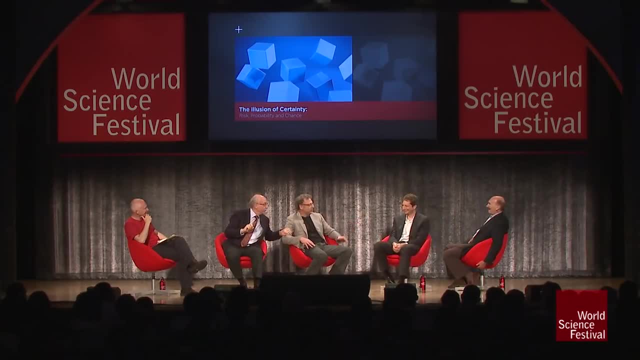 Go ahead and tell it No. no, I just want to make sure you do. Paul Erdos was a very famous and brilliant mathematician And you could not accept this. He had a hard time with this problem and he didn't believe it. 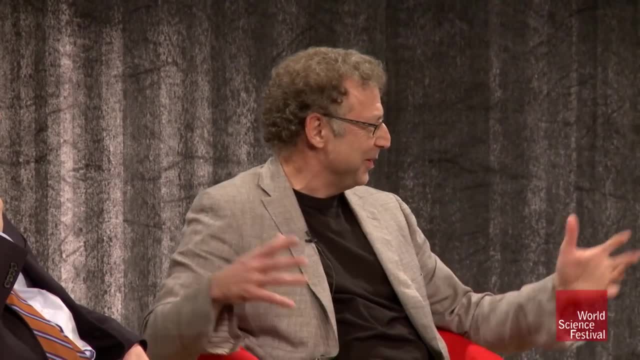 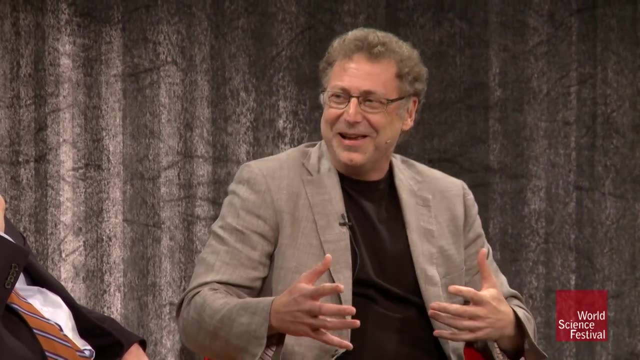 And what's interesting to me and mathematicians will probably- I mean the only time in history that he was finally convinced, when they did a computer simulation and he saw how it came out. And it's the only time I would hear of a mathematician. 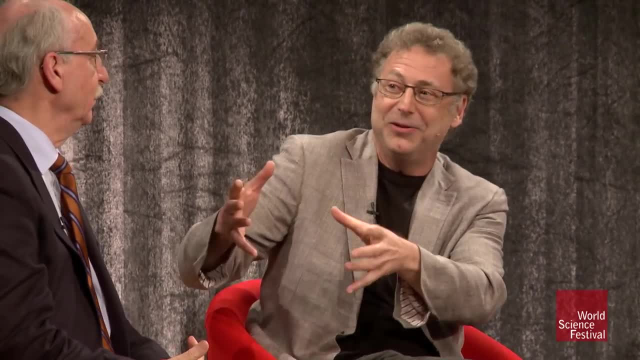 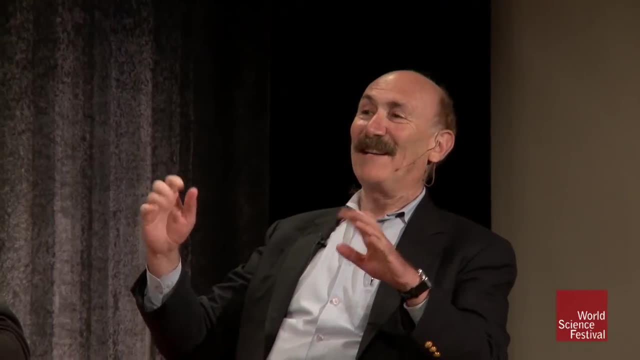 trusting a computer simulation and not the proof using Bayes' theorem. Yeah, yeah. So, Amer, I guess you're saying that mathematicians were also not terribly good. necessarily Right, You have to be trained in probability in order. it's like quantum mechanics. 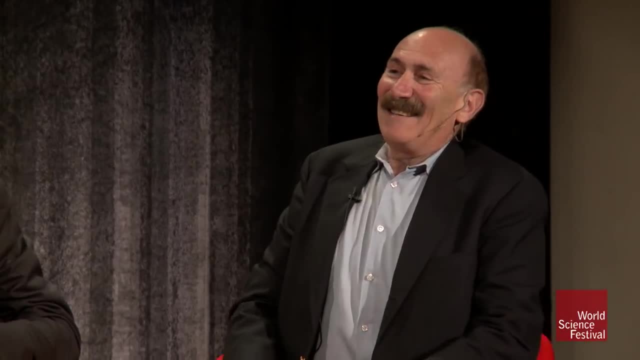 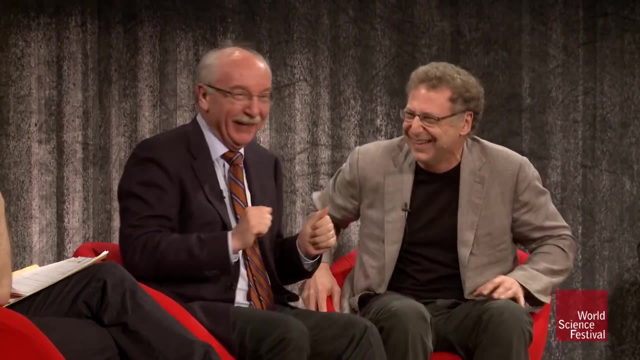 Even if he was Right, I disagree. Right, I disagree. Don't be fooled with what they're telling you. Now. look, Chances are. you're wrong. Yeah, And you too. So the solution that you should switch: 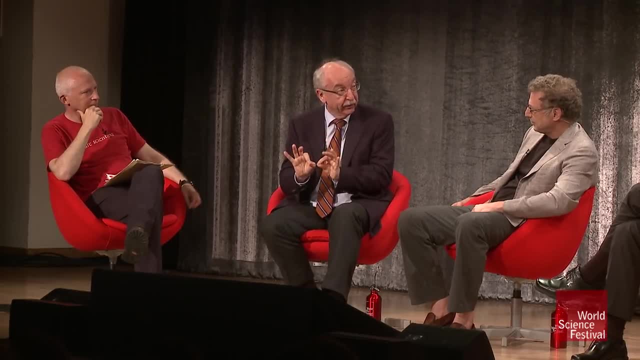 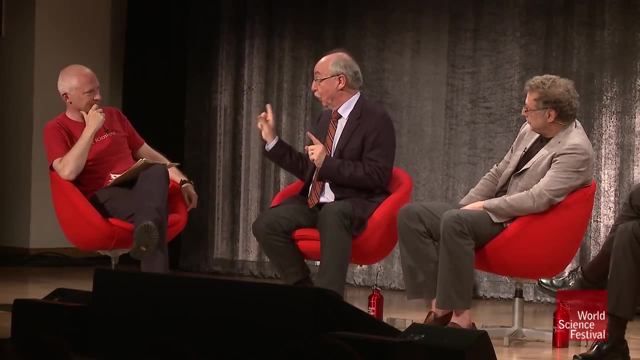 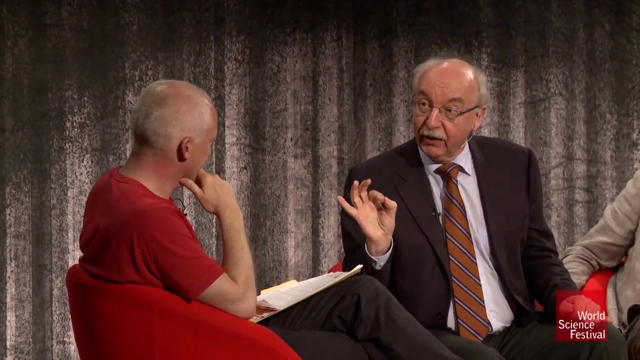 is correct, if the assumptions are correct, The assumption is that Monty always offers this, Or at least randomly, independent of whether you are in front of the right door. Assume Monty is a mischief, as Monty only offers you the choice if you're standing in front of the door. 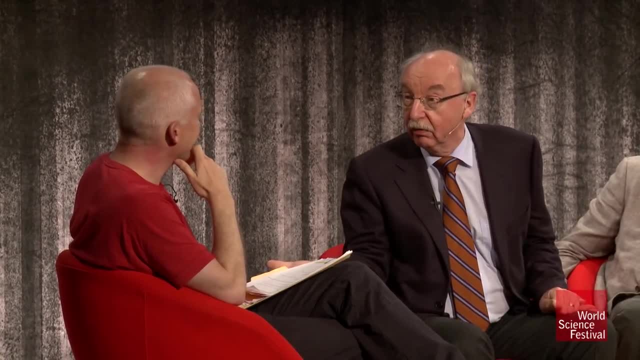 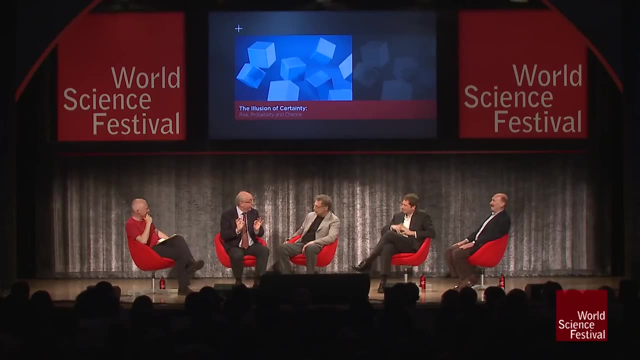 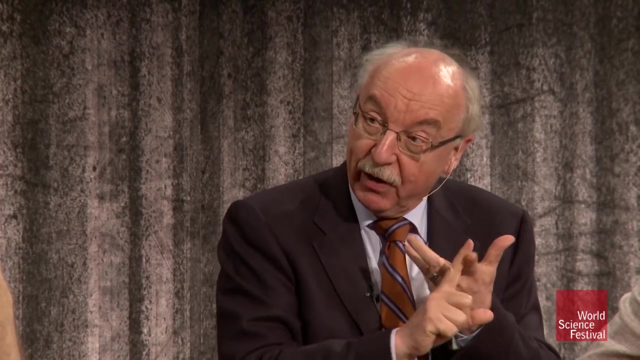 where the Cadillac is. yeah, Then you always get it wrong, So that's not a good strategy. So the key question is: did in the real show, Monty always offer this possibility? Answer: no, And actually Monty was asked about it. 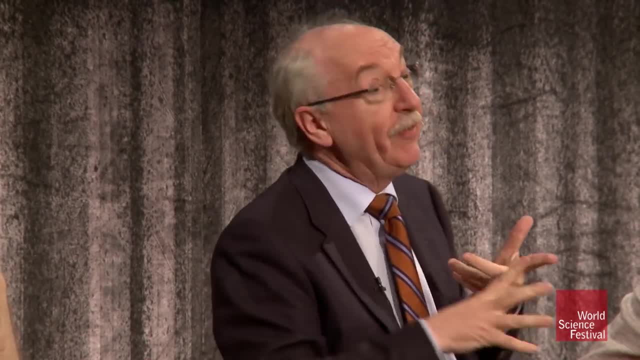 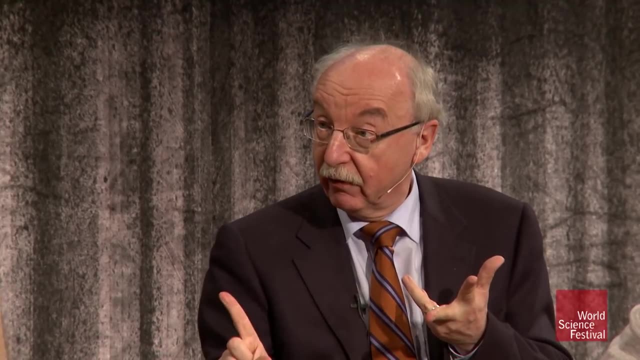 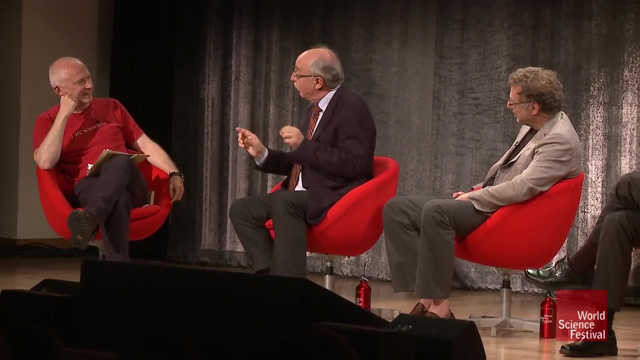 his assistant and the producer. So Monty said he sometimes offered it, but when he had a gut feeling. The producer said he never offered that choice And the assistant said yeah, sometimes he did, but nobody knows when. So here we have the real problem. 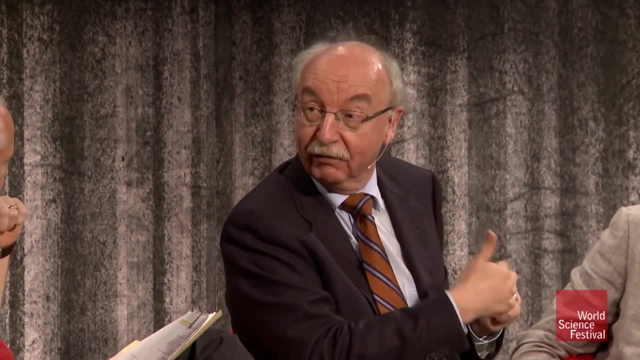 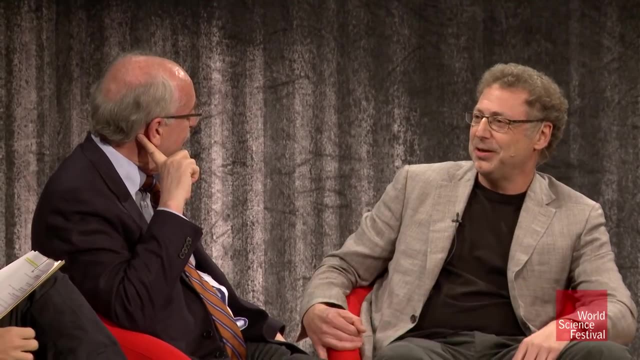 It's about uncertainty, not about calculated risk. Well, we're going to come back a little bit to The problem was presented to people, though it's presented in a certain way with the assumptions Right, And so it's not what actually happened in the show. 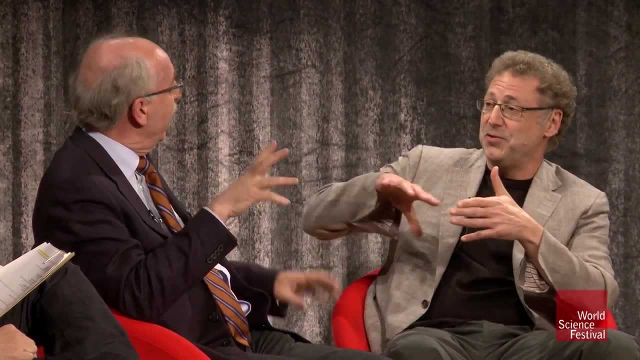 But I do think they analyzed the statistics from the show, If you. Anyway, we don't want to go too far. By the way, there was a book someone wrote recently on the Monty Hall problem, So look it up on Google. 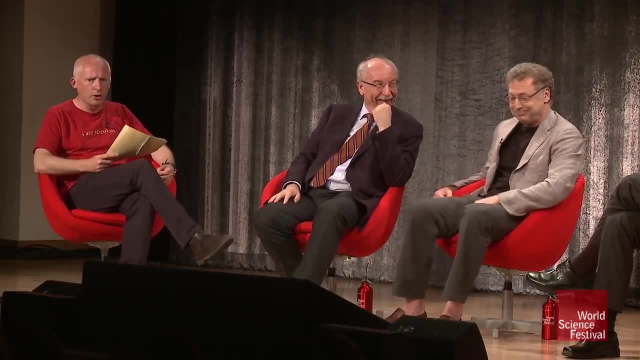 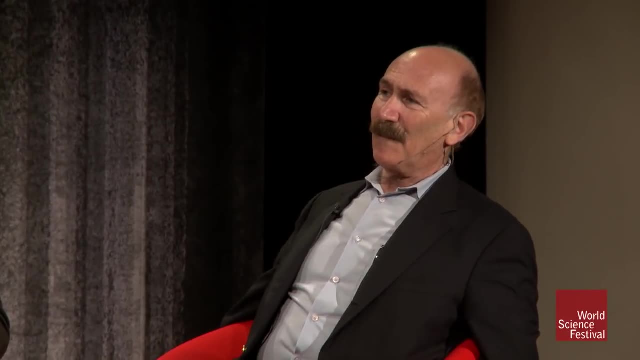 Let's come back to probability in a minute, because in some sense It's an abstract problem that has actually many other possibilities. The three-prisoner problem also. Well, there was a. They applied that. If you go on the Google and you 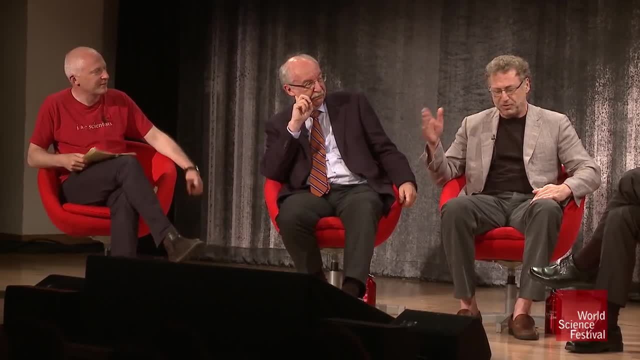 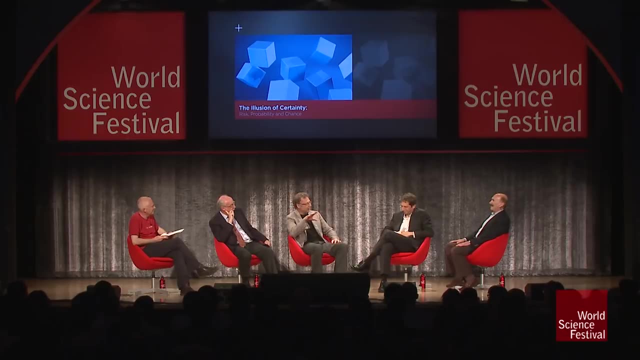 There was a very interesting article a few years ago where they show that psychologists were doing experiments that were equivalent to the Monty Hall problem- misinterpreting the data. So if you look on Google you can probably type in psychology experiment, Monty Hall. 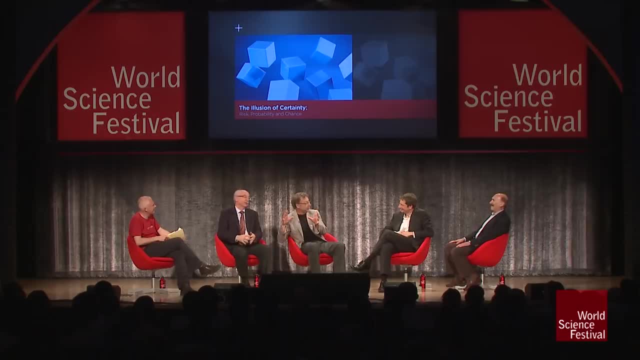 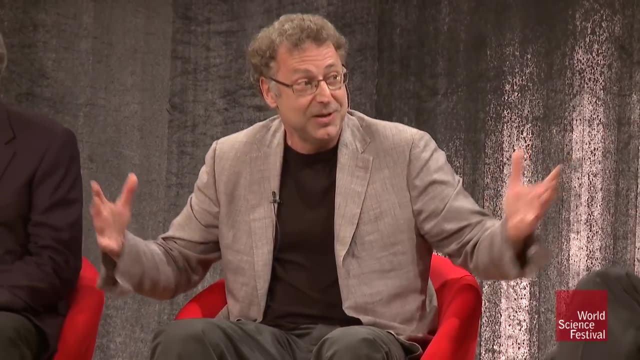 You'll find that there was an expose written of all these experiments that were statistically analyzed incorrectly because they misunderstood what they were doing in terms of the same idea of the Monty Hall problem. Right, Let's come back to probability a little bit later. 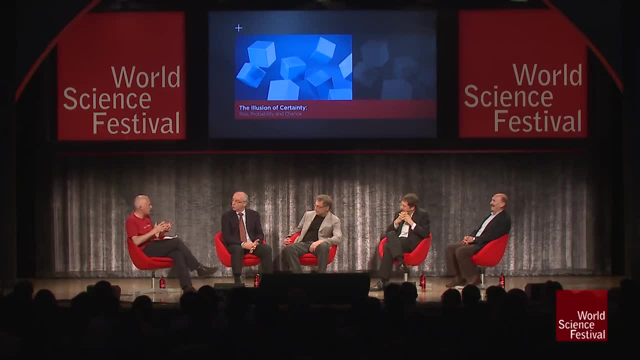 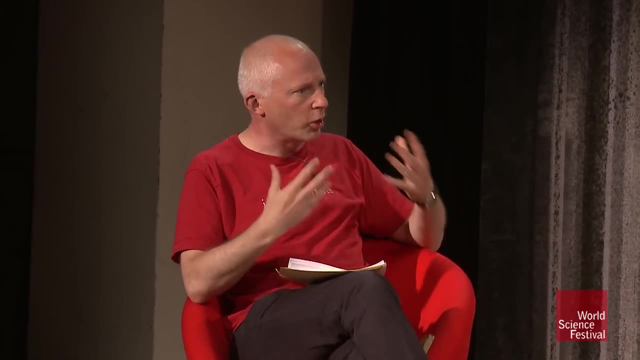 because I think, before we even deal with probability, we have just the issue of interpreting the world with numbers. I mean, I think that we've seen in the introduction a lot of the ways that we tried to navigate the world with numbers. I mean, do you think that it's you know? 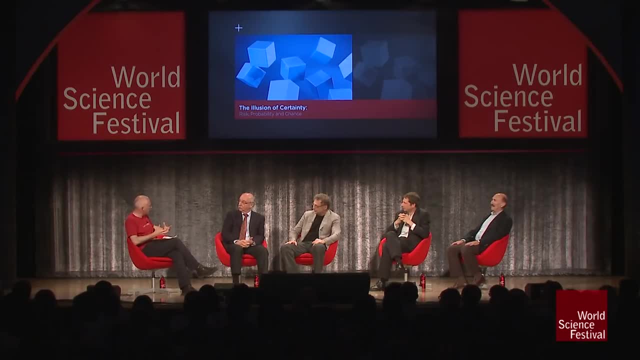 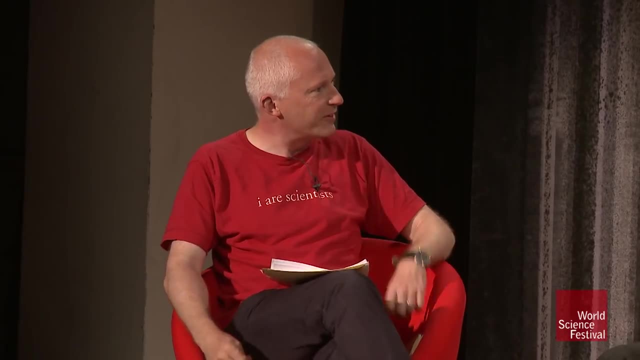 the right way to interpret the world. How powerful are numbers in actually trying to work out the way the world works and navigate our way around it? Good, I mean, are numbers important for sort of assessing medical things? I mean, why should? 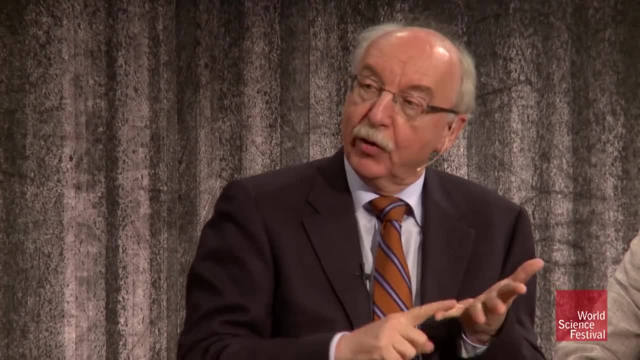 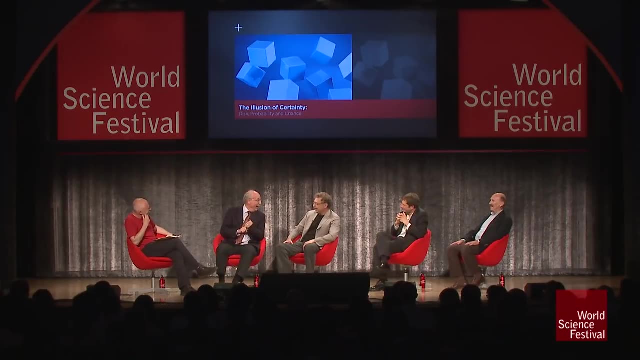 Oh, of course. Yeah, So there's the term evidence-based medicine. Isn't that strange? If there would be evidence-based physics, you would wonder: Well, it's not as bad as evidence-based education Doesn't exist. I mean here: 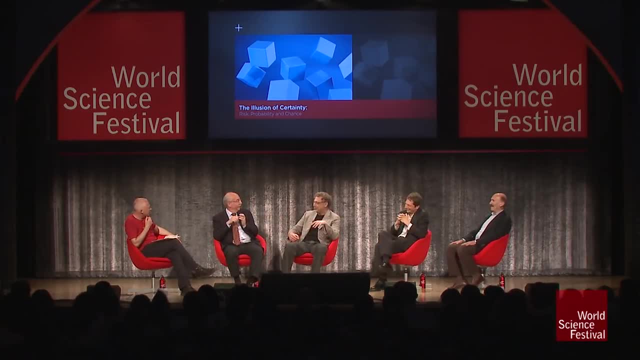 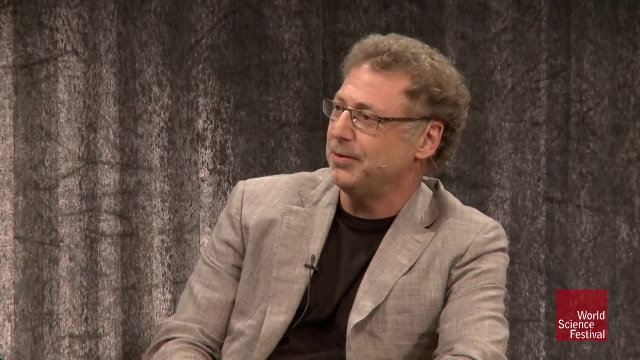 because there's a lot of education, big education community, and I question some of their evidence and their studies. So sometimes you have to be careful over-interpreting numbers and trying to quantify everything. Yeah, That's true. Yeah. 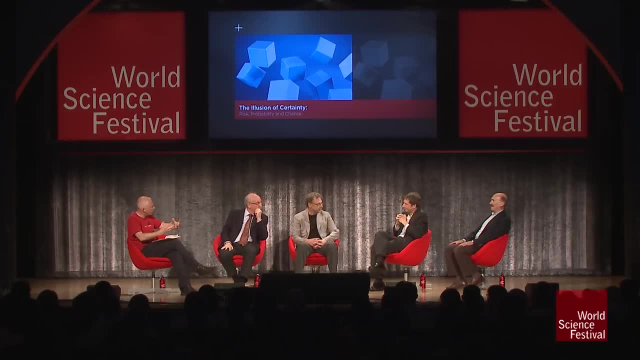 I mean because, Josh, you were in some sense saying at the beginning that perhaps numbers aren't the right way, that it's other ways that we interpret the world, visual or oral. Yeah, I mean a number of us. 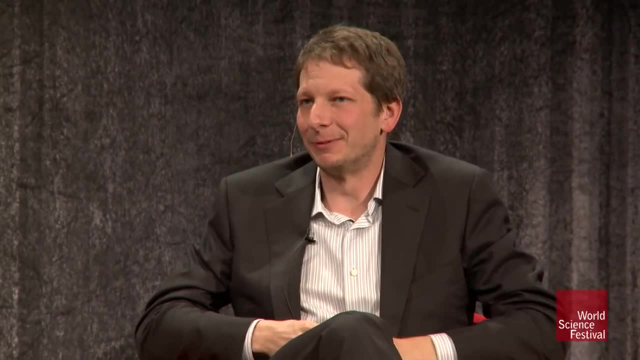 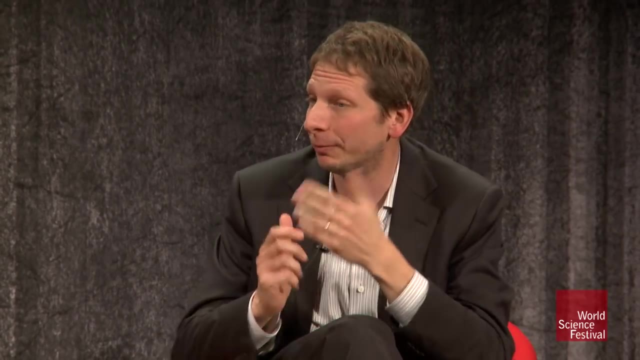 have looked at cases where the A number of you have. Okay, Well, you can present the very same data as a table of numbers or, you know, as a diagram, for example. Often, what makes a good diagram in a scientific paper? 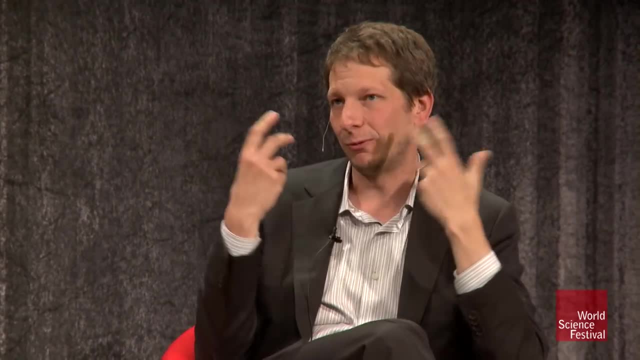 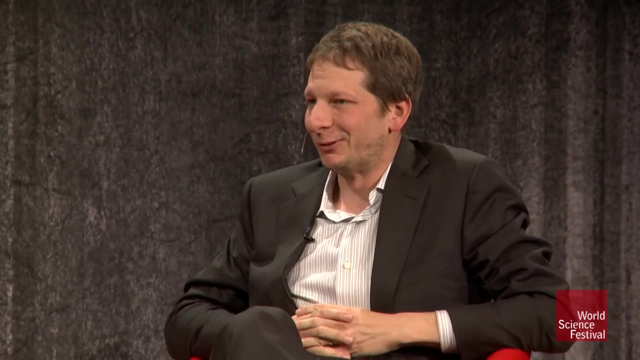 or when scientists are analyzing things, is something that appeals to the way that our brains are actually designed to process data. again coming into the senses The Yeah, I don't know if you We have a slide on this. We'll come back to it. 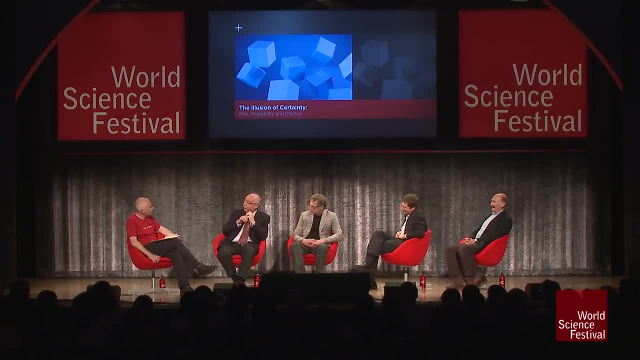 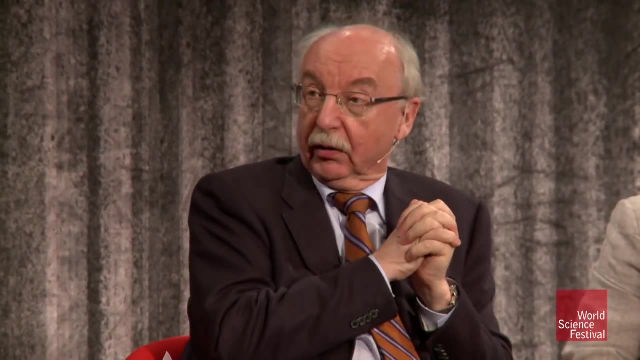 Yeah, yeah. There are good examples where numbers are useful. Assume you want to fly from, say, New York to Washington: Mm-hmm, Yeah, Yeah, Yeah, Yeah, And you want to get there and you have a choice. between flying and driving. The only thing you care about is whether you arrive alive. So question: How dangerous is flying relative to driving? Precise question: How many miles would you have to drive so that the risk of dying is the same as in a non-stop flight? 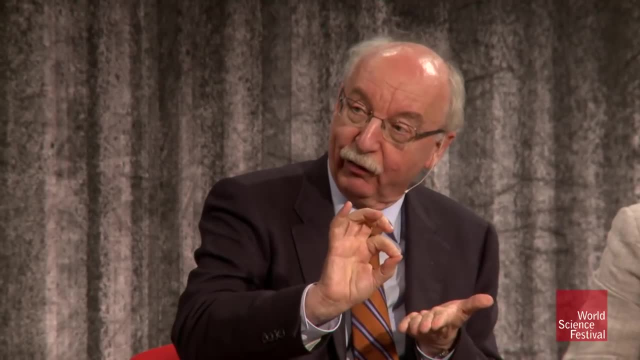 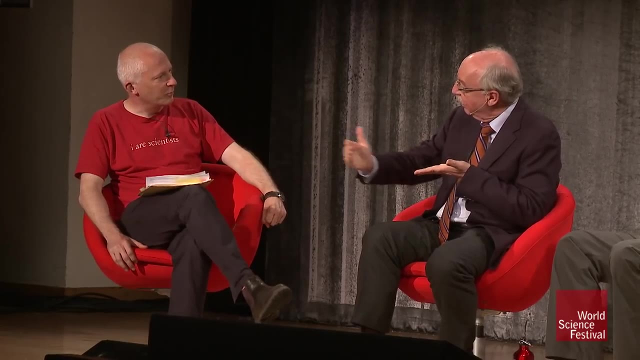 What do you think? How many miles? Well, probably you have to drive. huh, That the risk gets, as I know. as in a non-stop flight. Yeah, as in a non-stop flight. What do you think? 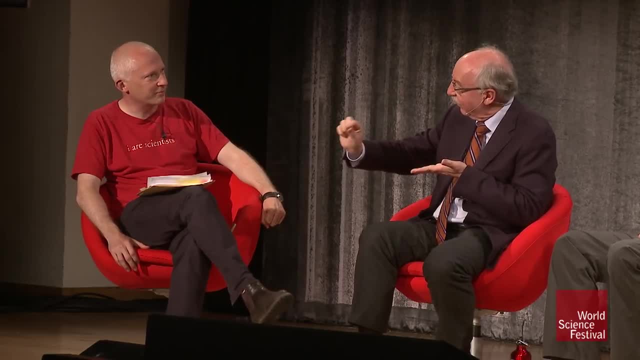 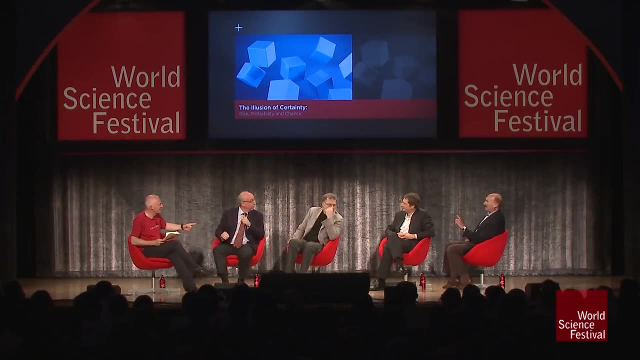 How many miles? Well, probably you have to drive- huh, I know that the So any non-stop flight because it's just taking off and landing, that's dangerous. Yeah, I probably have to fight my intuition In the United States. the probability is 12 out of 100,000 of dying in. if you drive In France it's about eight and the smallest for some Eight. Is that all the wine in Well? actually, in some European countries, it's as low as five, And the lowest I've seen- I checked it online- is about three and a half in 100,000.. So I think driving is as low as five. Yeah, So it's actually much less safe than flying. 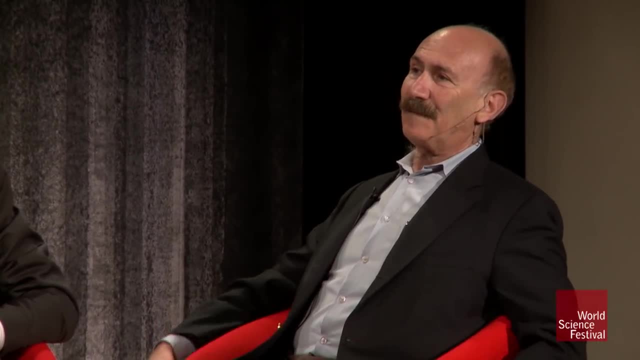 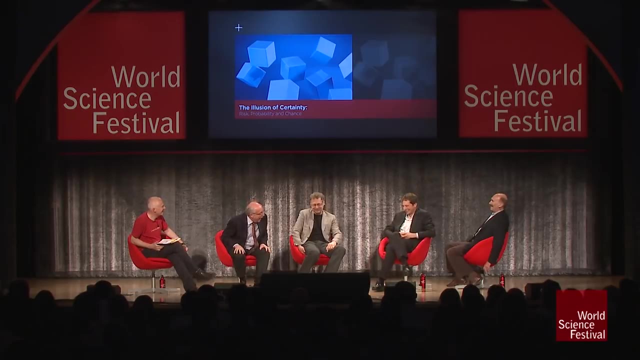 Yes, that's right, But how? So? how many miles do you have to drive? Yeah, Well, let's say That's the question: 5,000.. 5,000.. Josh, I try not to drive. 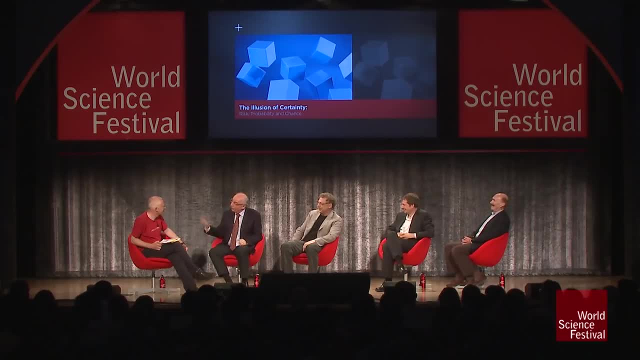 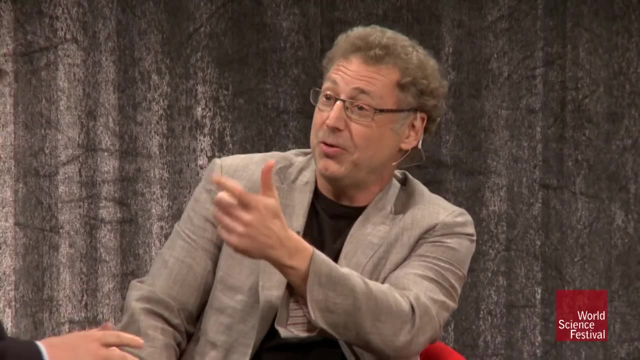 I have no idea. 500.. 500?? No, You're a more pessimistic driver. Well, I'm trying to fight my intuition. so, Okay, So the best. Oh wait, Yeah, because driving is more. 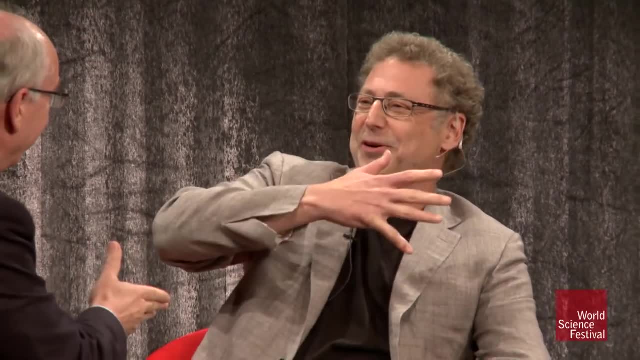 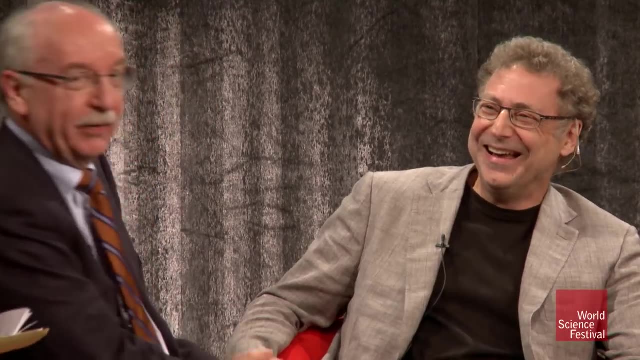 You're right, I went the wrong way, because driving, we know, is more dangerous than flying. Yeah, What's your new estimate? $4.99.. Okay, I have kids, I have to play this game. Yeah, You know how to play this game. Yeah. So the best estimate is: if you drive 12 miles- 12 miles, I want- Then you have the same risk to Wow, Yeah, to die as in a non-stop flight. Yeah, That means if you arrive safely. 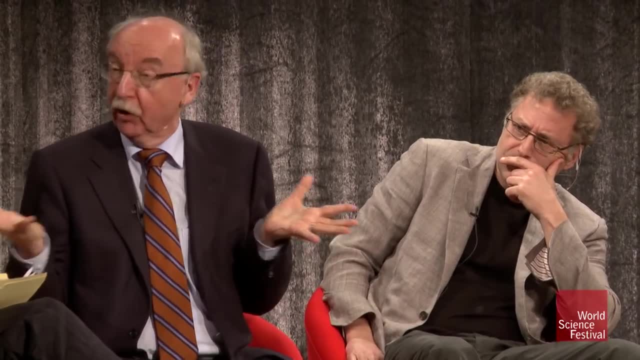 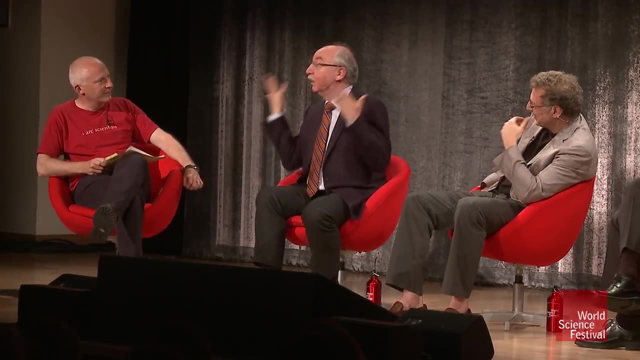 at the airport with your car. the most dangerous part of your life is to die. Wow, Yeah. So I think that's the best estimate, because the travel is already. Yeah. Well, that's But Amir, what about? 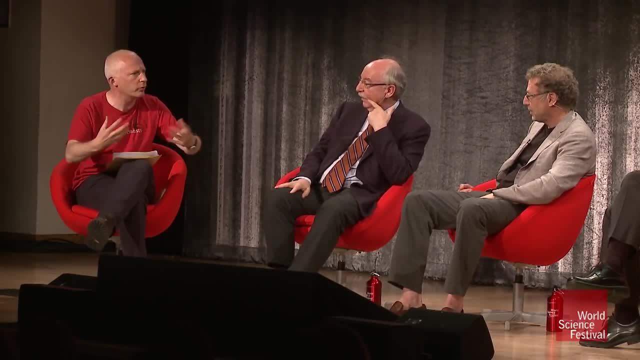 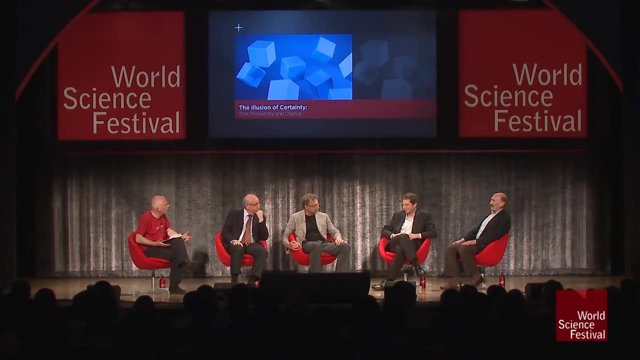 I mean numbers. we've somehow been evolutionary. You know, it's a matter of to fight or fly is about being able to count. So is the brain actually. Well, We've used numbers ever since, First of all, most accidents. 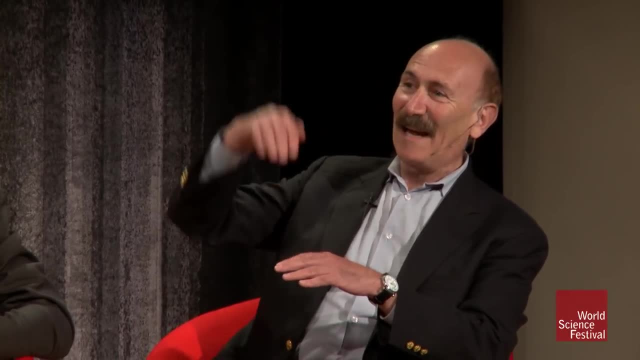 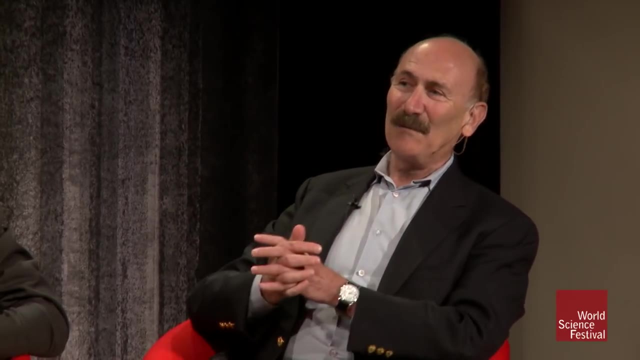 happen near your home, So the miles don't really come inside. The takeoff and landing of an airplane are the most dangerous, So the length of the flight doesn't matter either. and the question about numbers: obviously I believe in numbers. 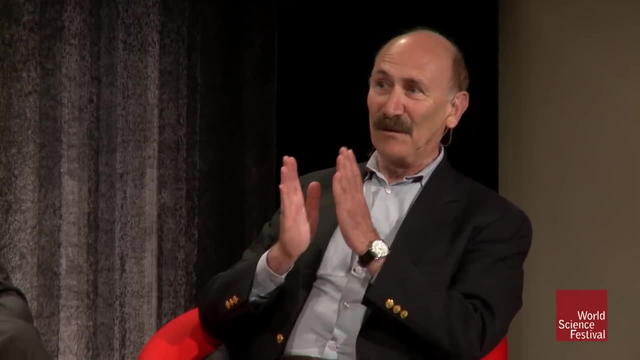 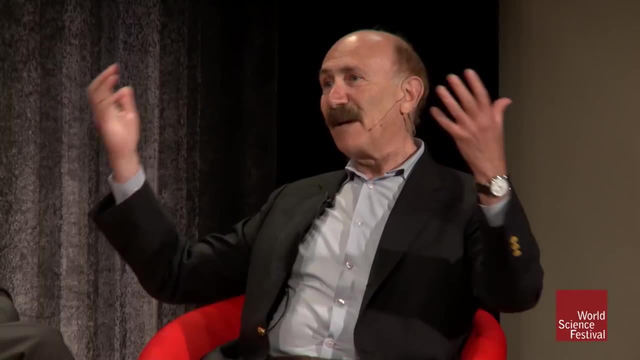 I just think we don't interpret them right. But I think a lot of science can be broken down to numbers and the meaning of numbers. if only we could really understand the meaning of numbers. In biology we tend to think: well, there are processes. 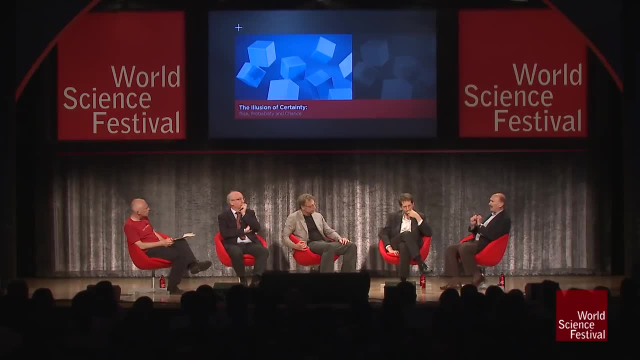 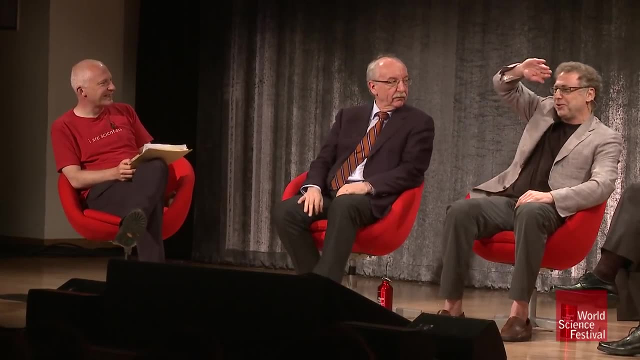 here and there. but if you could quantify them in a correct way, we'll have perfect information. But You won't agree with me, because there's quantum mechanics comes in and then, Okay, Who here drinks wine? Well, never mind. 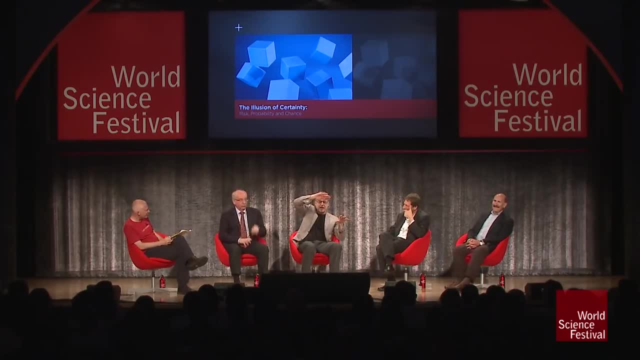 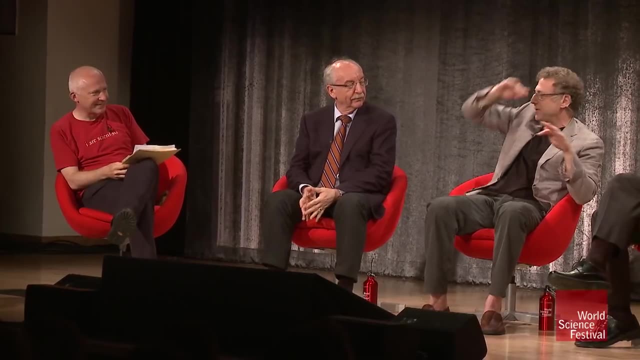 Who here looks at the wine ratings? You know 89,, 94? Anybody. Yeah, I do. Yeah, Only a couple. That's good, because my experience was people do, In fact, the economists- tell you how many dollars it's worth. 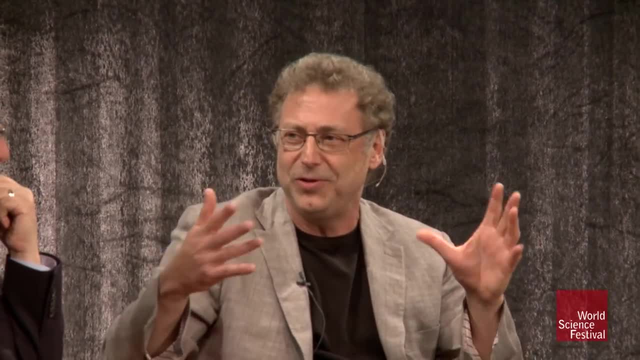 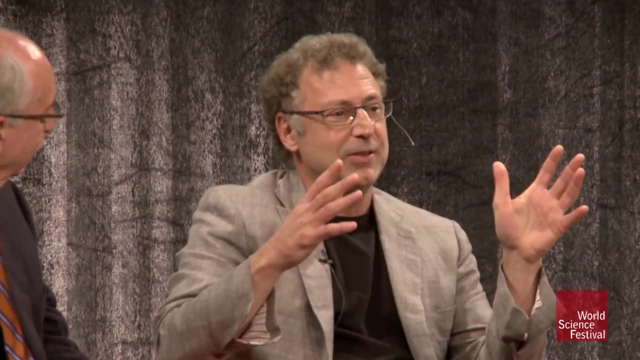 It's quite a bit between an 89, a 90, a 91. And they rate them on a scale that officially starts at something like 60. But really it starts at 85 or 90 and goes to like 99. 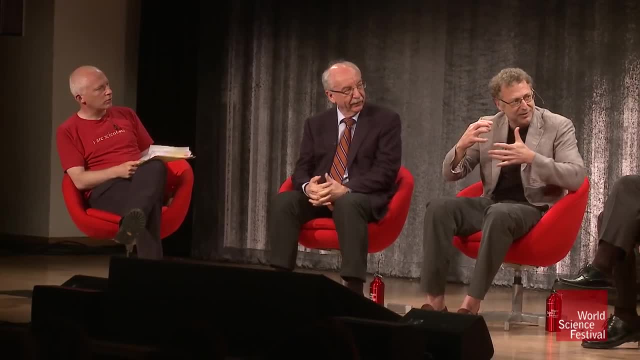 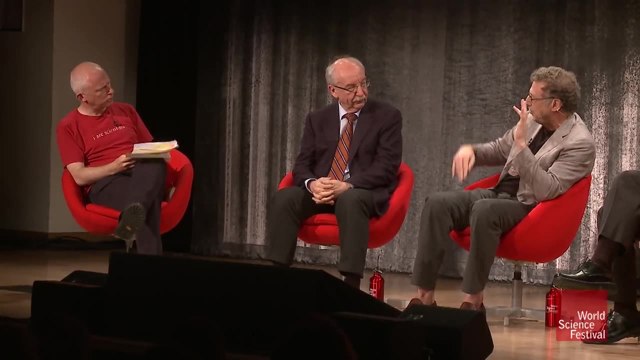 or 100, right, Yes, And people think that once you assign a wine rating it's meaningful. But suppose that you take a particular. Even People's tastes are different. But suppose you have a wine rater and you know that your tastes. 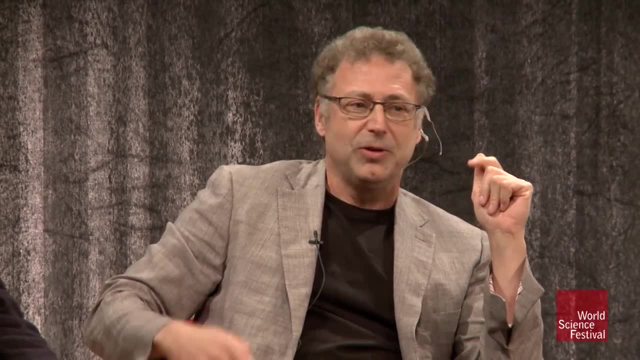 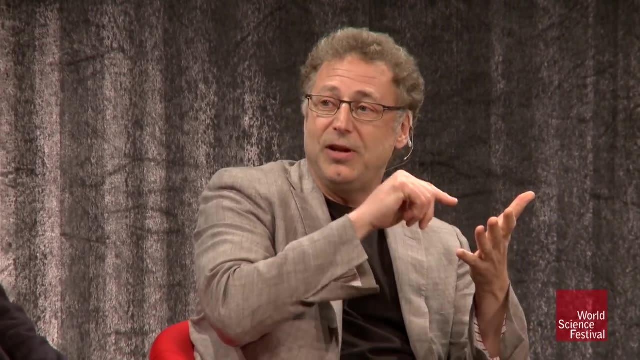 are very similar and that same wine rater tastes the same wine on 10 different occasions over a month in different times, right? So the number: If the person rates a wine a 92, that means a lot. It's a lot different. 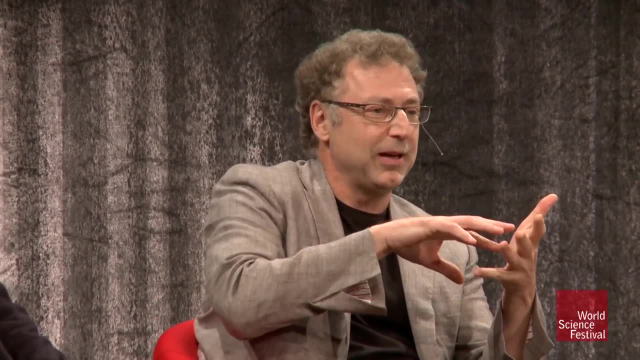 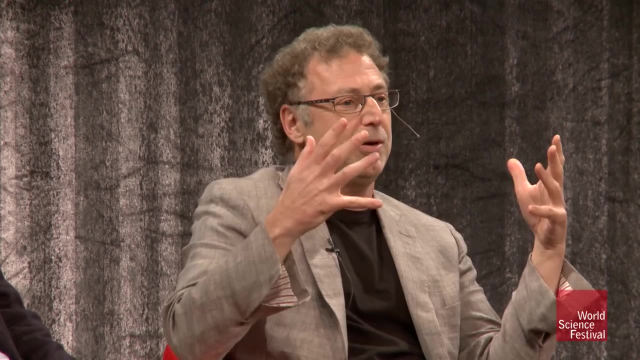 if that person gives it a 92 every time, It has to be a blind tasting, But if it's consistent, that means one thing, and if it's an 89 another time, it's a 95 another time and it spreads all over. 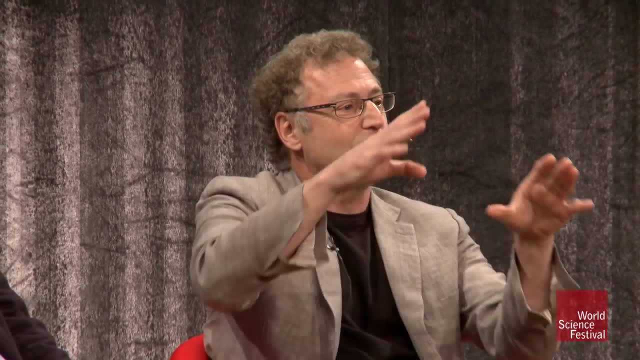 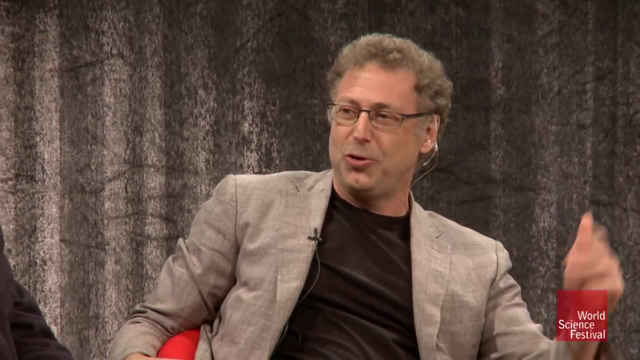 So, when you hear a number, what I'm trying to tell you is: don't just look at the number. You have to look at what's the uncertainty and what's the variance. But we have to Wait. wait, There's a punchline. 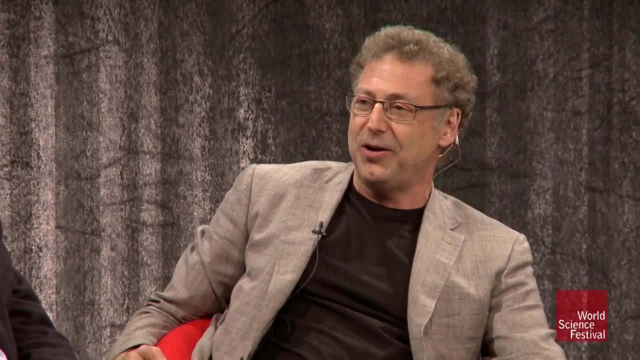 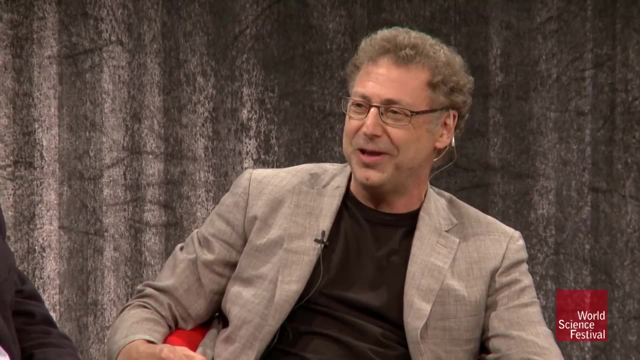 Okay, So Robert Parker, he's a wine guru. right, He's the guru, yeah, And he sets a lot of what these ratings are and his ratings are very closely followed. He started the rating system in the 70s and he knows a lot. 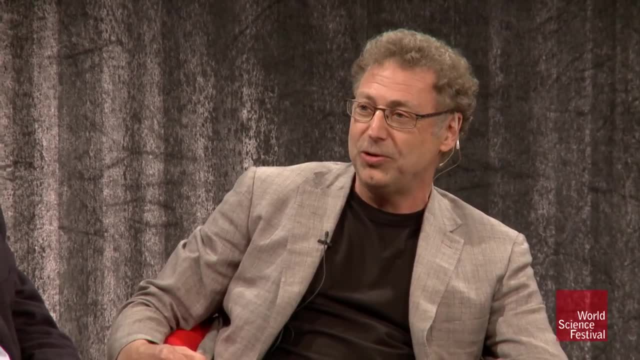 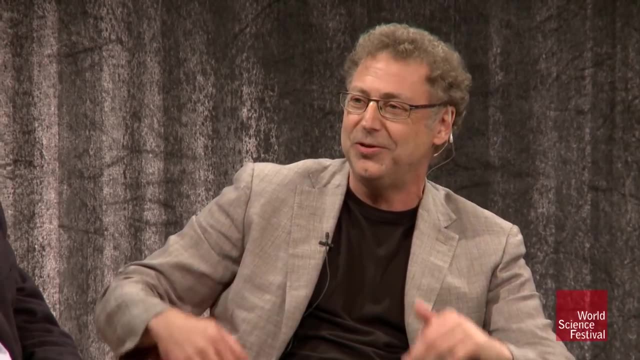 about wine. I certainly don't want to question that. I went to him for the Wall Street Journal and I asked him: you know, roughly speaking, how much variation do you have? And I had some data on his A couple of times. 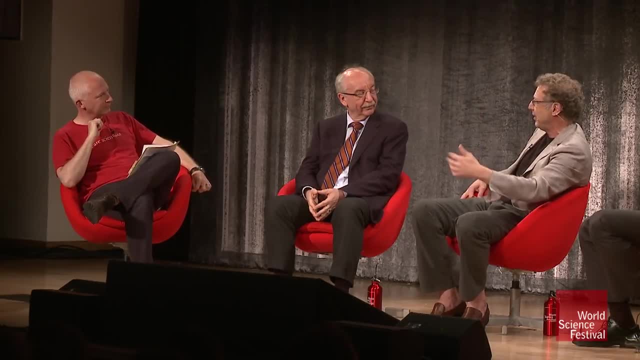 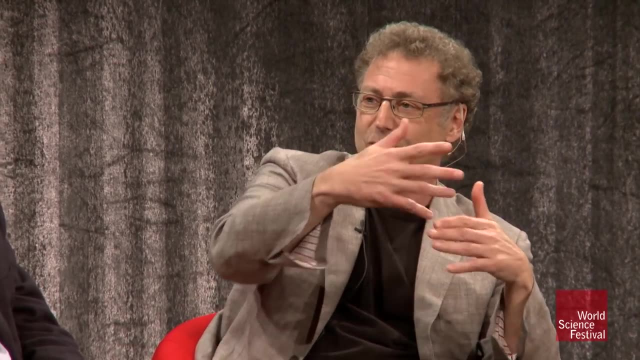 where he tasted the same wines and he said: maybe three points. It can depend on my mood, and what I ate in the morning will affect how I drink the wine in the afternoon. Well, if you think about the fact that the wines he's rating, 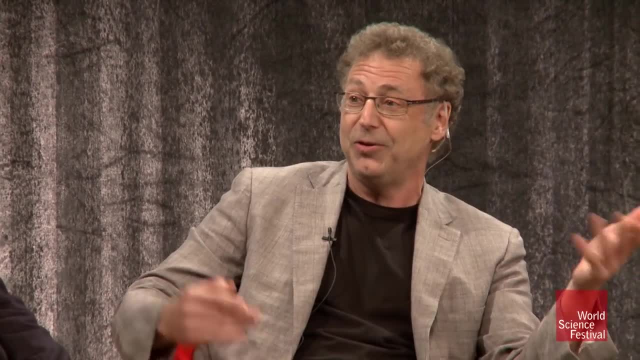 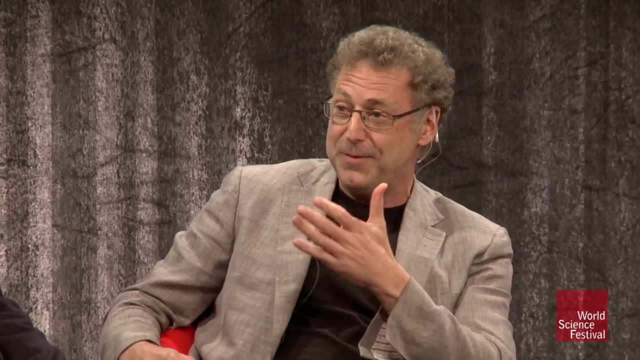 are more or less between 90,, 92, and 100, and it's a three-point plus from. So a 92 wine at a given time, the same wine could be either one. So you just have to keep in mind that putting a number, 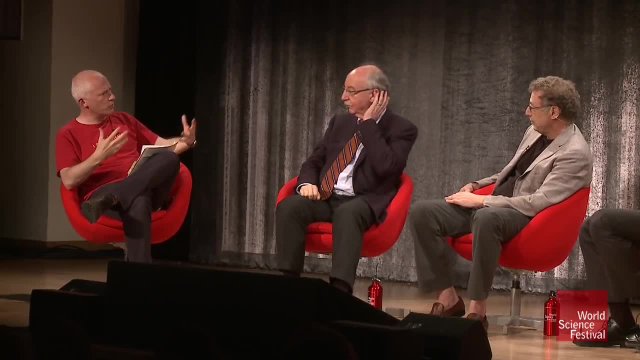 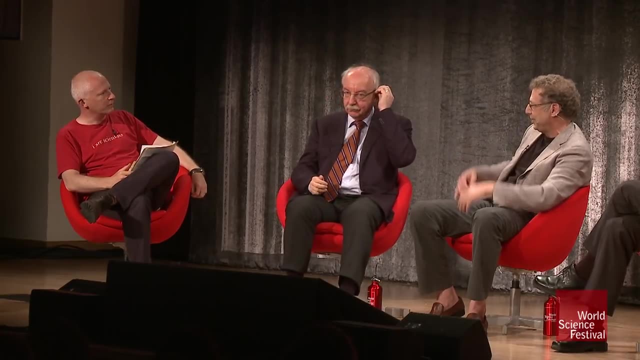 to something doesn't mean that it's meaningful. No, I mean not everything. In the introductory video we saw how to put a number to impact. I mean, not everything can be translated into numbers. Right, Yeah, They put a number. 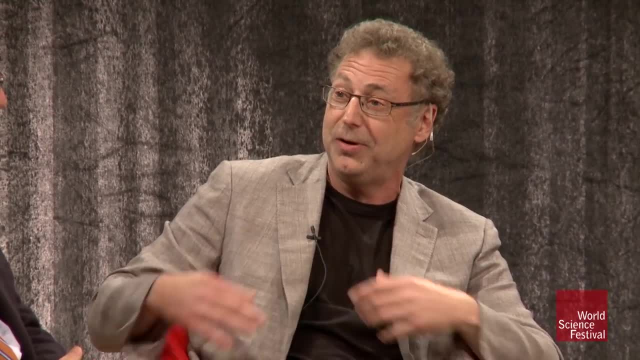 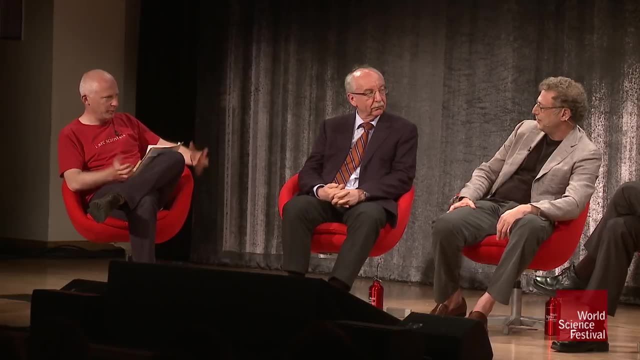 and people feel like it means something. I think there's a gut feeling that it means something. It's meaningful, just because someone assigns a number, Which we're going to come back to a little bit later- but we need to start the experiment now. 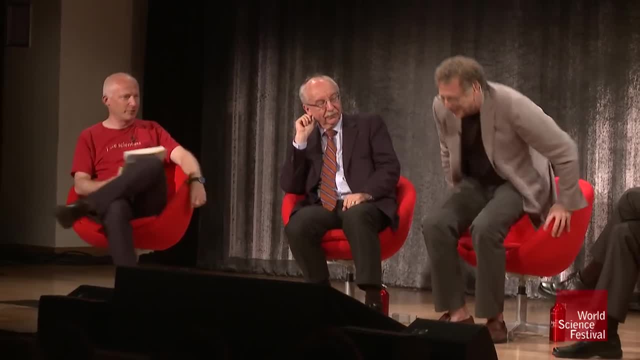 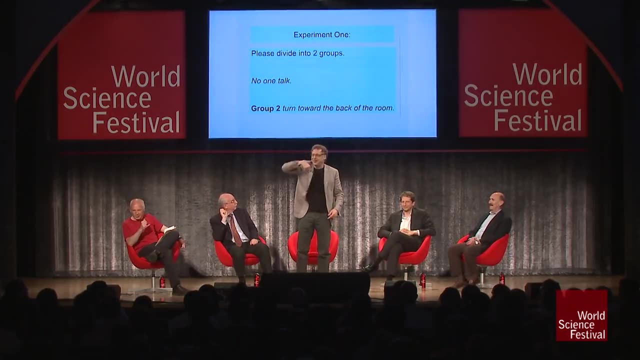 Just I won't say too much, else we'll spoil the experiment- Easily spoil. Take us through your numbers. Okay, Can I have lights? a little bit Some lights, Because we need to see the audience. You're going to be involved in this. 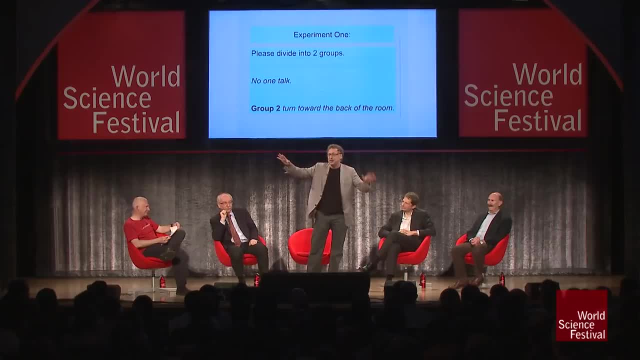 All right. So in this experiment, I'd like to divide you into two groups. First of all, let me say it's totally anonymous your answer, so don't worry about whether you're going to do it. So everyone who's to this side of me, 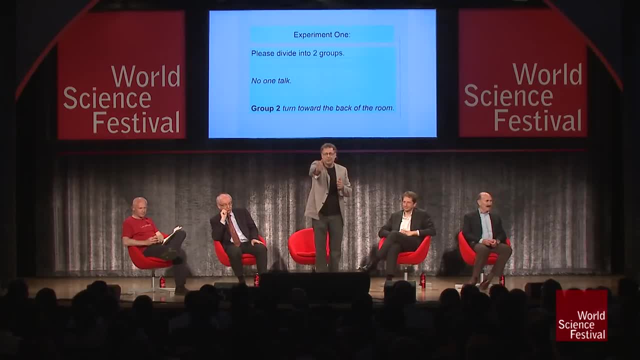 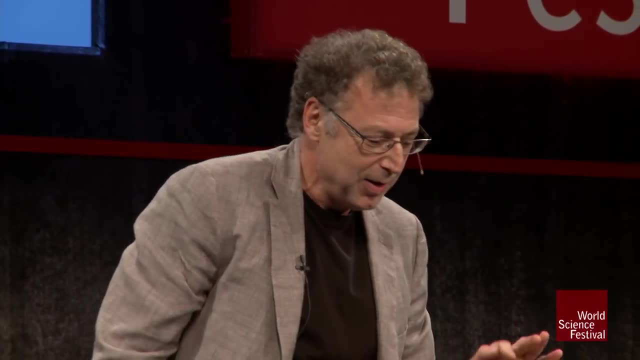 will call you group one And whatever it's you know. just make a guess which side of me you are, it's not that important. And everyone on this side I'm just trying to divide you in half is group two. Okay, So this is a proof. 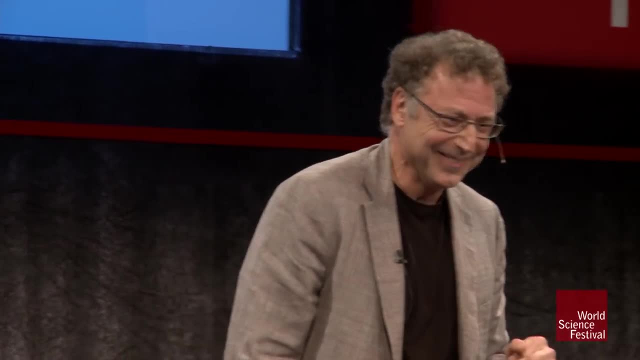 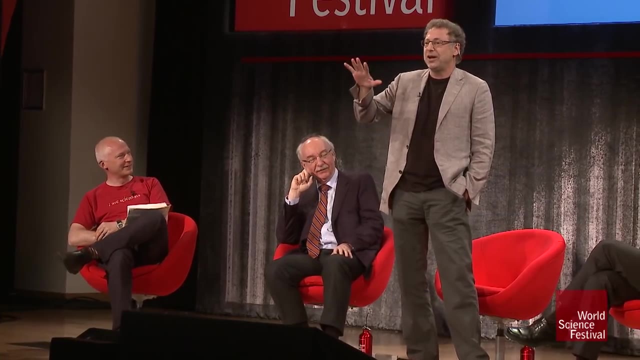 that numbers are very important. This is a. I don't want to say what this is. No, no, no. I'm just saying you've numbered your groups. I'm going to show some slides. I want you to. Everything has to be done. 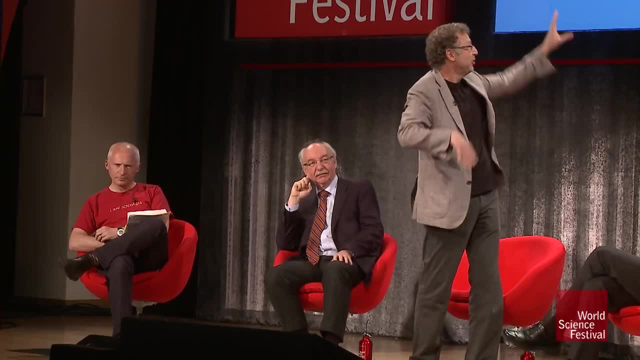 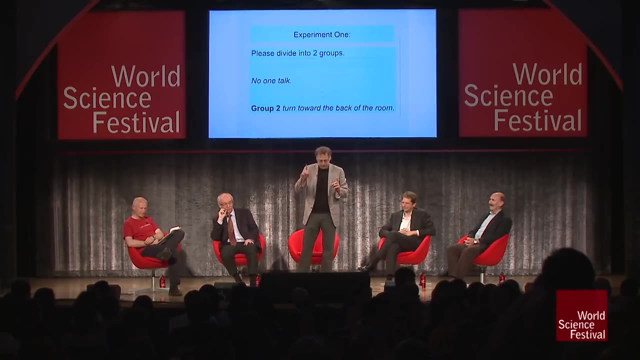 in silence. Okay, So group two. if you assign yourself to group two, please turn away so you don't see the screen. if you want to participate? Okay And Okay, Next slide. So please read this silently and you have presumably a next card. 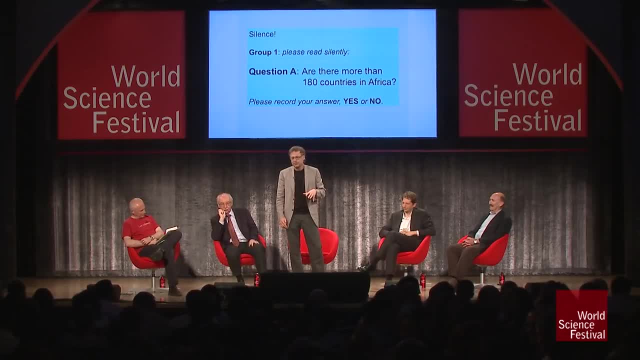 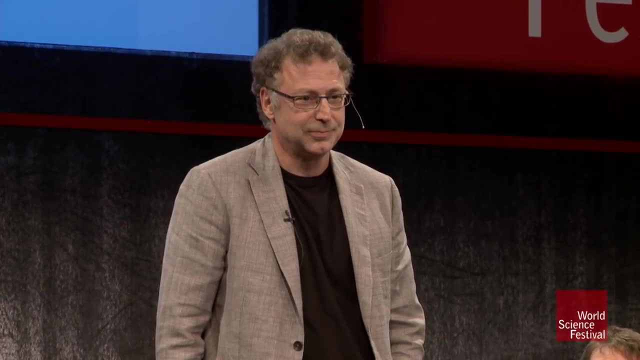 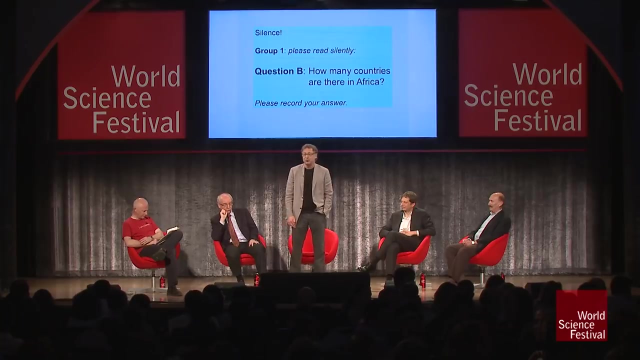 and a pencil and just write down your answer. Okay, Next slide. Okay, Please read this silently and write down your answer to this one. Okay, All right, Next slide. Okay, So, So, So, So, Okay, So. 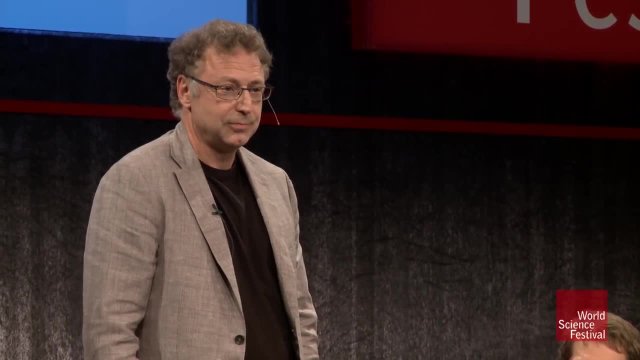 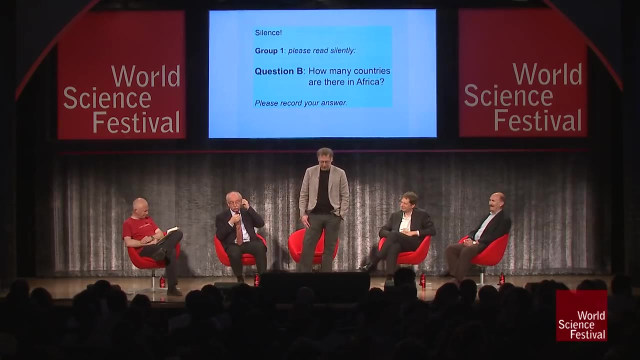 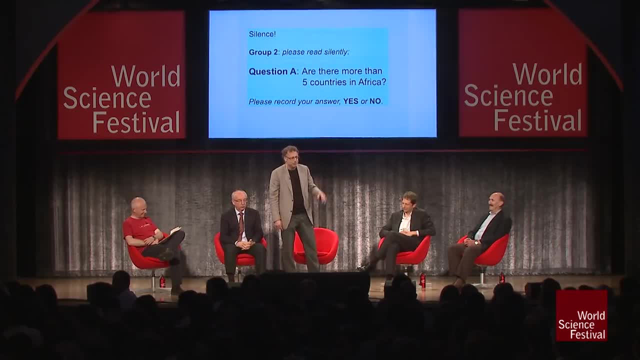 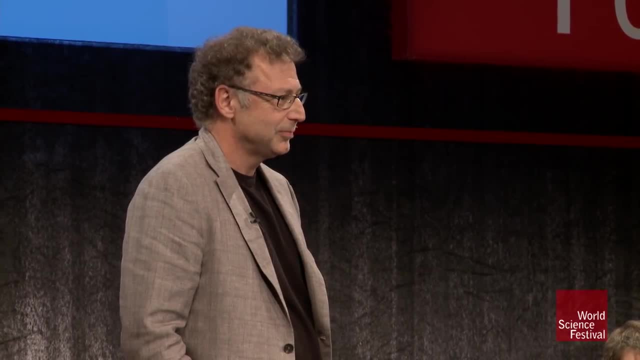 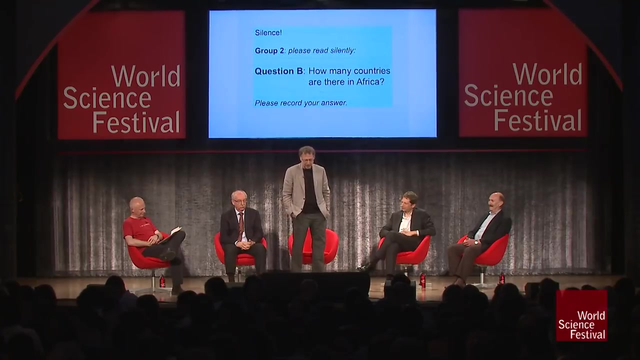 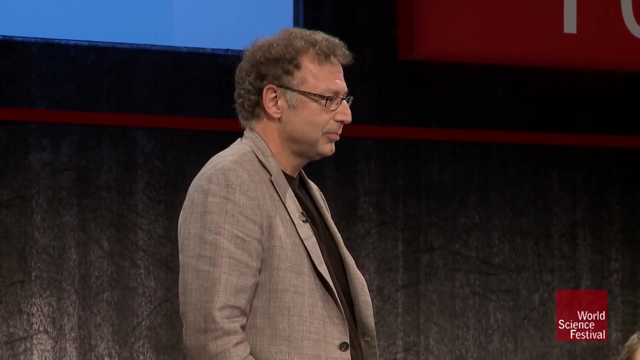 Next slide: Okay, Group two. please read this silently and write down your answer. Okay, Next slide. And now read this silently and write down your answer to this one. Thank you, Okay, Next slide, this one. Okay, next slide. All right now someone. 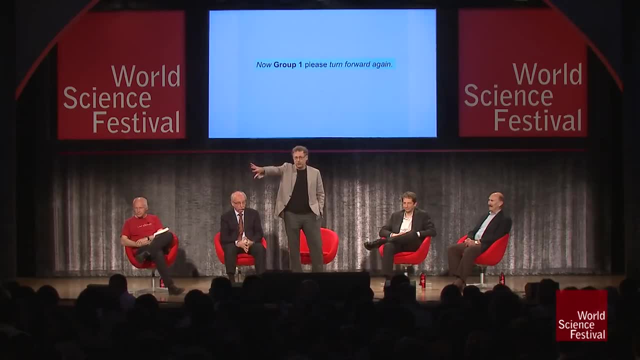 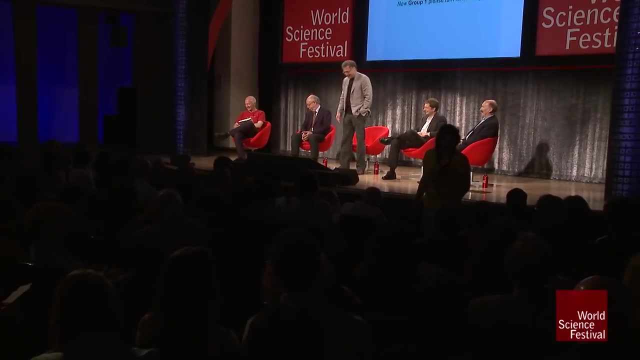 will collect from group one. pass your answers that way and group two pass your answers well, toward that aisle and group one toward that aisle. You know, I never talk to the person who's doing the calculation. I hope they know what they're doing. All right? 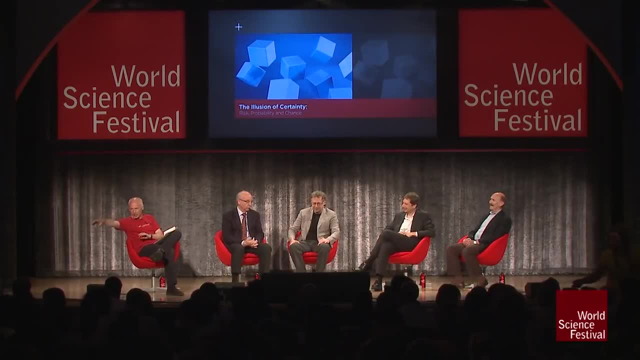 Great, so all group ones are going towards our volunteers down the aisle here. Group two's all converging down here And we'll come back a little bit later. Somebody's going to take all the data, analyze it for us and we'll come back later to interpret the information. 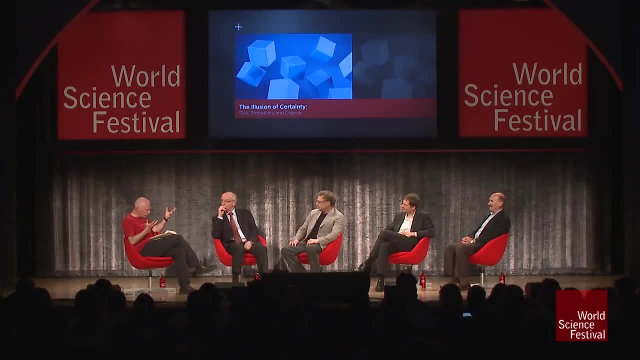 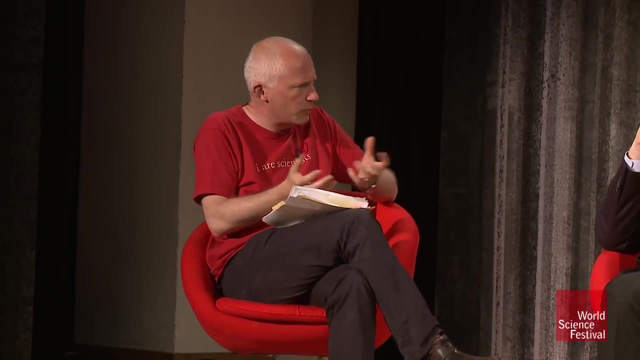 Now, Leonard, you think that there's some sort of data that we're actually really bad at interpreting and for various reasons, like the fact that how it's coached in terms of units and things like that, Can you perhaps expand a little bit? 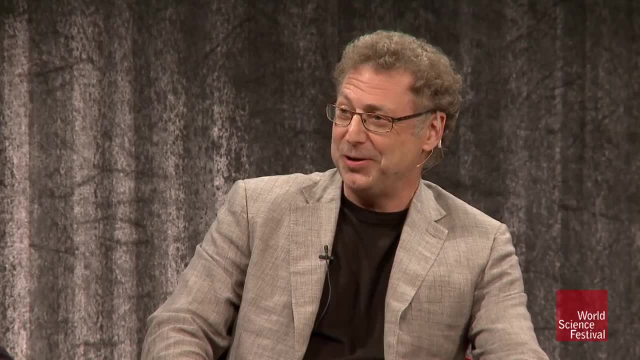 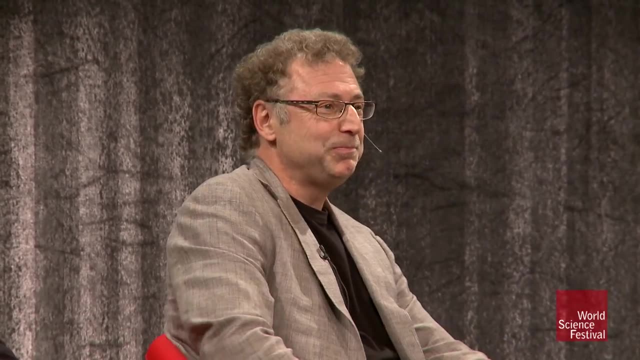 Oh well, actually I have something. I could a little audio aid if you want to. Oh, okay, right, yes, yes. So I mean, you'll see, this demonstration tells us, addresses that same point, but before. 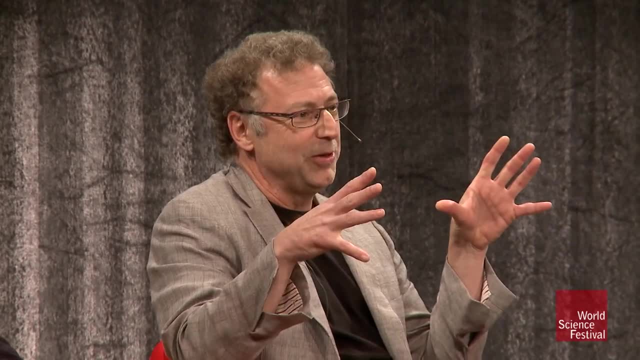 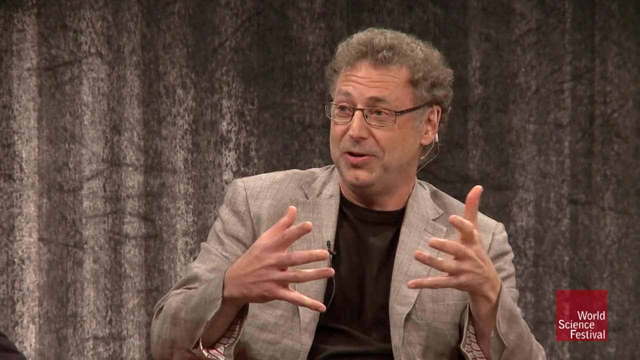 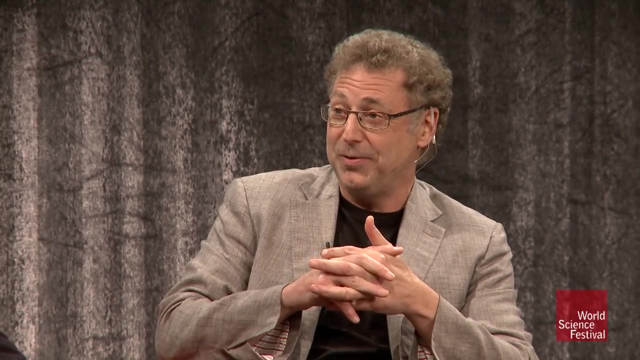 you really can understand the finer points of probability and statistics and randomness. you have to understand even basic things like arithmetic or units and numbers, and unfortunately our society and our educational system does a very bad job at that, I believe, and that's. 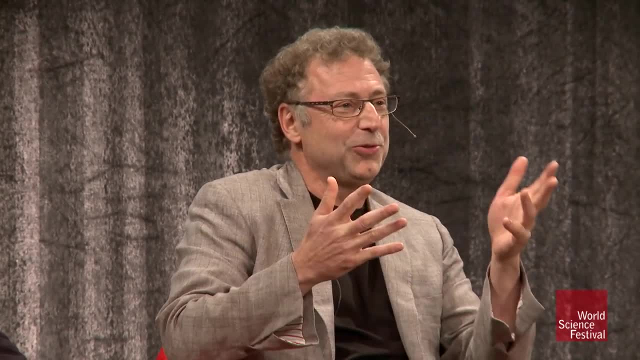 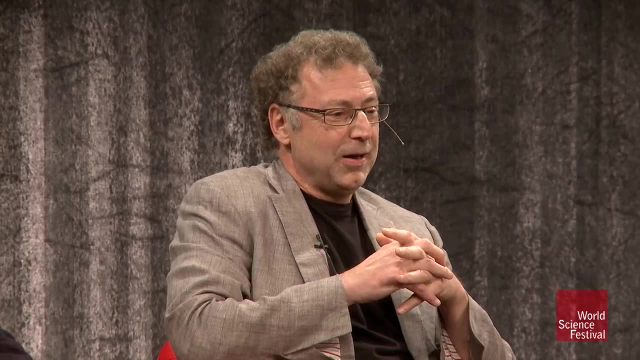 a whole other panel. we should have some time. So here's just an illustration of that that I just thought was great and let me. I got to set it up. I'll tell you what's going on. There's this fellow, an American, who has a packaged data plan from Verizon, and so 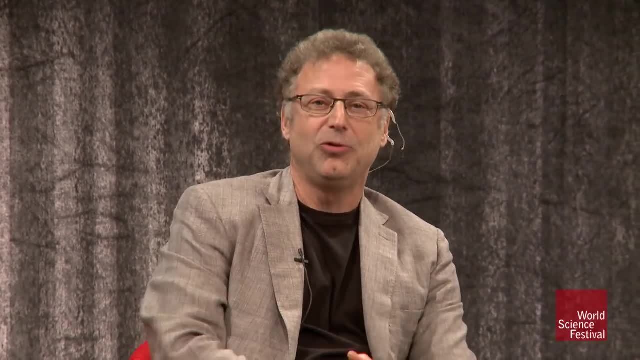 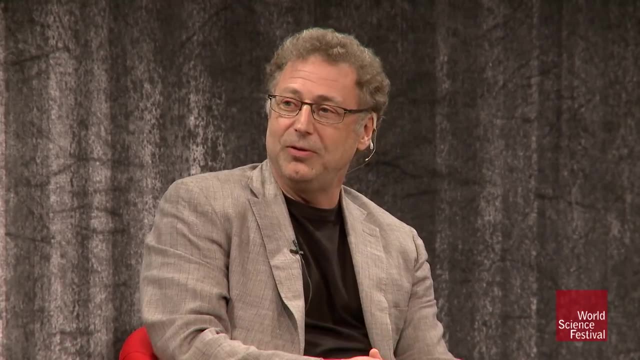 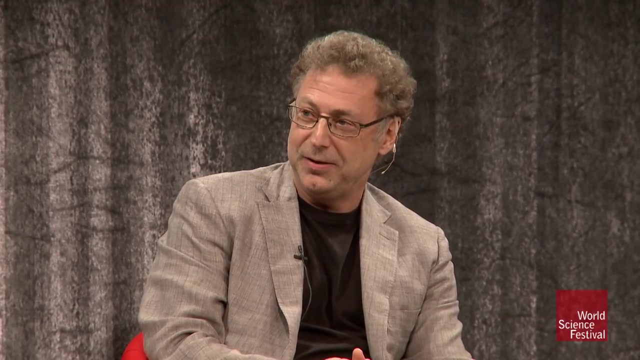 he pays a flat rate for his use of data and he was going to Canada And So he calls Verizon and he says what's the rate for Canada? So they said to him it's 0.002 cents per kilobyte. 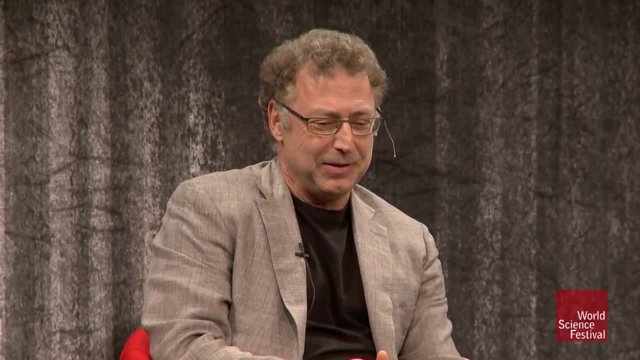 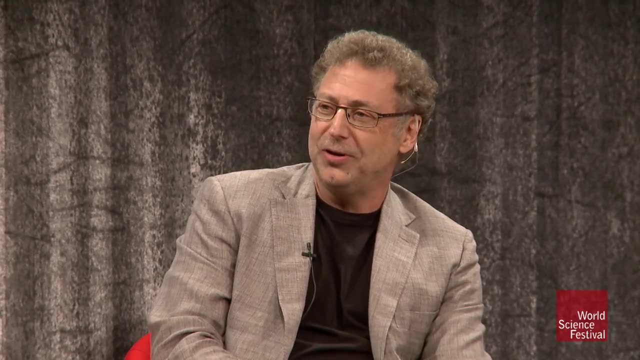 And that's 2 1,000th of a cent per kilobyte. And he said: I don't know what it normally costs. I don't know what that is, but I just want to double check. Is it 2 1,000th of a cent or 2 1,000th of a dollar? 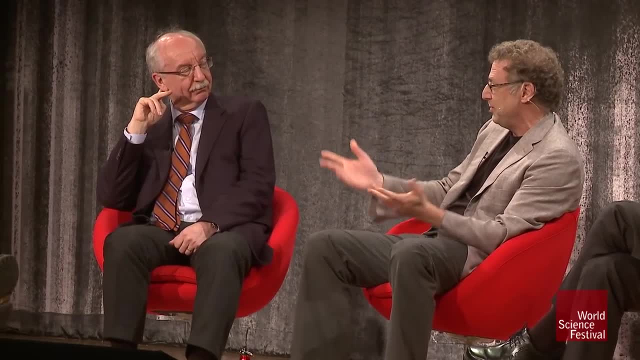 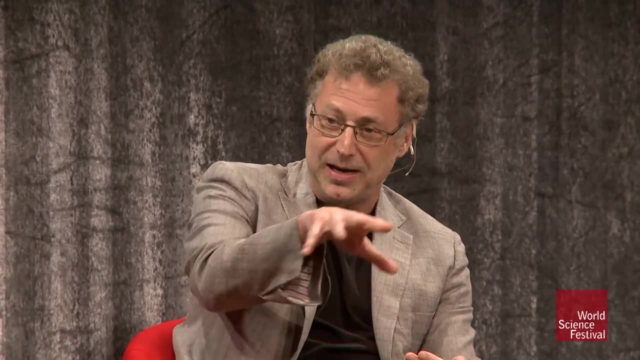 And he had a gut feeling that maybe it should be dollar. but he really didn't know what was normal. And they looked it up and they read it to him and it says 0.002 cents And they put it actually in his file that he asked that question. 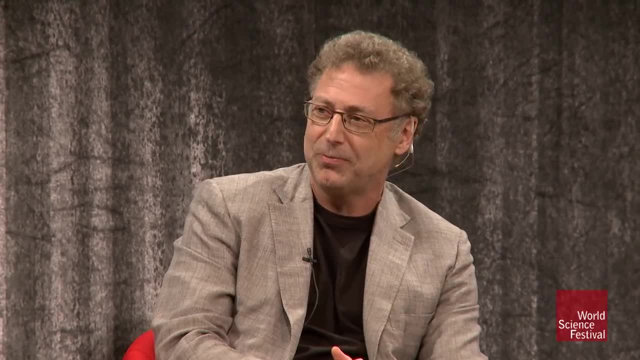 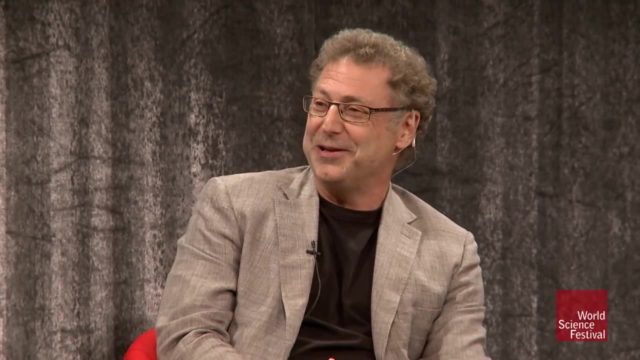 He asked them to put that in his file. It's 0.002 cents per kilobyte. So then he goes to Canada and he uses either $79 worth of data or $0.79 worth of data, depending, I guess, on your point of view. 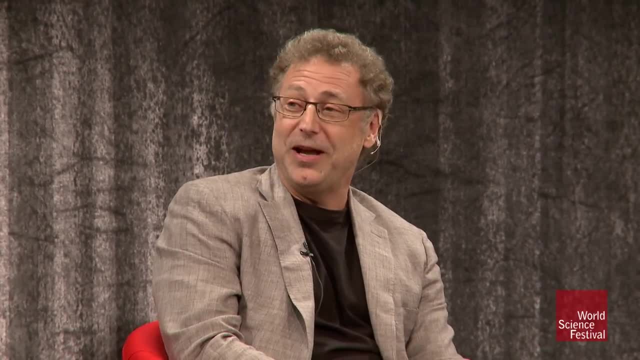 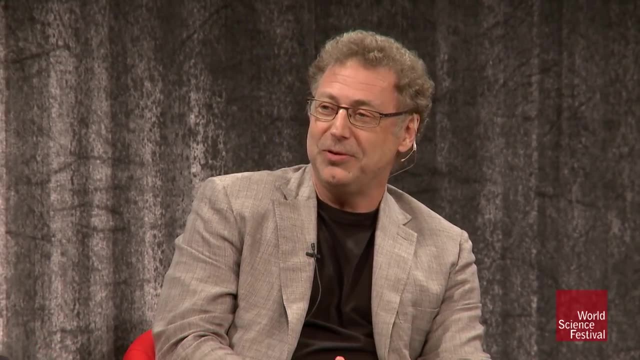 But he got charged $79 worth of data for his data usage as if it would cost $0.002.. So he calls Verizon back And tries to get it back And tries to tell them that it was 0.002 cents. 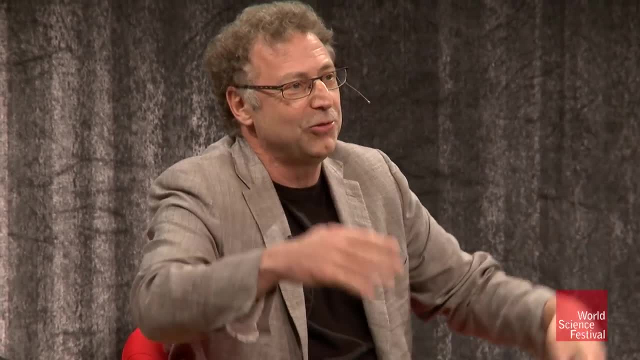 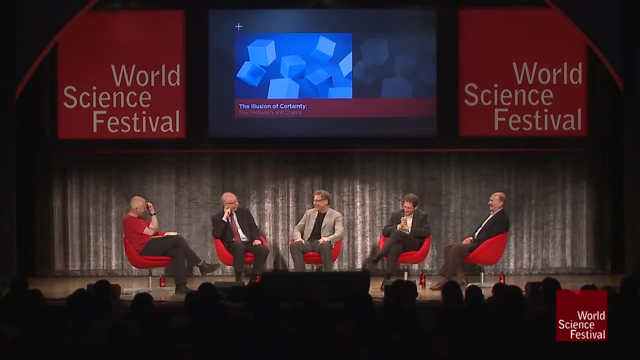 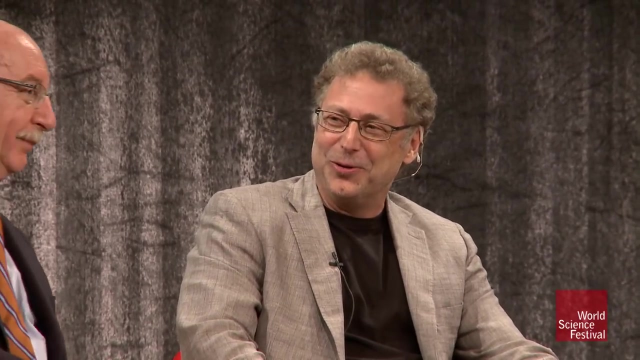 So there's two audio clips. Actually, if you go online and search for this, there's a- Well, if you're a mathematician, a hilarious 20-minute conversation. But the people at the World Science Festival in your service insisted that we cut it down to about a minute and a half. 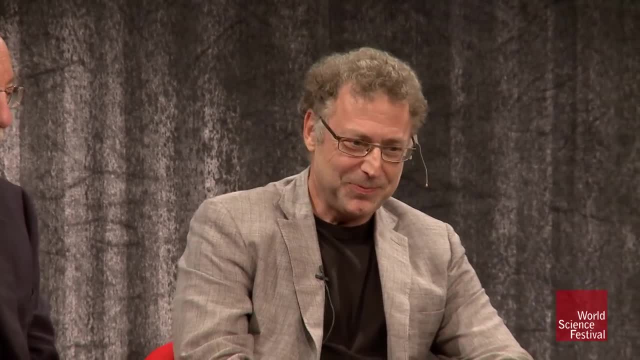 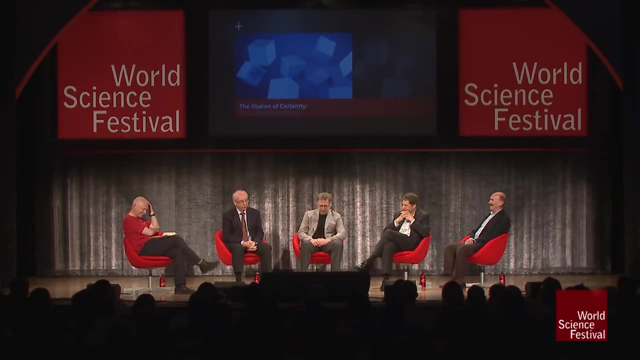 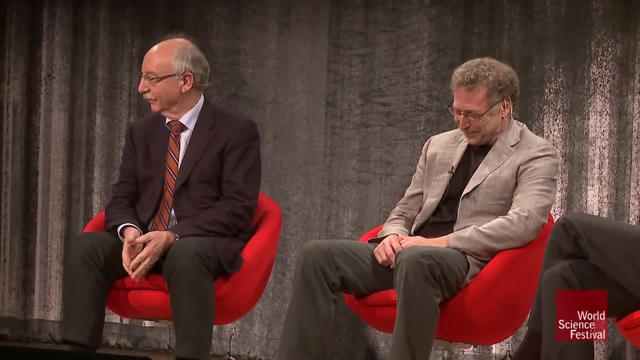 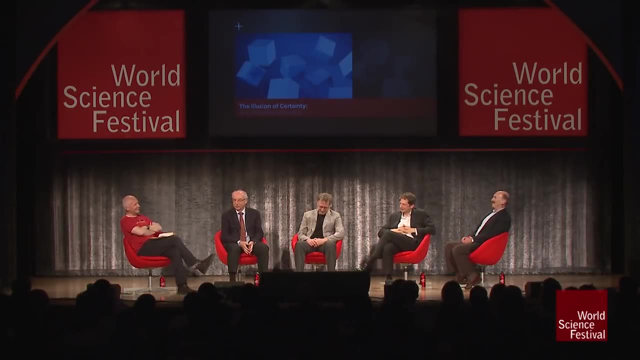 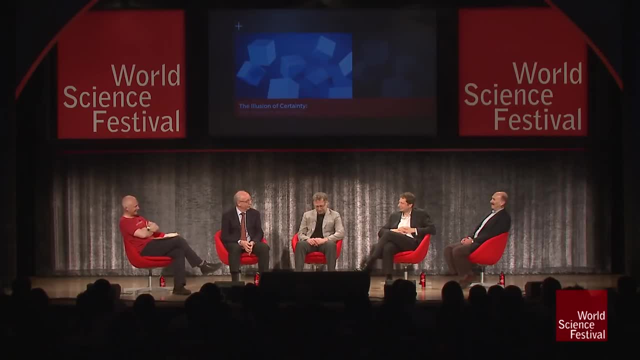 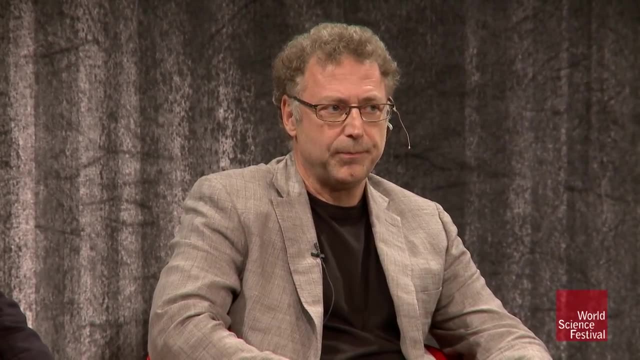 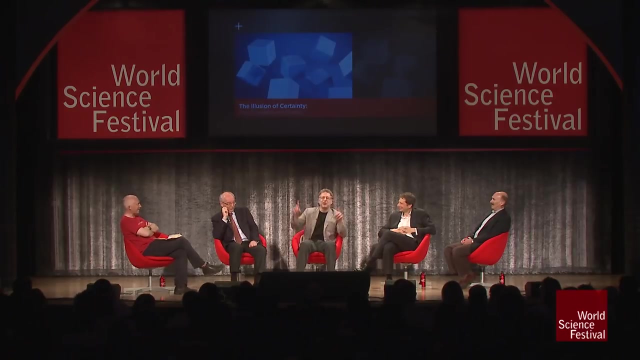 That's two one-thousandths of a cent per kilobyte, Right, My bill reflects $0.002 per minute. What do you mean, $0.002?? This is a supervisor. Okay, I think I have to do this again. Do you recognize that there's a difference between $1 and 1 cent, Definitely. Do you recognize that there's a difference between half a dollar and half a cent, Definitely. And then do you therefore recognize there's a difference between $0.002 and $0.002?. 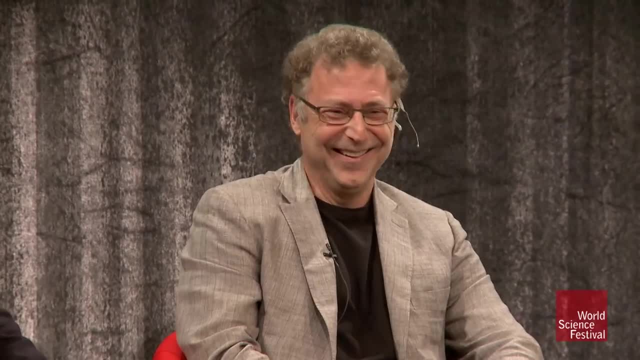 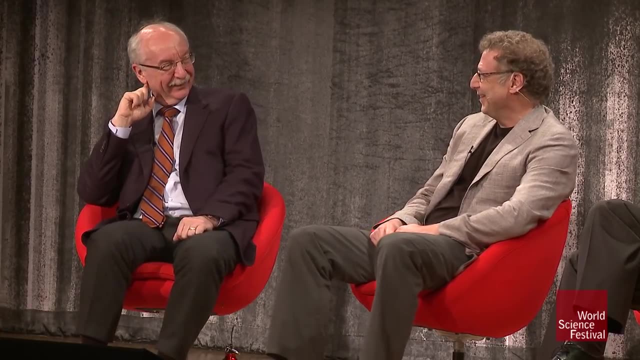 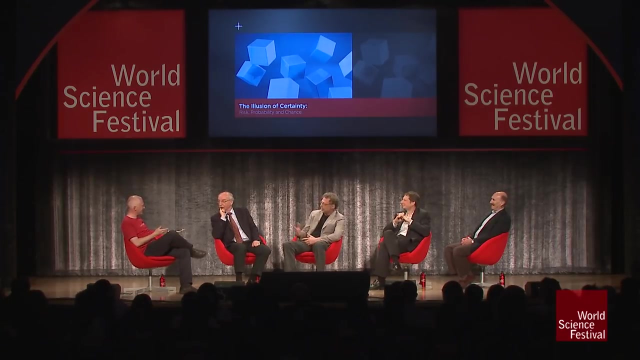 No, No, I mean there's no $0.002.. I recognize that conversation. I've had that one a few times. So why do you think they got the difference between $2 and 2 cents but just shifting the decimal? why did it mess them up so much? 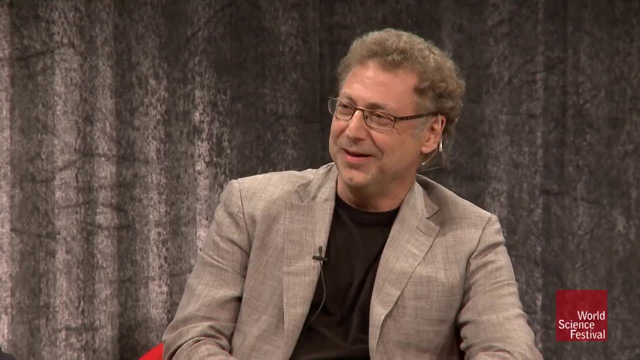 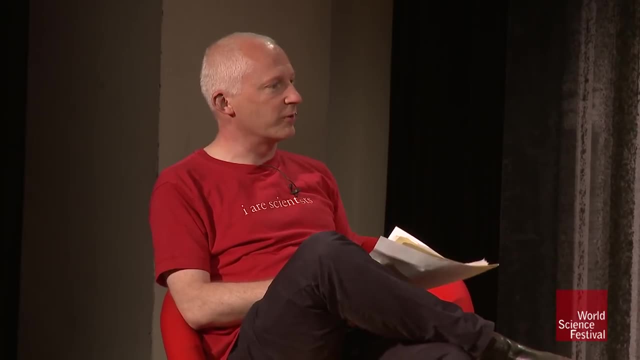 I guess decimal- Because decimal points are- can be difficult. yeah, If I had the answer, though, I would, But I suppose you know, working with different units and things, even the Hubble telescope collapsed because you know people weren't talking the same language. 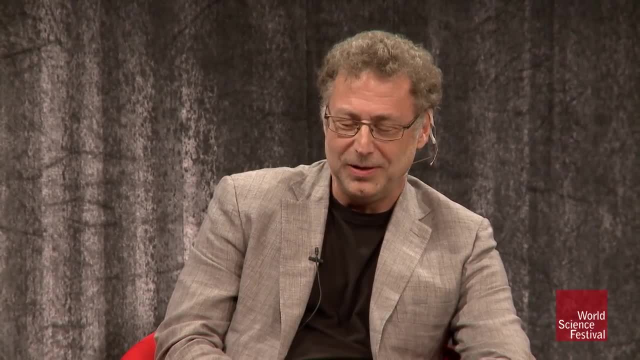 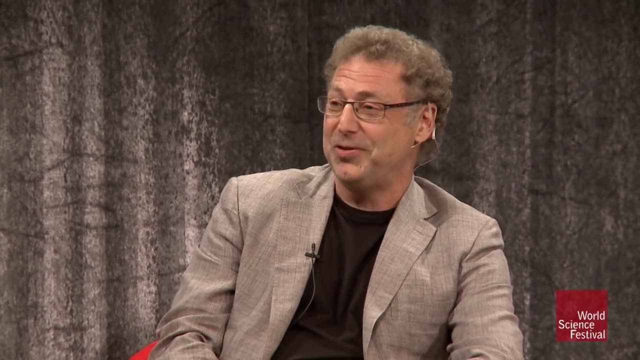 Well, but it's different if you're talking a different language and you don't. and if they said $0.002 and one person was assuming dollars, one person was assuming cents. yeah, that's bad, Yeah, yeah. But if one says $0.002, the other one says $0.002, and you say, oh, that's the same thing. 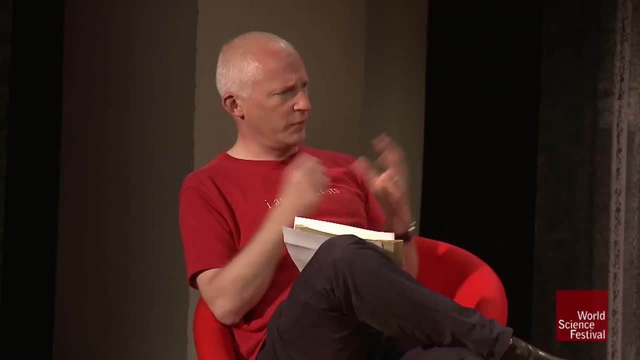 Yeah, Yeah. But if one says $0.002,, the other one says $0.002, and you say, oh, that's the same thing, That's worse, Yeah, Yeah. What about the other end of the spectrum? 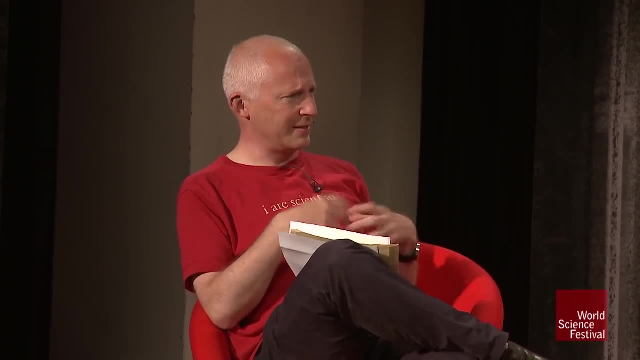 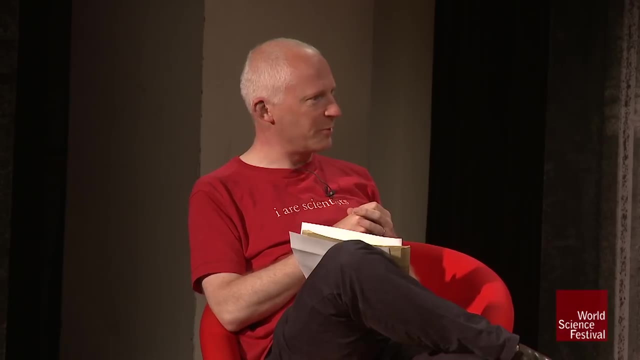 I mean just, I think people. you know, we've had so many statistics about the credit crunch of billions and trillions and millions. I mean people. I think they think those are. they're all infinite, aren't they? 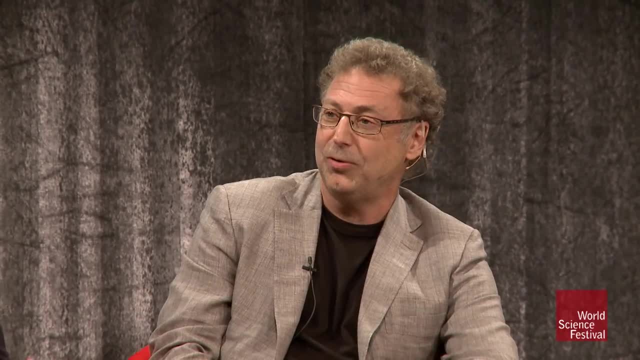 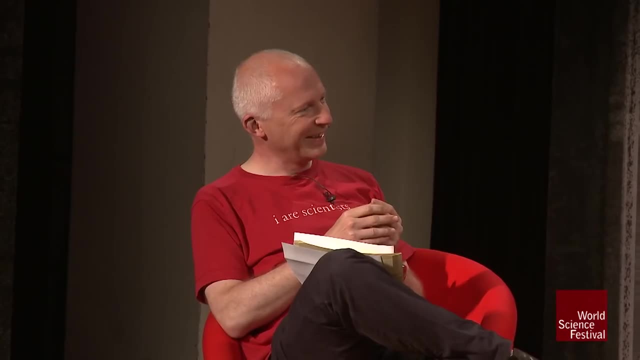 I think so. Yeah, Yeah. Well, it's very hard to envision or visualize or feel that. you know, have a feeling for those numbers. Yeah, And if you're a scientist- not if you're a mathematician, but if you're a scientist, because, right, mathematicians, you 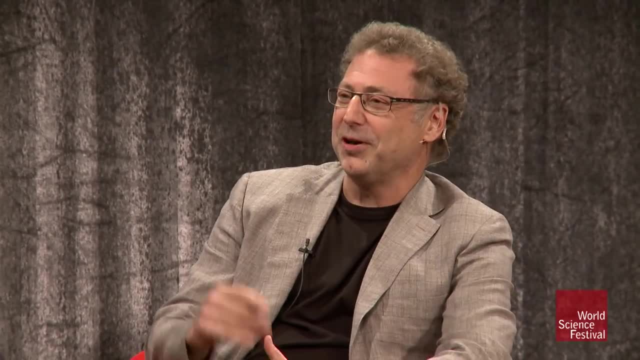 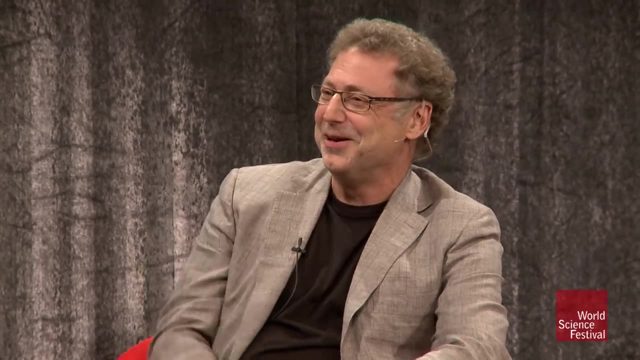 you work purely with the theorems and the symbols. but Yeah, let x be a number, It doesn't really matter what, it is Right. In fact, when I was a graduate student, we used to laugh at the math grad students because we could do stuff. you know math much better, at least our math, because we it's, it's. it's much different. 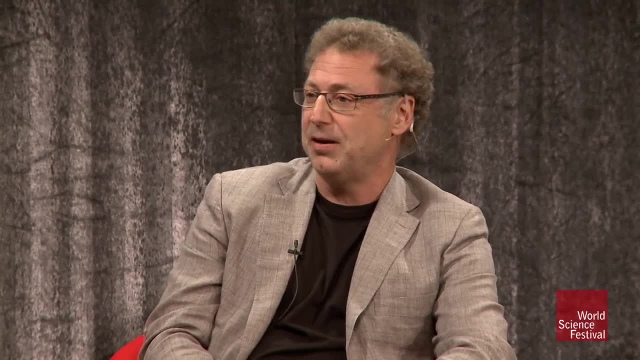 But if you do deal with data, whatever kind of scientist you are, then you get a feeling for that You just, you know, forced to over the years. It's not that hard, You just develop it by working with it day after day. 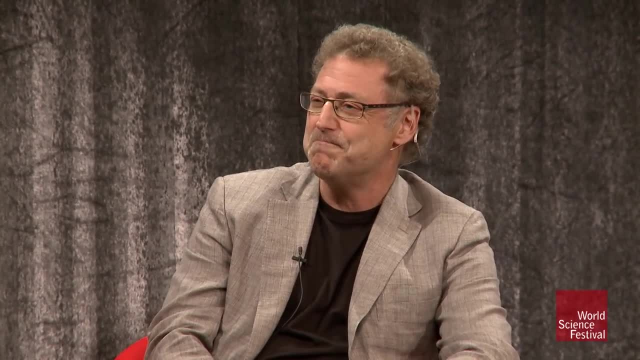 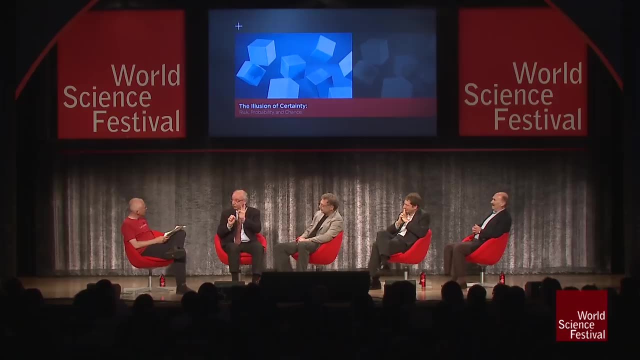 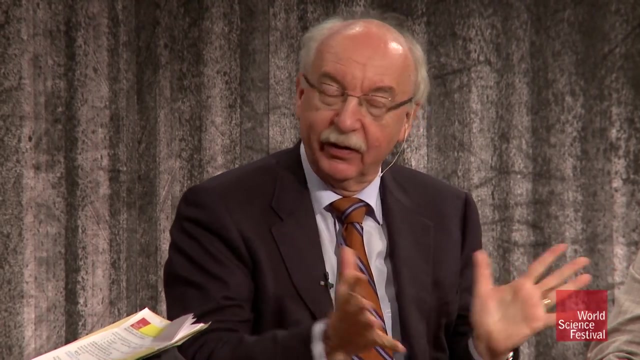 And if you never do, and if you never run into what a trillion means, then Um, yeah, you know. here's one fact. so we are on these zeros behind the point, and so we have asked 1,000 Americans, representative study, the following question. 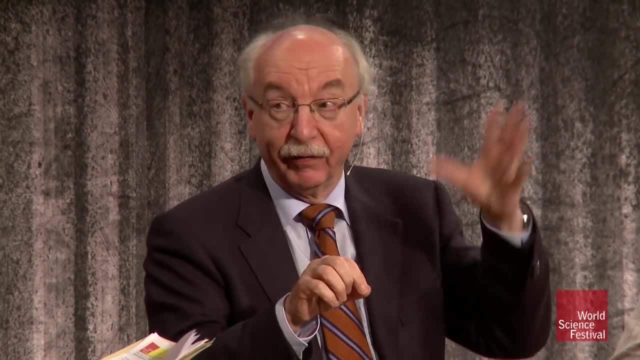 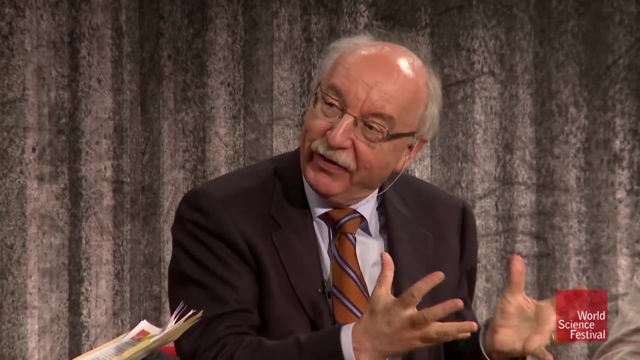 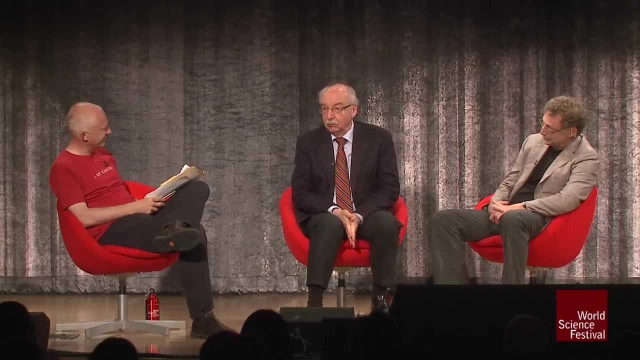 Assume you play a lottery and there is one winner out of every thousand tickets. so what is your chance that you win? So basically translate one in thousand in a percentage. Can you do this? Can anyone do it? Who of you thinks he can do it? 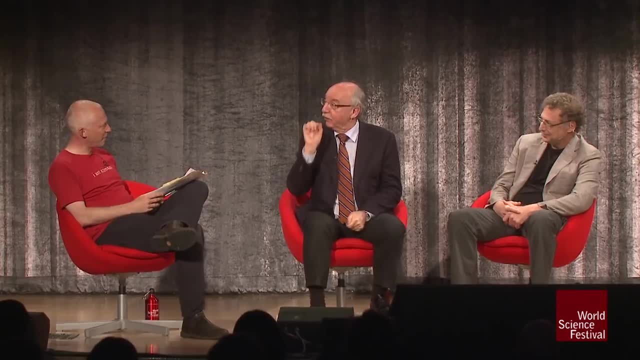 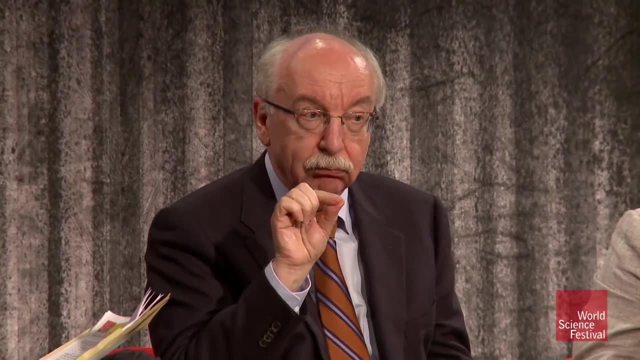 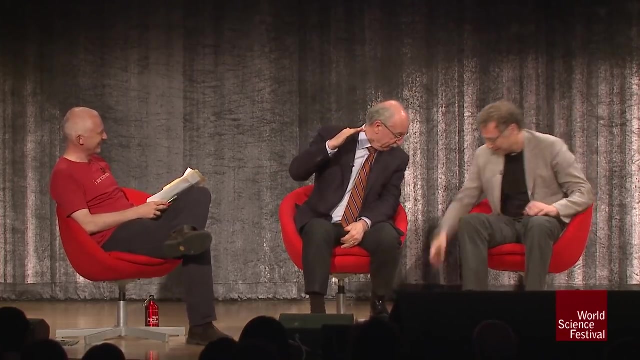 Nobody, I mean. so what proportion of Americans representative study age 18 and older? you think find the right answer. Hint One in a thousand, no Point. one percent, Oh, what do you think? What percentage of Americans can do this? 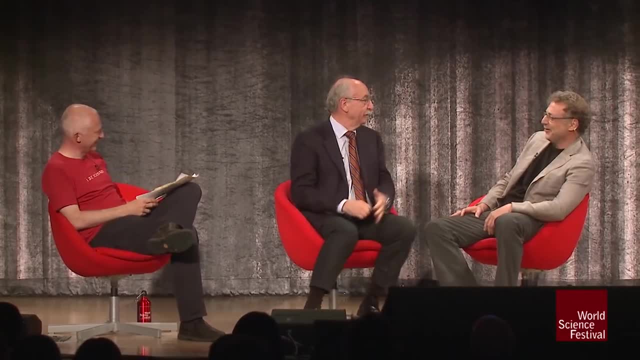 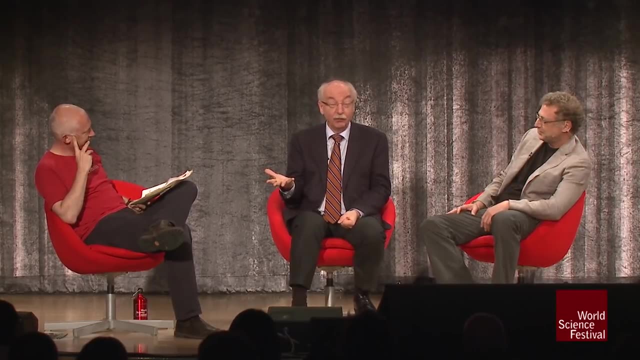 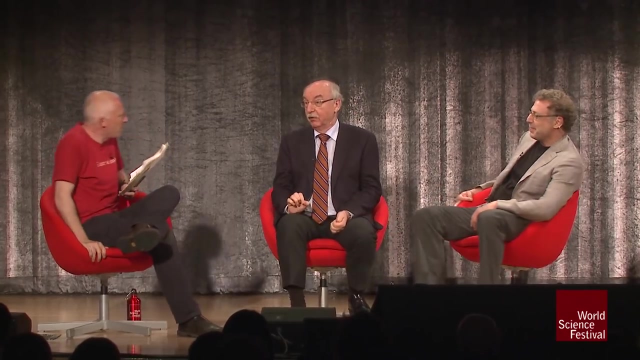 In Washington or around the country, Around the country. yeah, Twenty-four percent, The rest doesn't know it. Germans: Forty-six percent, Don't dare, We learned you gotta watch those Germans. American doctors, what do you think? American doctors? 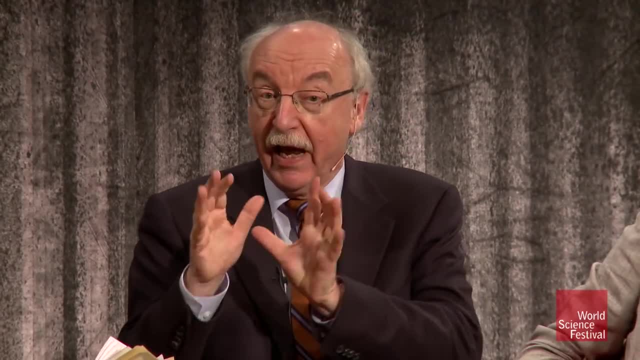 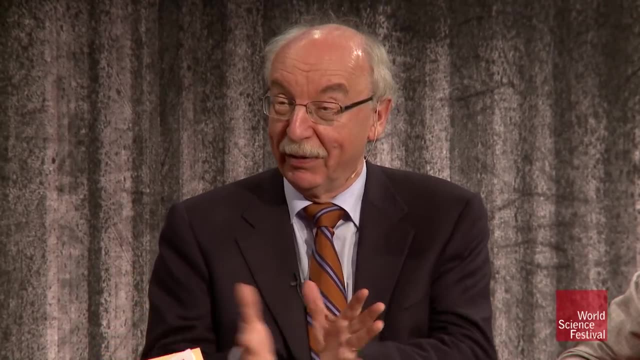 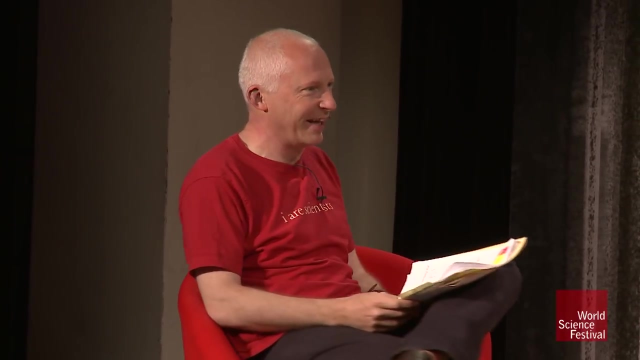 Seventy-five percent. That means still every forced doctor cannot do that. Can you think how that works, How they practice? Yeah, that's a bit frightening Now. I want to come back to Josh now, because you know we've had a lot about how bad and horrendous people are at interpreting data. 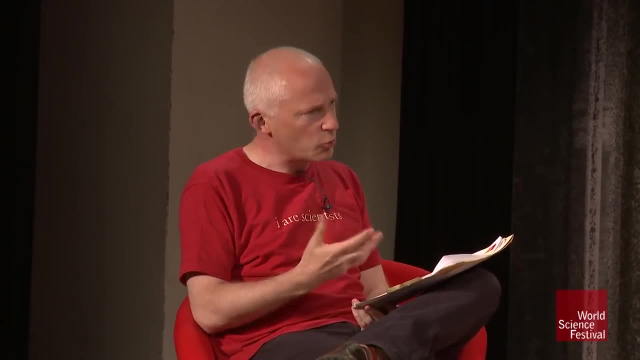 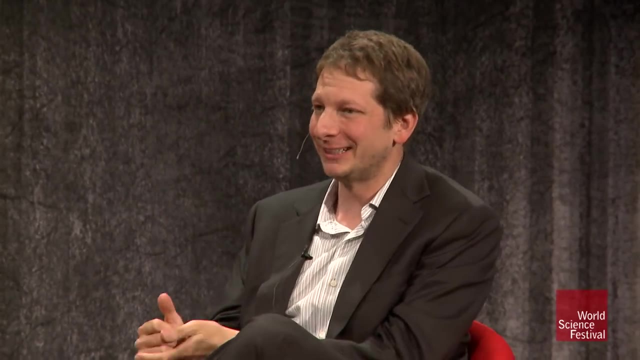 I mean, the telephone conversation is terrifying, I think. But, Josh, you actually believe that people are much better than we give them credit for. So yeah, we've heard all these examples of numbers and units. you know dollars and cents and decimal places. 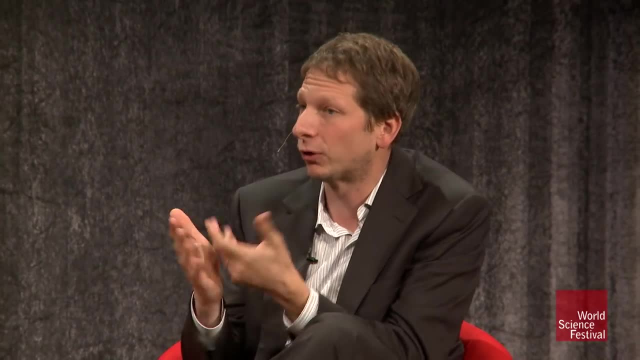 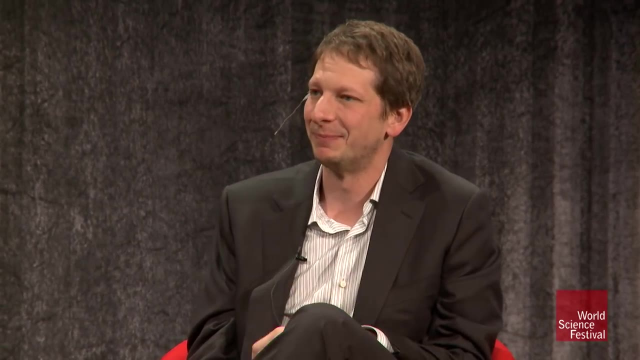 These are cultural artifacts that we've invented to do very useful things Right, And that's what we're trying to deny our experience in the societies that we live in now. But maybe think back to a more prehistoric time and think about the mechanisms in our brains that have evolved for dealing with data. 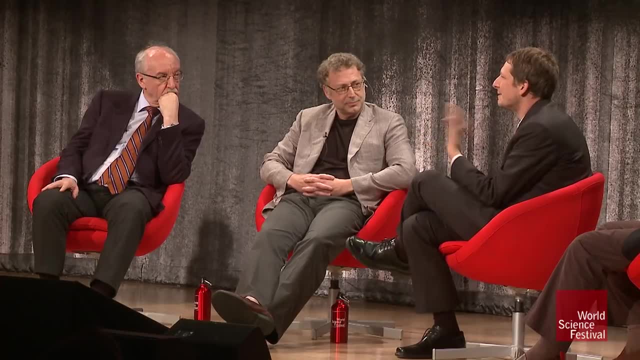 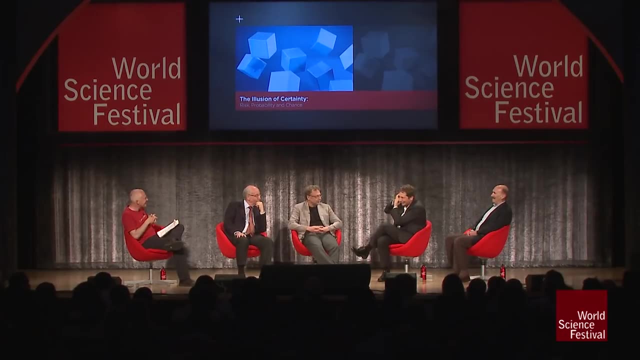 An example that occurred to me as I was walking through Central Park today. well, maybe not so much a park, but out on the savannah, On the savannah, or in the jungle, you see something move behind a bush. What is it? 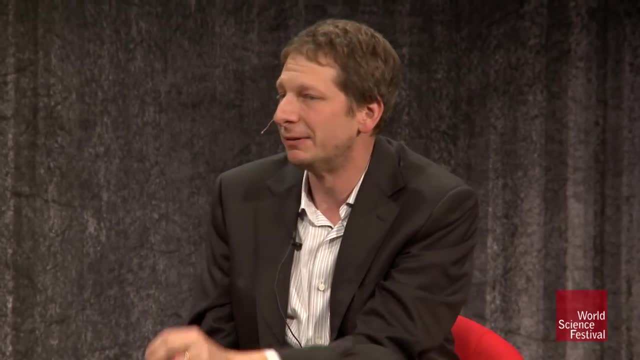 A leopard, maybe, that wants to eat you, or a gazelle, something that you might eat. Right Now we call that in cognitive science or in the study of vision. that's a kind of statistical inference. It's just a good guess. 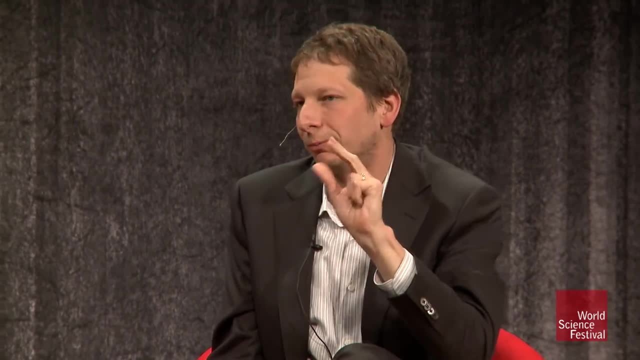 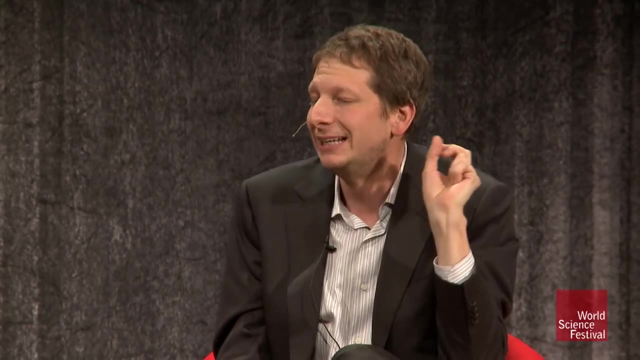 Right. Sometimes you're wrong, Sometimes you're right. What your brain is doing there is seeing data that's in the form of just flashes of light, little patterns of motion all across the visual field behind the bush, And it says: there's something there. 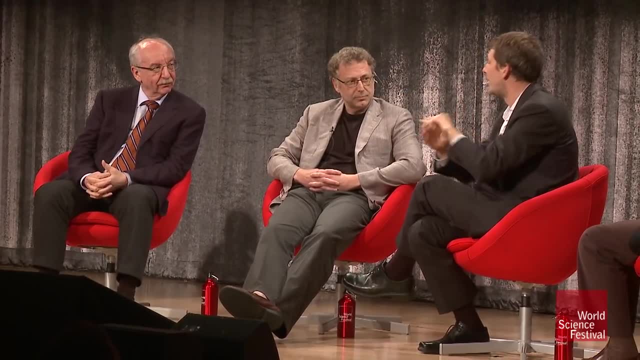 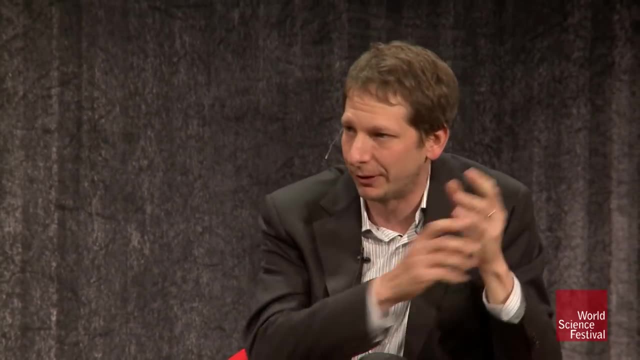 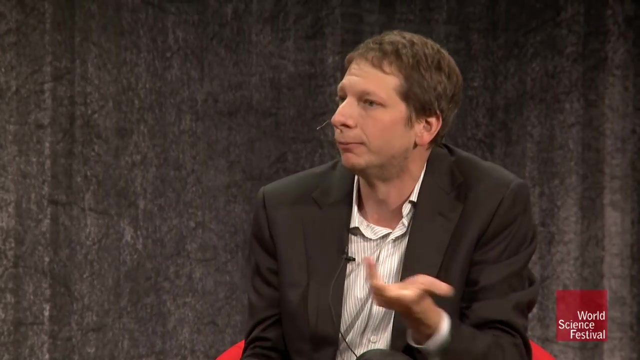 It makes an inference about a thing that's out there in the world to explain that high-dimensional pattern of data. And what we find is that these mechanisms are surprisingly good in that, as the data gets stronger, provides more objective statistical evidence for there being something there rather than nothing, our brains are more likely to detect it. 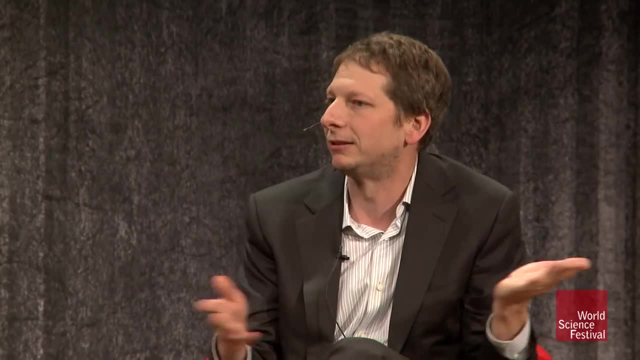 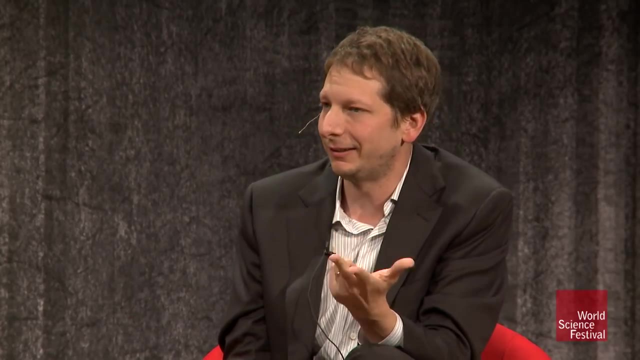 Now, there's also a kind of a bias, which is a very interesting bias. It's one that we see in a lot of other kinds of examples, And it's one that I think also has a very natural explanation. It's a bias, maybe, to be more likely to see things than to not see things, or to see things that aren't there more likely than, say, missing things that are there. 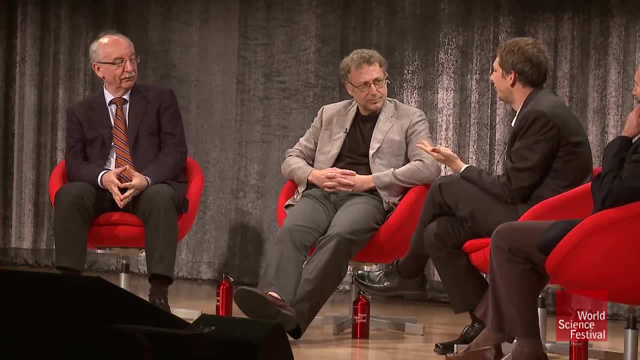 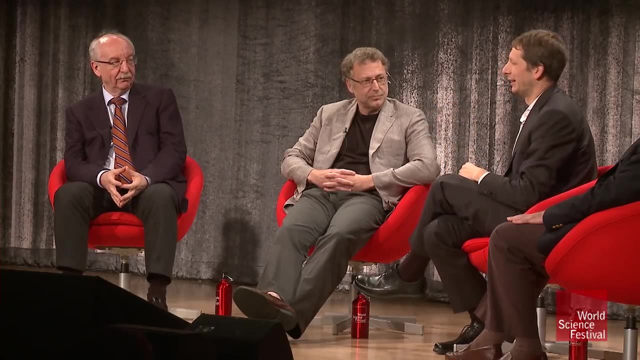 Think about why it might make sense to say: be more likely to think leopard or gazelle when there isn't one than to say no leopard, no gazelle, nothing there when there is one. If there's something there that wants to eat you or there's something there you can eat you, better get it. 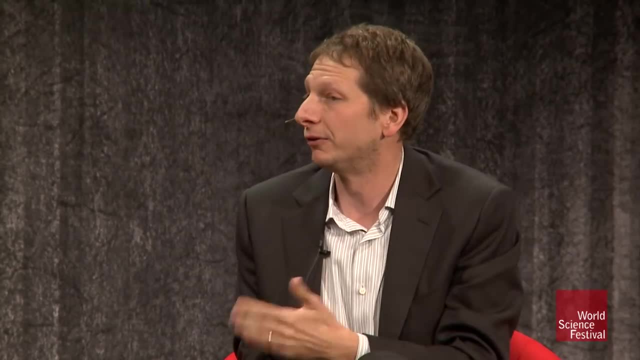 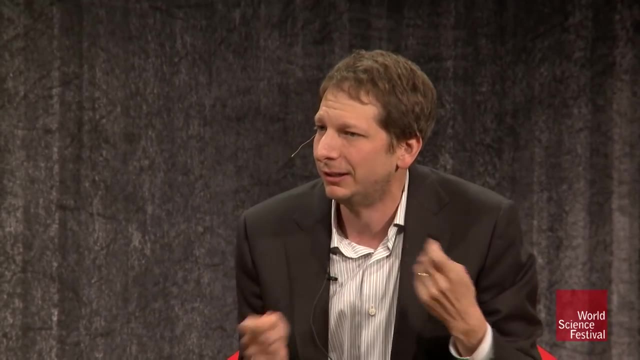 But if you make the other kind of mistake, you see something when there's nothing- well, it's just maybe gets your pulse racing a bit or you jump out and waste a little bit of time. But there's a huge asymmetric tradeoff there in the costs and benefits. 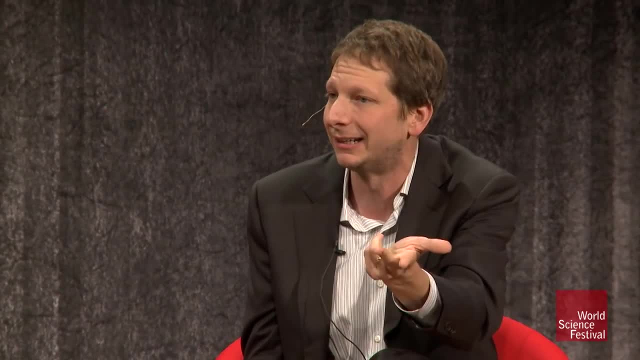 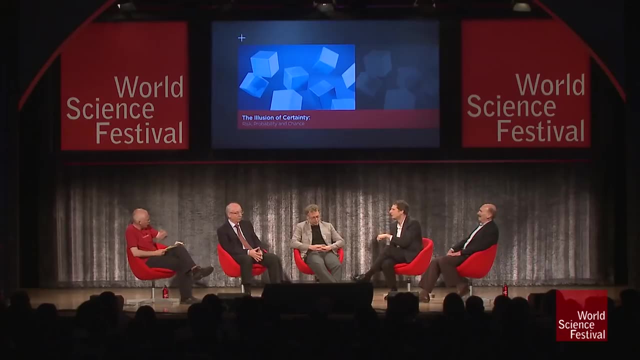 And it makes a lot of sense for our minds to be. We want to be able to detect these patterns and data and maybe make an error on one side in exchange for getting it right when it really counts. So you think we're a sort of evolutionary program to be very good at spotting patterns. 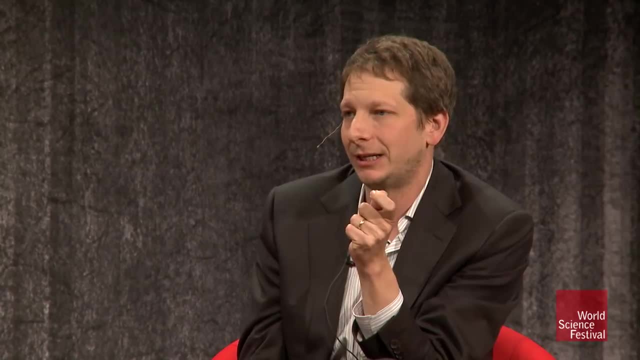 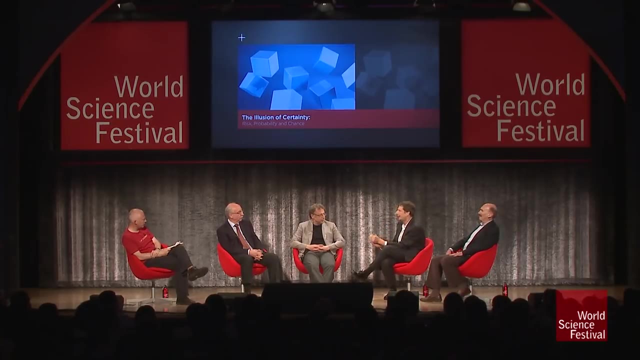 Yeah, with potentially that kind of bias and with the right kind of data. Now is this a good time to show you? I think it's a good time to show your slide. So here's an example from an experiment that we've done in the lab, which takes the kind of data that you might normally look at, say in a table of numbers, but presents it in a diagrammatic form. 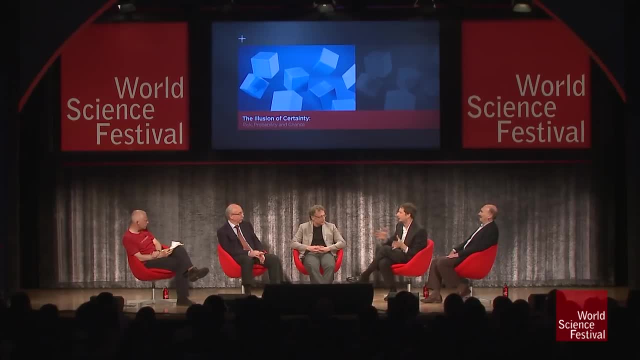 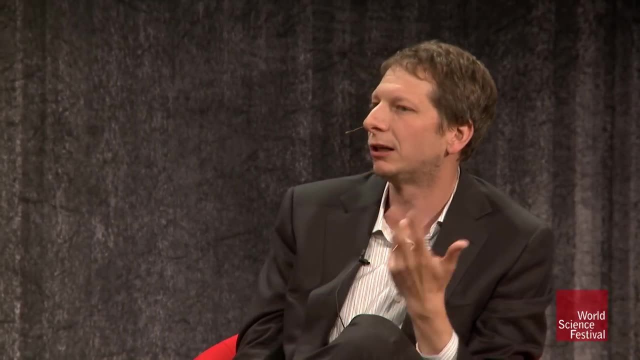 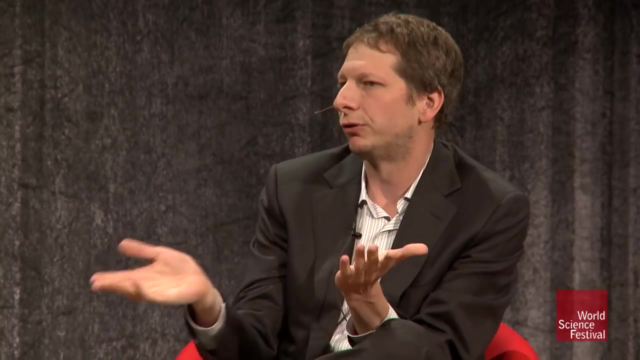 which allows us to see how well tuned our brains are to the amount of evidence in the data. The background for this is a familiar example: what we're used to reading in the paper about, say, cancer clusters or clusters of rare diseases. We often read about cases where there seems like some kind of suspicious coincidence over the course of a year, maybe an unusual number of instances. 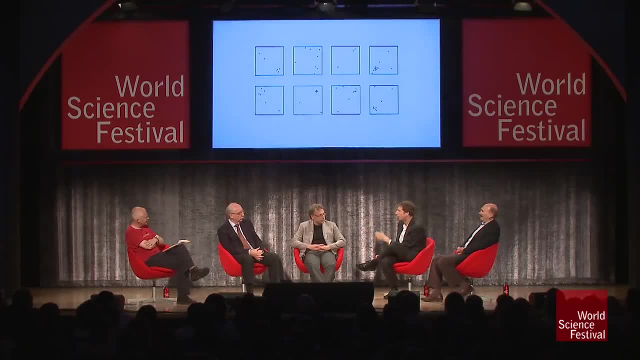 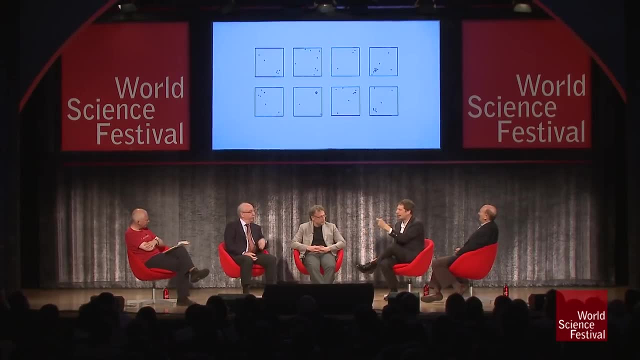 You know the SIDS case, for example. that seems like one of these things, And often it's true that you know what looks like a coincidence, something pointing to some conspiracy or some environmental cause. you know, maybe there's some toxic waste in the environment that has to be dug. 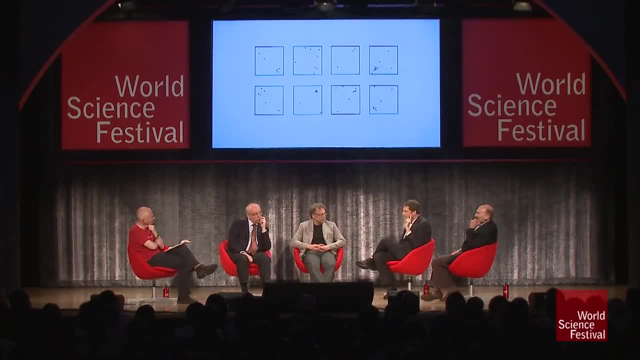 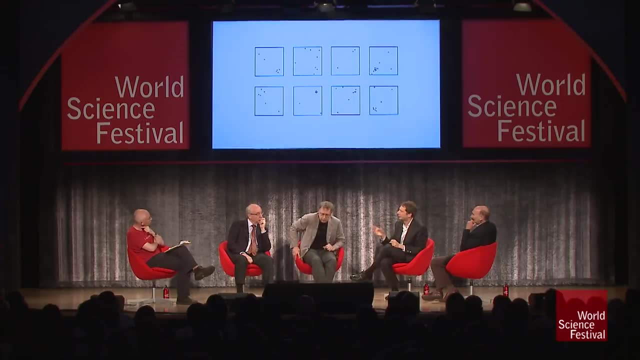 No, it was just a coincidence, right. But what we would say, and what this experiment here shows, is that our sense of what the data are actually telling us is very well calibrated with the objective measure of the statistical evidence for something rather than nothing. 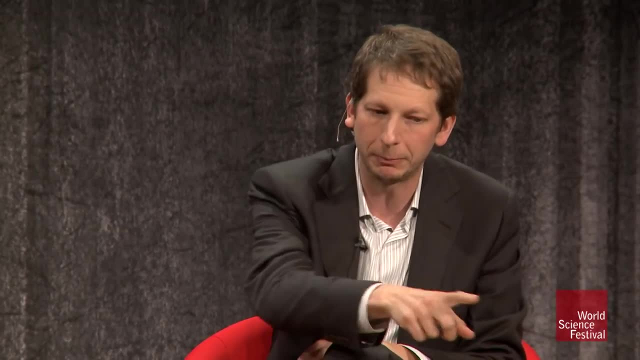 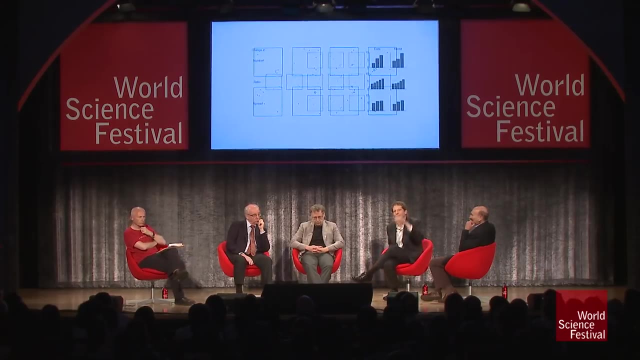 So in an experiment that we do in our lab, we show people patterns of data, these diagrams like you see here on the slide, And you can just go through this and, just you know, maybe raise your hand. Raise your hand just to get a sense of this. 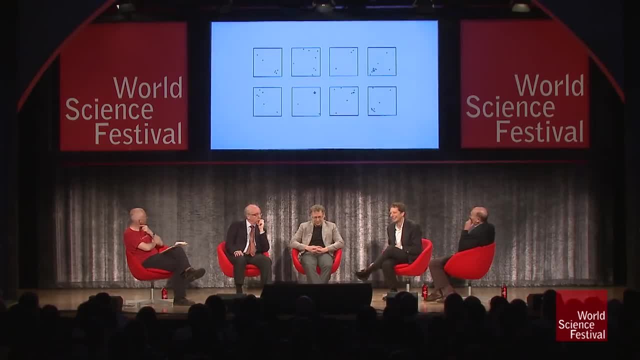 Wait, Sorry, Go back to that one. Don't show them yet. Can you go back to the last one? Yeah, So just say going along the top row. how much of a coincidence. How much do you think there's evidence? 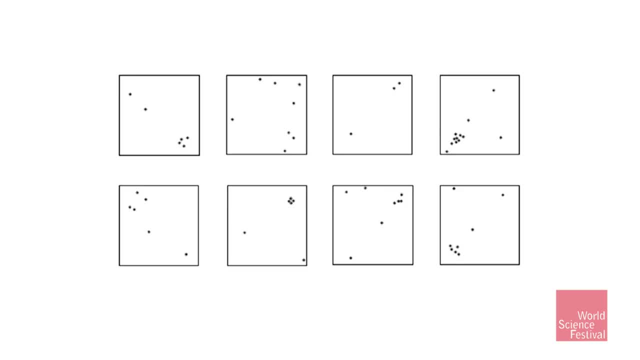 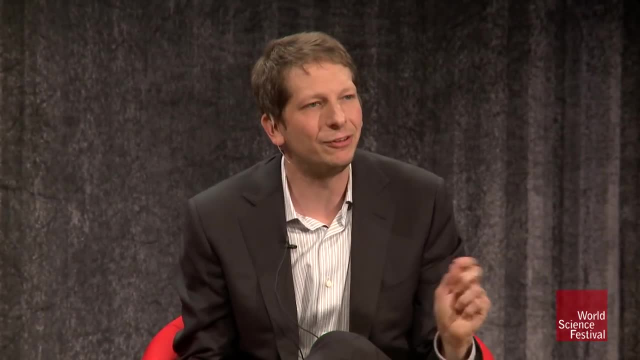 Let's say this is. each dot represents one case of a rare disease that occurred in a year in one square mile of a city, let's say of New York. right, How much evidence is there for some kind of environmentally localized funny thing going on in some part of the city? 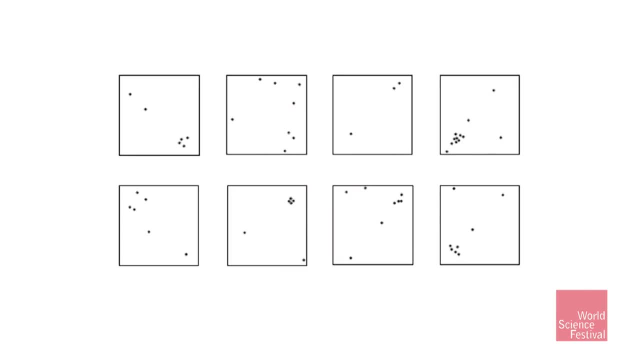 Well say, how about in the first one up in the upper left? Raise your hand High if you think there's a lot of evidence, or low if you don't think very much. Okay, How about the one next to it? Keep your hands up and just raise and lower as you go through. 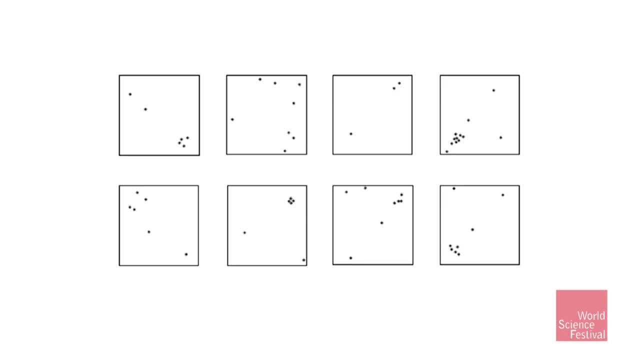 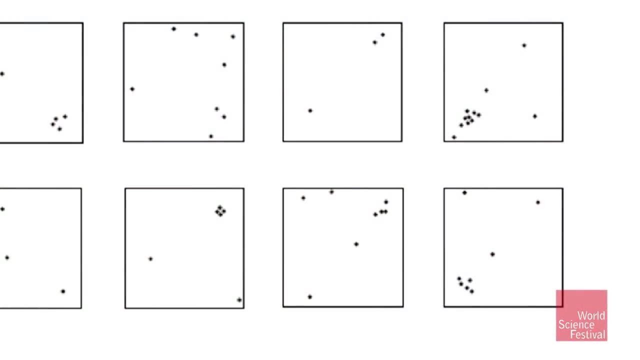 The one next to it. Less or more Less, Yeah, Yeah, Most people say less, Okay. The next one: Yeah. And how about the fourth? the one on the upper right? Yeah, That's a walk-in The upper right. 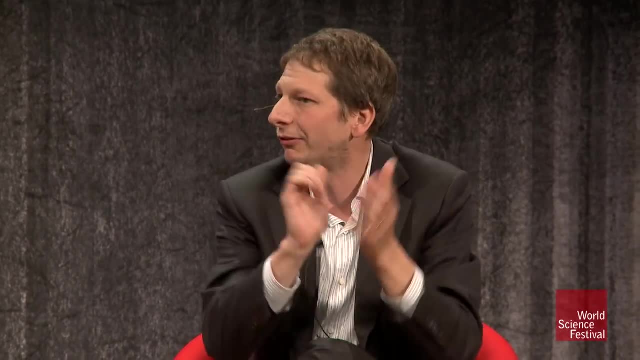 Right, That's right. So we can do this sort of experiment. You just have people you know. look at this pattern of data shown as these dots and rate on a scale of 1 to 10.. And what the next slide shows is just some of the results from experiments. 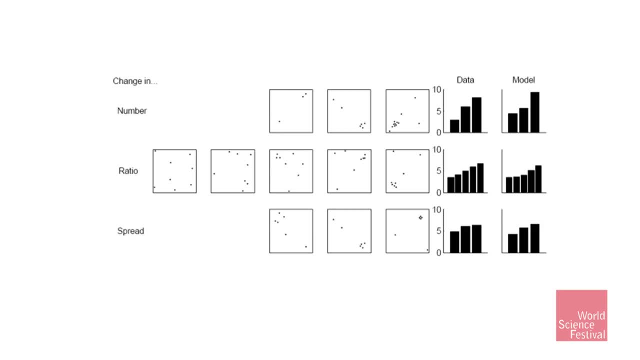 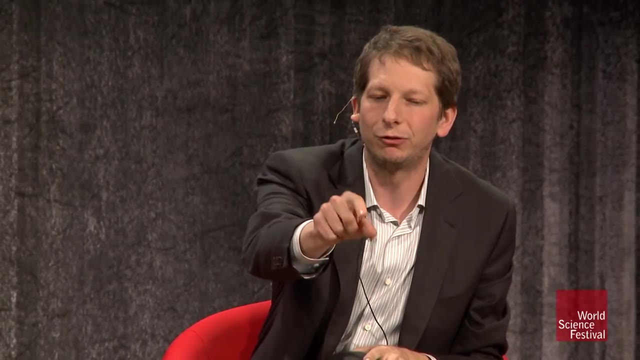 We've done many experiments like this. What you see here is we're varying across these different stimuli factors which, in an objective statistical analysis, provide more or less evidence for there being something there, some spatially localized hidden cause, And what you can see, what we call. there's these two bar graphs there, one called data and the other called model. 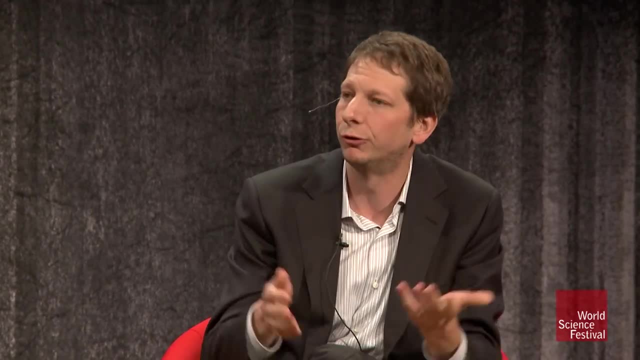 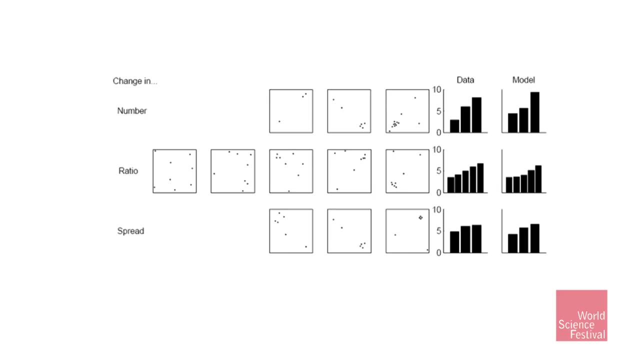 The data here are behavioral data from people from 100 or 200 subjects. average judgments on a scale. The average judgments on a scale of 0 to 10, where 10 means there's definitely something funny going on and 0 means nothing- it's just a coincidence. 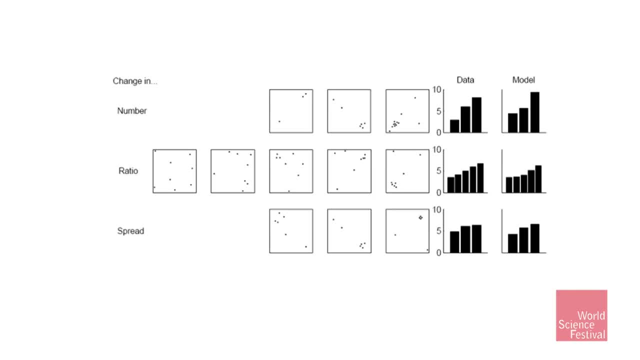 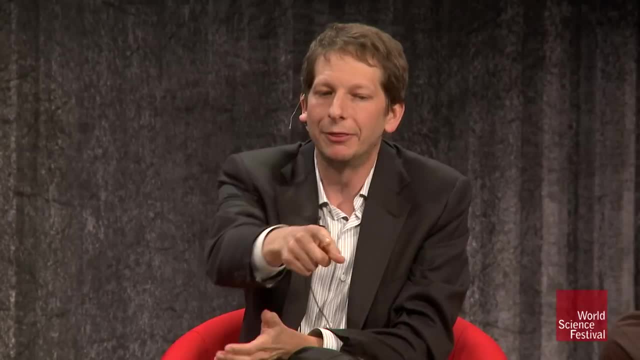 And what you can see is that you know, just like you had your own intuitions there, people are giving you more or less of a sign in their gut feeling that there's something, rather than nothing, in these different cases And the model there. that's this objective statistical measure of evidence. 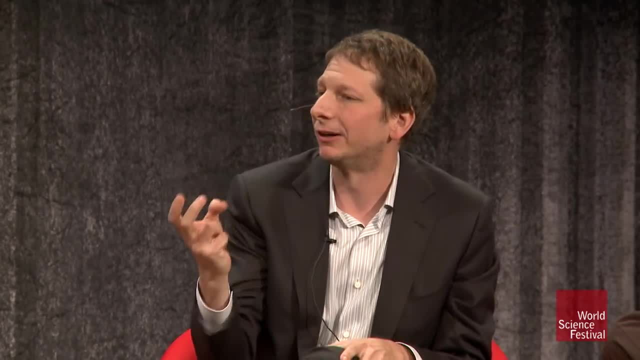 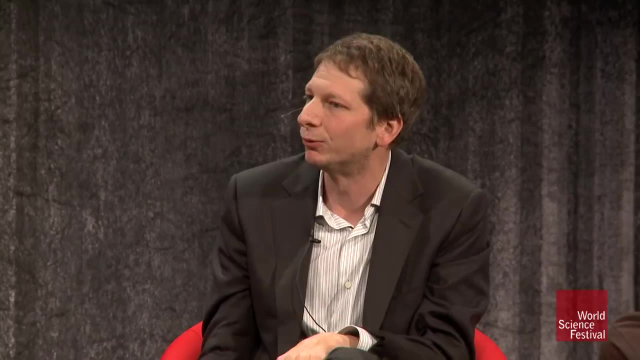 It's what we call a log likelihood ratio. It's what the data are telling us, as opposed to separately from what. I guess we might talk about this later when we talk about probabilistic reasoning, what you might call the priors and bays rule. 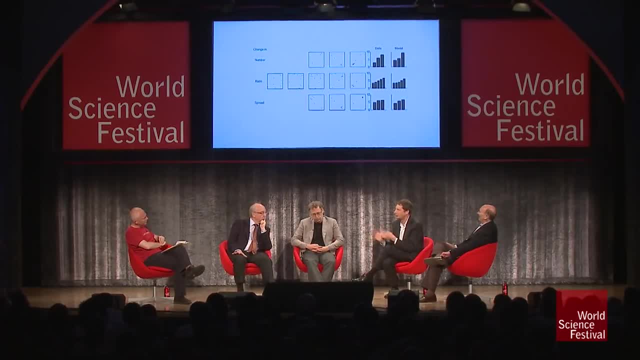 It's just about the data. It doesn't take into account the costs or benefits of getting it right or wrong. Just how much structure is there in the data? And it's almost perfectly calibrated with what people are giving you. there It goes. there's a big difference when people say there's a big difference and a little difference when people say there's a little difference. 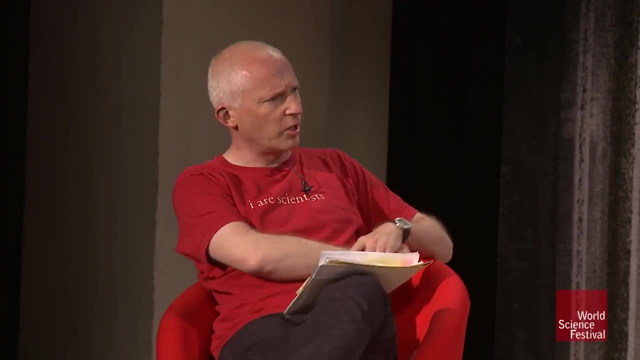 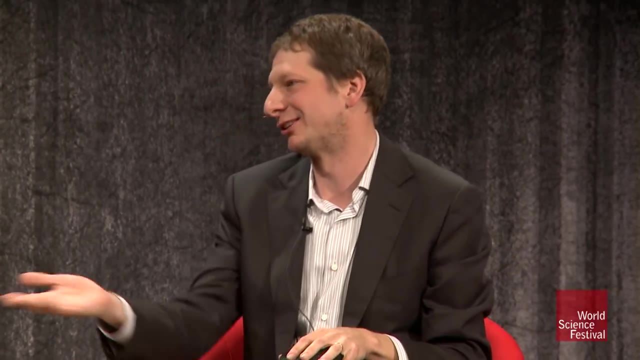 And it almost turned into numbers. Yeah, if you presented the same data as, like, a table of, you know, An Excel spreadsheet, Yeah, probably most of us wouldn't know what to make of it, right? Yeah, Just like I didn't know what to make of your you know some of the examples. 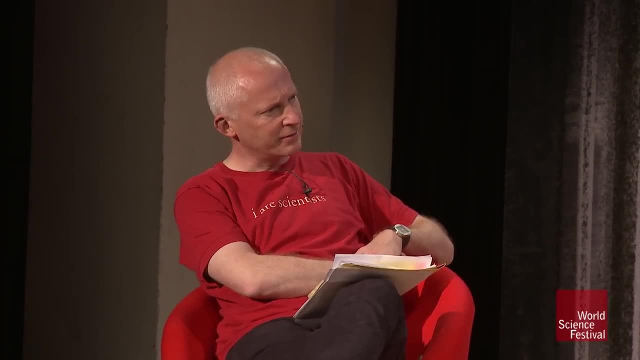 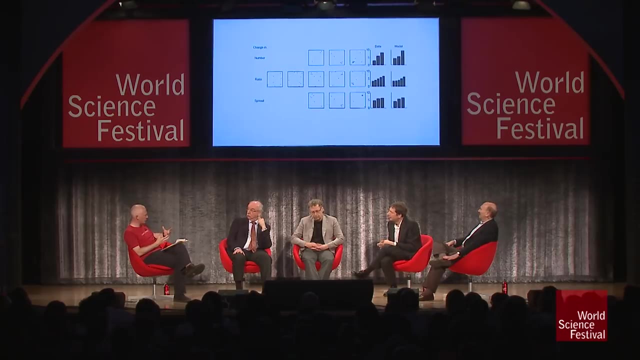 Yeah, Some of the examples of the miles in the car and the airplane, You know those kind of numbers or billions or gazillions, So yeah, yeah. So you think that that's sort of a more sort of later cultural development? 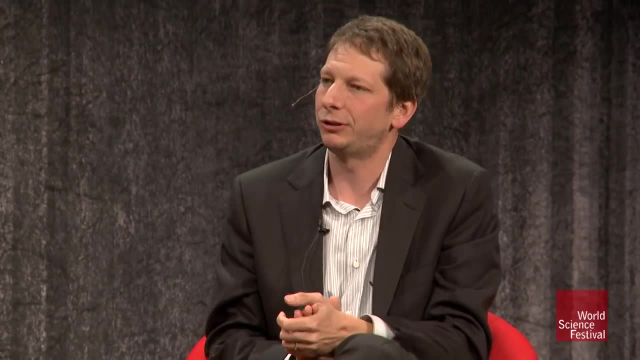 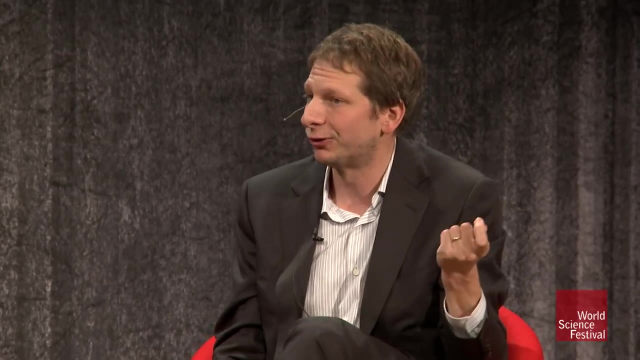 Well, right, And there's, for certain purposes, for computation, calculation, We do need numbers, right, But we also, you know why do we have diagrams like this? It's a different cultural artifact that's designed to take the patterns of data, or patterns that are in data, and present them in a way that our brains know how to do the right thing with. 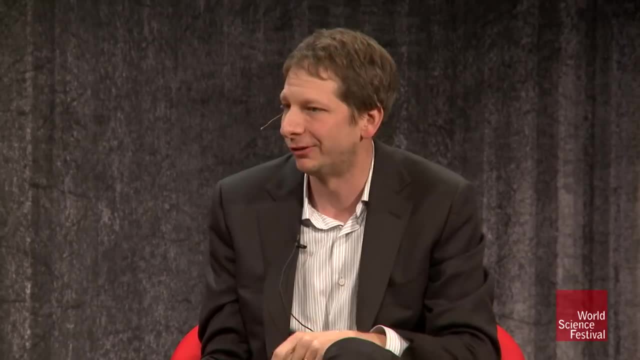 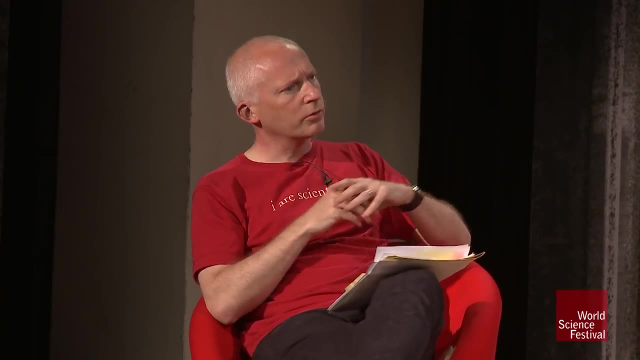 It's taking the mechanisms that were evolved to you know, find the leopard or the gazelle behind the bush and put them to work finding what's really out there in the data that we have in our environment today. Yeah, I have a question about that. 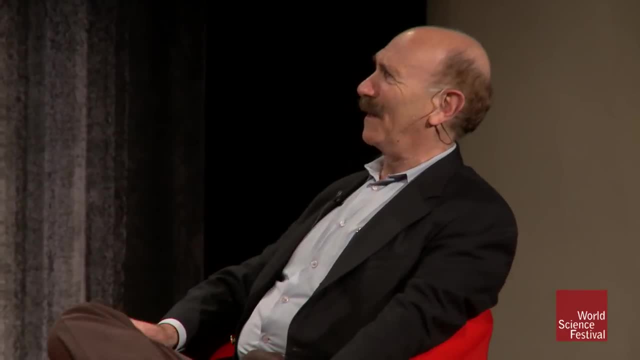 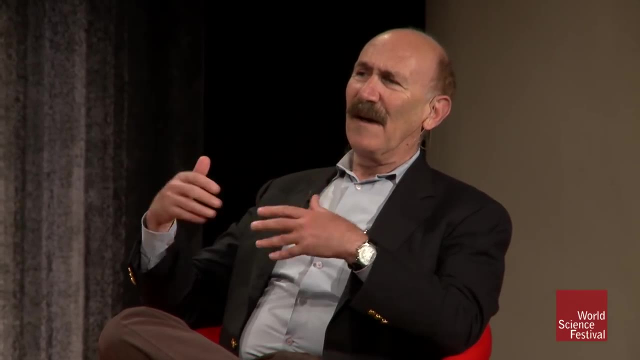 Actually, my question is to you, Marcus. You've been asking us questions. Yeah, Okay, Go on. Yeah, As a mathematician, I have a problem with data that looks certain ways without a probabilistic structure behind it, And I want to ask you about Fristenberg's theorem. 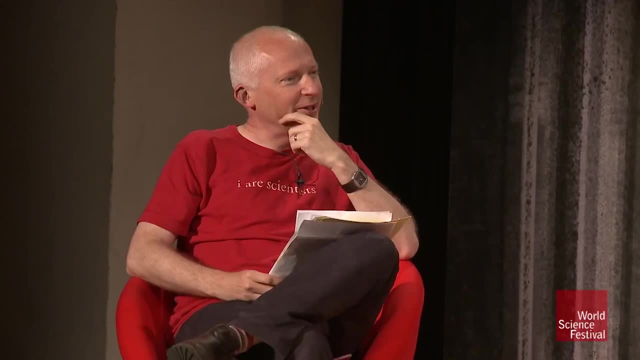 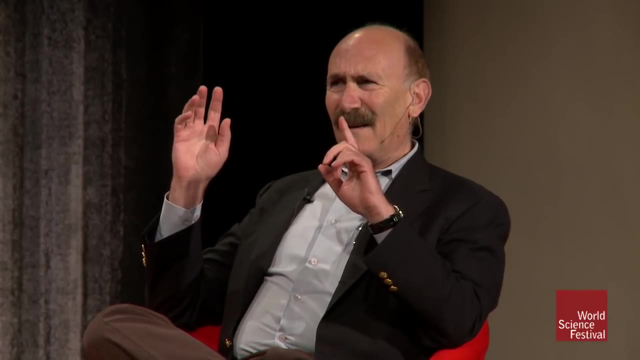 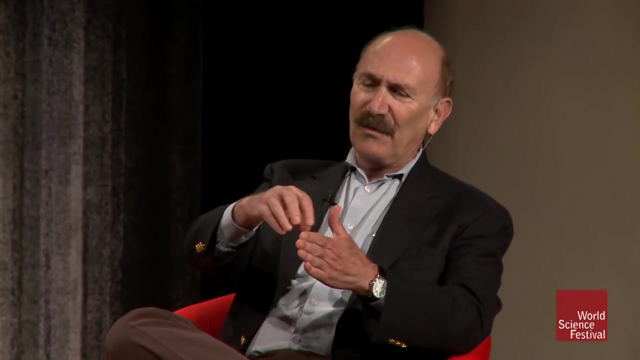 I think you know him. Yeah, I know Fristenberg. Yeah, So Fristenberg's theorem allows you to find any kind of pattern you'd like, So sometimes you can look at data If you don't have an inferential structure where you have a population and you draw a random sample and the sample has to be random from this population. 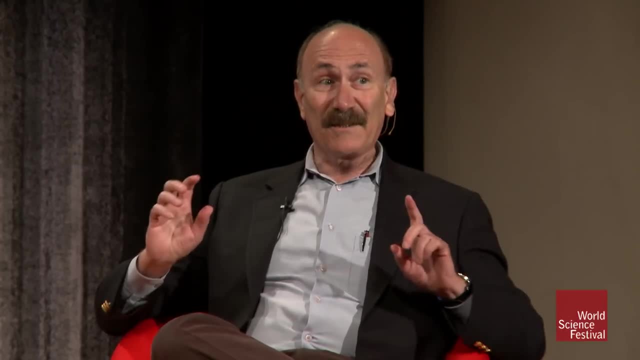 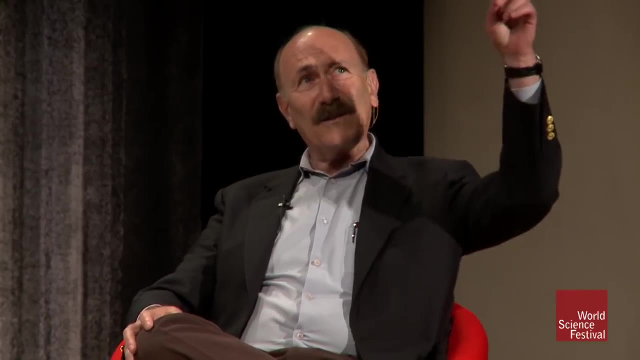 you really get into problems by interpreting structures that you see. Basically, Fristenberg's theorem tells you- I think it's in the movie A Beautiful Mind where he points to the sky. Yeah, And it's not, for I forget what it is like a kite or some kind of structure. 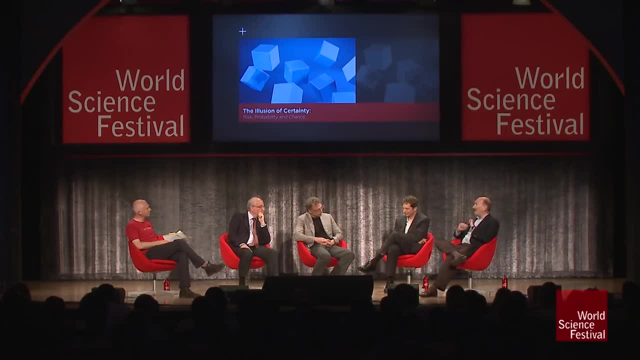 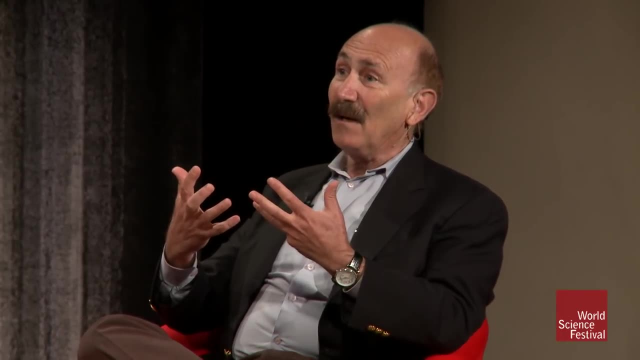 You can always find one when you have data. You just have to look at it in the right way. So I think we have to be very careful when looking at data visually, because we can be fooled Exactly, And that's why often it's important to turn it into numbers. 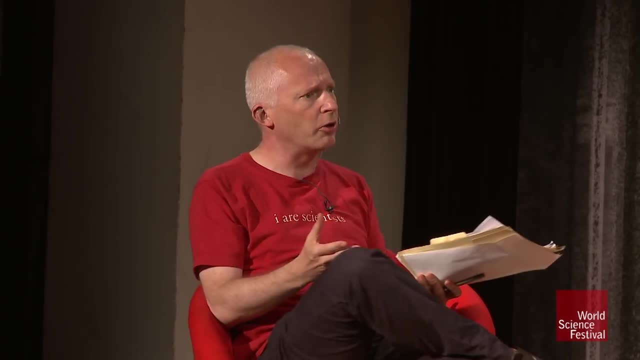 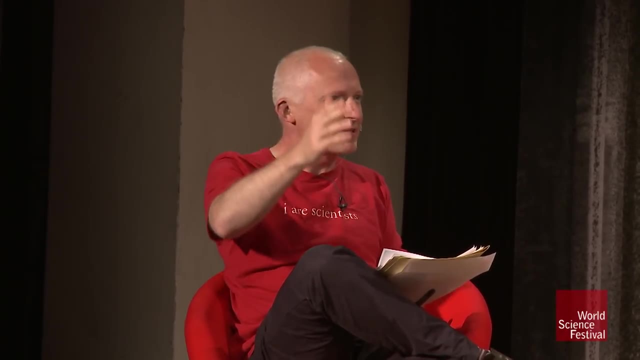 But I think even when it's turned into numbers, we can be fooled. I mean things like the Bible code. you know, really that's a probabilistic argument, saying you know these are unlikely numbers. You know unlikely events. 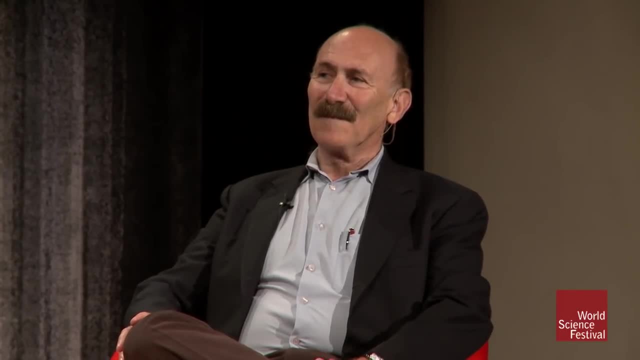 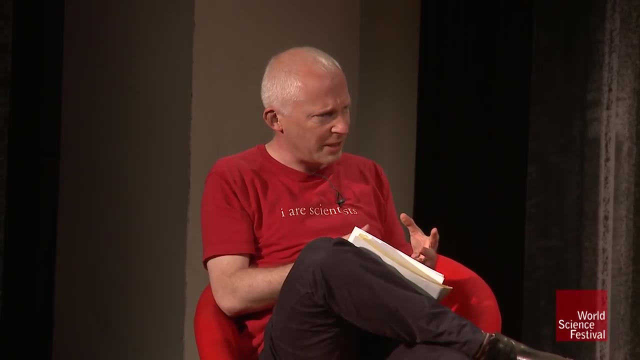 And so perhaps we can turn to probability, because you know that's a way of trying to interpret numbers and data. So, Amir, I mean actually it's quite a late development in the history of mathematics. Probability, you have a roll of a dice. 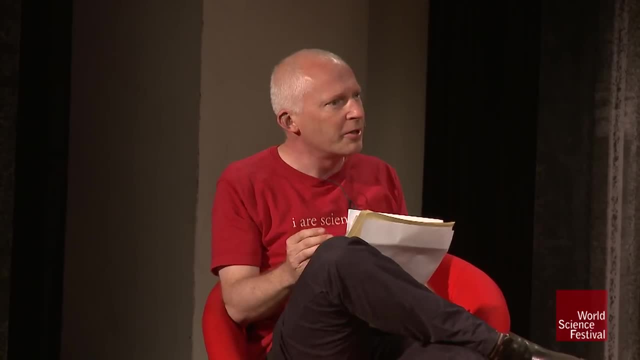 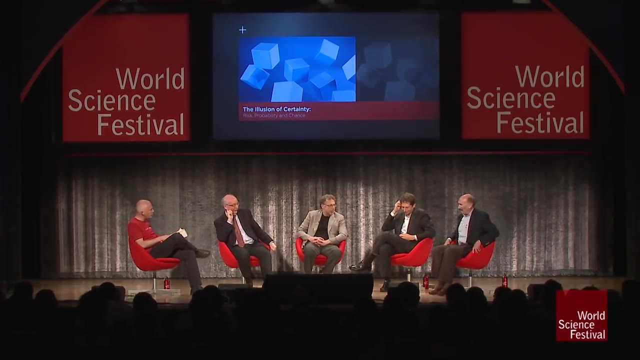 It didn't look like it'd be something that could be mathematized. 1654.. Right, So yeah. So perhaps you could tell us a little bit about how we managed to make mathematical analysis of something which, at chance, doesn't look like it could be mathematized. 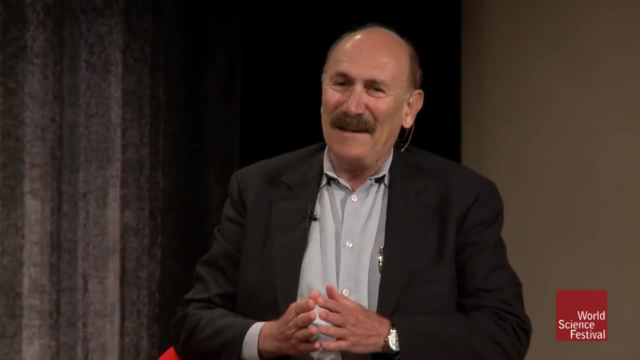 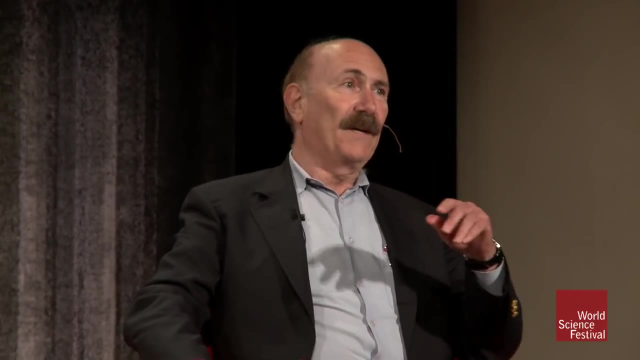 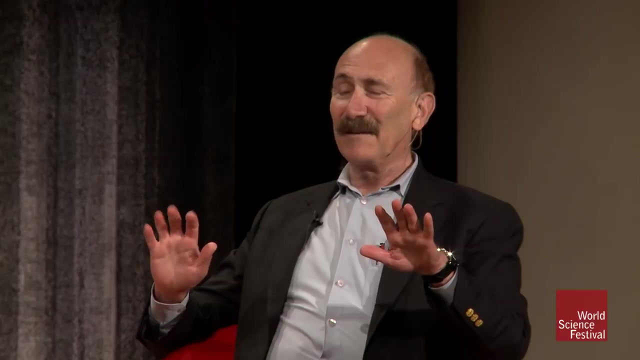 Good Math is about certainty. What I had in mind was a game called the birthday problem. So there are about 380 people here. Actually, they're missing. There are some seats that are empty, So I think we're about at 365.. 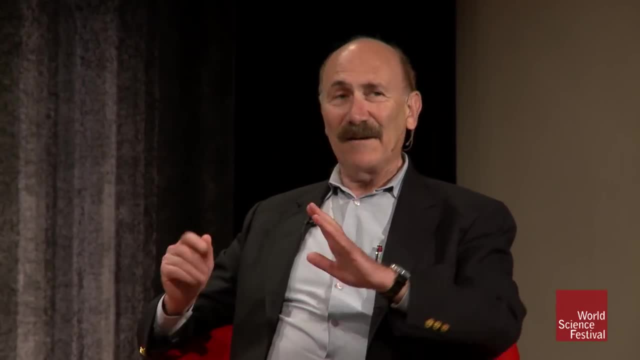 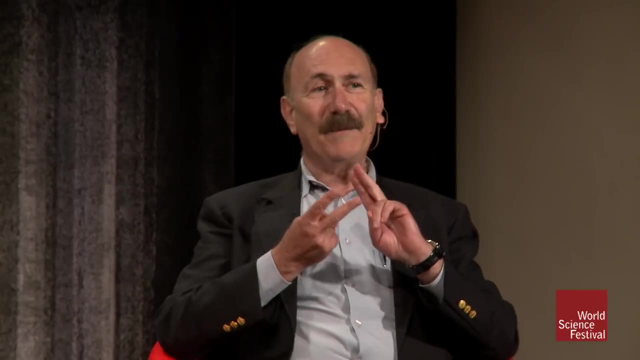 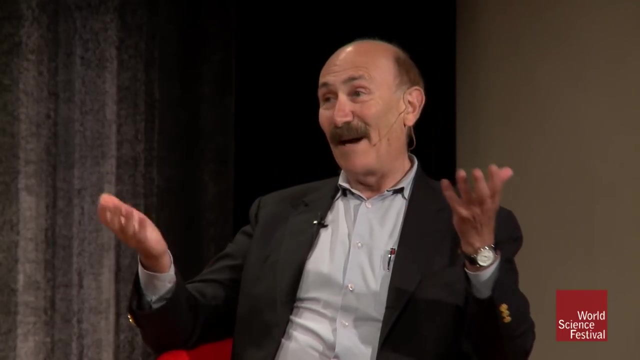 So as many days as there are in a year, there are people in this auditorium here roughly. So the question is: what is the probability that two people share a birthday? Now, obviously, if there are 365 people here, then the probability is well one. 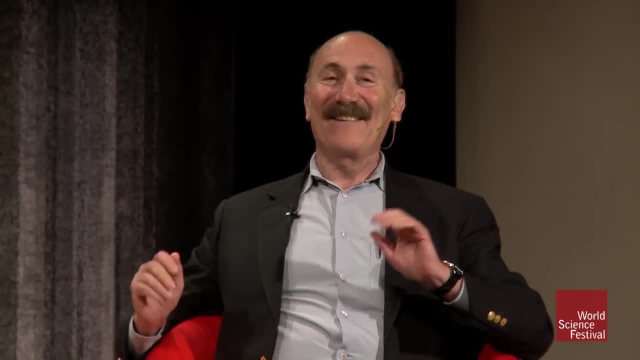 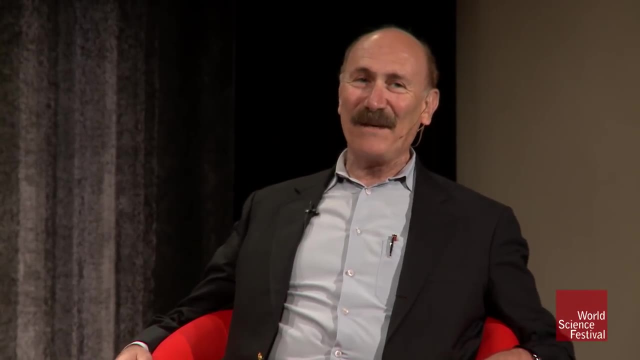 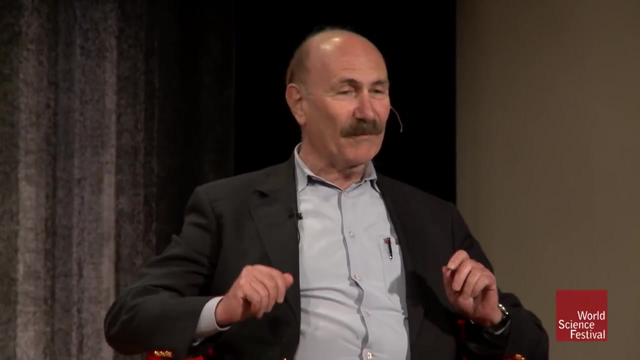 Well, 366.. Yeah, and 66,. the probability would have to be one. I think everybody would agree with that, But probability theory teaches us that the probability is quite high with even a much, much smaller set of people. So I'd like to play this game. 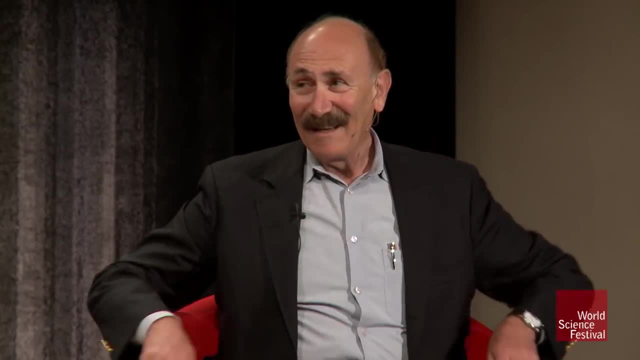 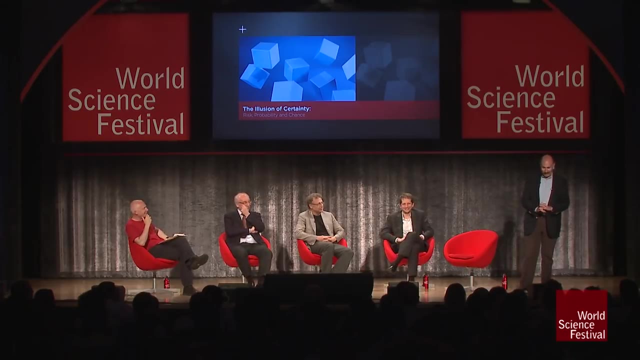 Sometimes it fails, So if I fail, forgive me. That's the trouble with probability, Right? That's exactly the problem. That's why I hate the subject Probability. So I think people ask me if I get nervous. I only get nervous now, in case it doesn't work. 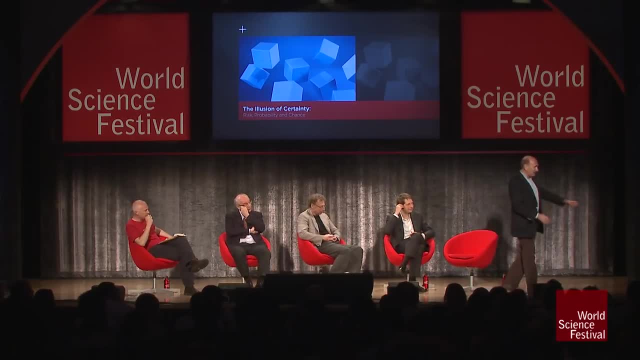 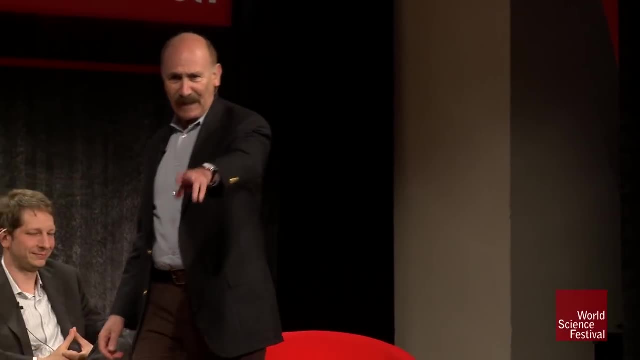 Yeah, okay, So here's what I'd like to do. There are six people here and ten here, Nine right: One, two, three, four, five, six, seven, eight, nine. So that's a total of 15.. 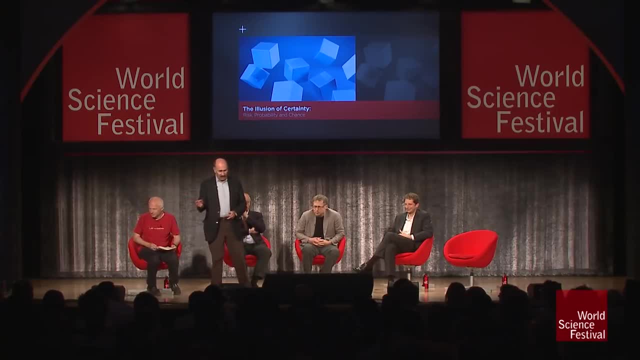 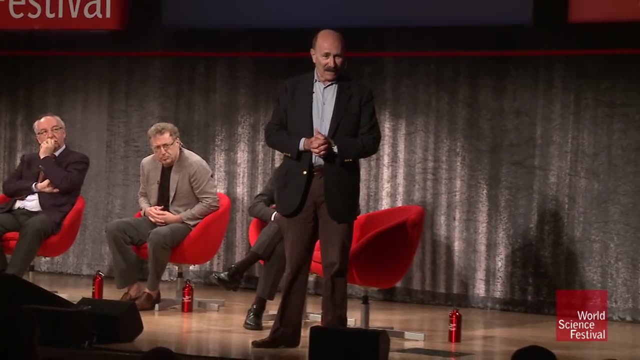 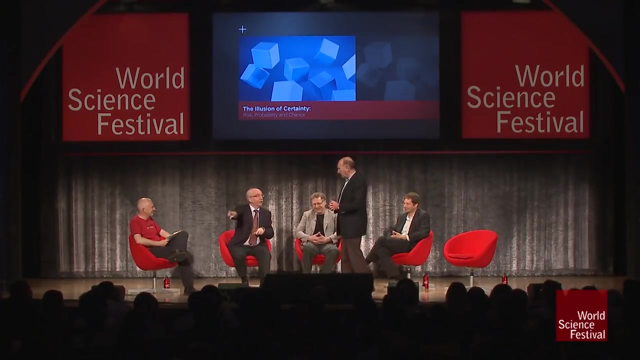 The next row has 12 and three here, So that's 15.. And what did we say here? Twelve, Twelve and three. I think that gets you to third, Twenty-eight, I'm sorry. Sixteen and twelve. Sixteen and twelve. 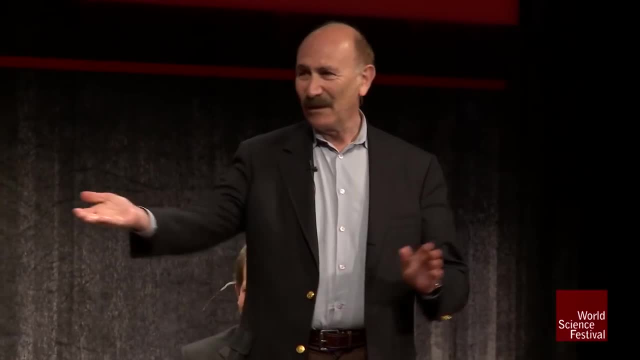 That's 30 people, right, Roughly Twenty, Twenty-eight, Okay. You said mathematicians can't count. Yeah, that's right, We can't count Twenty-eight people. Do you know what I mean by mathematicians? 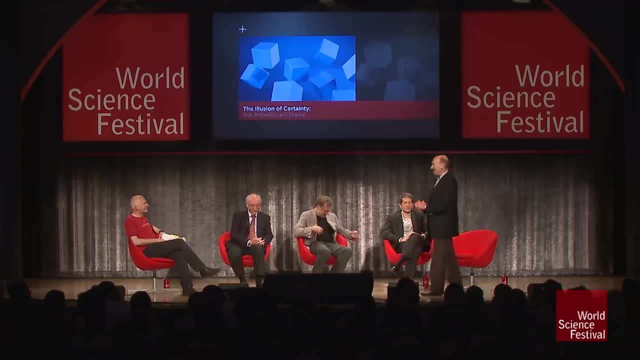 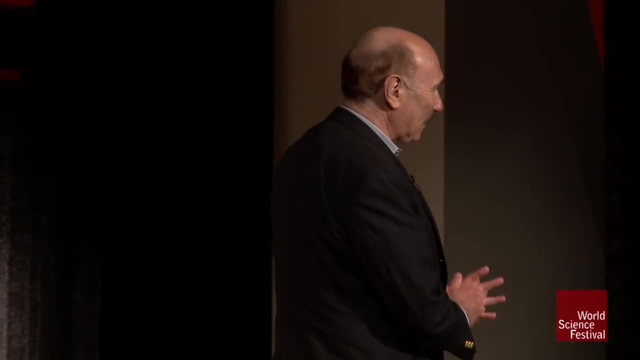 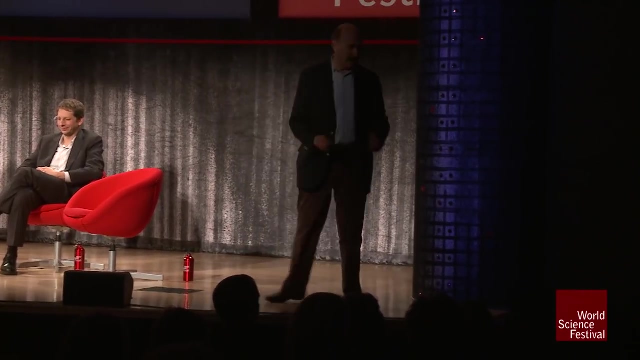 I know a mathematician who can't do the. you know the tip needs a table for the 15% tip, So we're all the same. So what I want to do is to have the first person here say aloud your birthday, if anyone. 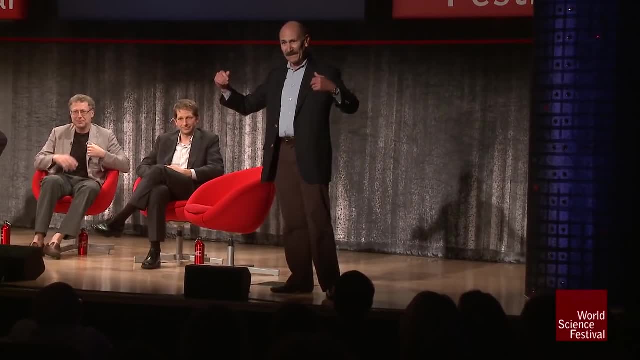 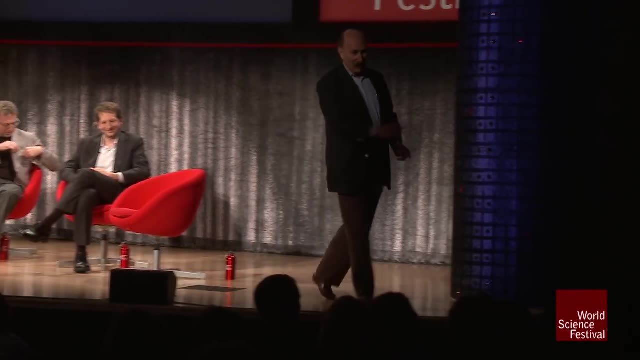 here in the first two rows here, which is a much smaller set than the whole auditorium- matches. I want you to say bingo or something, or match. So I'm going to go around and I want you to loudly say your birthday. 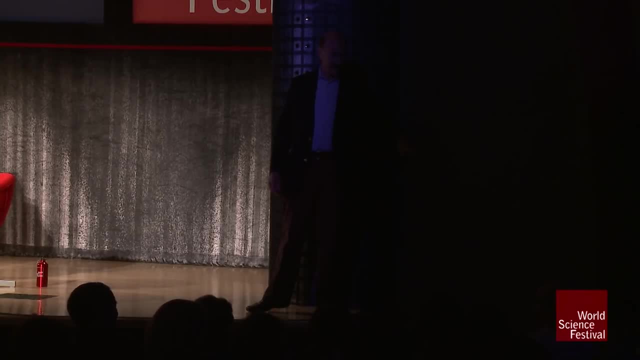 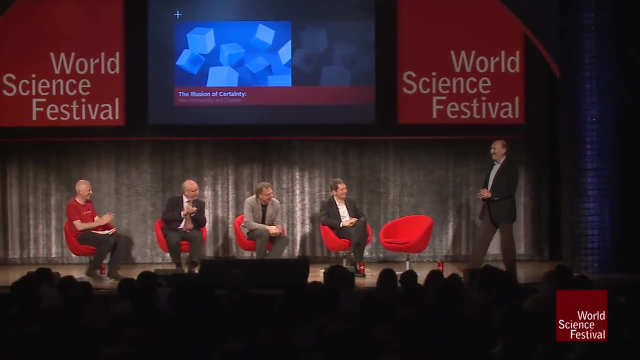 Not the year, just the day and month, November 6th. I match with you. Oh, well, done, That's a, But I'm not sitting there. Yeah, you're not sitting down there. I'm not sitting down there. 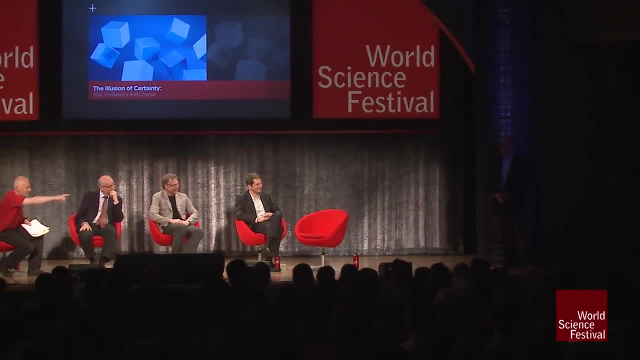 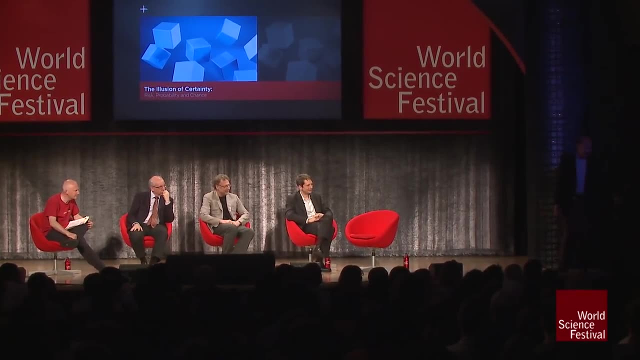 So you don't count, That's probably your twin brother over sister or something. Sister right, January 4th, Everybody heard January 4th. Okay, October 18th, October 18th, July 25th. 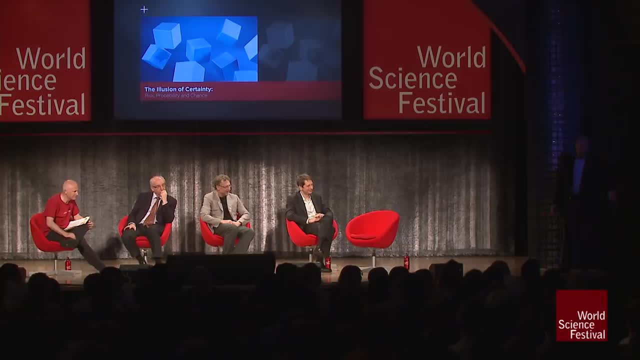 July 25th, May 21st, May 21st, August 21st, August 21st, That's a match. Oh my gosh, You're going to November 14th, November 14th. 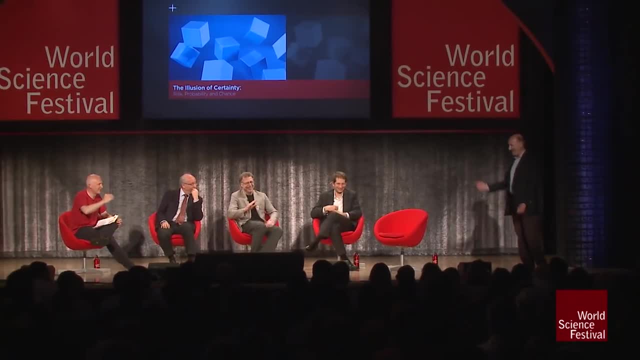 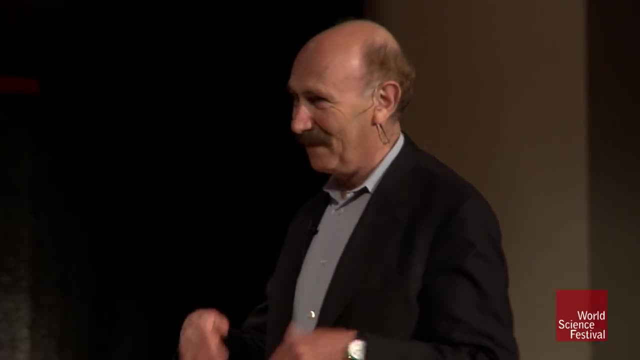 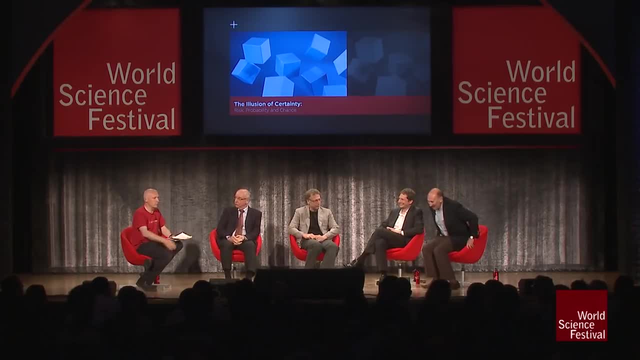 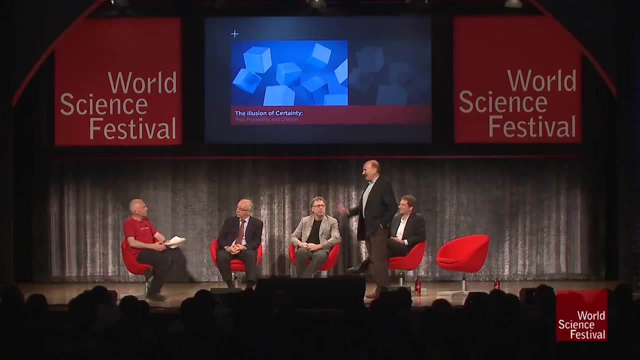 But it worked, So let me explain it, I guess. Yeah, yeah, Why is it so? Okay, I think most people's intuition: you might need about 150 people or something. Yeah, I think we talked about the two soccer teams. 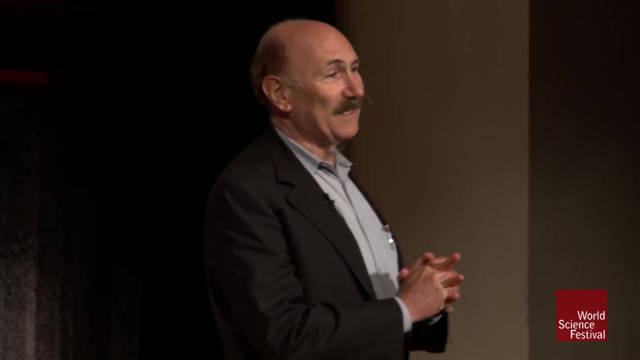 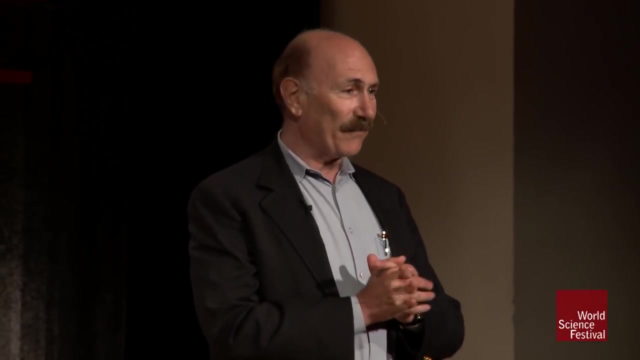 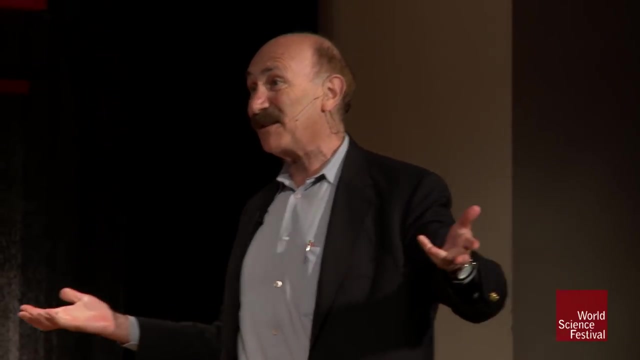 Well, 23.. With 23 people, the probability is already 50%. Twenty-three people: 50%. With 30 people, it's 70%. With 40 people, it's 90%. Imagine there are 365 days with 40 people, 90% probability that they'll match. now why? 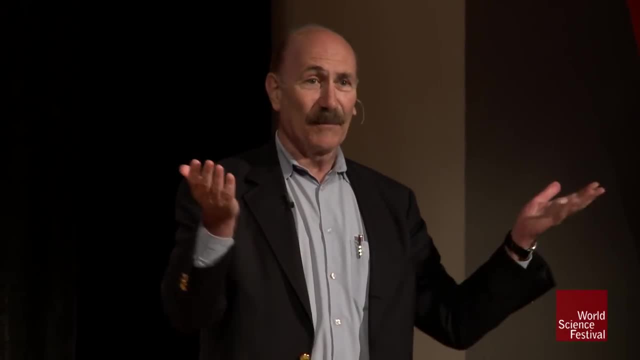 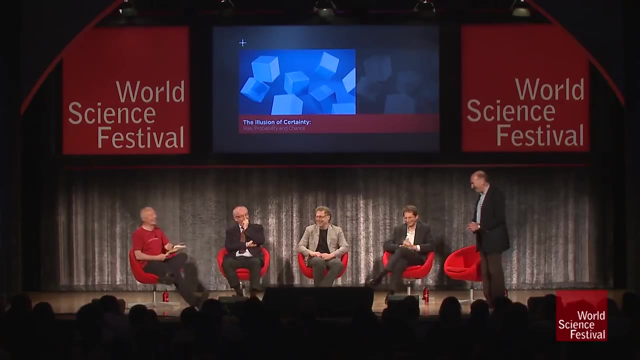 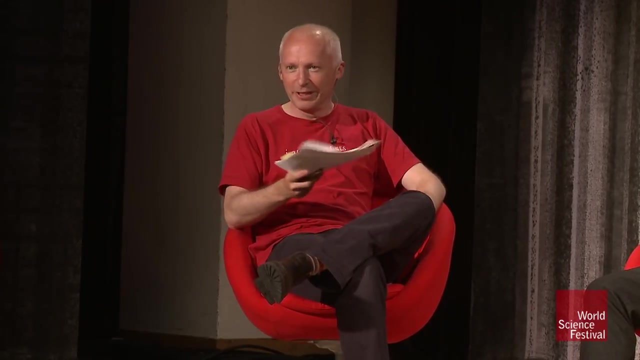 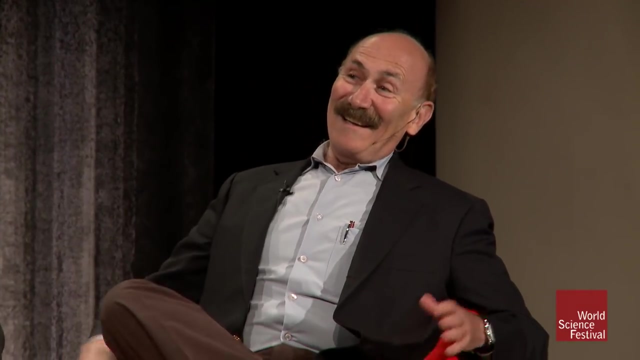 is it? why does it work? does anybody have an idea? yes, so the answer was that there are more periods of time when people might be likely to have the children. no, that's not the answer, is it? I mean that that's the biologist answer and the mathematicians answer. it's actually a good answer because you get. 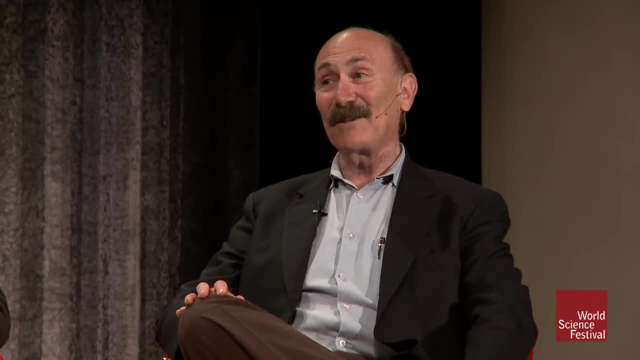 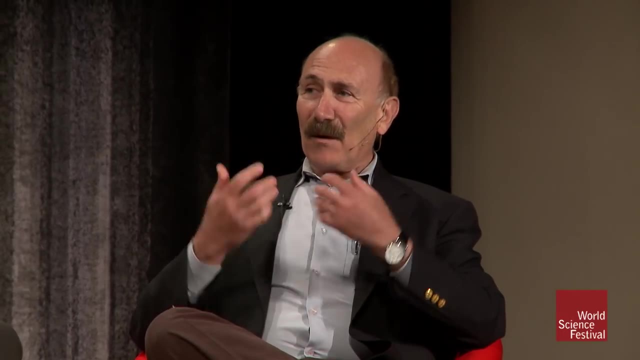 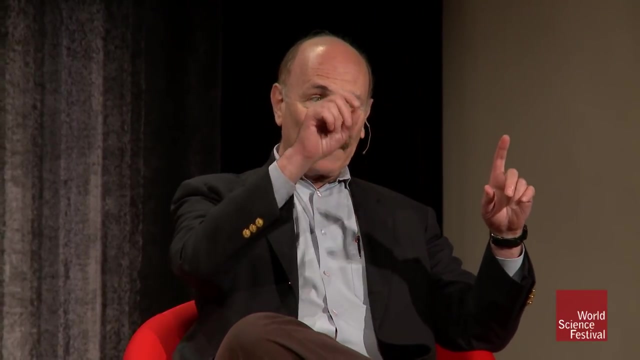 congregation unevenness. so it's actually a very good answer. but even if that doesn't happen, you do get it, just because of the way the numbers work. so to prove this, the rule for finding the probability is 1 minus 364 over 365 times 363 over 365, and so on up to 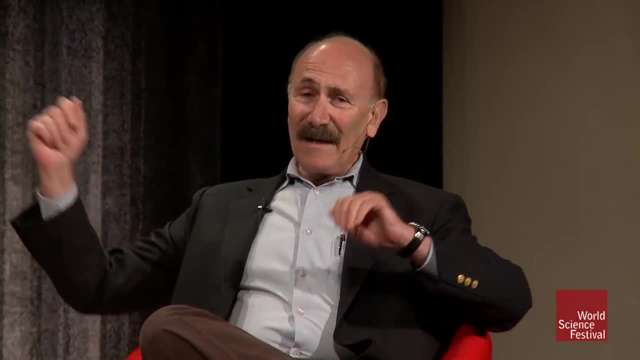 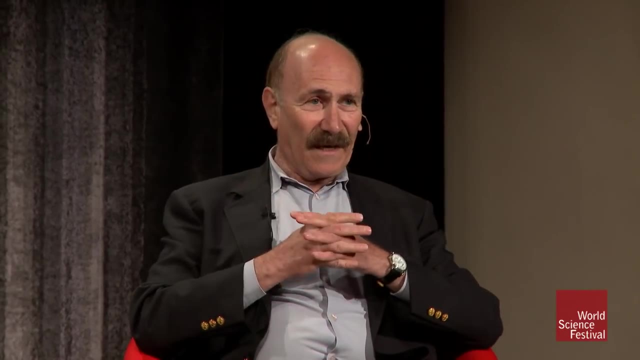 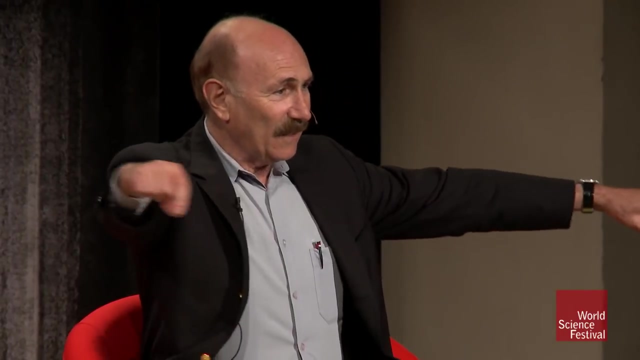 20, 23 of them or so, or 30 or so on. the reason is that the way to explain it in the best possible way is in a sort of a, a mental experiment, or you know. what you have is 365 little boxes here. imagine 365 boxes that are lined here and their 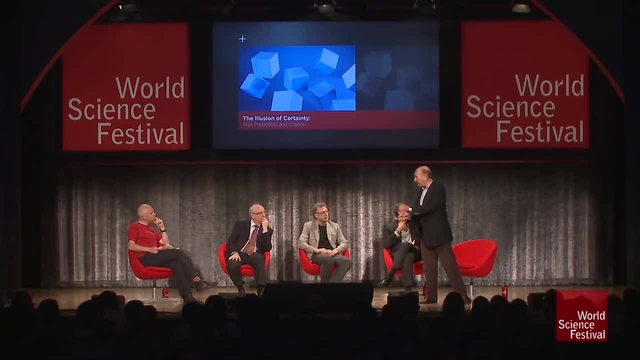 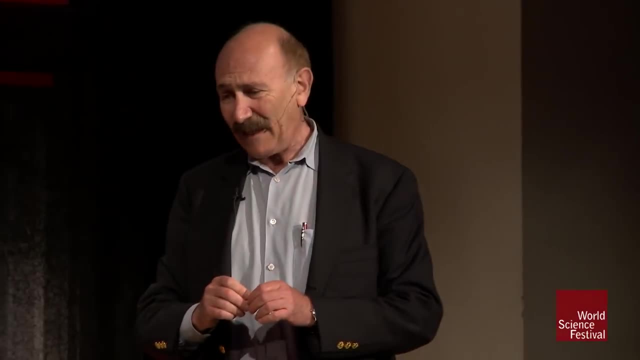 little balls that fall down from the sky and fall into these boxes. now you say there are 365 boxes. that's a lot of boxes. what's the probability that it will match? you say: well, there are lots of places. every ball can go right. we all agree on that. on the 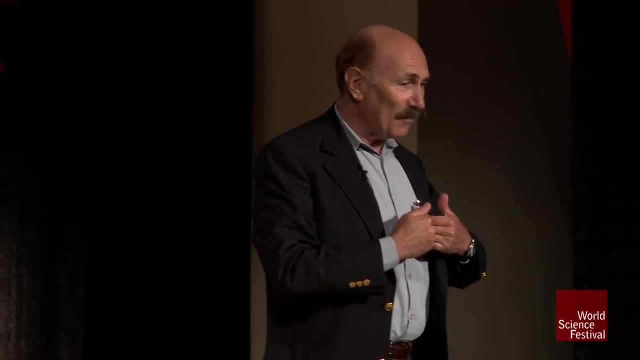 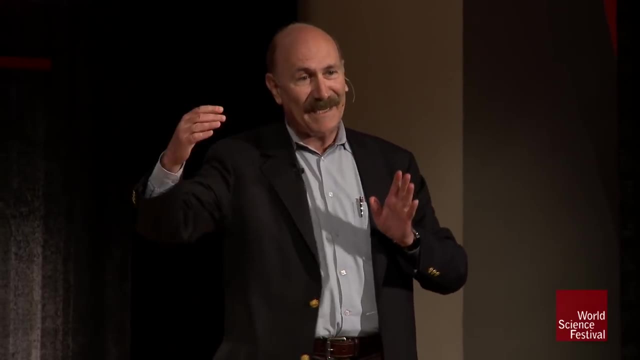 other hand, to think of this kind of problem, you have to think what is the probability of no match? and if you know a little bit about probably, you see that I did one minus 364, 365 and so on. you really have to think of the probability. 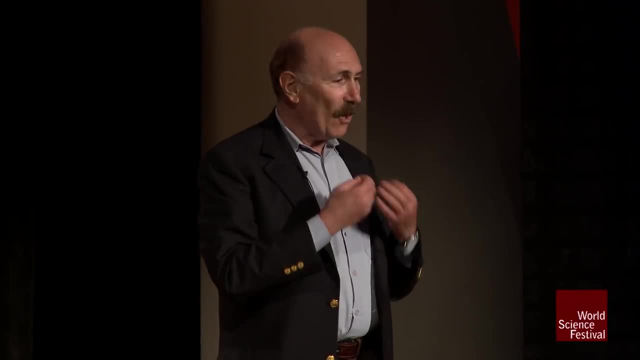 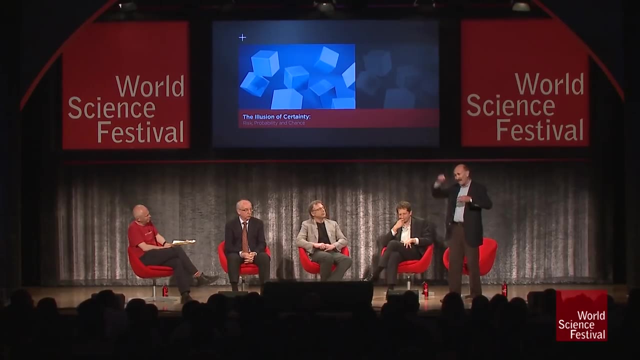 of no match and subtract it from one. well, when does no match happen where every ball is separate? there's no aggregation at all. but if you kind of visualize, if you see as balls fall down, they're likely to be two of them in one box. it just is the. 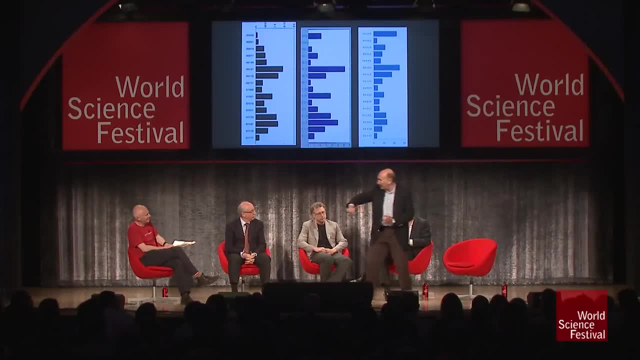 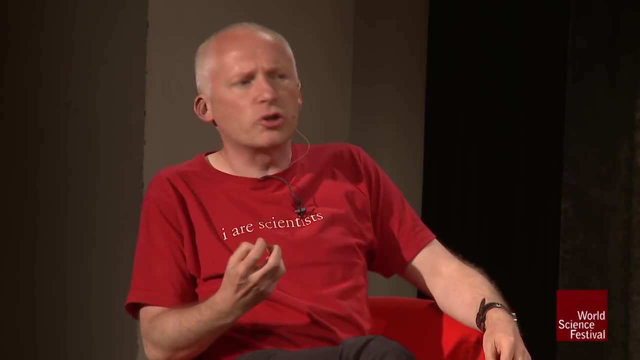 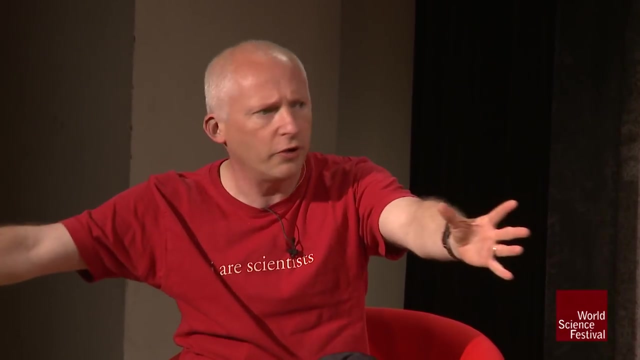 way it is, otherwise everybody, every ball, has to fall into a unique box and that just doesn't, doesn't tend to happen. so I suppose in some sense it's about. I suppose our intuition is: what's the probability that somebody has my birthday? and of course that's different, the different number of you know, with the 30 people, the, the. 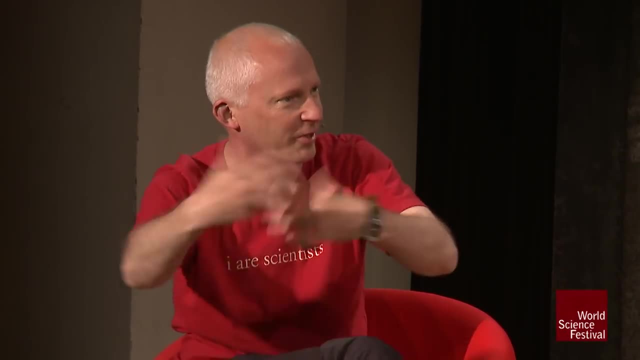 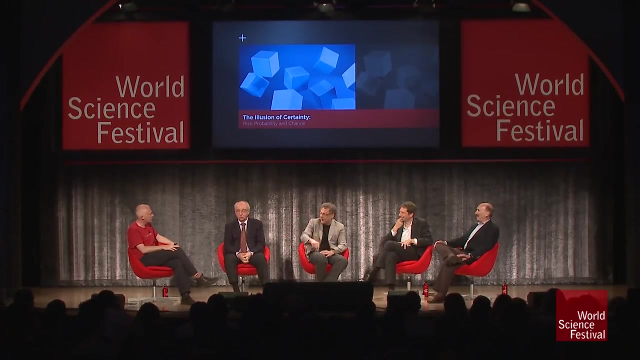 way, the number of ways you could have paired them up is is much larger than just 30.. right pairs of birth. exactly so, that's right. you're drawing from different pairs of birth, right, yeah? yeah, question is: when are two paired, the same versus different? that's a different question. 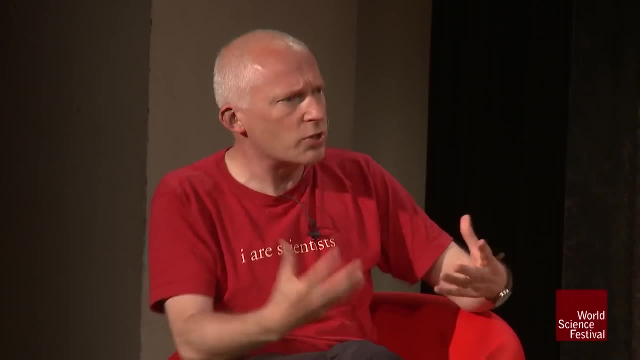 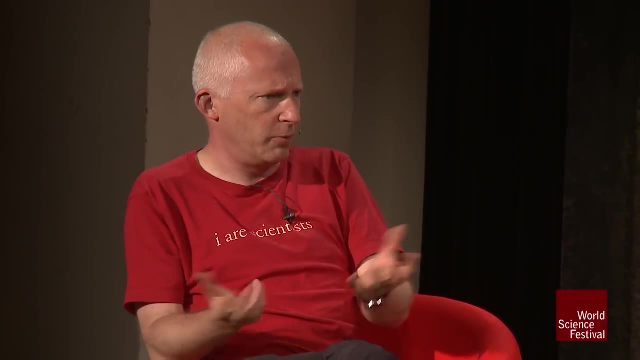 then do they have your birthday right, exactly. but I think it's interesting because it does both. the example we had at the beginning of the uh Monty Hall problem, which is counterintuitive, and I think this example is very counterintuitive. it's very counterintuitive. on the other hand, 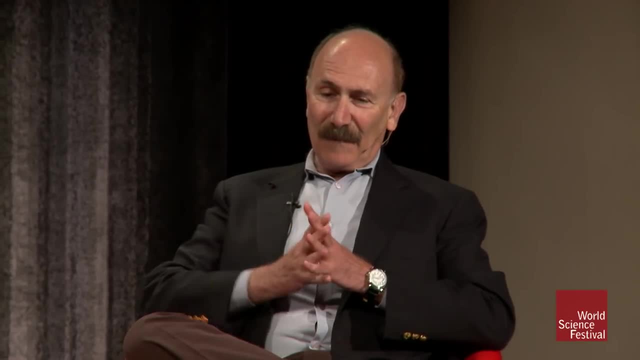 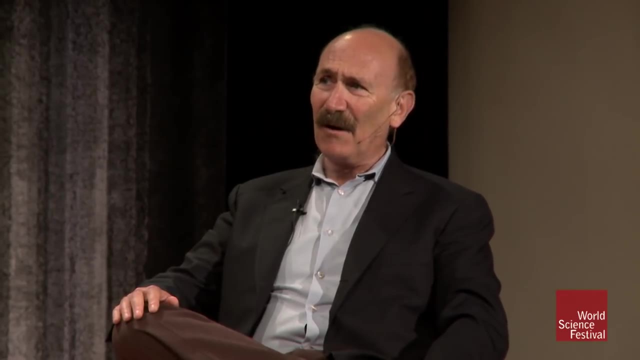 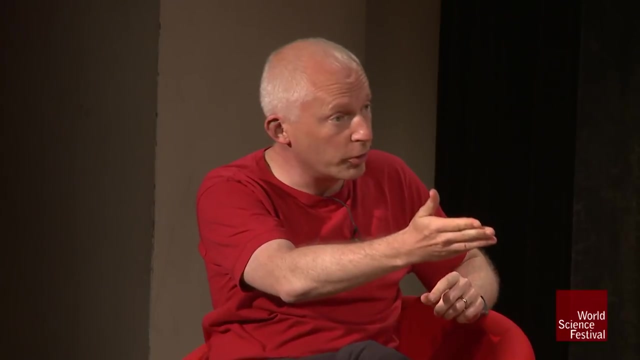 it's a basis for a lot of probability Theory. uh, um, there's a a mathematician named uh, Percy diaconis at. he used to be at Harvard. I think he's at Stanford now. he's at Stanford. yes and uh, he expanded this problem to explain a lot of probability Theory. uh, well, he also blew the. 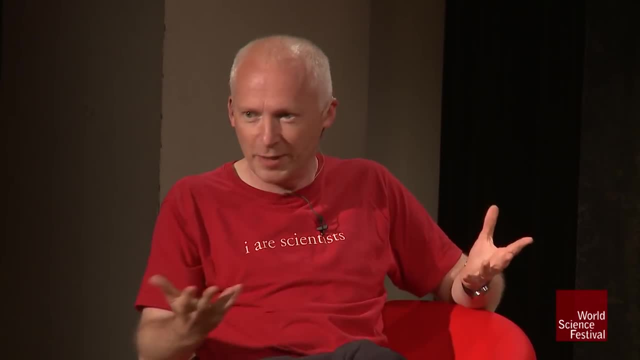 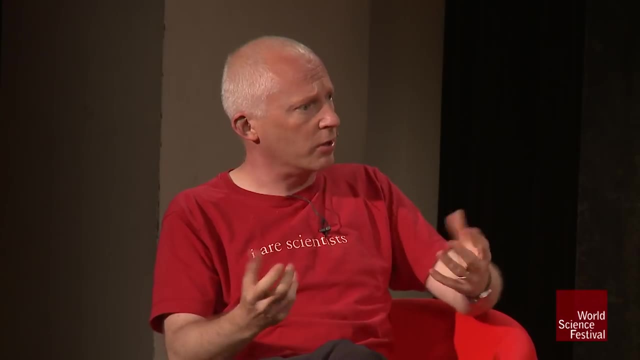 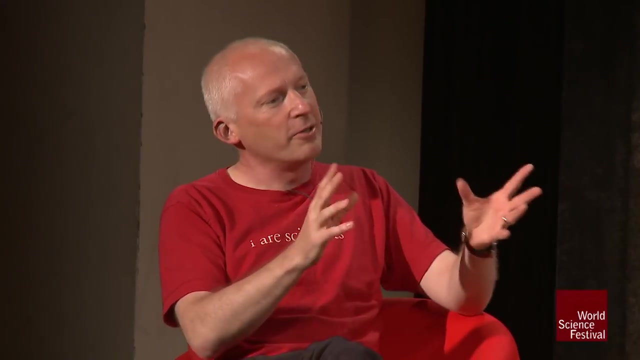 Bible code out of the water, because he showed that Moby Dick could also have as many um predictive messages in it um as the Bible. so, uh, so it's important to turn things into numbers, because without time, what's up? um, but yeah, my nice take on that. you know 23. I play a lot of uh soccer, as you call it um here. 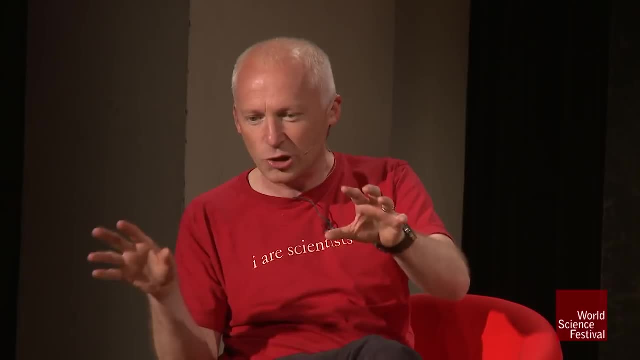 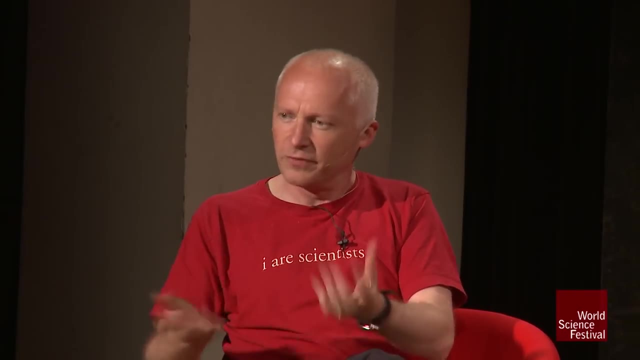 in England, um, and you have 11 players in each team plus the referee, which is 23 players. so sometimes I do this game where I ask for everyone's birthday and the likelihood is over 50 of the games that are played will have two people on the pitch with the same birthday. so which is? 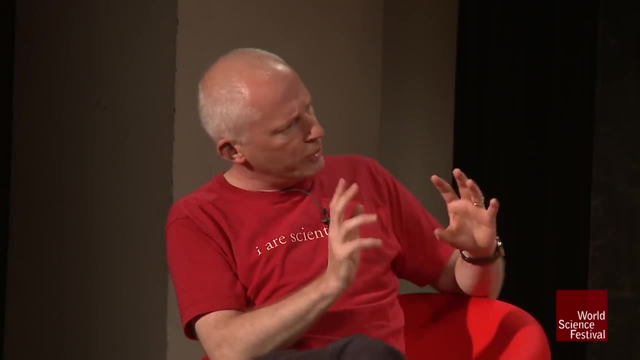 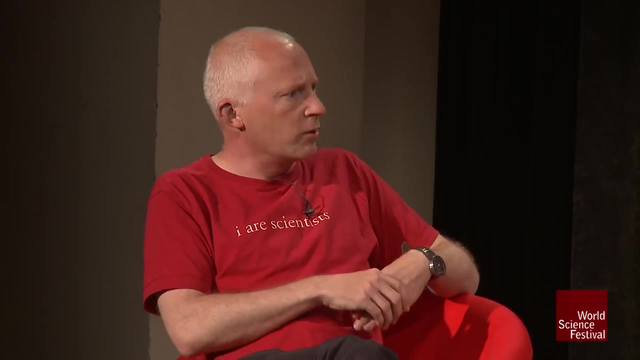 quite a nice one, but I want to come to you good, because you believe that, um, actually you know probabilities, the way we interpret, which are very important, say, in medical cases, that you know there's a such a percentage chance that I might have a disease or whatever. 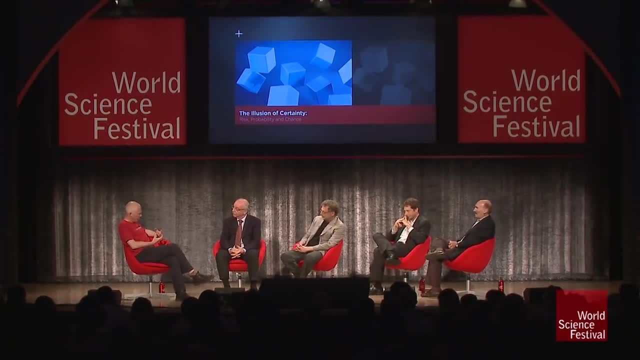 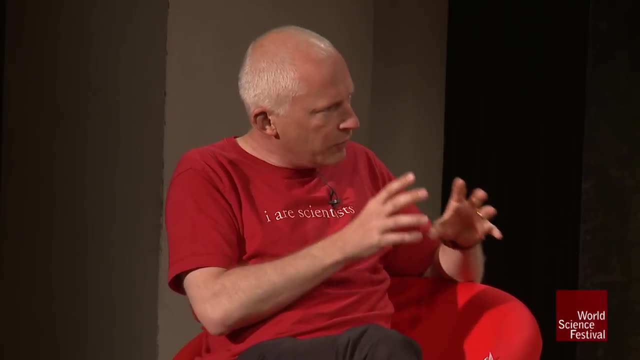 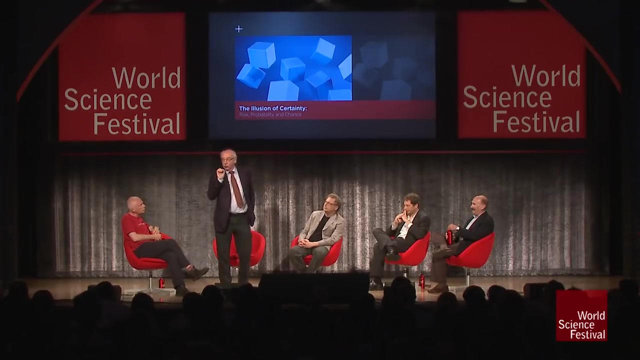 that actually, it's sometimes the way we phrase these probabilities which is key. so perhaps you could take us through a sort of a, an example where the way that you talk about probabilities can really influence how good you are at interpreting them. okay, so I would like to teach. 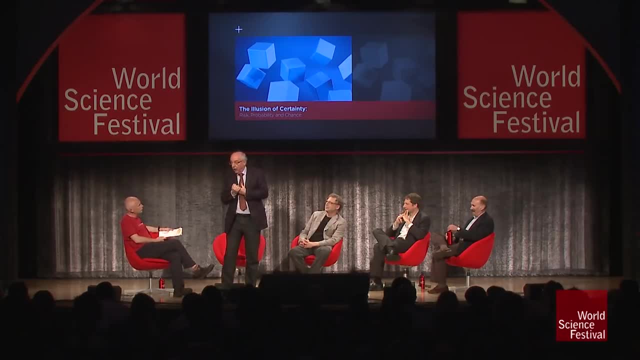 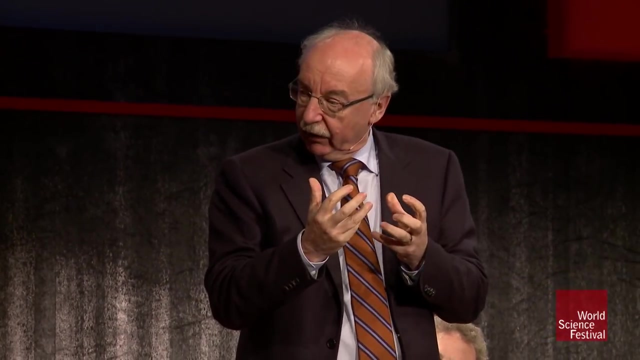 you something, um, and it's about health care, and in order to, to, to get the the background, so, at the Max Planck Institute in Berlin, that's in Germany, uh, we, we develop methods that help people so that they can understand the probabilities, yeah, which they usually don't. yeah, and I'll walk. 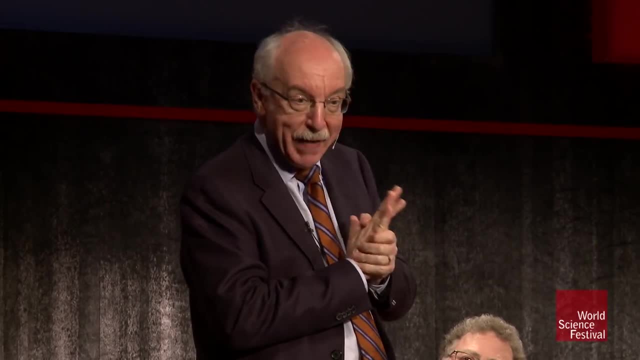 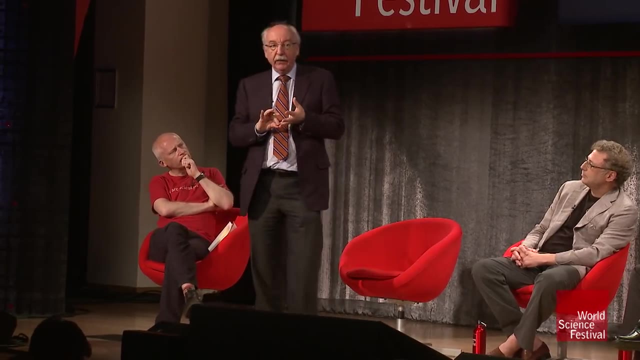 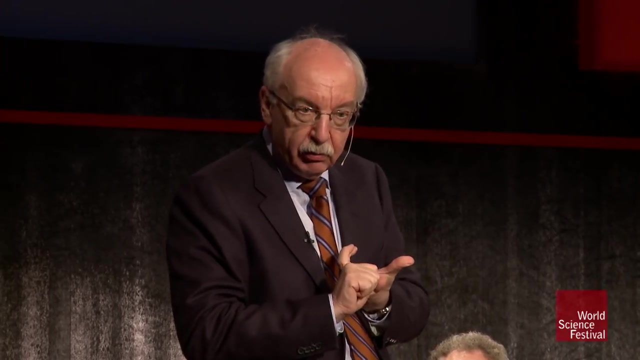 you through a little slice of a continuing medical education session. so I've trained in the last year hundred and thousand doctors and, uh, we'll take a bunch of. assume you are gynecologists and you have had in medical school no training in statistical thinking. that's typical. 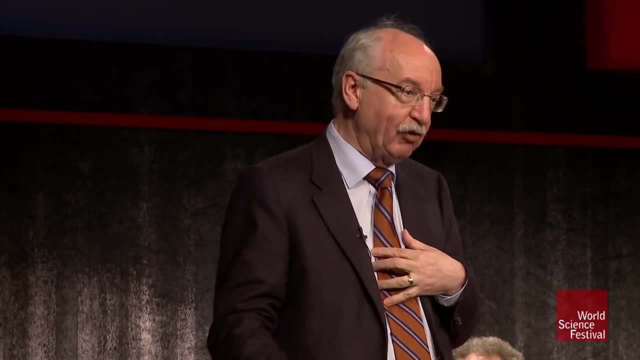 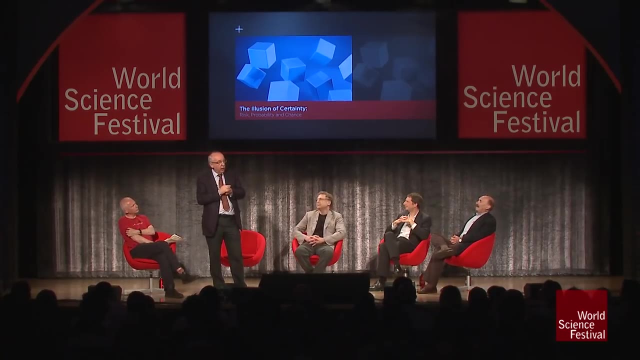 but also you think it's just you. you have no mass gene and all the others no things. so that's the basic setting. so when I start this I'll uh started with a problem, and that's an everyday problem for a gynecologist. so assume you conduct uh breast cancer screening. 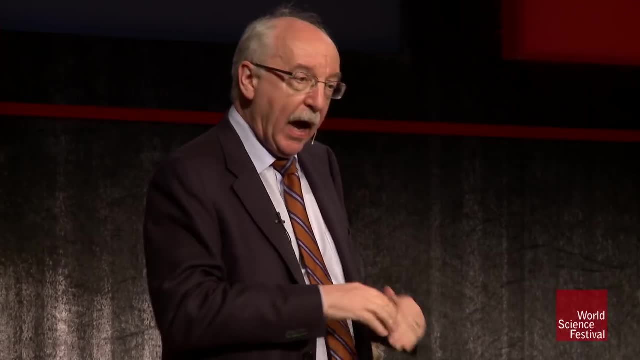 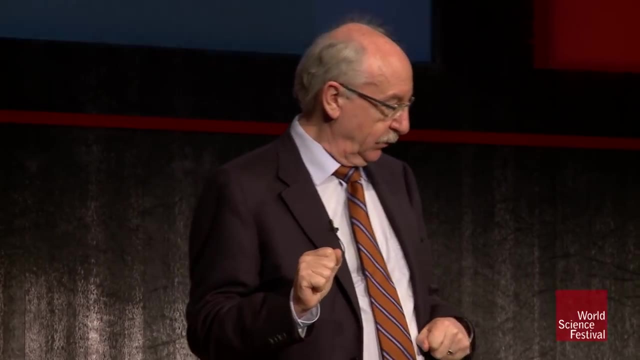 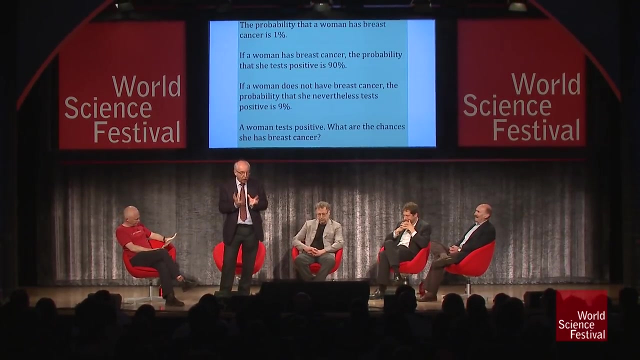 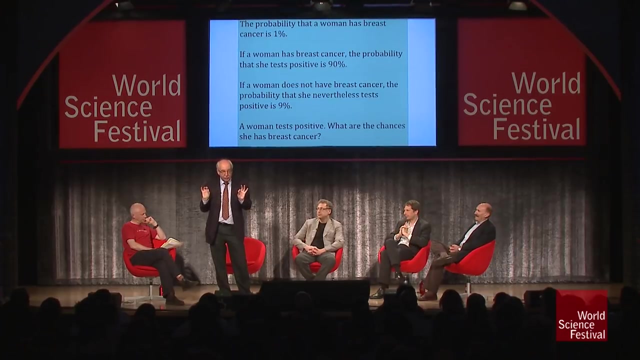 with uh, with mammography, and what you know about a certain region is the following: can I have the first slide? so I give you now the information in the same way as medical doctors get them in their books. the information is technically called conditional probabilities. we'll go through this. conditional probabilities confuse your mind. 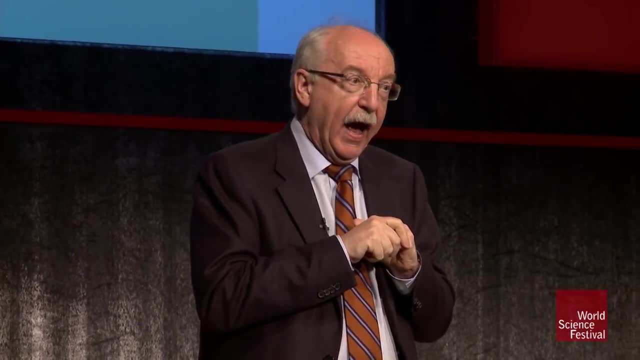 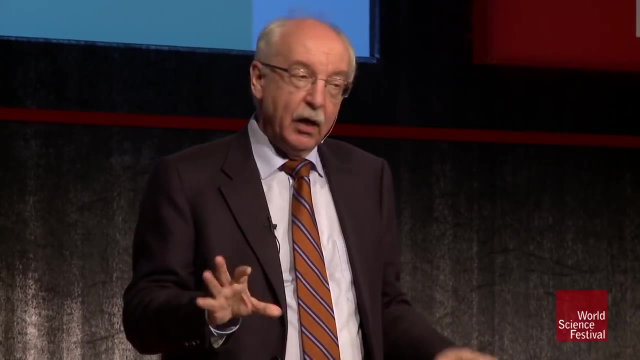 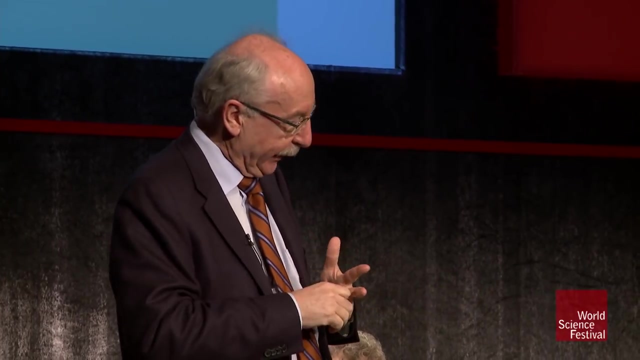 not everyone's, but I hope so. and so what you know is the probability that a woman has breast care, that a woman has breast cancer, is one percent. all these numbers are highly realistic, but we just make them simple. okay, that's a simple probability. the second information is: if a woman has breast. 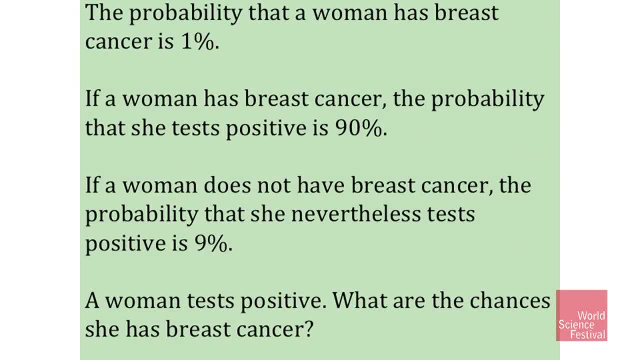 cancer, the probability she tests positive is 90%. This is a conditional probability. If a woman has breast cancer, the probability that she tests positive is 90%, also called the sensitivity And the final information. if a woman does not have breast cancer, the probability that she nevertheless. 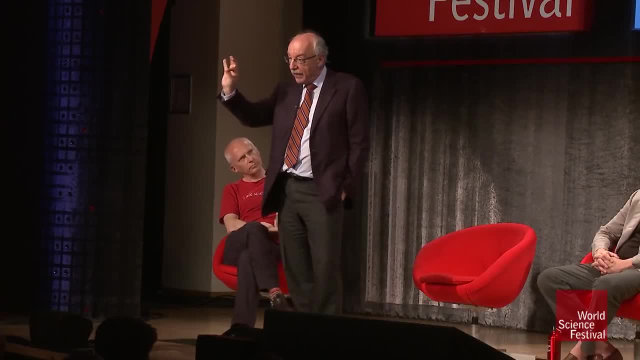 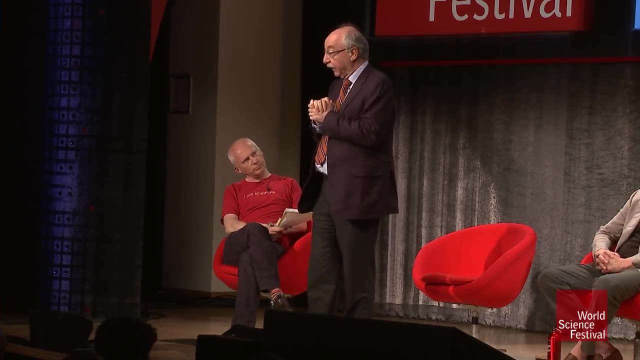 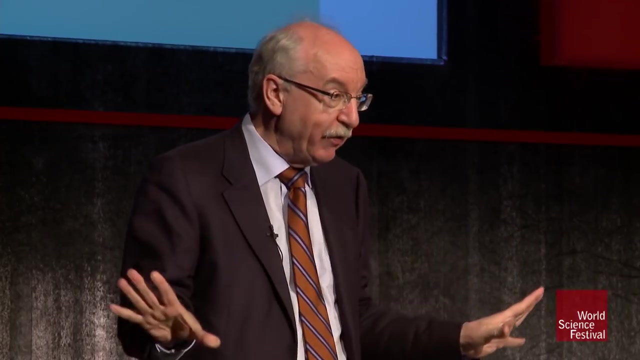 tests positive is 9%. So we have a base rate or a prevalence of 1%, a sensitivity or hit rate of 90% and a false positive rate of 9%. Now here is a woman who just tested positive in screening. You know nothing else about her And she asks you, doctor, tell me do. 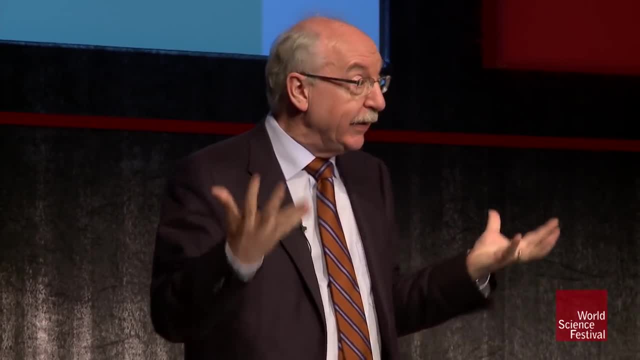 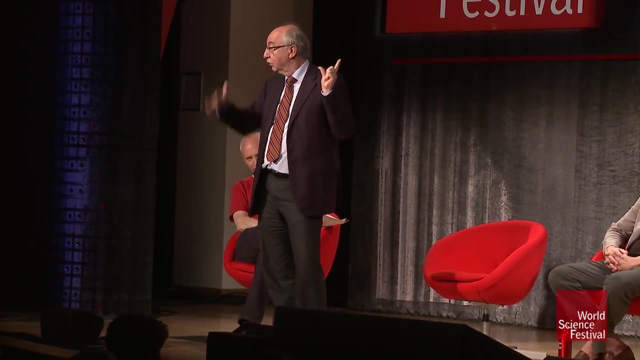 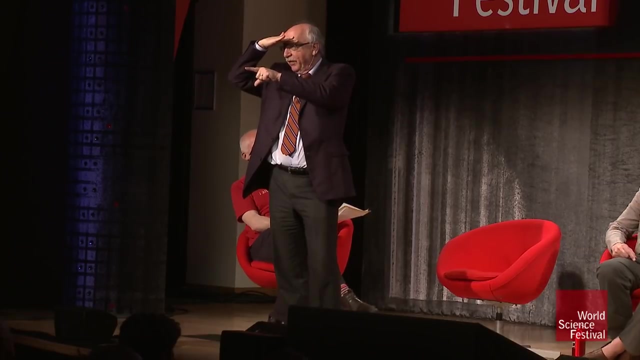 I now have breast cancer, Or what's my chances? 99%, 90%, 50% less. Tell me So. 11%, 9.3%, 9.3%, 9.3%, 9.3%. 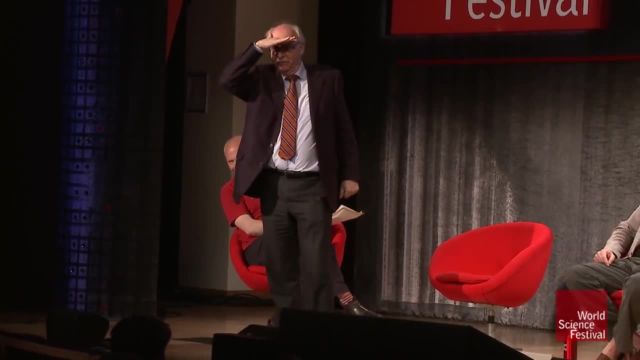 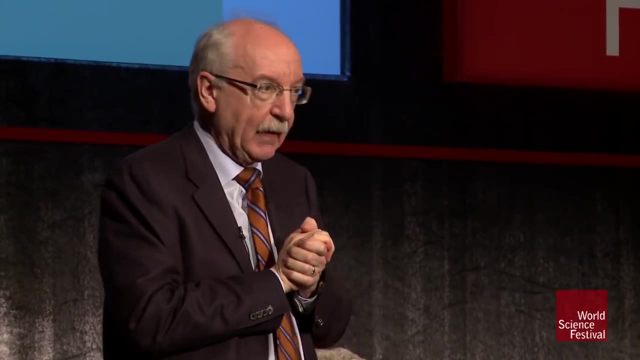 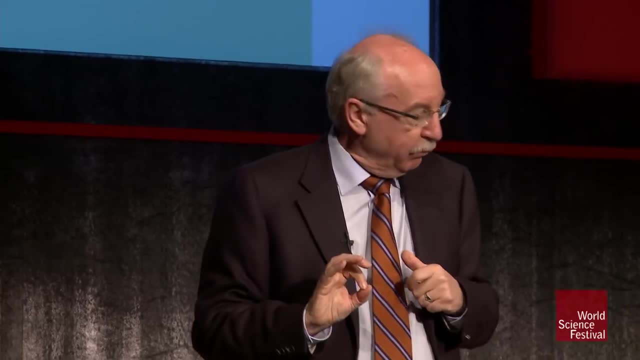 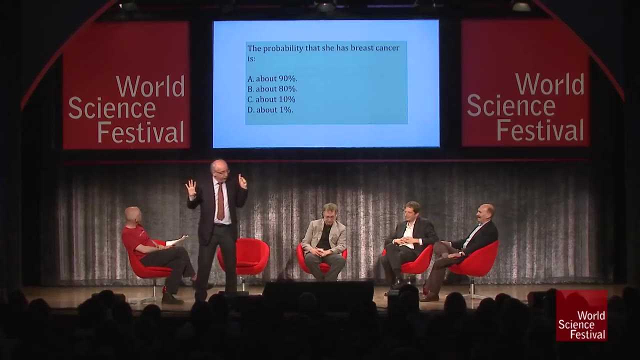 Okay, we slowly get this spread The point here. let's make a vote. Can I have the second slide? So keep this in mind. I give you four alternatives. One is the probability that this woman has breast cancer in screening is. here are the four alternatives. 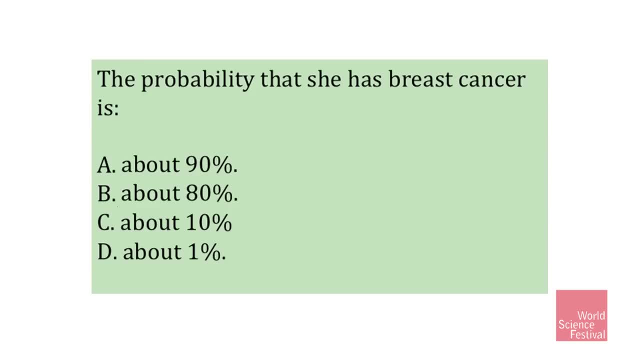 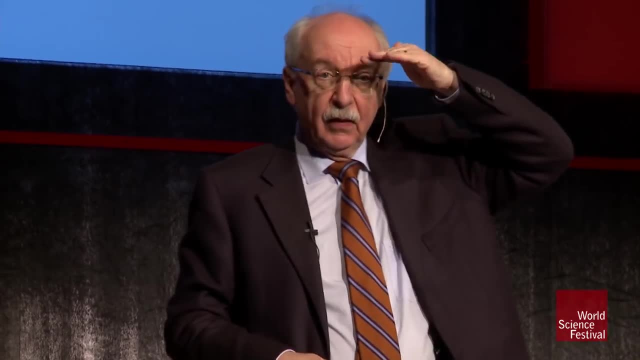 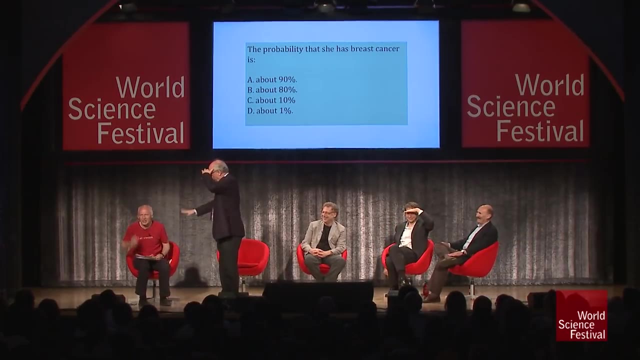 90%, about about 80%, about 10%, about 1%. So who of you start with A? Can you count? No, we've already proved that I'm rubbish at counting. But yeah, I kind of estimate. yeah, I do my best. 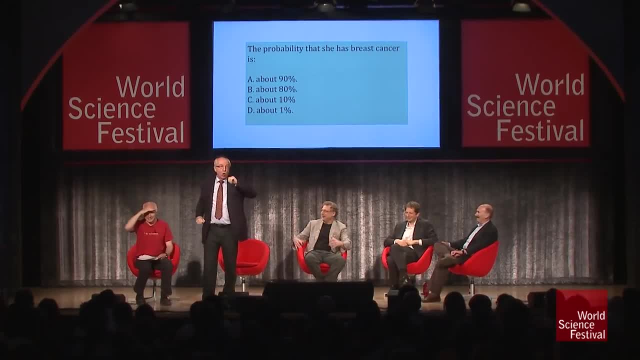 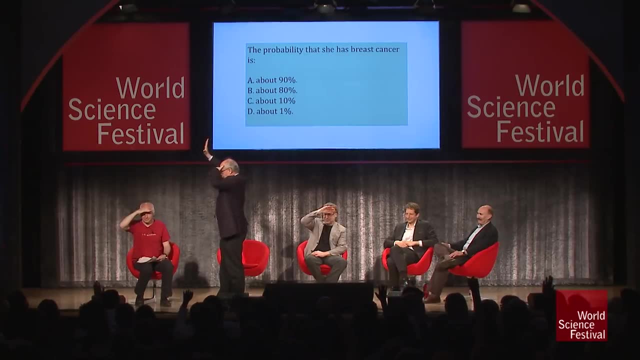 So you decide for one of these alternatives. yeah, Who thinks that A is the best answer? Hands up What is your count. Yeah, yeah, sort of. yeah, it's quite a lot, It's a lot Good. 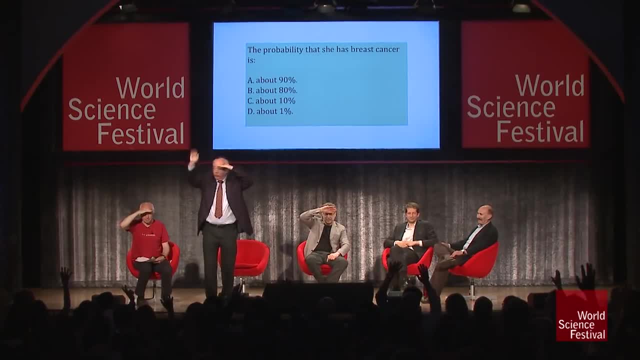 Who thinks that B is the best answer? Oh well, yeah, that's, That's also quite a lot. Yeah, quite a lot. And yeah about equal Yep. Do we have another category besides quite a lot. Yeah, I will do. 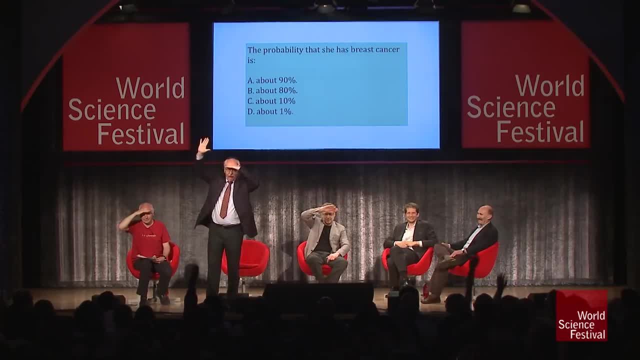 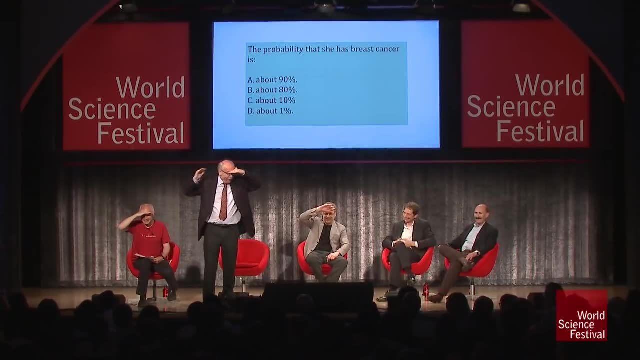 Don't worry, Okay. Who thinks that C is the best answer? Well, yeah, quite a lot, That's quite a lot. Who thinks that D is the best answer? Oh, fewer, That's fewer, That's fewer, Okay. 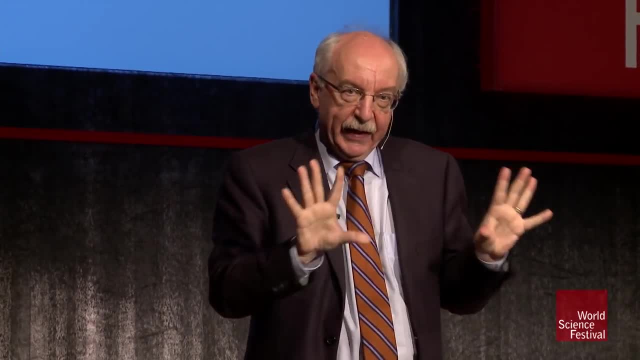 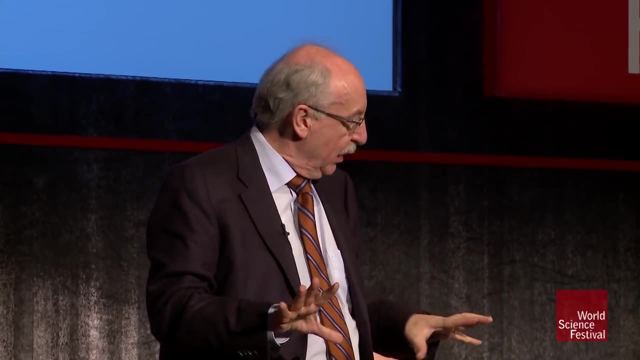 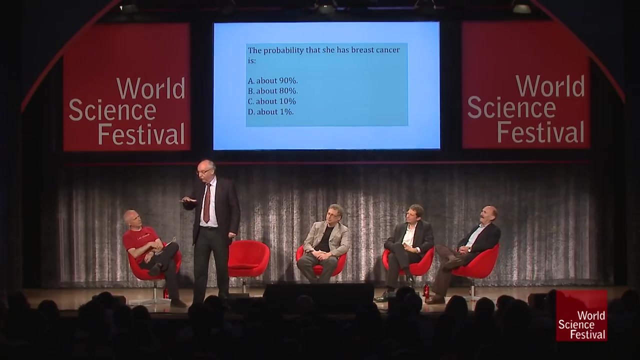 Three times quite a lot. Yeah, yeah, exactly. So before we get to the solution, I tell you what the average gynecologist thinks. the answer is: And it's exactly the same here. So in my studies. so about 20% of gynecologists think it's D, 1 in 100.. 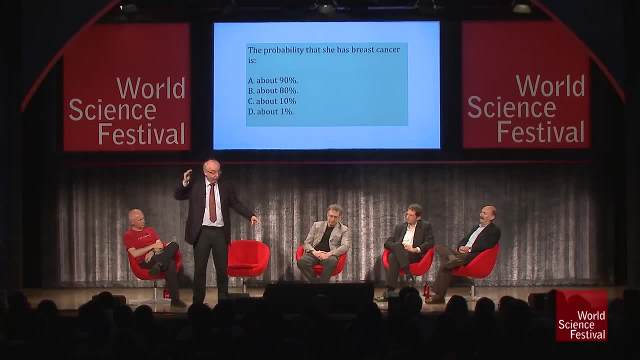 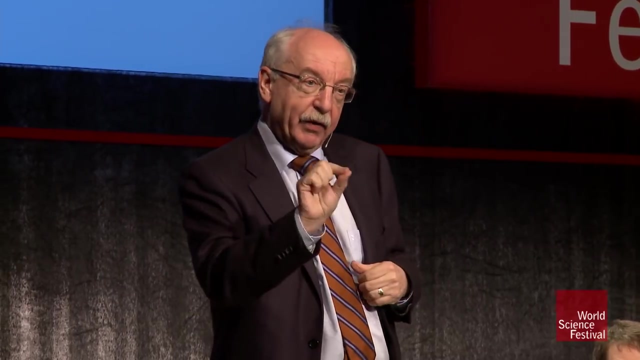 Another 20% think it's C, 10 in 100.. The majority, so 60%, thinks it's A or B. If you just look at this, you understand that medical training fails. And if you ever go to your gynecologist, ask for numbers. 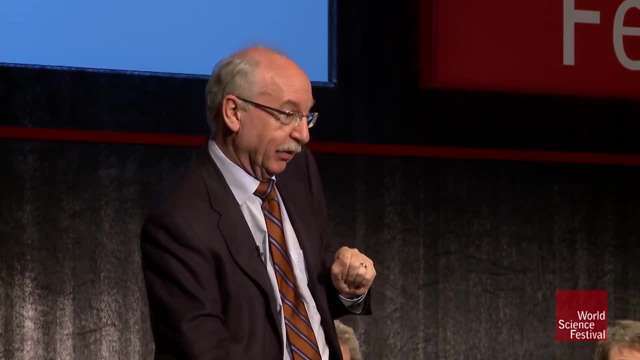 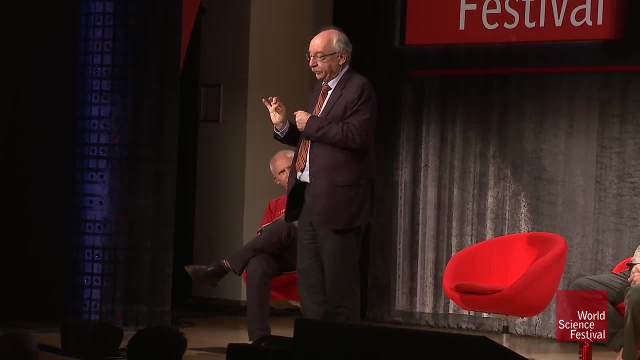 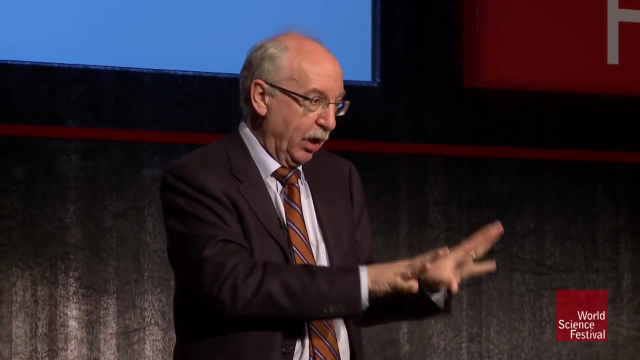 Don't behave as a little child in front of a white coat. It's your health. What I do now with you is the following: The point is that conditional probabilities cloud the minds of many people, including doctors. They have the same minds. 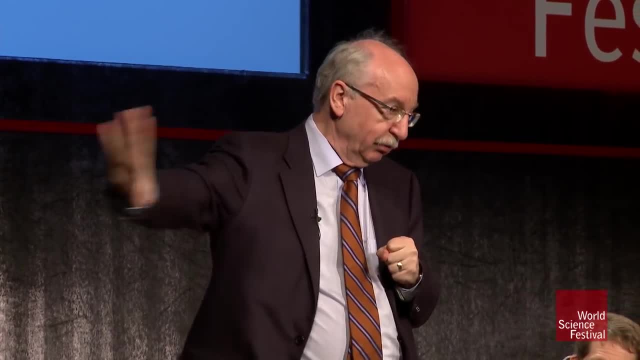 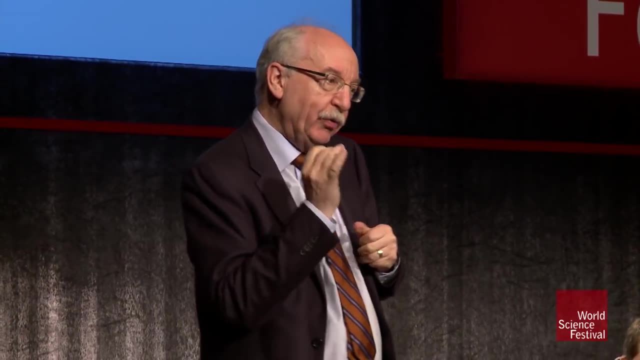 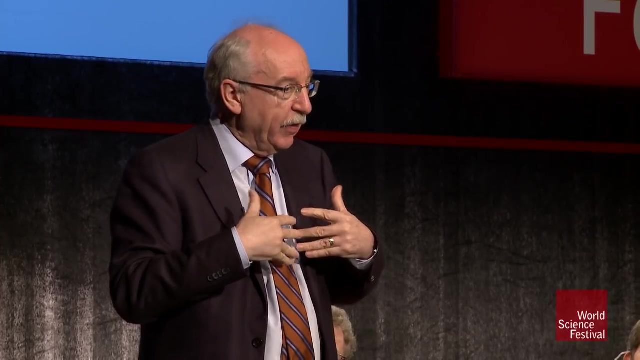 The solution is now not to send doctors into a statistical course, because they might just learn something and forget it immediately, but to do something that has to do with the psychology of their mind. And the interesting thing is, what I teach them is to change the representation of the 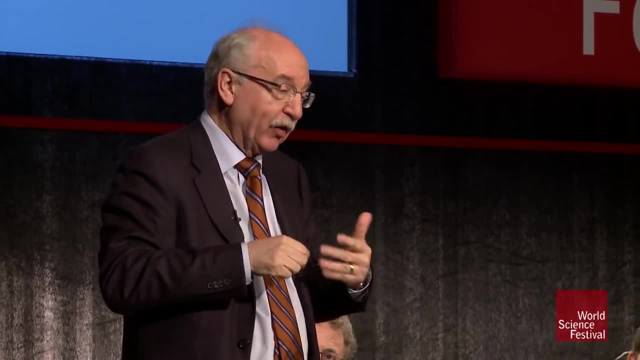 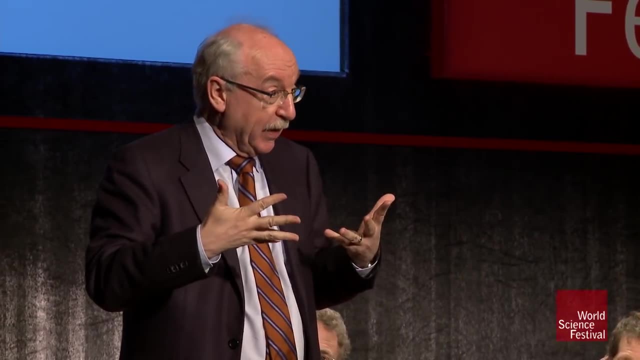 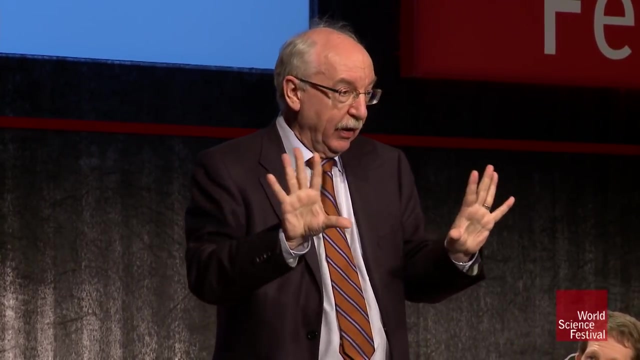 information into something that our minds can easily digest. We call this natural frequencies. That's the way that people learned about information before the time of statistics and probability. Okay, are you ready? I give it in a simplified way. You always start with a concrete number. 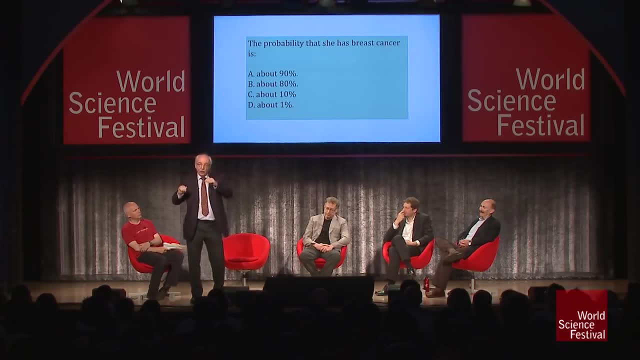 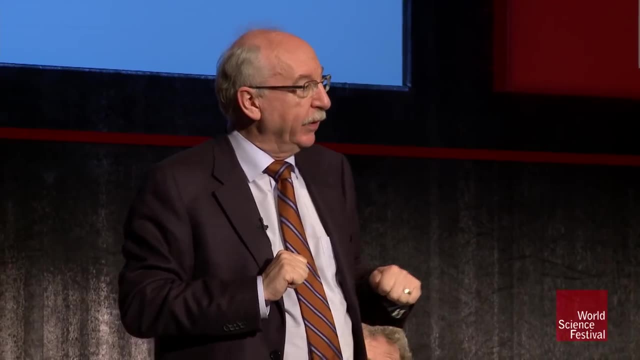 Say 100 of them. So I'll just translate the numbers and then we go in the exact numbers. Okay, So think about 100 women. We expect that. how many have cancer One? This person most likely tests positive. 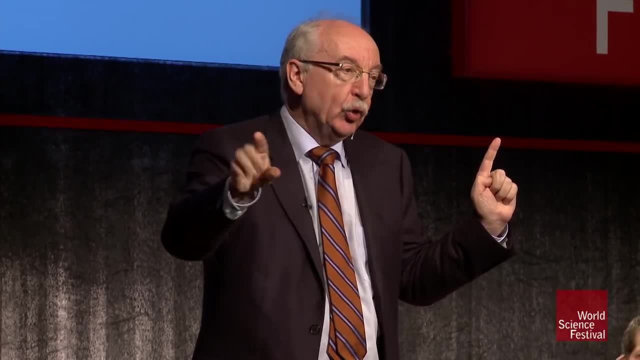 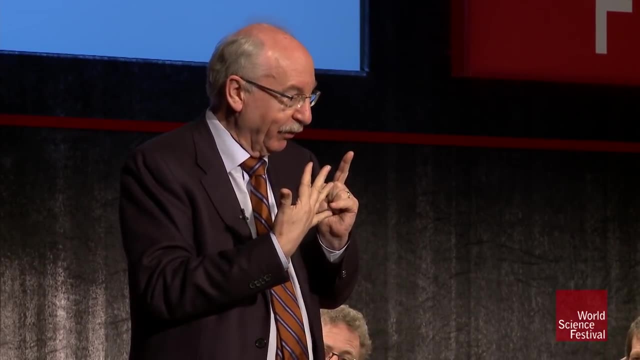 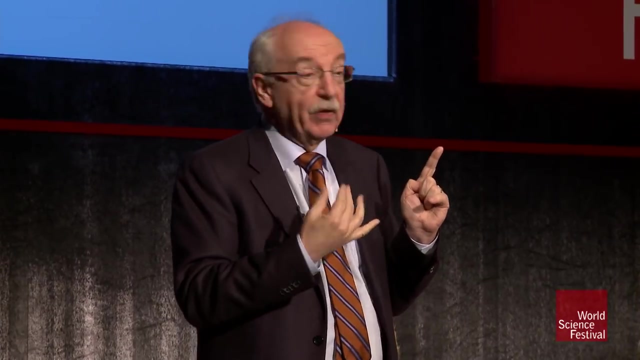 That was 90%, And of the 99 who do not have cancer, we expect another nine to have cancer. Makes 10 who have cancer. Question, Sorry, Makes 10 who test positive. Yeah, You got it. So we have 10 who test positive. 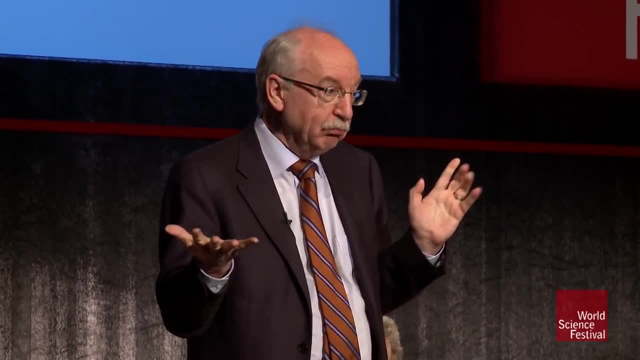 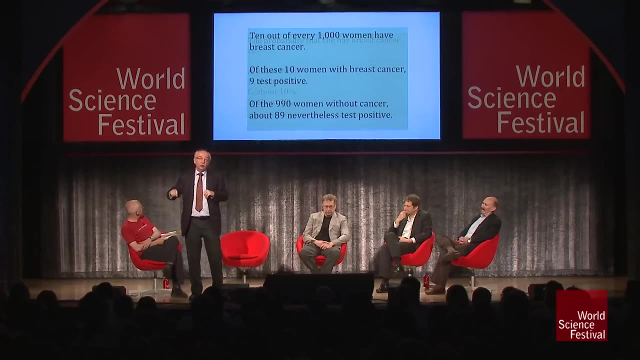 How many of these 10 do actually have cancer? One Let's see. C is the right thing, And can we get the next slide. So if you want to do the more precise numbers, you start with 1,000, but you end up with 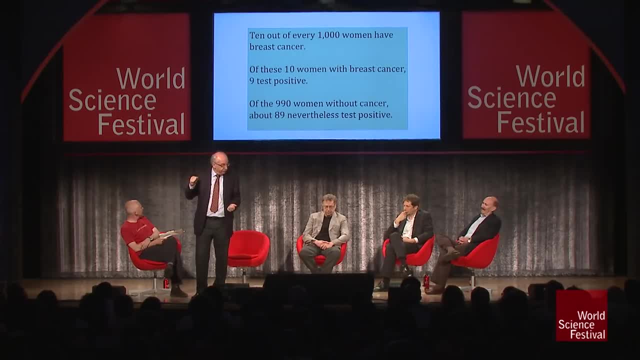 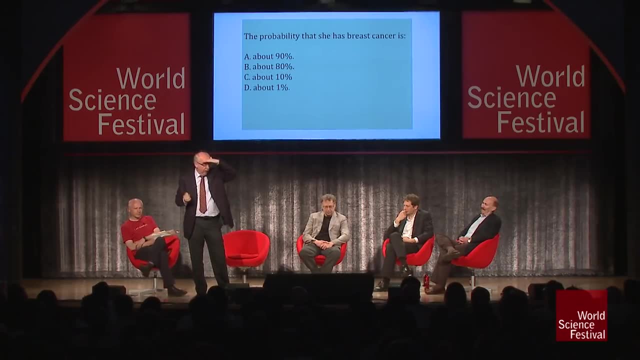 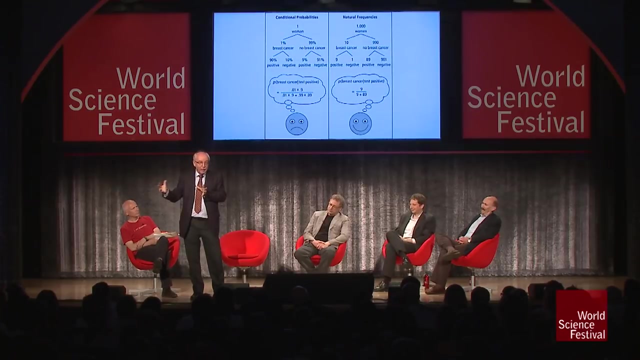 the same problem. Can we get the next slide And the next Now? we can now make a vote, but you know it. So when I do this exercise with doctors, so at the end of the 90-minute continuing medical education session, I don't give them the right answer. 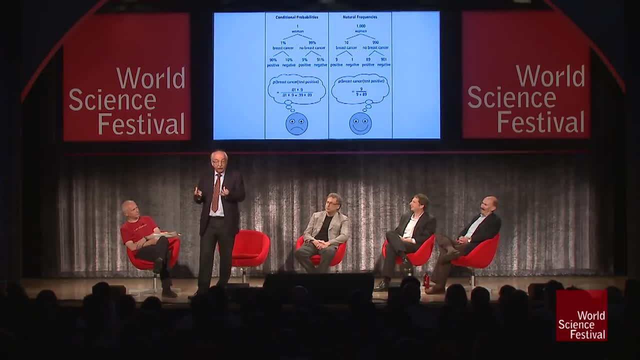 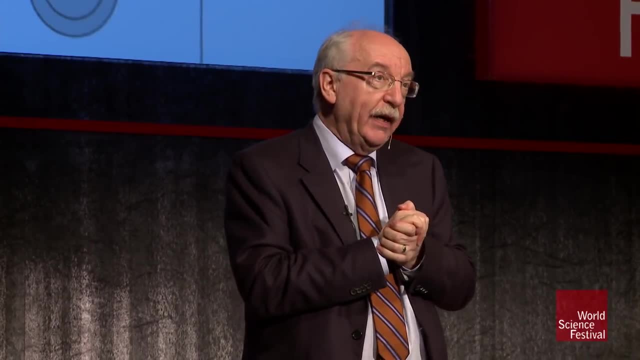 Now they get the same problem again in probabilities. and now they know we have to translate them- Think about 100, and that works. And then usually I get something between 85 and 90% of them now see through. 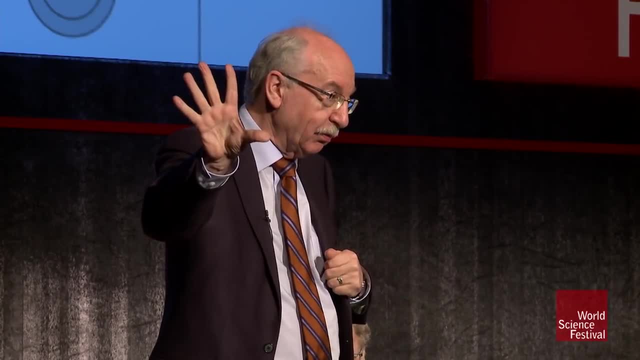 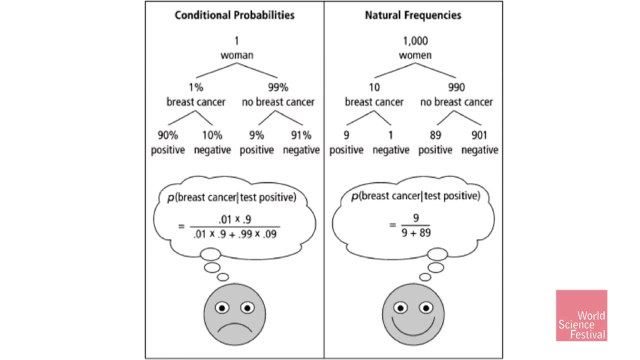 They understand now. There are always a few hopeless cases, but most get it. Why does it work? So here you see, on your left side, the situation with conditional probabilities, And you see a formula that's known as Bayes' rule. 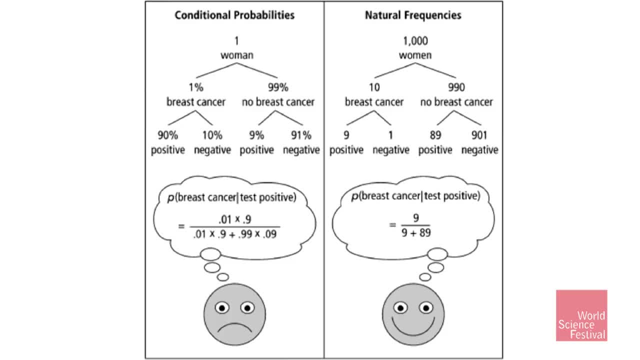 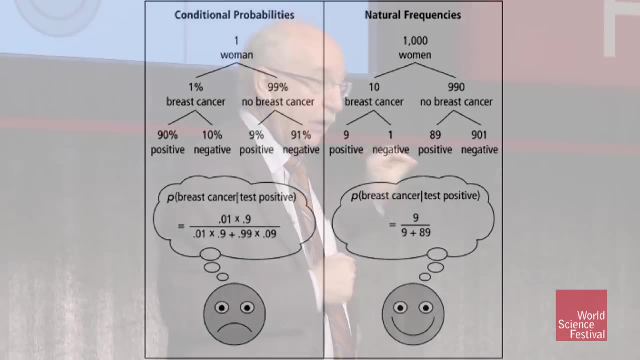 If you don't know Bayes' rule, it doesn't matter. Look at this and you know why you were confused. And the interesting and theoretically interesting point is that we can show why one now sees through with natural frequencies: Because the representation, the external representation, facilitates one's computations. 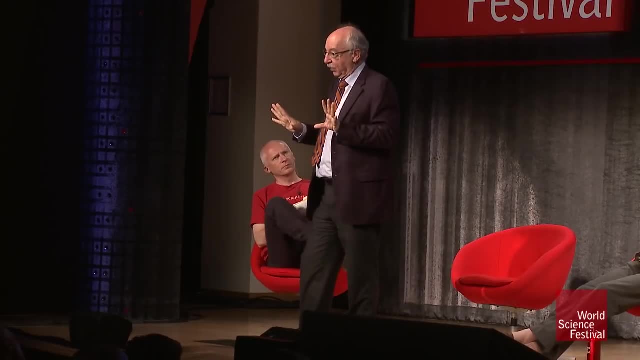 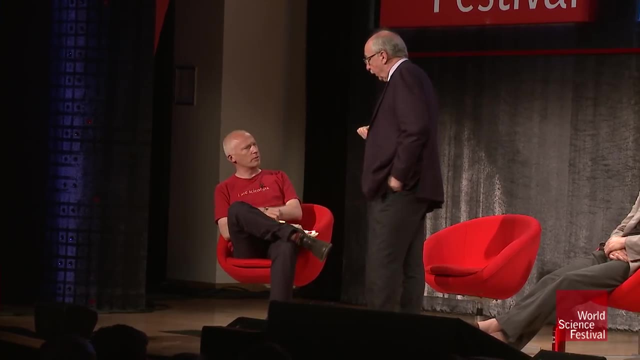 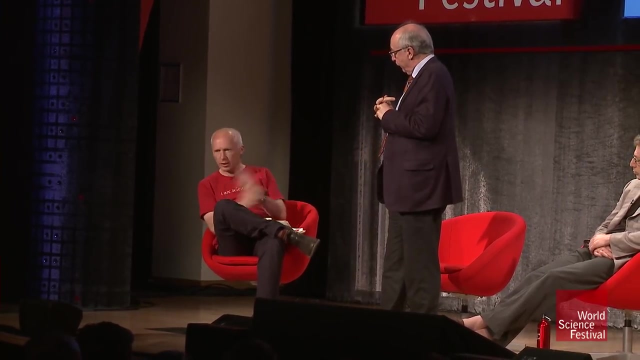 And the entire formula is very simple. So you think that it's the way we actually talk about the numbers that is important in establishing a different intuition. I mean, when you described it in terms of what you call natural frequencies, I think most people just saw it immediately. 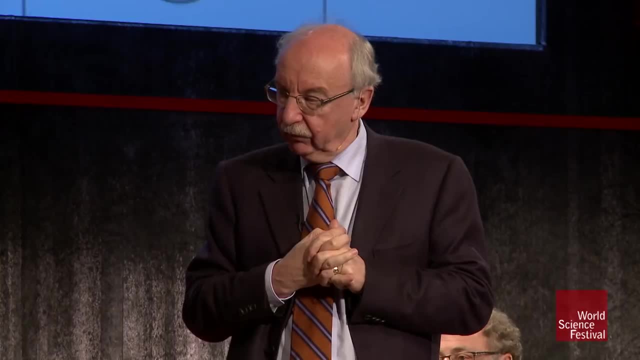 But in those percentages I'm also. I'm a mathematician, I should be all right with these, But it just messes with your mind. You're human. You're a human mind. I'm human, at least Yeah. 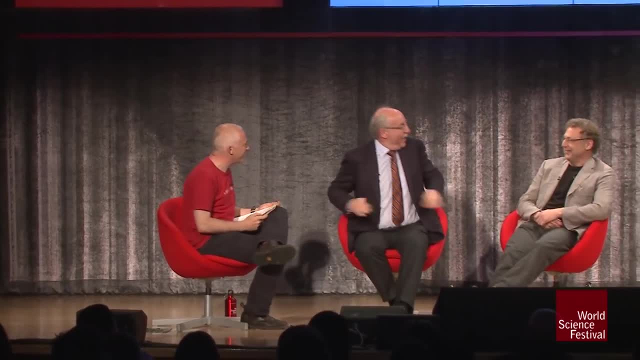 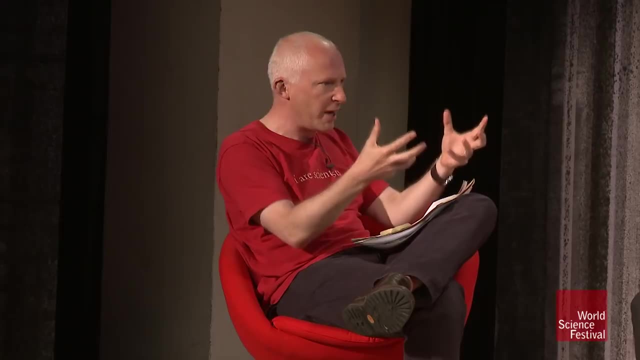 That's why it doesn't work. Yeah, Josh, would you say 99% sure of that? Conditional, All right, Josh. I mean, would you say that that natural frequencies is just. The brain is much better at dealing with these kind of interpretations. 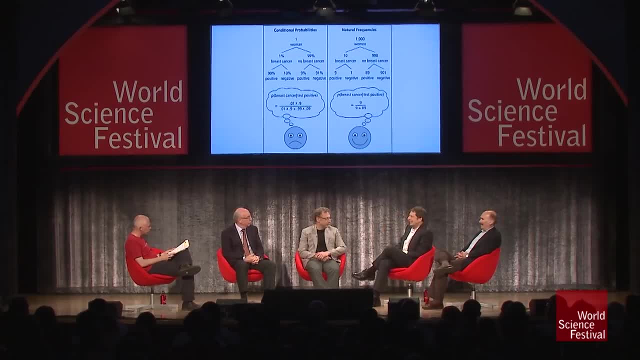 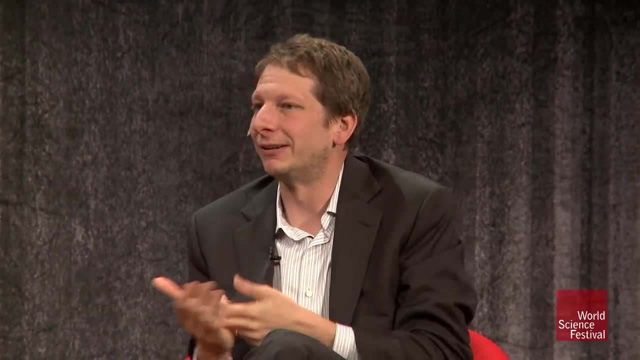 Yeah, I mean, that's very much what this research shows. I mean, people are tracking events, the things that actually happen to us, as opposed to manipulating decimals. That's one of the things our brain does. We have what's called episodic memory. 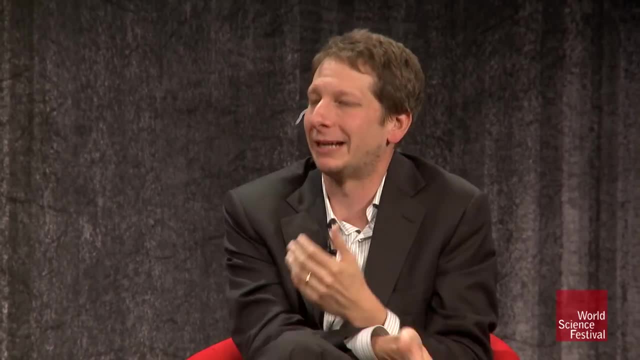 We keep track of. well, this is what happened today, That's what happened yesterday, And I think Gerd would say, and has said, that you're harnessing those mechanisms when you present data in the form of cases like this. But what about? 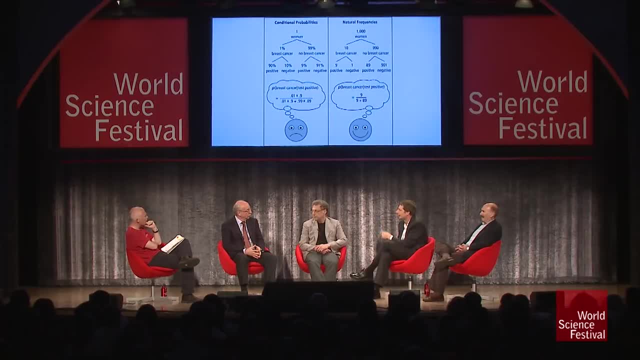 We had in the opening video the idea that your DNA matches and there's a one in a million chance, And I think for most people we don't have a conception of a million, So for us one in a million means almost nothing. 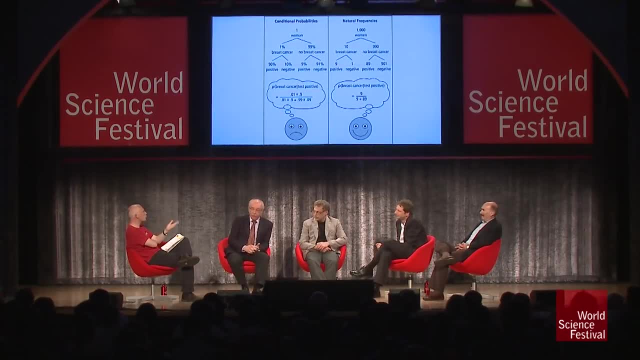 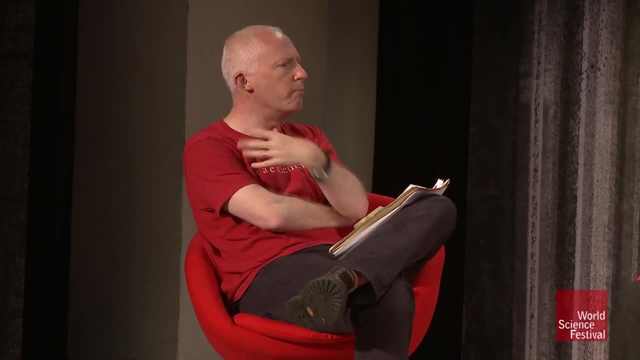 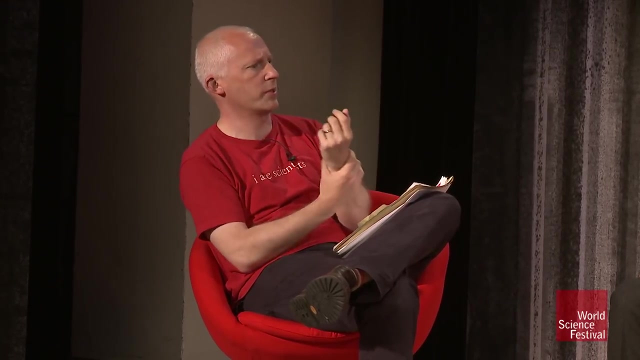 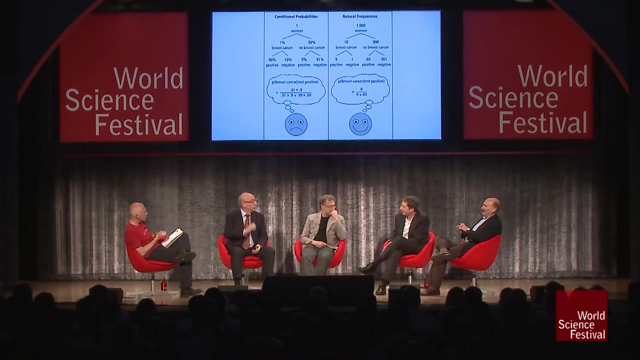 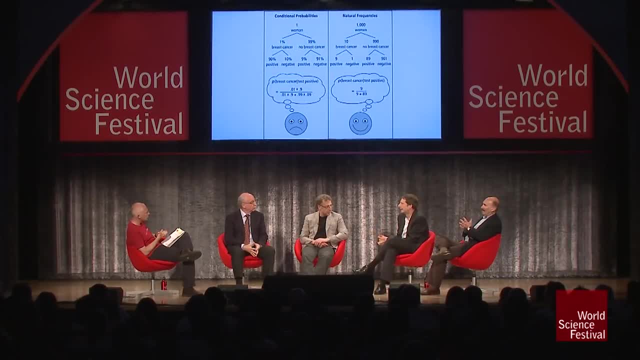 One of the interesting things about how number works in the brain is that this is an area where a lot of research has unfolded over the last, say, decade or two. we have certain basic mechanisms for tracking very small numbers like 1,, 2,, 3, 4 objects. 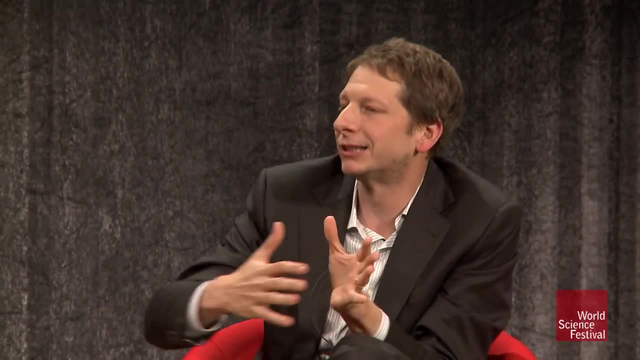 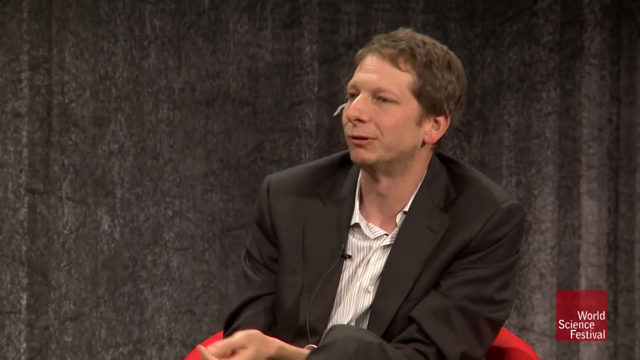 keeping those straight. We also have mechanisms for tracking that, approximatelyrichting a set of dots, like the ones I showed you, and being able to say well, whether it's 10 or 20 dots, being able to tell the difference between those. But those mechanisms don't scale up to a million. they maybe go up to 150 or something like. 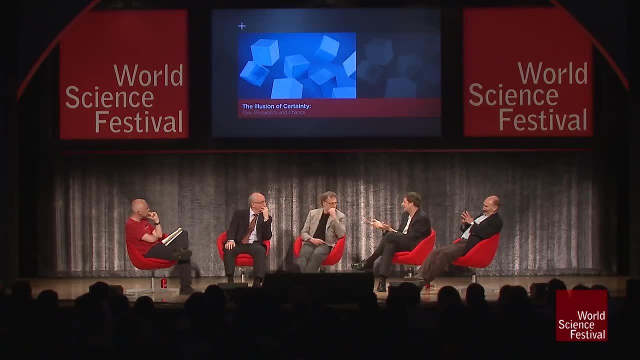 that. So once you go beyond one or two orders of magnitude, you know- and that's where you really need these units like dollars and cents, .002.. Right, but the example you gave, that's not the problem. It's not the problem that people don't know what one in a million means, but they're asking. 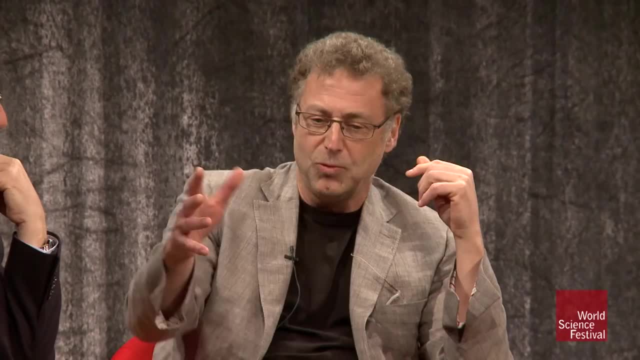 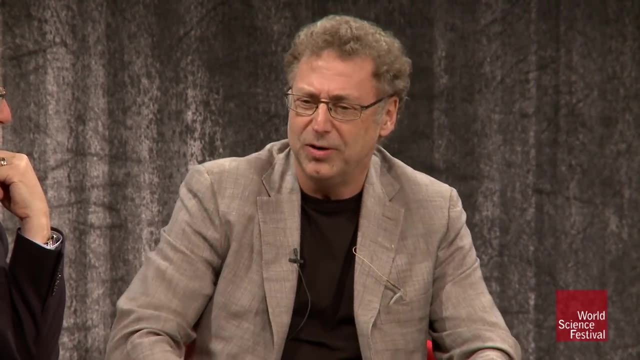 the wrong question, okay, Because when you have the say, there's a one in a million chance that someone will test what will have. I don't know what it was, the fingerprints or the looks or whatever it was. the question is: and what are the chances that a random person will match that? 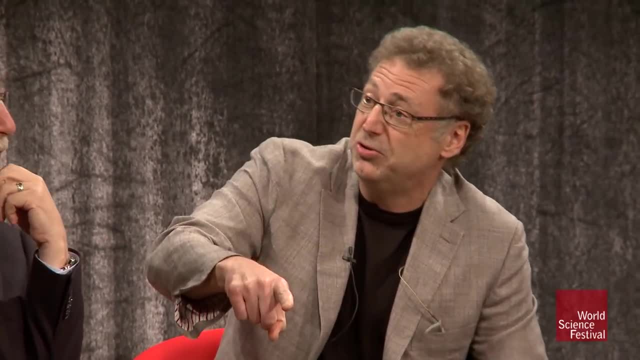 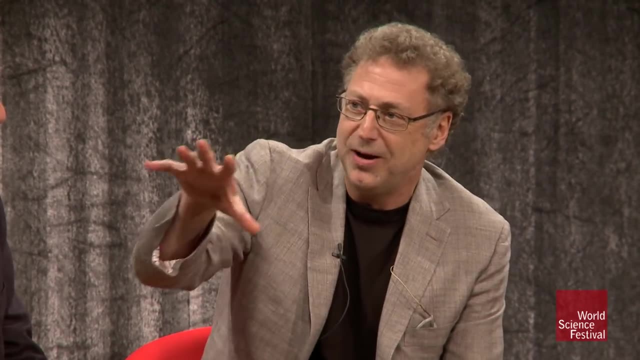 The question is: given that you match that, what are the chances that you didn't? And so, in the prosecutor's fallacy, the problem is that there's- maybe you said, three or eight people in town, or whatever it is that match that. 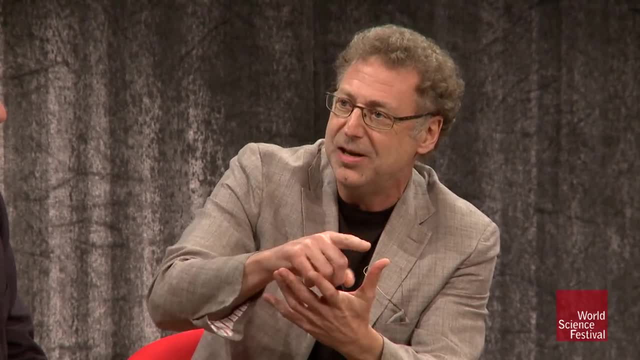 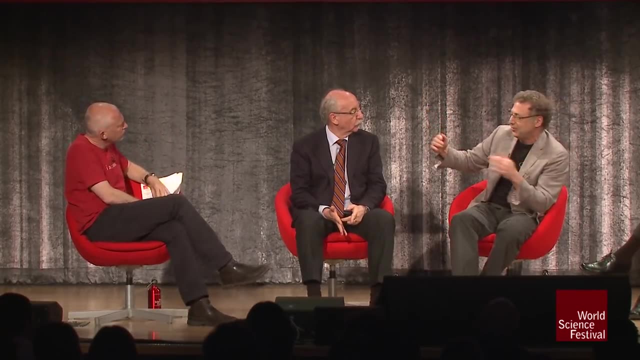 So, given that you match that, the chances that you did it are one in three or one in eight And one in a million is a red herring, Exactly Just like it is in this, in the breast cancer. you have a test or another test that'll tell. you that a false positive? The chances that you test positive if you're not, don't have the illness? one in a thousand, one in a million? it doesn't matter. What matters is: how does that compare to the actual number of incidents of the disease? 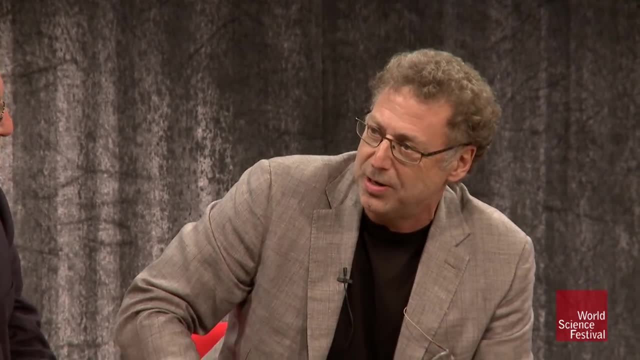 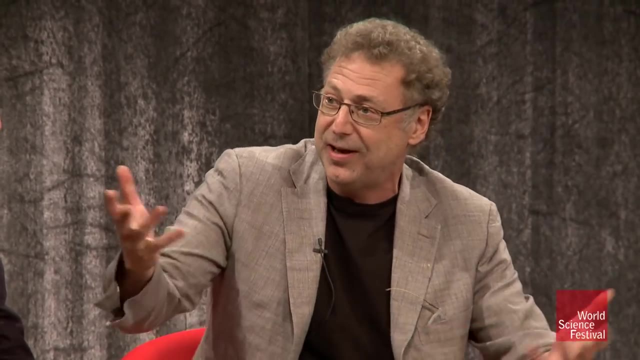 So if you test, the test could be great and one in a million people- only one in a million people- ever test positive. they don't have it, but one in a billion people actually have it. then the chance that there's still about 999 out of a thousand if you test positive. 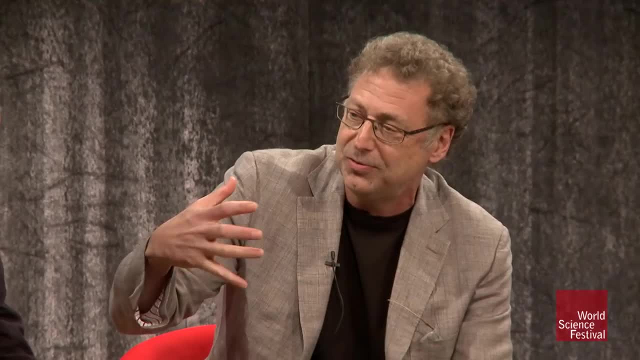 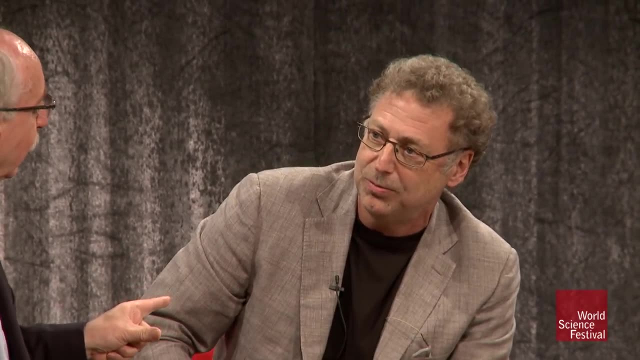 that you don't have it, Because the positive, the false positive, they don't have it. The positive tests are still a much higher frequency than the actual disease, And so it's important to keep that in mind. What happens when you talk with your doctor in this way? 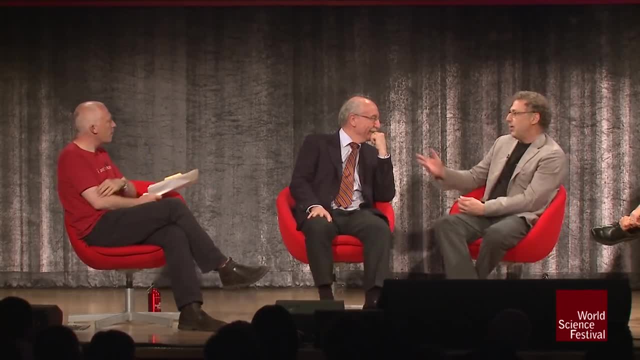 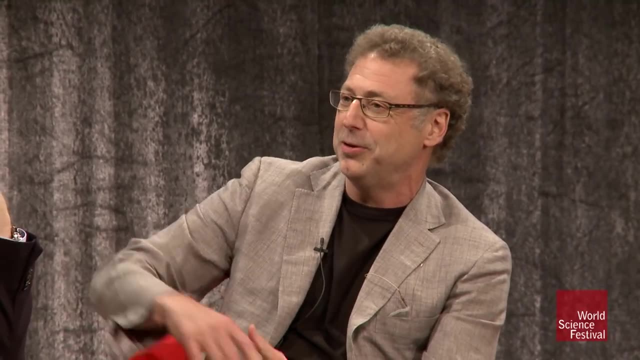 Oh no. Well, my brother, for instance, is a doctor, and he tells me that they don't, they don't care, They don't. I mean not that he doesn't care, but there's no way you're going to. 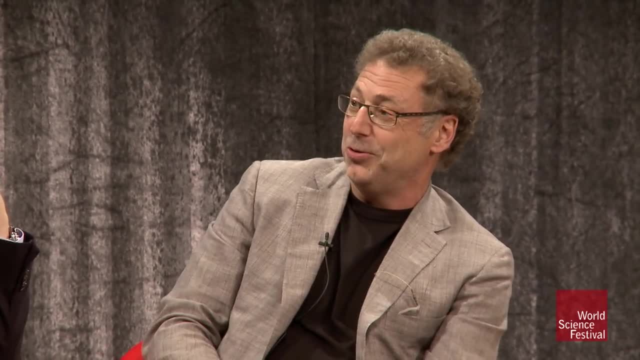 But I had a. you know I wrote about it in Drunkard, so I have my own, my own experience with this. I had a false positive AIDS test back in the 80s and my doctor didn't even give me, didn't. 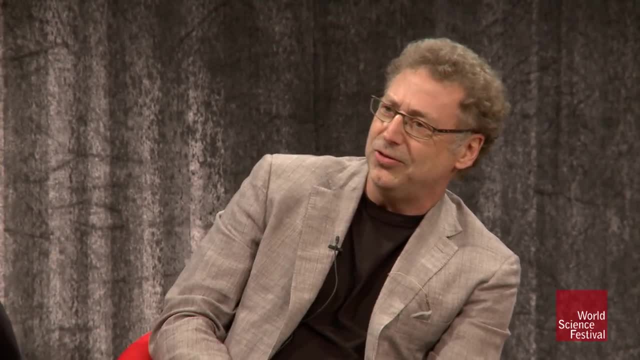 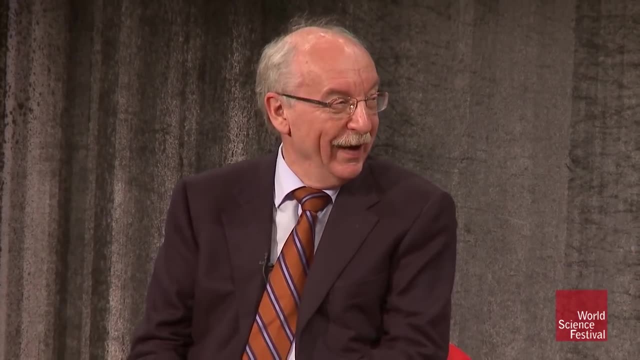 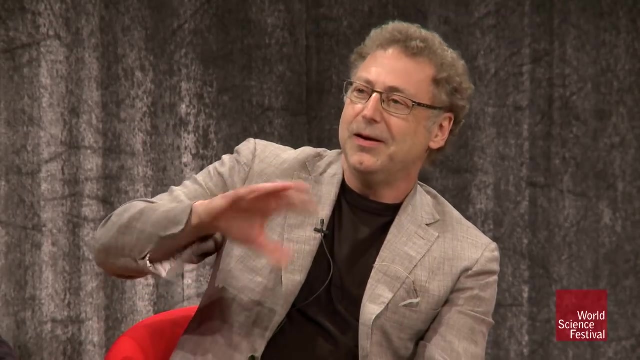 even use the word false positive. He says: well, the chances that this is wrong are one in a thousand. That's wrong. Well, that was the false positive rate back under that test. but given my circumstances, the chances of you know, given my- you know, drug use level, homosexuality and all the 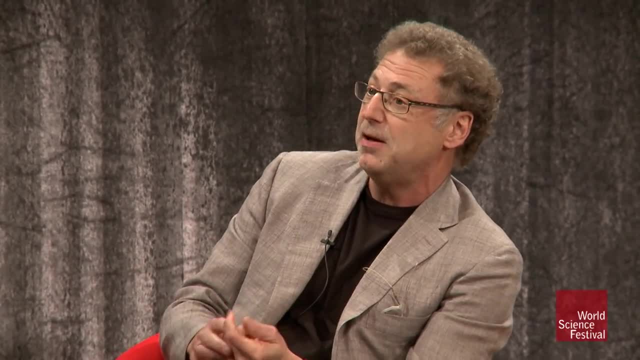 other things that you put in my, my, my population, the chances of having it Back, then we're one in 10,000.. So he should have told me that chances are nine out of 10, that this is bullshit, I'm sorry. 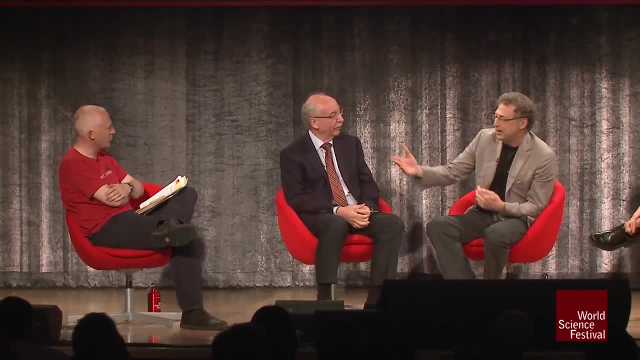 Can I say that? No, that's fine. Yeah, It's my emotion. It's after the. He didn't even he didn't know it was the worst false. He just gave me a pronouncement. Like I'm the doctor. 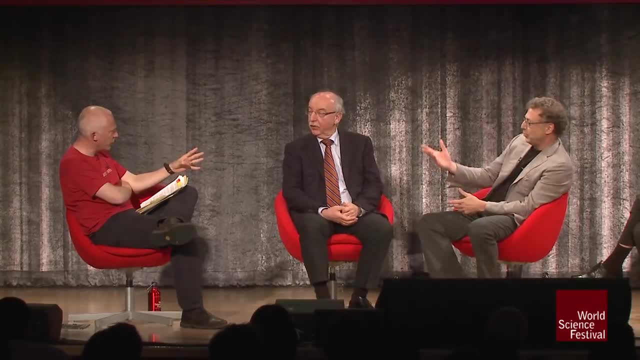 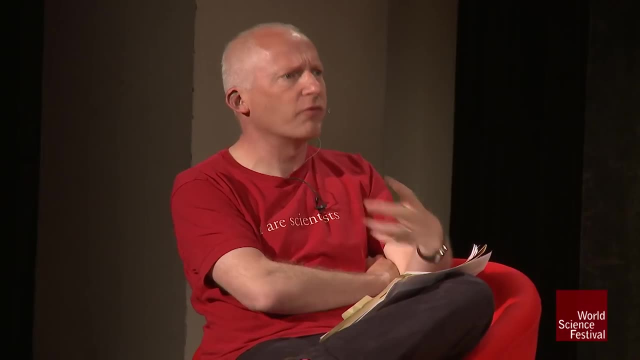 Here's the answer. But that was ignorance on his part, wasn't it In some way? But I think that, well, what about the media? Because I think so often headlines, you know that things like cancer, if I can, you know. 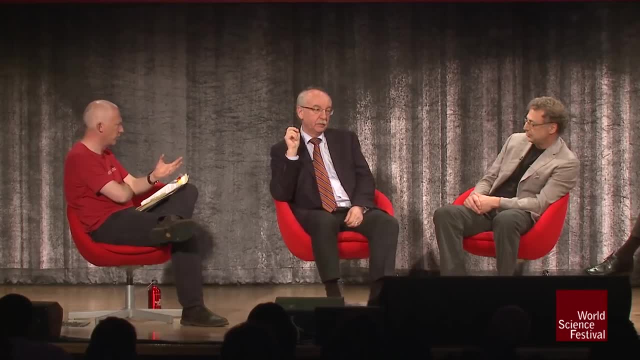 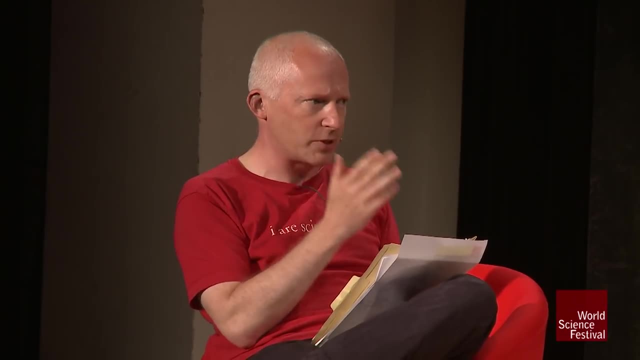 50% increase in the chance of cancer if I eat bacon, Bacon or something, And actually you know, it sounds scary, It sounds like, oh my God, I'm going to get. but but the get that that seems to me sometimes. 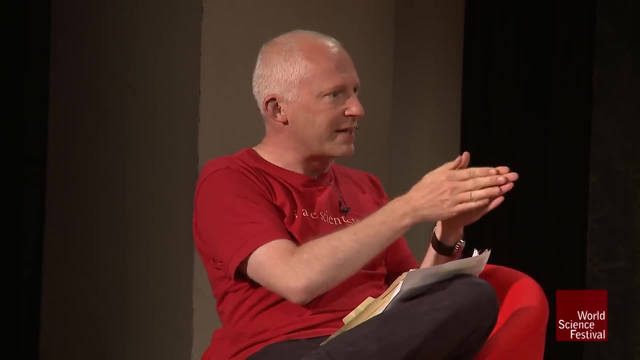 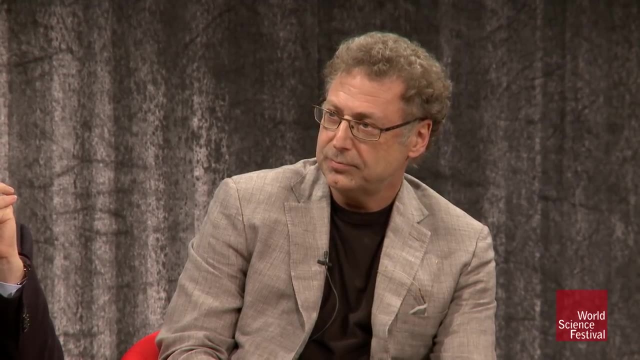 a malicious use because you know the number of people who might get cancer in eight out of thousand And now if there's a 50% increase, it's again coming back to these natural frequencies make sense of. actually that it's a very small increase in the numbers, but it's a very scary. 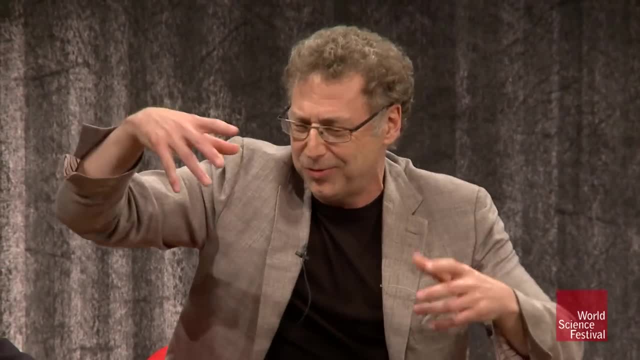 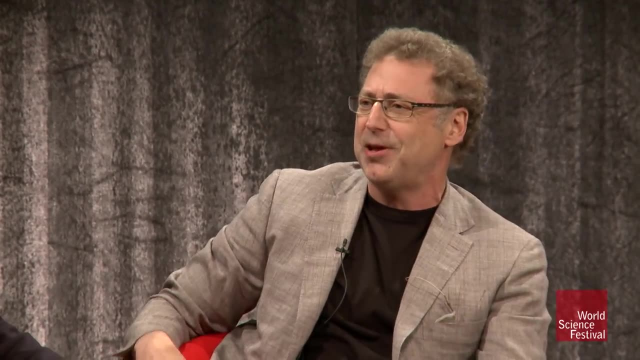 sounding statistic. This will double this whole. this, this uh, whatever it is on the radio, uh, using your cell phone, Yeah, We'll increase the kind of brain tumors by a factor of three. three times as many people. 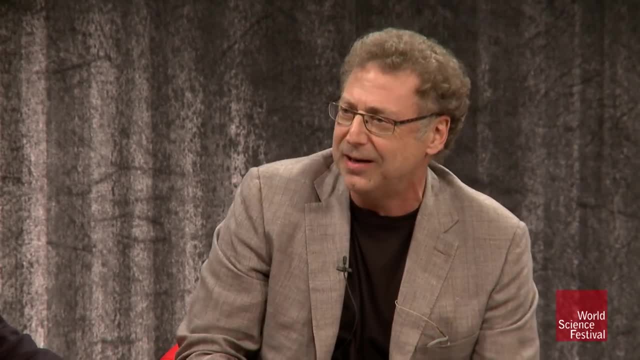 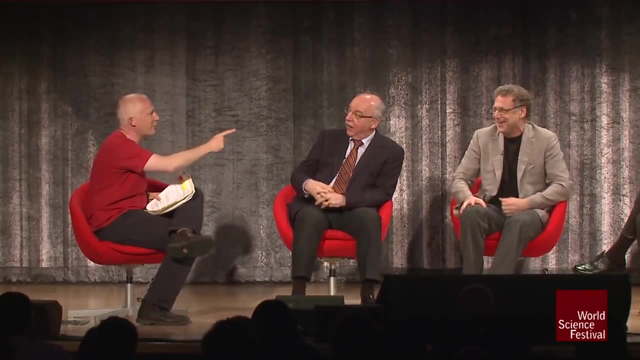 That means, instead of one in a hundred million, three in a hundred million are going to get it. Yes, I worry about it, Exactly, But as a media story, it's much more exciting to hear Um, so, uh. but well, I am going to get you started, because I mean, do you think that? 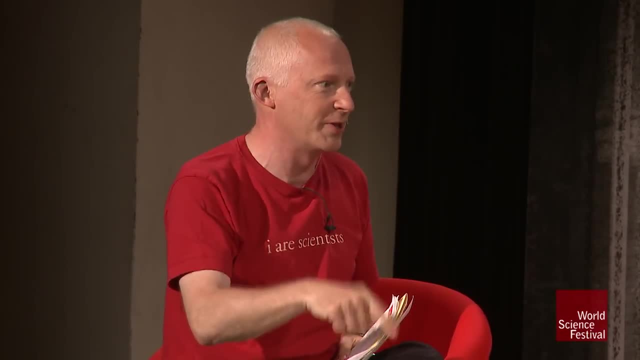 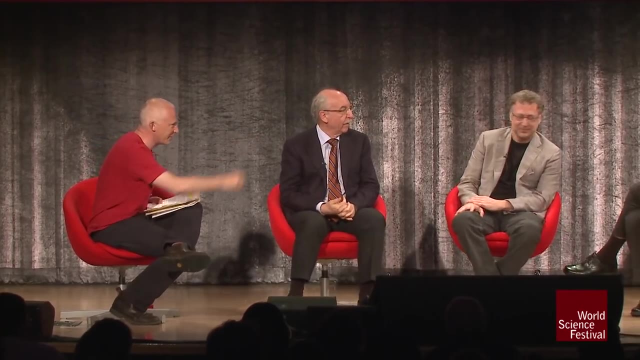 actually it's journalists not understanding, or journalists who understand, but they sell more newspapers because if they do it in that way, it's a much more exciting story. I think they don't understand. You think they don't understand, but somebody's selling them. 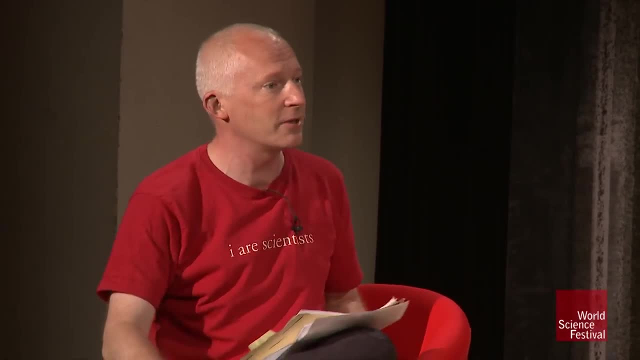 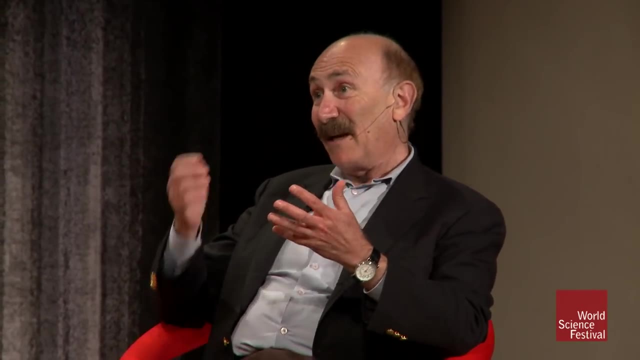 Who's who's Who's giving them that statistic, then? Is it the scientists who are telling them? the problem is- the problem is to be fair- that Bayes theorem is very complicated and we should maybe mention part of its history. Uh, when Bayes derived it in the 1700s, he was trying to prove the existence of God by 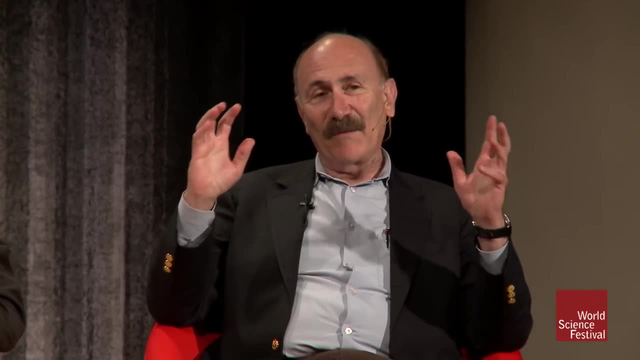 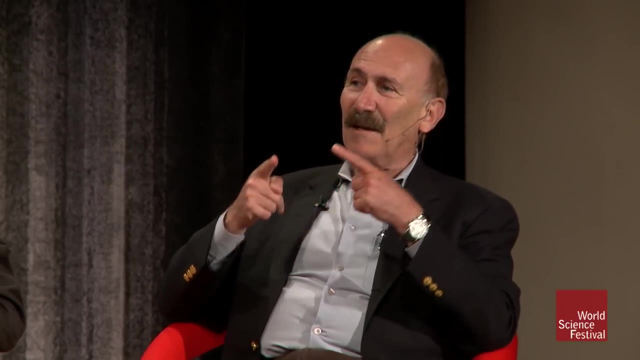 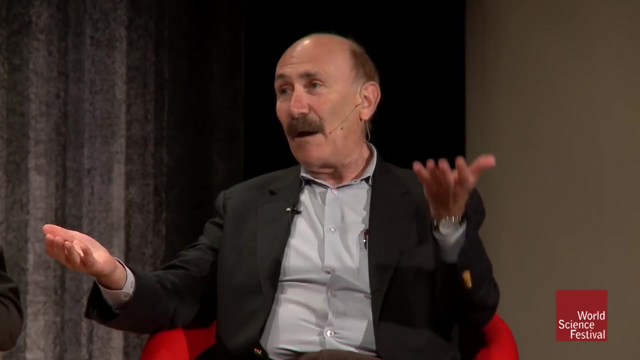 changing probabilities around. So the problem of Bayes theorem is is is a very complicated thing and what it does, really in simple world words, is to mix, put together two things: the prior probability, which is very small. I'm basically saying that, with the reliability of the test, the test may be very reliable. 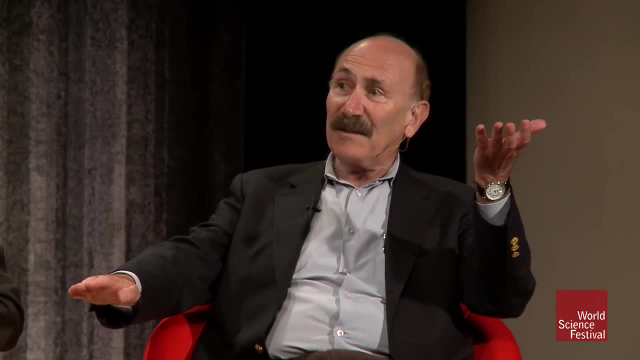 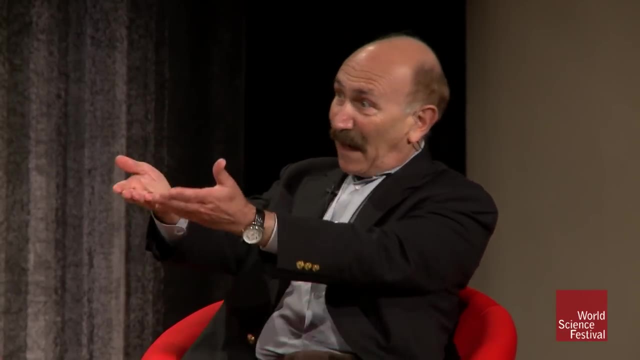 90% of the chance it's right. but if the probability in the population is very low, of course you'll still get a small number, even though it's orders of magnitude higher, or say, an order of magnitude higher in your example, than what you started with. 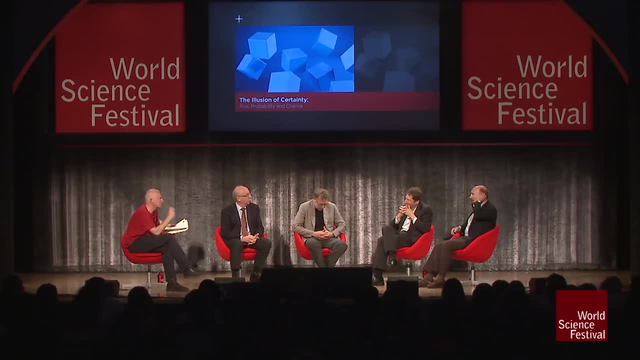 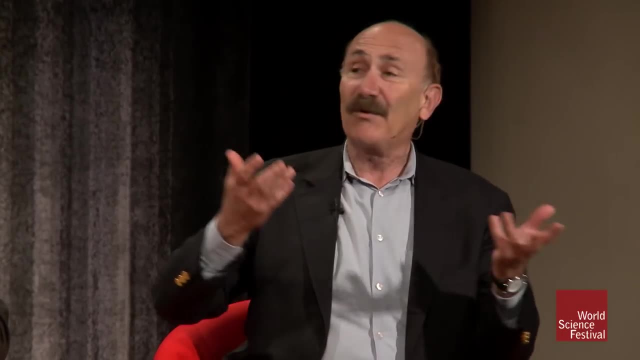 But hold on. The problem here is sometimes the priors are not used correctly. That's the main problem with Bayes theorem. Sometimes we don't. What is a prior? A prior is a probability that we think we know from something else. 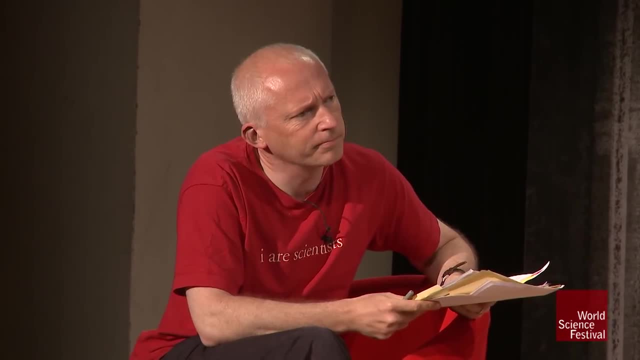 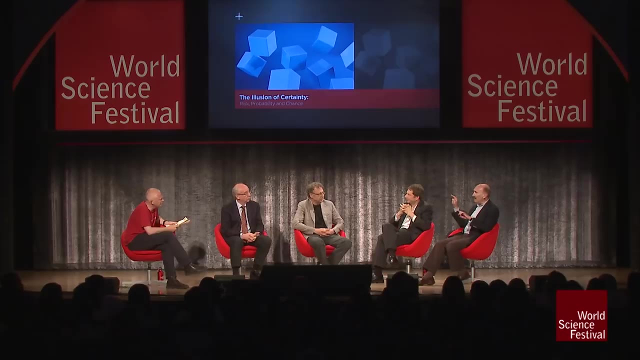 Like we know that in a population so many people are ill with the disease or something. In that case it's okay, We do know. But if you give the test in a hospital, you can't. you can no longer use that prior in. 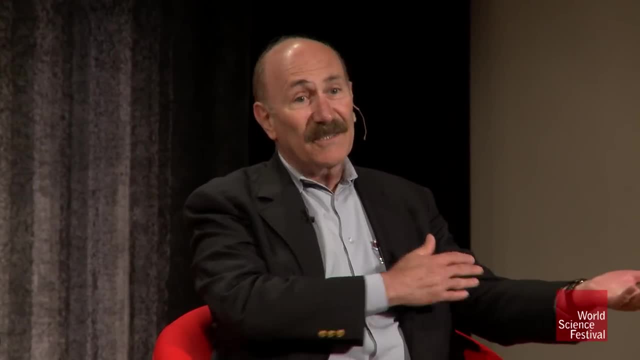 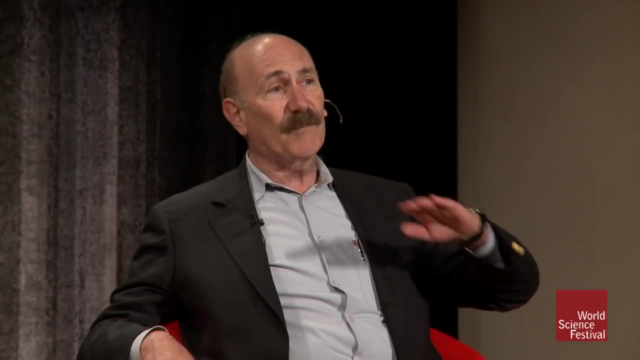 a whole population. Somebody comes to the hospital to get the test because there's a reason they're not feeling well, They have some kind of symptoms, some some of the symptoms. So if you're going to use that prior, that comes from the overall population you are. 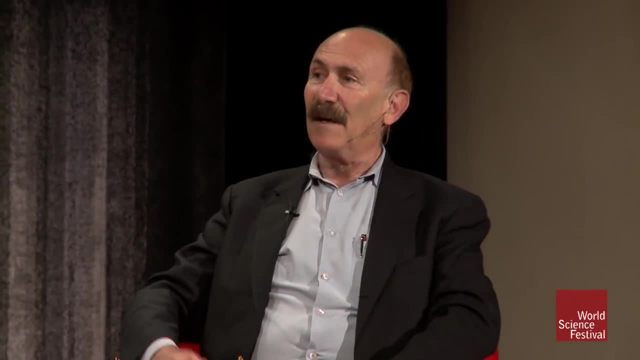 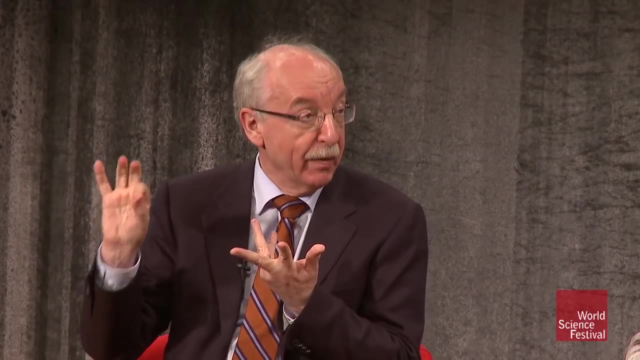 doing something statistically very wrong, And that's yeah. That's why, for instance, the- the numbers I gave you- they hold for screening but not for diagnostic mammography. That's important, But there are other examples about confusion that are much more simpler. 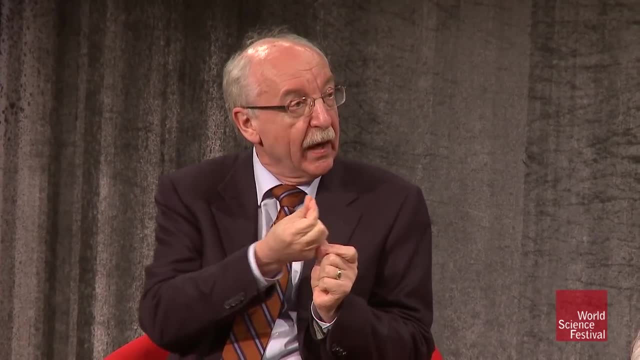 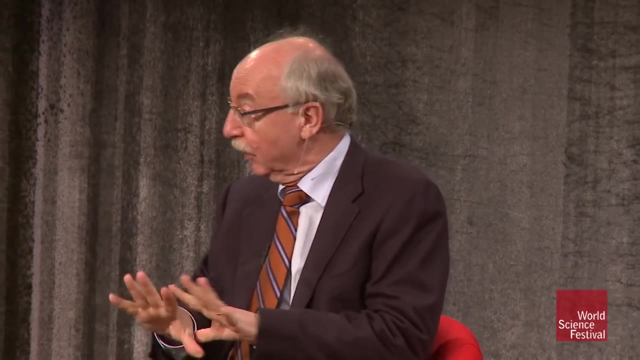 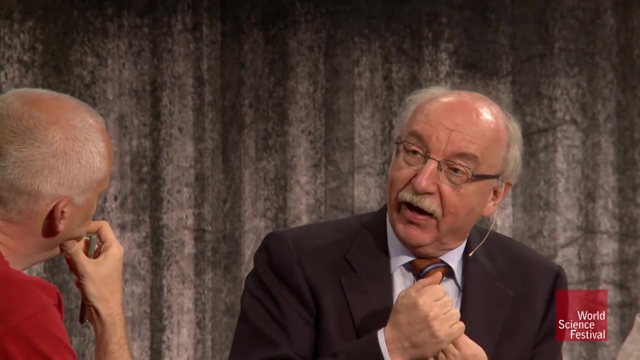 And the example that was here was about relative frequencies And the to answer your question. so I I'm training journalists. Most of them have they learn everything in journalist school if they go, But not statistical thinking. To go, take an example from your country. 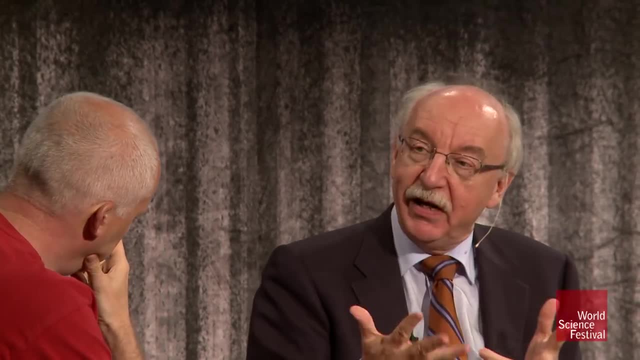 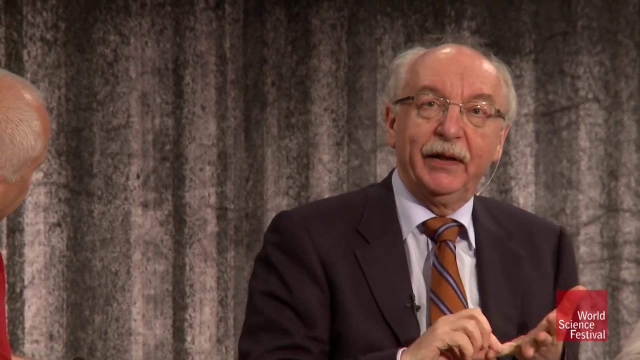 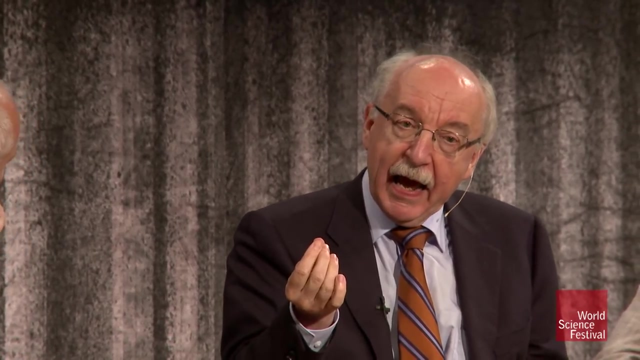 So in in the UK there is every a few years a contraceptive pill scare And it's done exactly this way. So one of the most famous one went this way: The newspapers reported that women who take the pill of the new generation their chance. 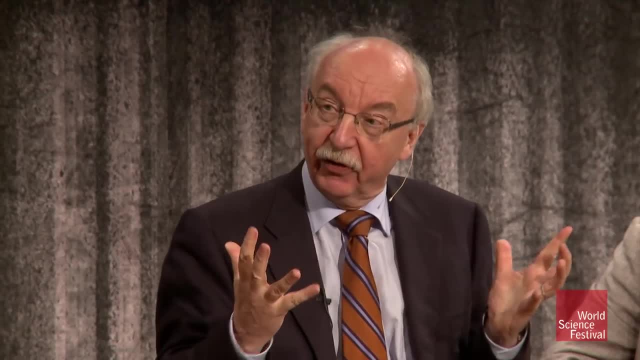 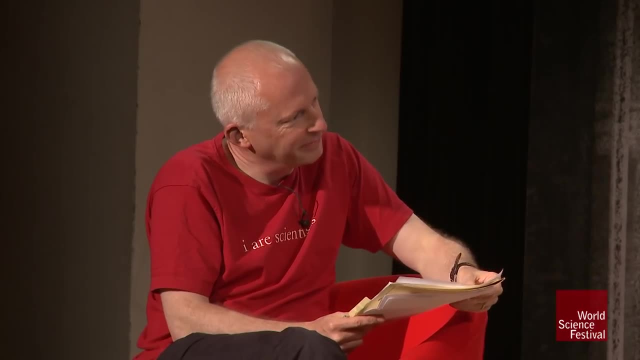 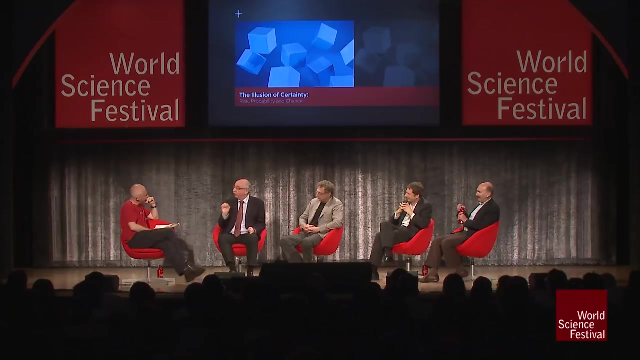 to have a thrombosis increases by 100%. Now, 100%, that's certain, isn't it? So many British women were frightened and immediately stopped taking the pill, which led to unwanted pregnancies and abortions. What had the study shown? 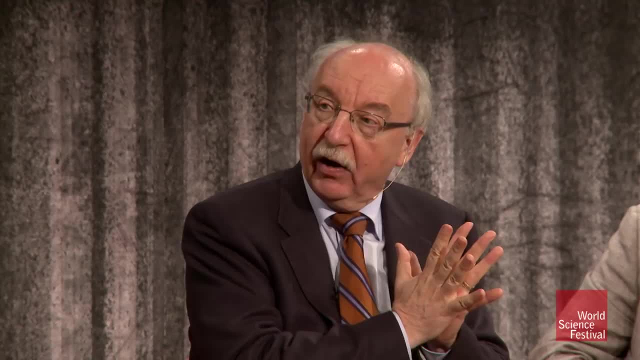 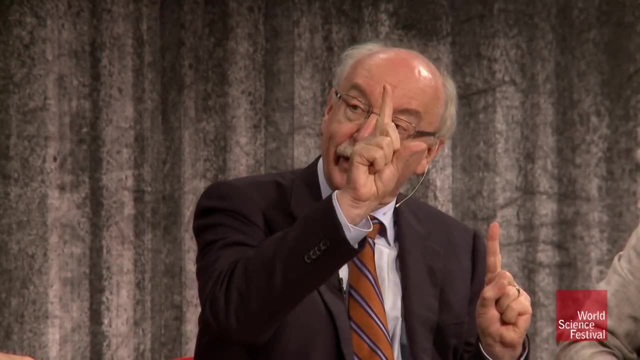 On which the journalists reported. It showed that out of every 7,000 British women who took who took the pill of the previous generation, one had a thrombosis. And out of every 7,000 who took the pill of the new generation, only one had a thrombosis. 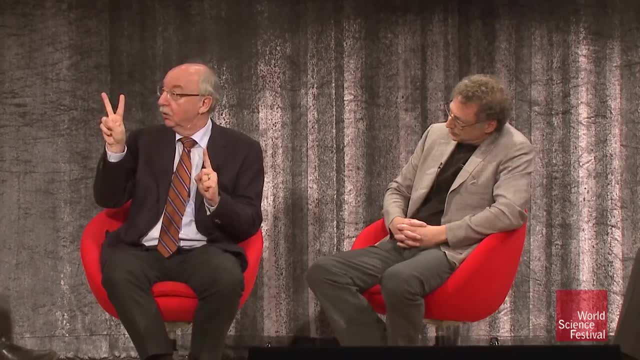 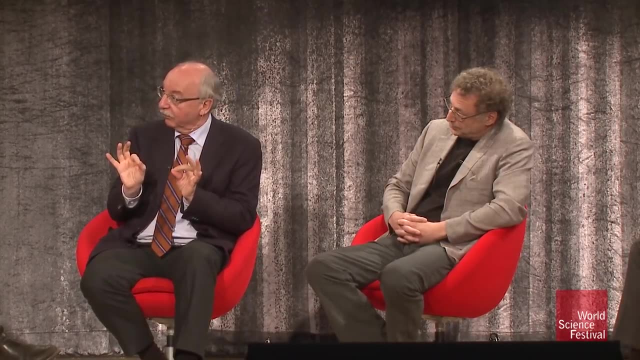 So what does that mean? it increased from one to two, but that's 100%. That's called a relative risk. That's the same as one in 7,000, that's called an absolute risk. And the difference between absolute and relative risk. 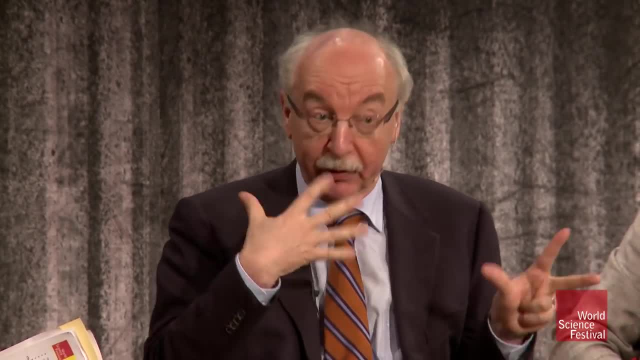 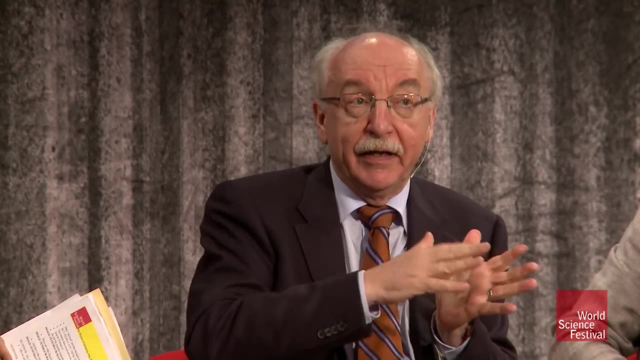 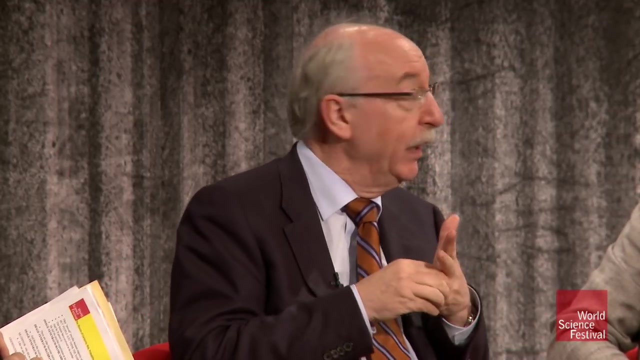 is still not known to the British population, nor the German nor the American. And this, only this one news, caused in the following year 13,000 more abortions than usual. And the answer was: in this case, everyone was hurt. this poor woman. 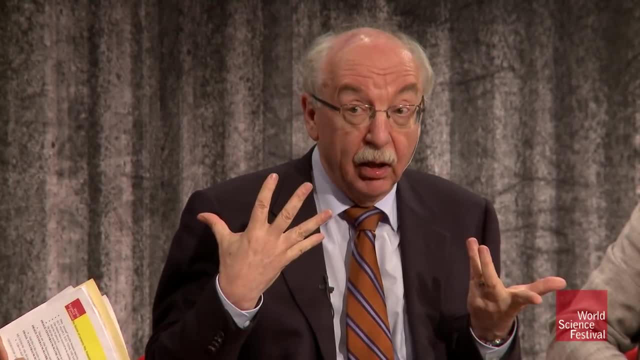 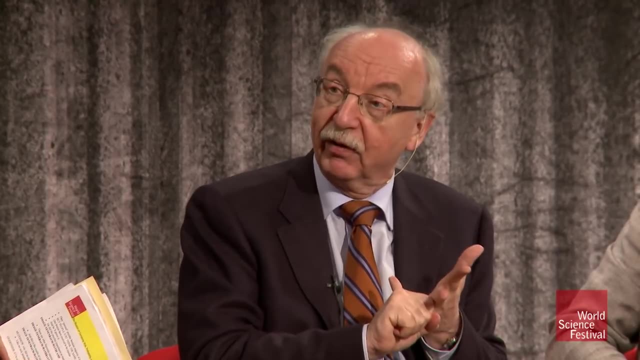 And an abortion is something that stays in with this woman for the rest of their life. The pharmaceutical industry was hurt. The only one who had something from it was the journalist who got it on the front page, And it's repeating. It's repeating all few years in the UK. 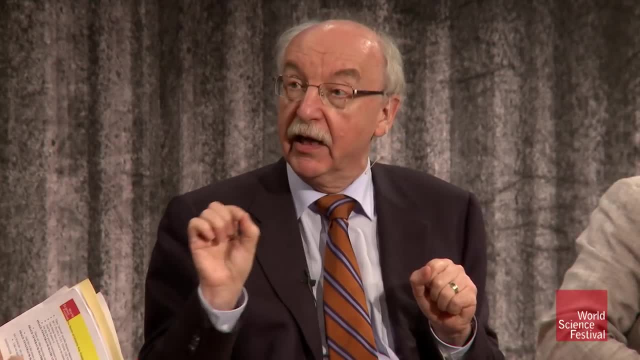 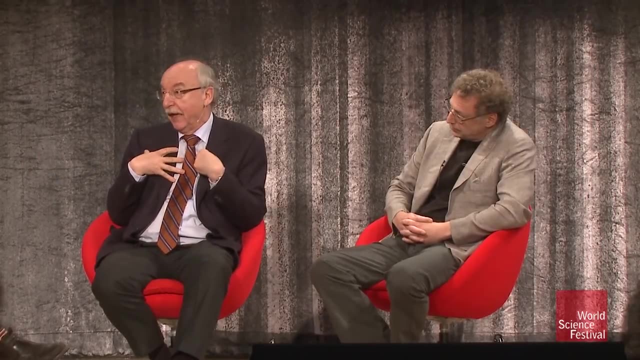 and there's no learning. And your question: where do the journalists get the number from? From the top medical, from the top medical journals, The British medical journals, for instance. I wrote last year an editorial in the British medical journals about how the journal misleads their own readers. 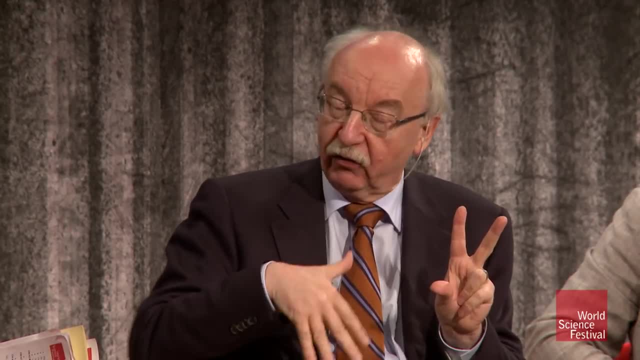 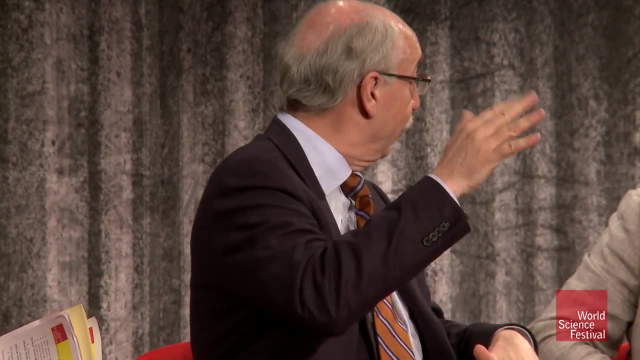 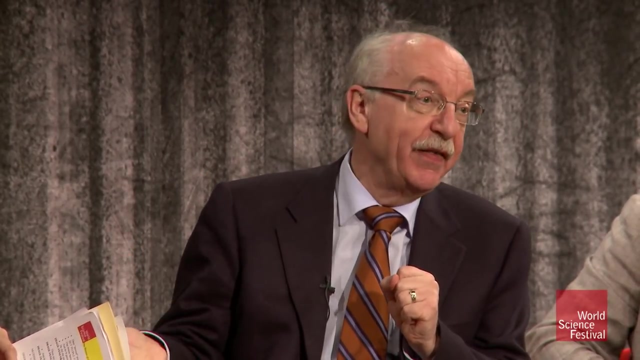 by, for instance, reporting, allowing the studies report the benefits of a drug, for instance in relative risk decreases 50%, Lipitor 50%, but the harms in absolute numbers, one in 1,000.. Yeah, It can be more or the less. 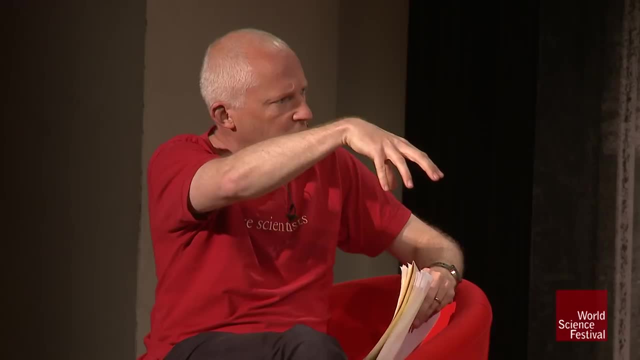 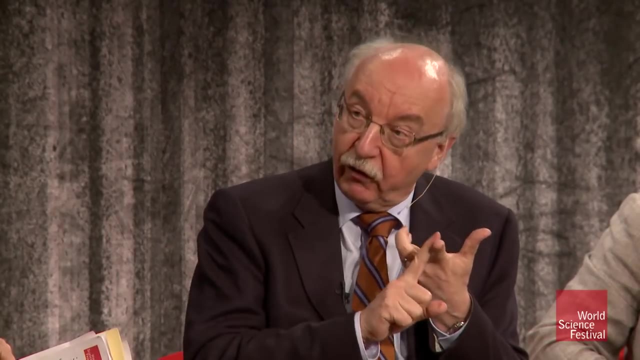 So you think there's a kind of miscommunication between, say, the academic world who understand these numbers, and then they look at the journals and I would say there is at least in health care but also in finance. there's a systematic attempt. 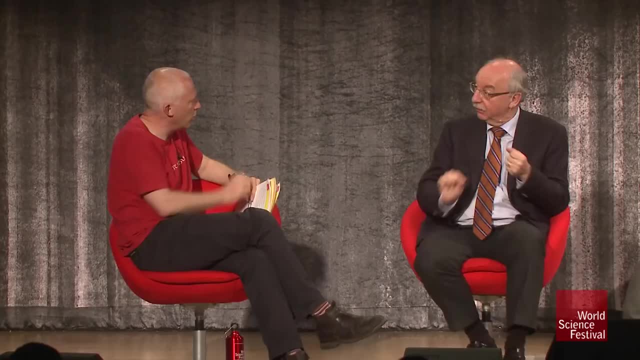 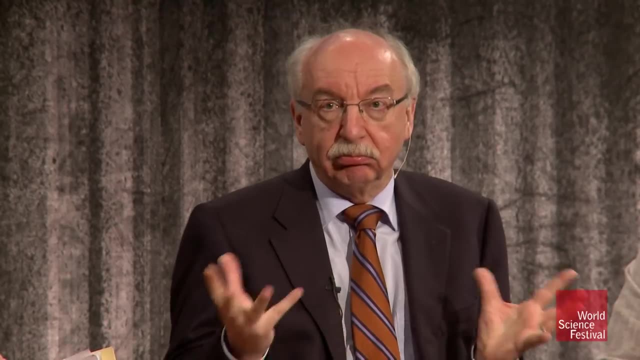 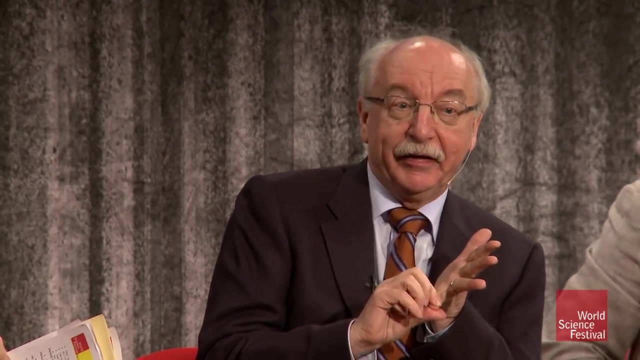 to mislead the public. A system on behalf of, by the journalists or by the academic. The journalists are more or less hopeless. They don't know, But it is. It's The, The editors, the editors of the major journals. 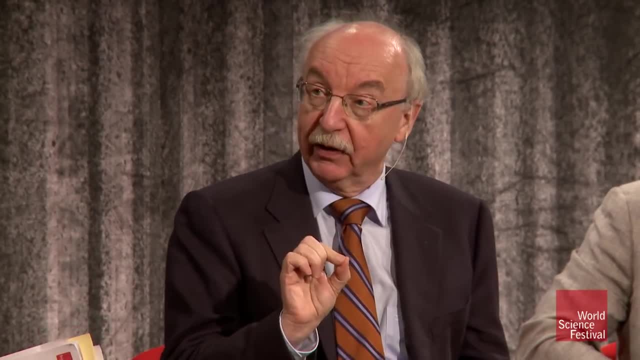 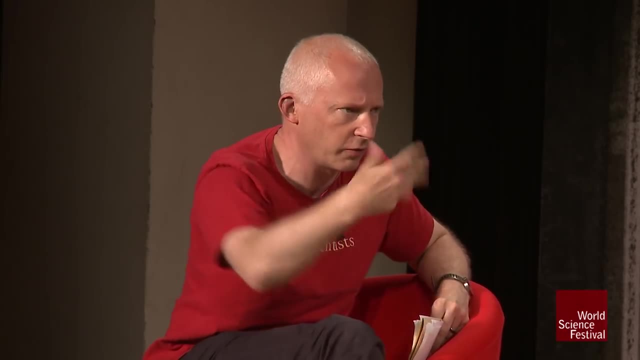 in the US or in Great Britain. it's their responsibility to change things. I'd like to come a little bit to sort of the idea, because the experiment you did with the birthdays, I think, shows how amazing that. See, if you'd done that without telling us. 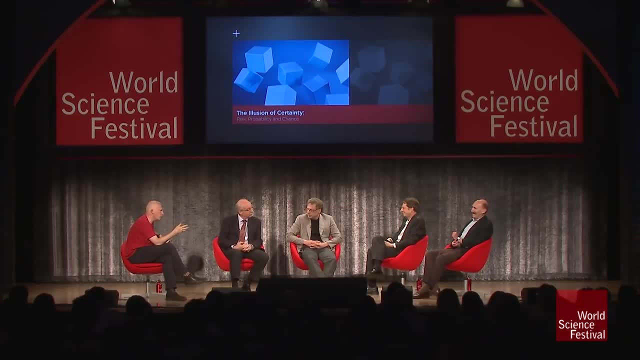 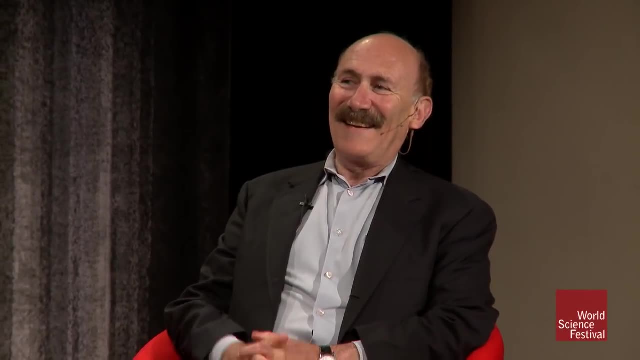 it's an amazing coincidence. You think that- And the idea of coincidence is used, I think, also sort of abused by people in sort of reinforcing the idea of spirituality. Yes, amazing things I mean. Josh, I think you've got some slides which explore. 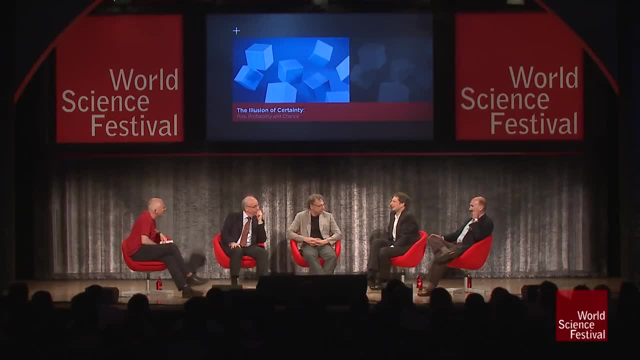 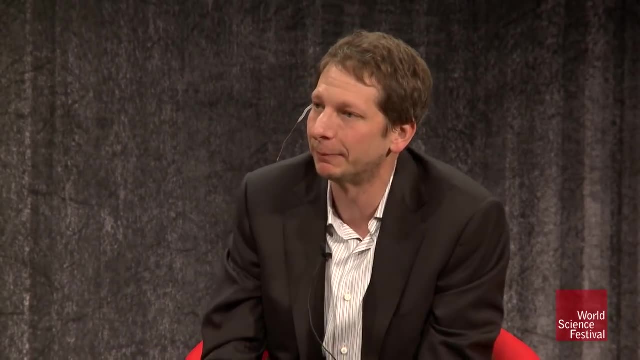 I mean also your experiment at the beginning, I think Yeah, I mean I wanted to jump in a little bit to defend the honor of Bayes' rule. Okay, Bayes' rule is very complex when you apply it to the kind of numbers, the decimals, we're talking about there. 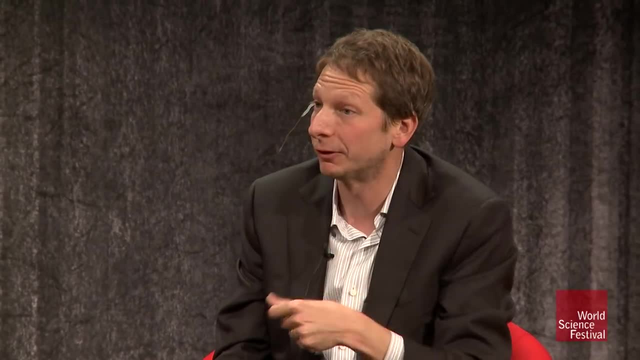 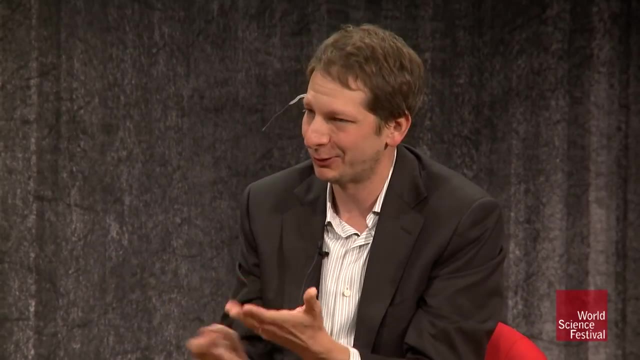 But all the models that we're talking about, about how our brains see patterns up, they're essentially doing a kind of Bayesian inference. I mean, I think you can see this in the intuitions. like you know, medical diagnosis from statistics. 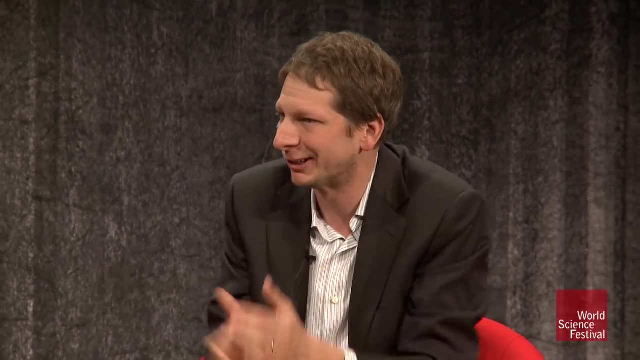 like the kind that you're talking about are. you know, all the errors that you've talked about are real, But think about our intuitions. you know our friend is coughing one day. or just see someone you know on the street. 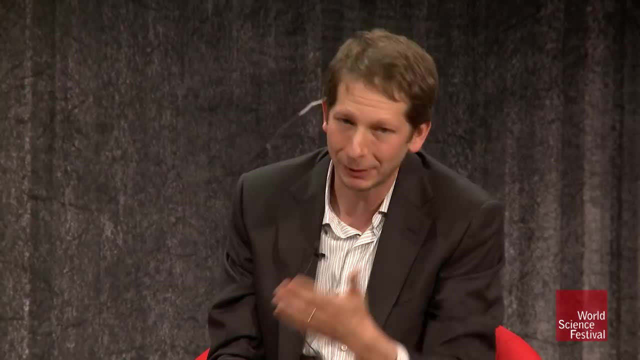 or next to you here in the theater coughing. What do you think's wrong with them? Probably you know they have a cold. maybe you don't want them to breathe on you, right? But there are other possible alternative hypotheses. 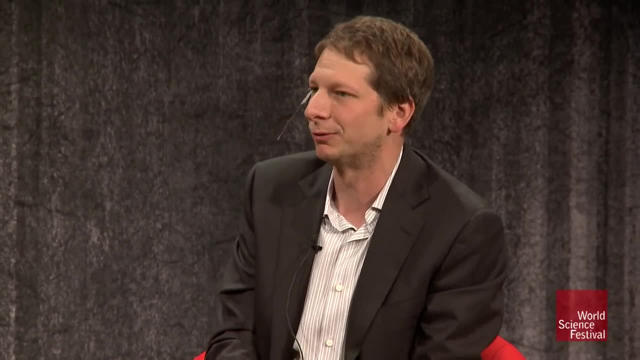 Maybe they have lung cancer or emphysema, or maybe they have, you know, extreme, drug-resistant tuberculosis. Now why don't we think those things? Well, we don't think those things, We're optimists, Because we're optimists. 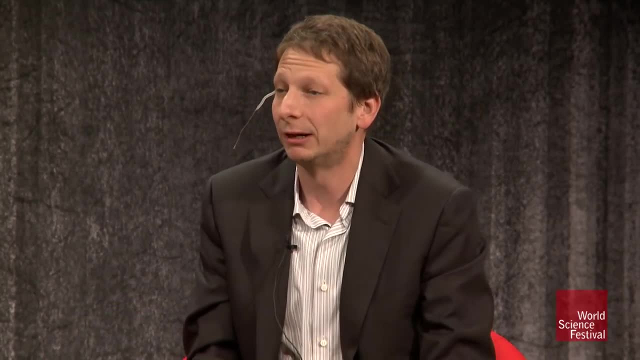 and maybe because we have some sense that those are less common, thankfully, right Now. if they're older and maybe you saw them smoking before, then you might be more likely to think: oh you know, maybe he's got emphysema. 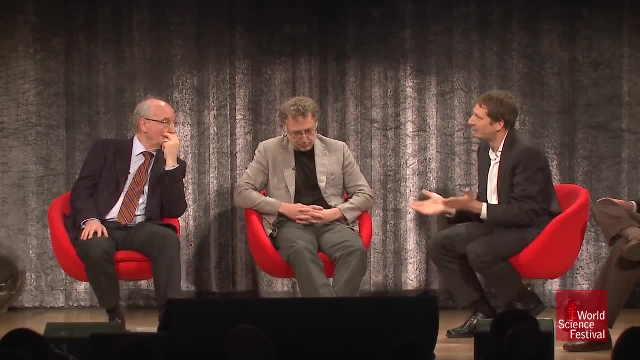 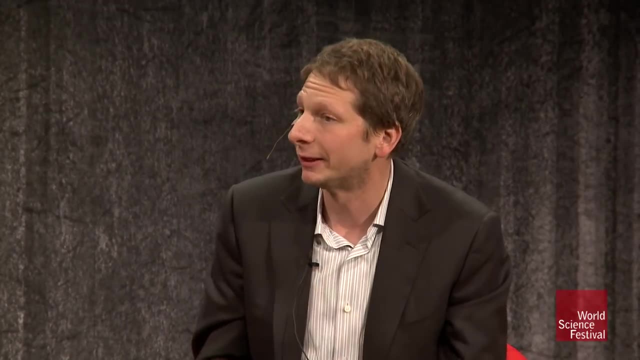 or he's on the way, Or if you, you know- let's say you were in the hospital on the, say, infectious disease ward and somebody's got a bad cough- then you know, you might think a little bit differently. 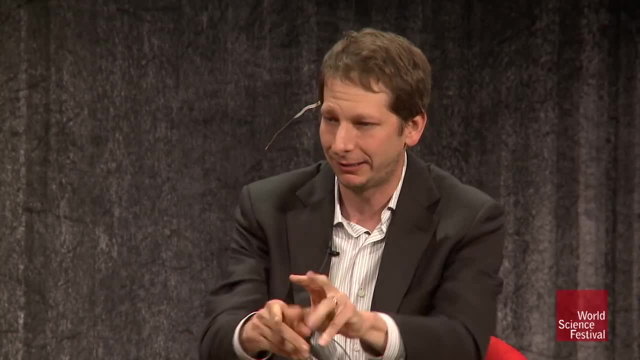 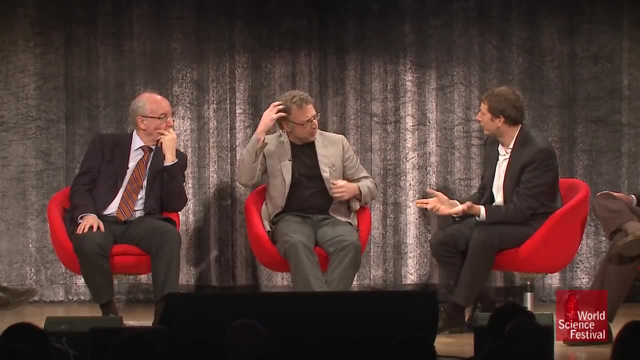 And so there is, I think, unconsciously, implicitly, not in you know, data in the form of numbers, but this kind of more experiential reality. Have behavioral economists done experiments to see if people use basing? Well, that's one of the main things from. 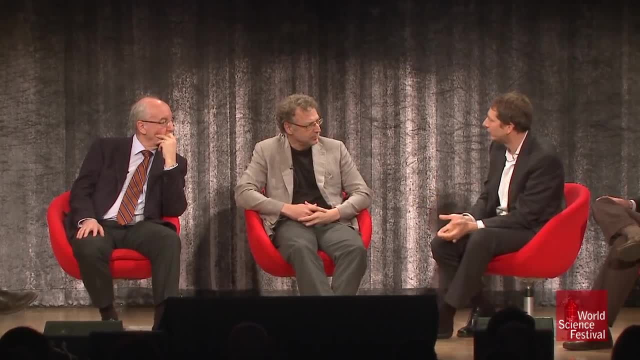 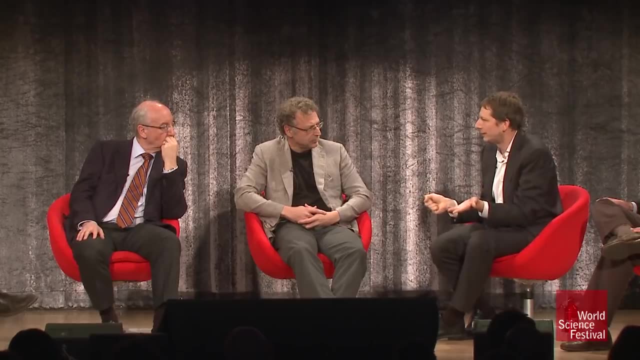 that comes out of psychology, of judgment and decision-making and behavioral economics, is that it makes a difference when you experience events like this, that it's very different than just you know seeing the numbers in the form of decimals, And we are, I think, implicitly 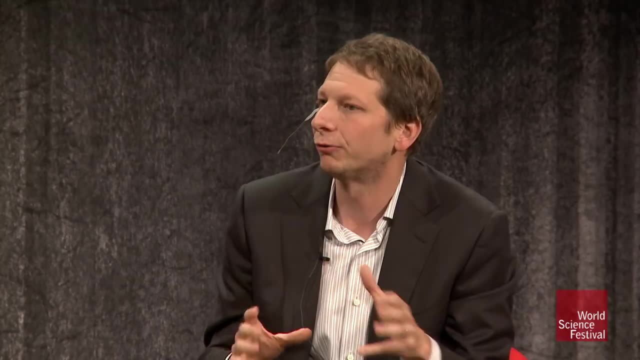 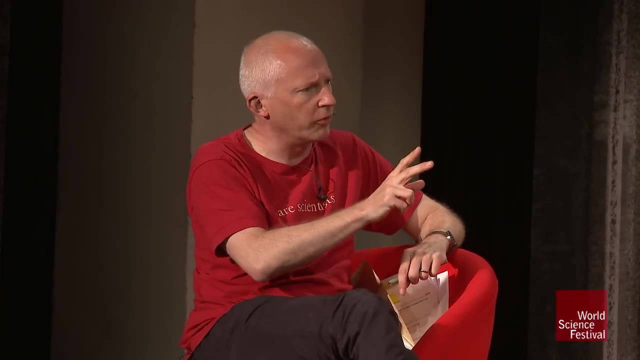 not ideally or perfectly, but taking into account all the different kinds of things we should in roughly the way that we should. Now I'd like to come back to your: how good your psychic abilities are. Yeah, should we take a look at that? 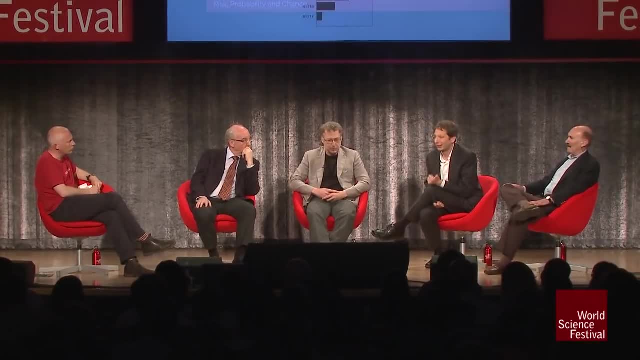 Should we take a look? Yeah, I mean because. So people might be wondering first of all what that was about. Wait, hold on, don't show that yet. Don't look this way, don't look. You might be wondering what that was about. 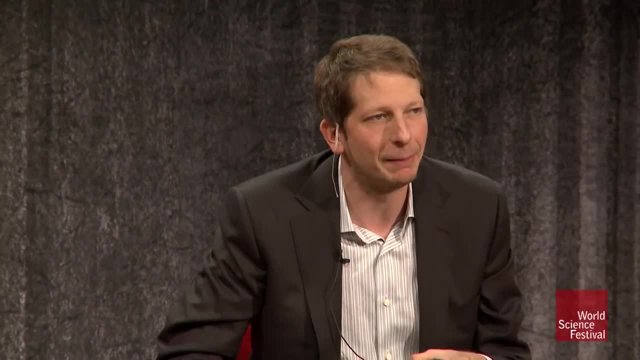 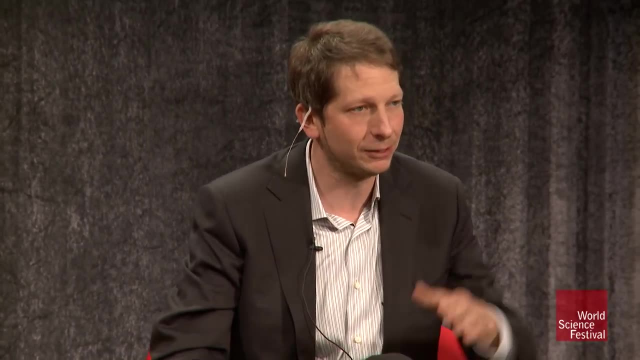 and whether you got it right. So let's first see how many people got it right. If I remember right, the sequence that I flipped was heads, heads, tails, heads, tails. Now, do you guys remember? Oh my God. 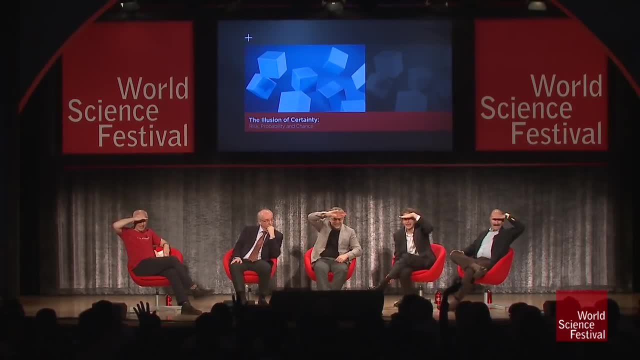 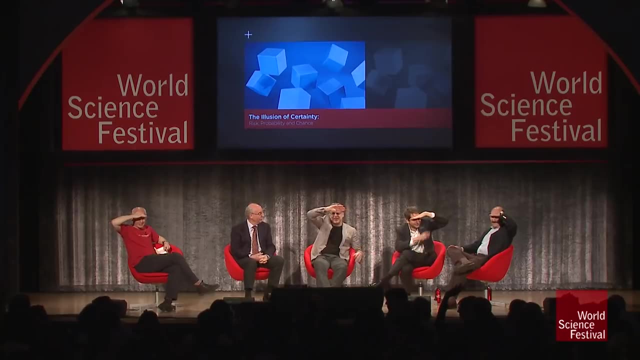 Can you raise your hand if you remember getting that right? Oh, my Heads, heads, tails, heads, tails. Now can you count that up? Is that It's a lot? Yeah, that's Quite a lot, Not quite a lot. One, two, three, four, five, six, seven, eight, nine, 10,, 11,, 12,, 13,, 14,, 15,, 16,, 17,, 18,, 19,, 20.. 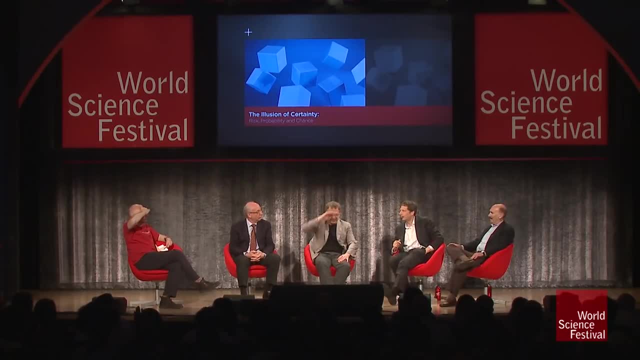 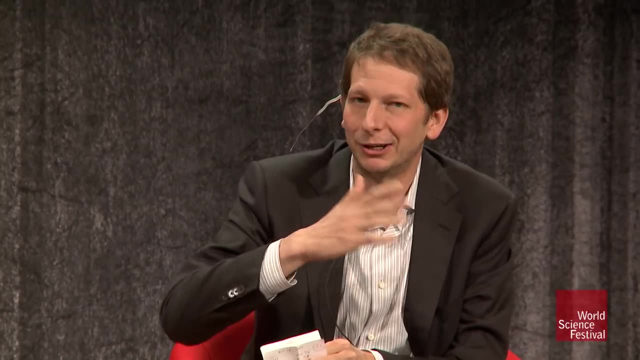 Well, double the size of them, about 40.. Now I actually wrote down before thinking, based on how many people they said were here, what's the p-value, The probability of getting a number that extreme by chance, And it actually goes off my chart. 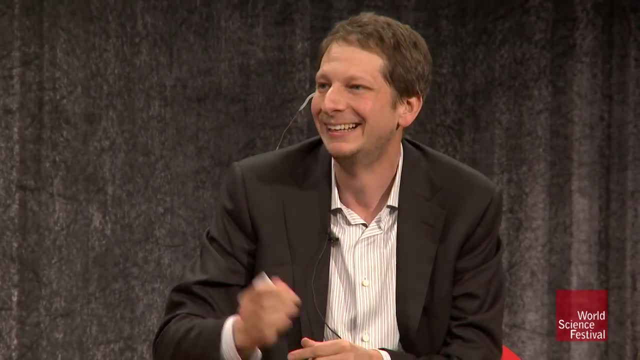 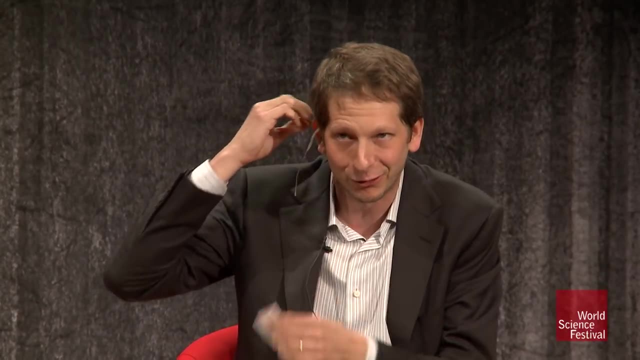 It would be less than one in 10,000, actually. Oh, okay, So you could publish that result in any journal And, as we know, many people read about this in the Times and other places. There's all sorts of 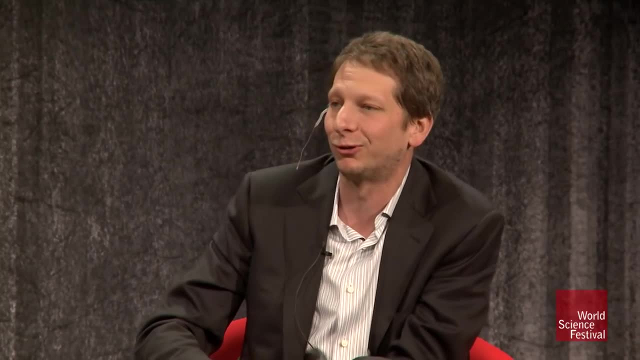 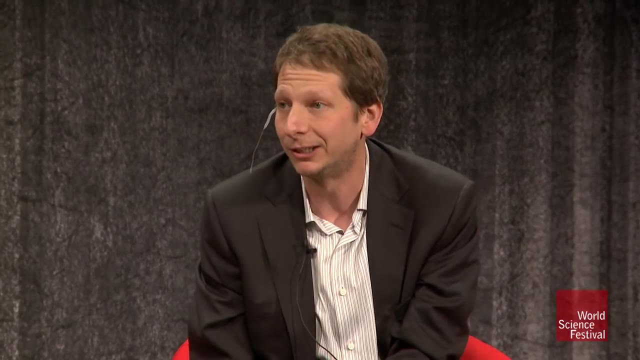 or there's some recent research published in the most prominent social psychology journal, by Darrell Benn on people's psychic abilities. Now, those are very subtle and interesting studies and I'm not gonna talk about them. But what's really going on here? 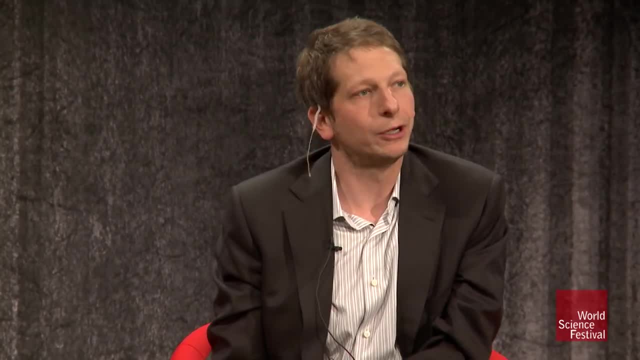 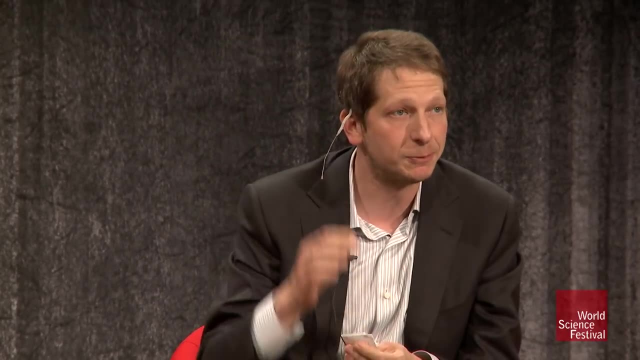 Well, it could be that there's psychic transmission going on, or it could be that maybe you're just writing things down at random, And this is actually a replication, if you like, of an experiment that was originally done by the Zenith Radio Company in the 1930s. 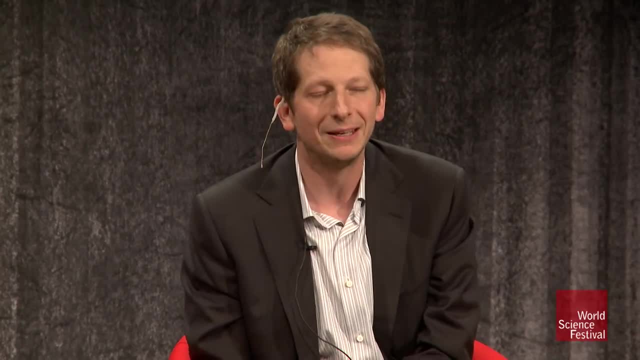 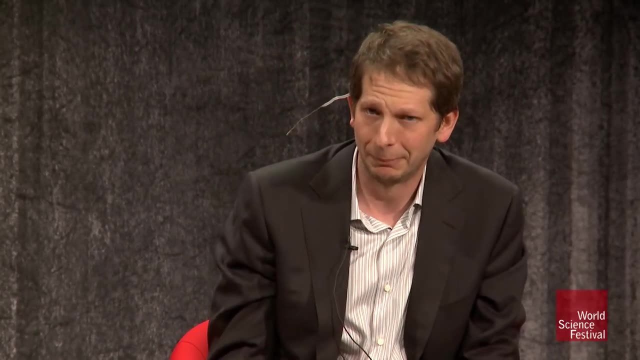 the golden age of radio, but also a golden age of interest in ESP, And they wanted to test the ability to send messages psychically across the country. And they had psychics in the studio, I believe, here in New York. I'm not sure about that. 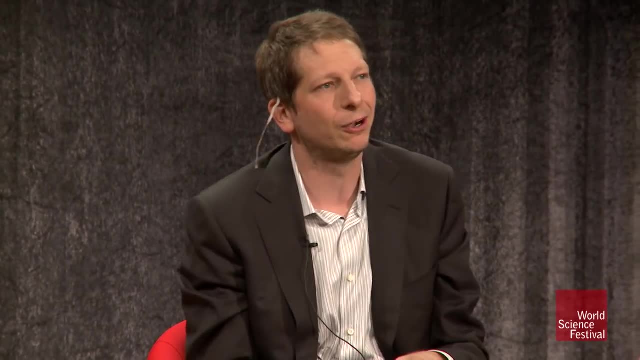 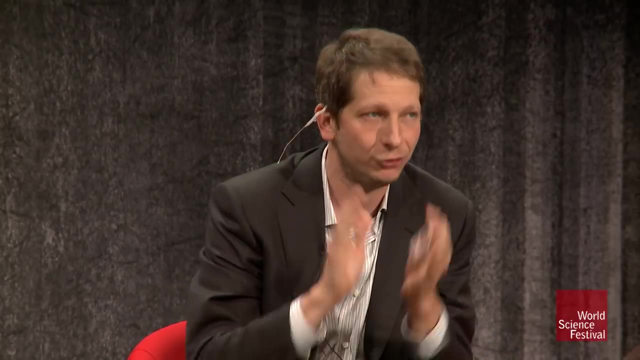 flipping coins or looking at these ESP cards- You might have seen pictures of them- wavy lines and crosses and so on- and sending out these sequences just like that, And then having listeners all around the country try to get the message and send in postcards. 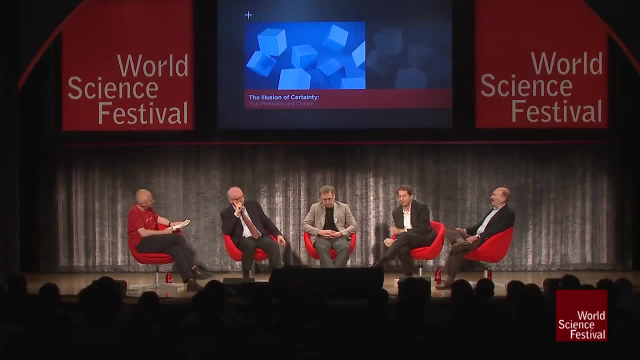 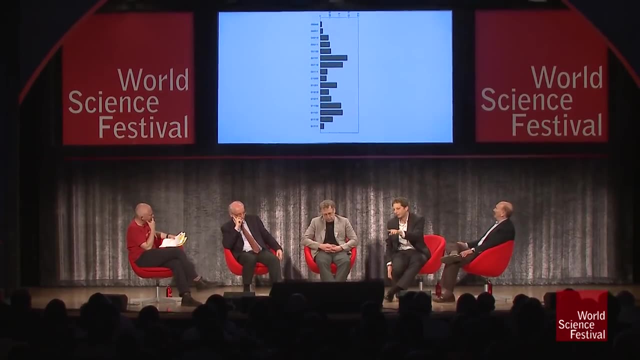 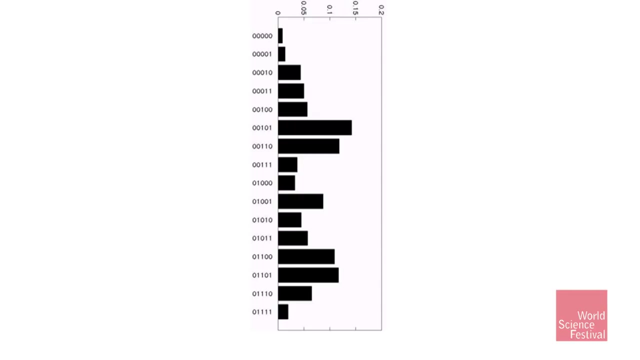 reporting back the data Now. the first slide is actually the data from those Zenith Radio experiments done in the 1930s And it's collapsed in a slightly interesting way, but I think you'll probably be able to get it If you have these five-bit sequences. 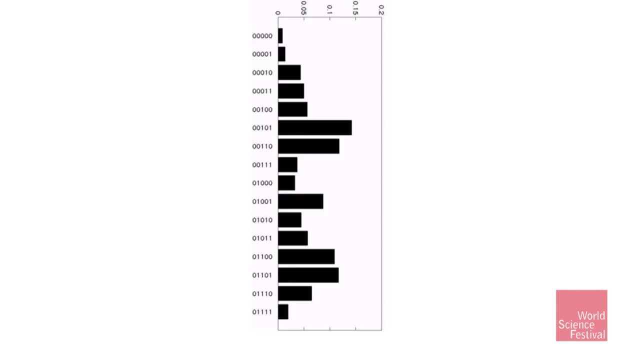 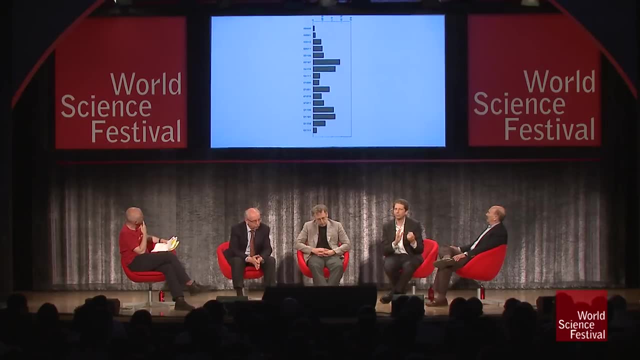 sequences of binary two possibility outcomes like heads, tails or black, white, or here it's all written in terms of zero and one. what we're really interested in is your sense of coincidence and randomness in the sequence of the data, So we don't really care about the difference. 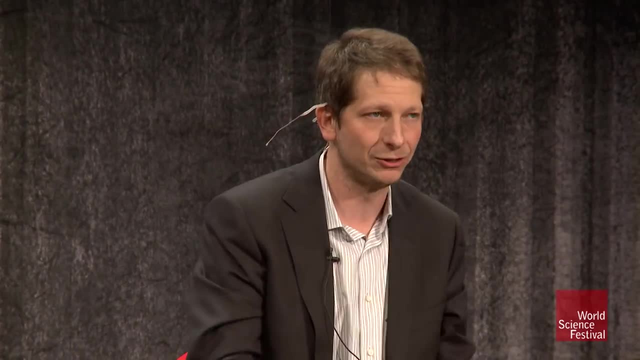 between heads, heads, heads, heads, heads and tails, tails, tails, tails, tails. What matters is that's a run of five things in a row. Similarly, we don't care about the difference between heads, heads, heads, heads, tails. 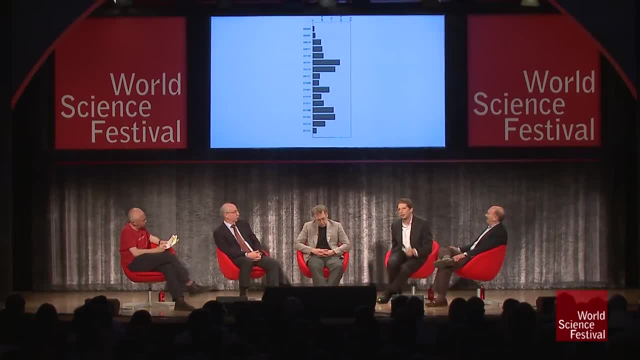 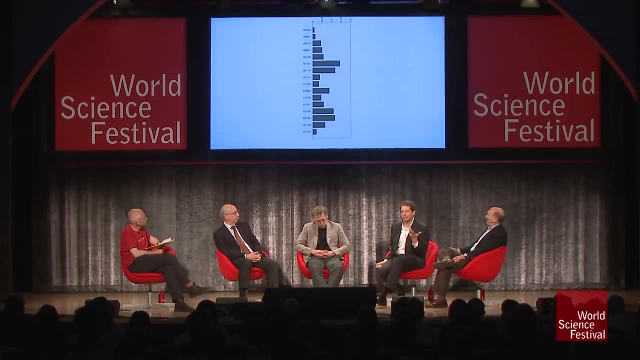 and tails, tails, tails, tails, heads. So here the data has been collapsed across what we call parity, or replacing heads with tails and vise versa, And what you can see here is that some patterns were just much more likely to be written down than others. 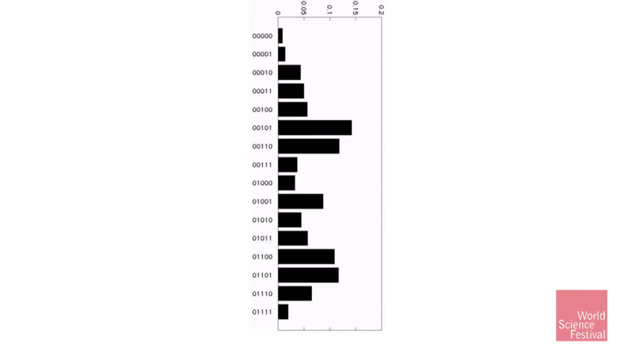 So, for example, the one that I happened to flip tonight is this one: 00101.. That would be heads, heads, tails, heads, tails, or tails, tails, heads, tails, heads, And the number of people who wrote that one in the name. 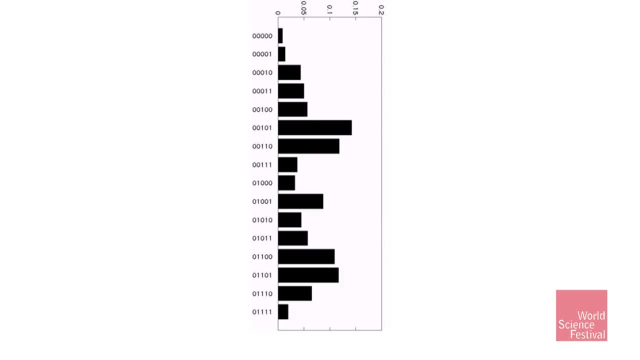 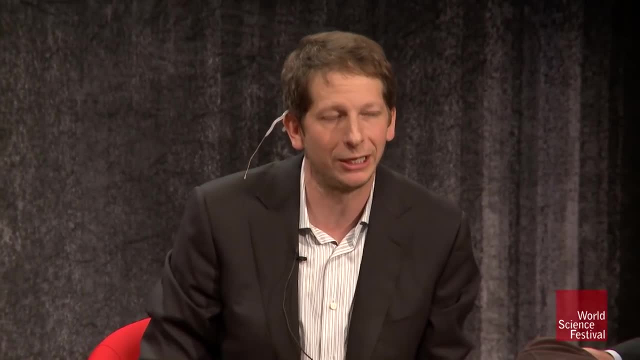 in the 1930s is well, maybe 100 times some of the other sequences. Again, if that just happened to be the lucky sequence, then it would provide extraordinary evidence for psychic powers. But we would now say: and psychologists have long. 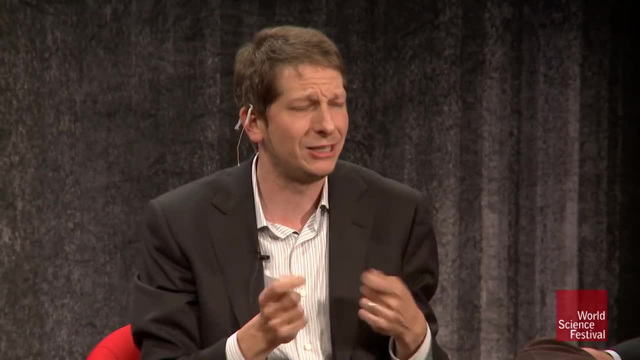 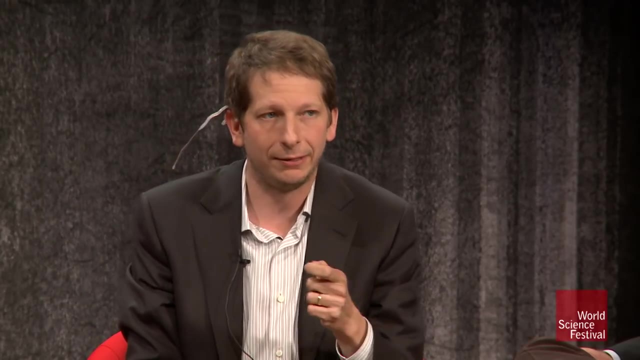 understood this as just tapping into our intuitive concept of randomness, saying not all patterns of a random process look equally good, equally like random. Now it's interesting here, I think, that what makes something look random or not? Well, a sign. 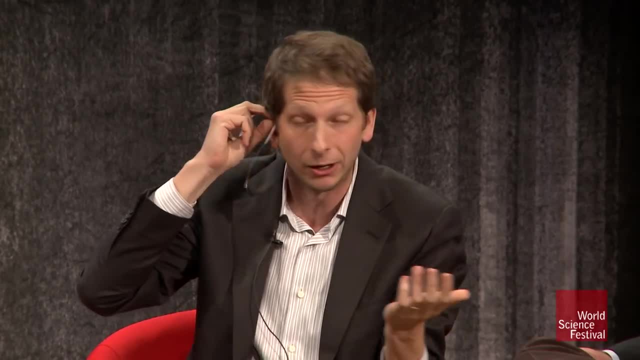 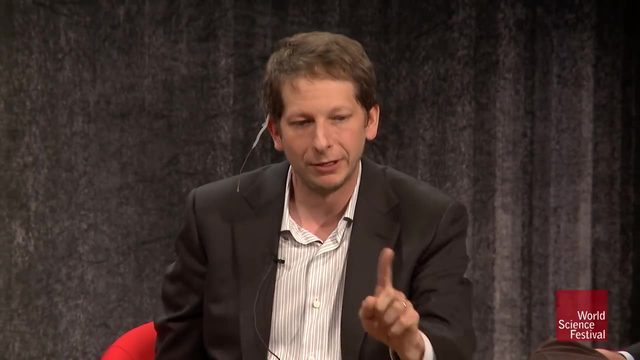 Sorry about that. A sign that I think there's really something quite fundamental about our brain's mechanisms for finding structure in the world is how replicable this experiment is across time and space. So the next slide shows a replication I did about 10 years ago at the Canada-USA Math 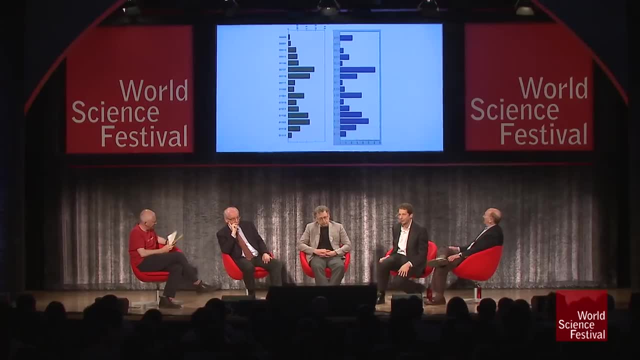 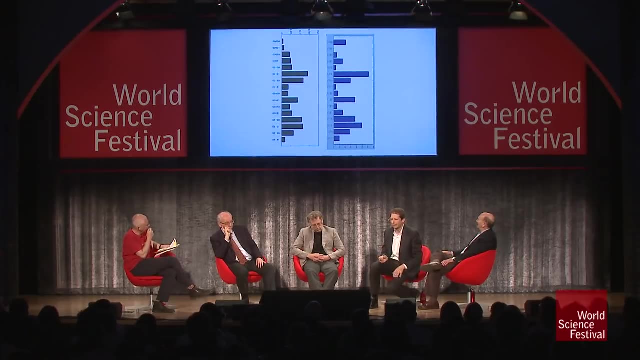 Camp, a camp for math whizzes in high school who actually understand quite a lot about probability and lots of other things in math. But you do the same experiment and you get almost the very same data, except a bunch of them are smart Alex. 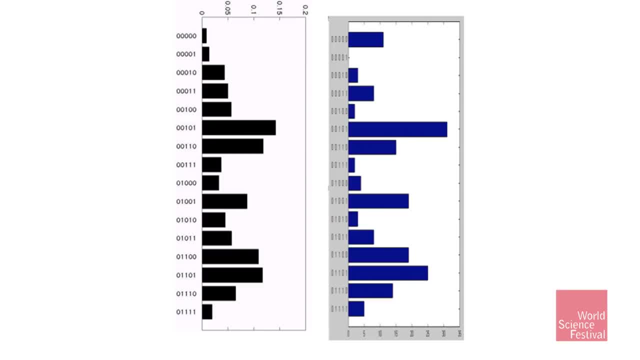 and wrote down 00101.. Yeah, those are the true mathematicians. You know that's as likely as anything else, But look at how striking the similarities are between high school kids in 2003 and whoever was listening to radio in the late 1930s. 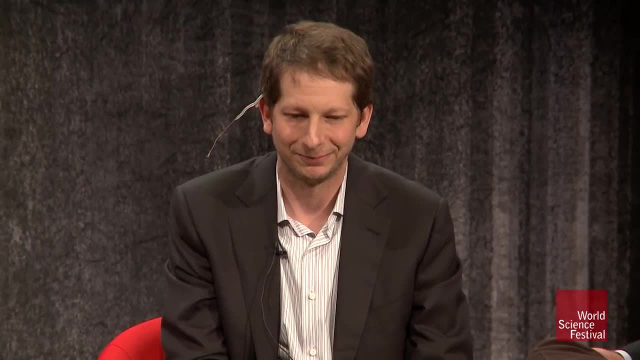 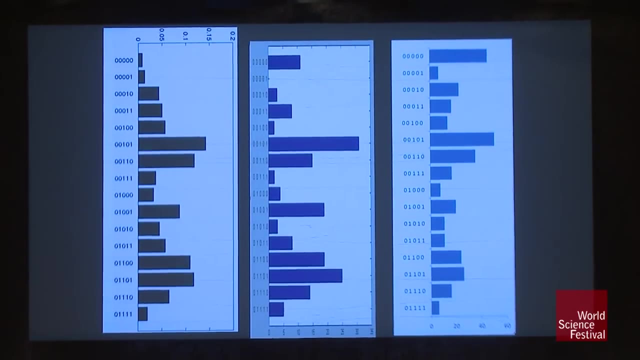 Now let's see the next one. I haven't actually seen the data yet, So this is the data that- oh, you see, there are a lot of mathematicians in the house Come out. Excellent, I mean, I have to say I mean yeah. 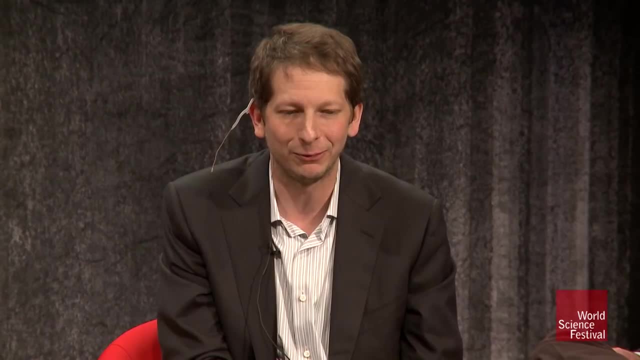 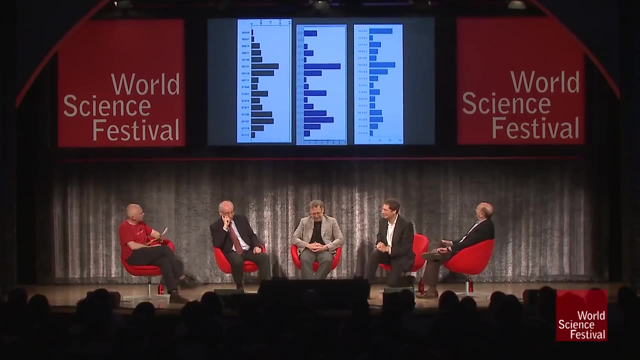 And a lot of psychics, yeah, And a lot of psychics. yeah, Look how well. what can I say? I'm impressed. I'm impressed by this experiment. I have to say It worked even better than I hoped it might. 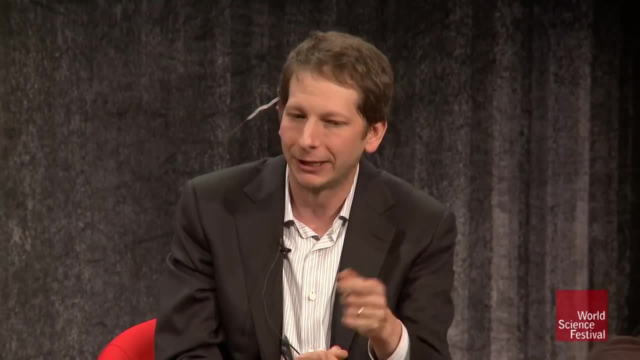 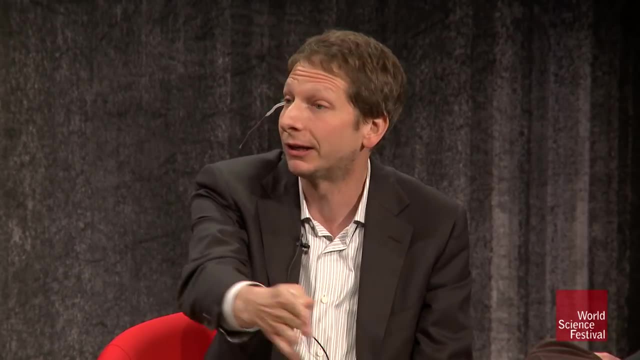 But it just shows that there is really something quite fundamental. Now, nothing here tells you what that structure discovery is, what's fundamental, But we've actually built models that can predict these kinds of things, basically doing a kind of Bayesian reasoning in which 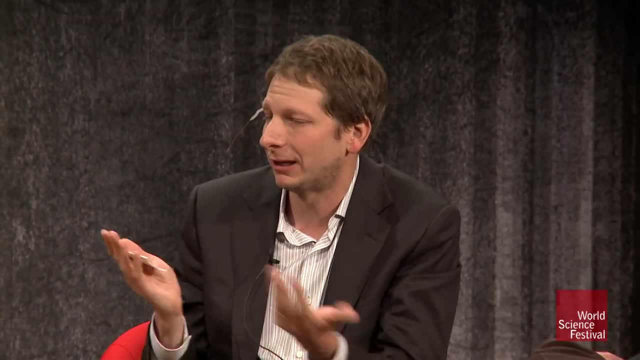 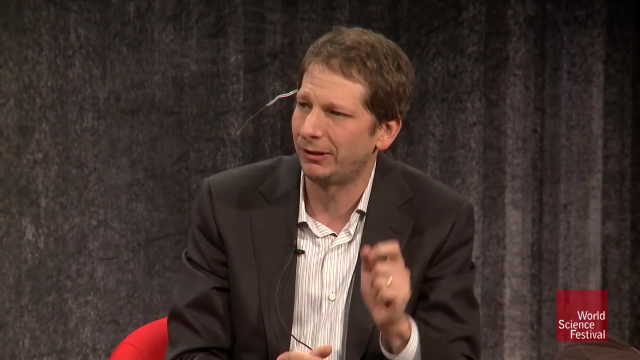 what you're looking at is a comparison of the alternative hypotheses. Just like you're saying, it's all about the different possible explanations And we basically say what are the different kinds of sequential dependencies, things like runs or repetitions- And we say that our concept of randomness is that you know. 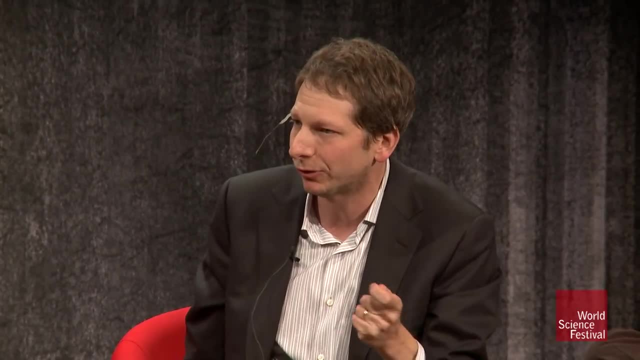 we're not interested- the brain isn't interested- in just things that happen completely at random. What we're interested in is the structure, the non-random things. So our intuitive concept of randomness, which this is tapping into, is really just anti-structure. 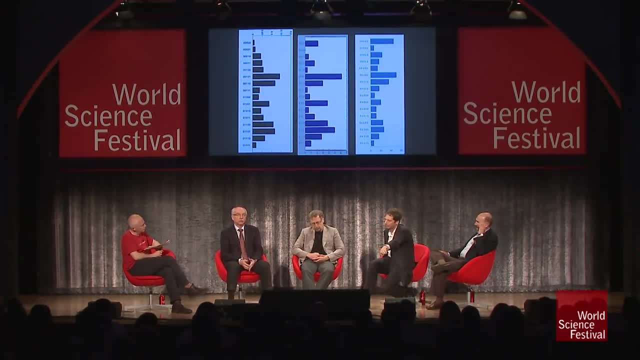 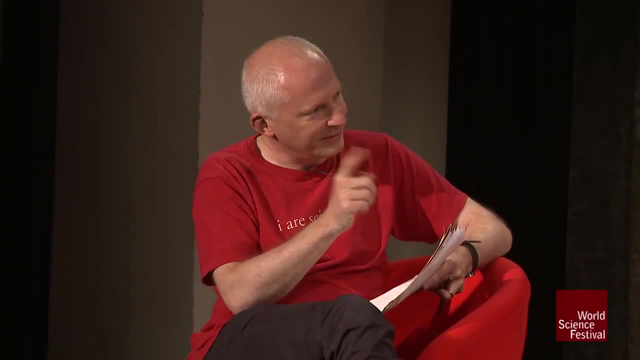 And we make a Bayesian model of structure perception And that's able to predict these kinds of things quite well. So, Leonard, we should come to your experiment that you all said, which is about: how Can I ask one follow-up? Yeah, go, yeah. 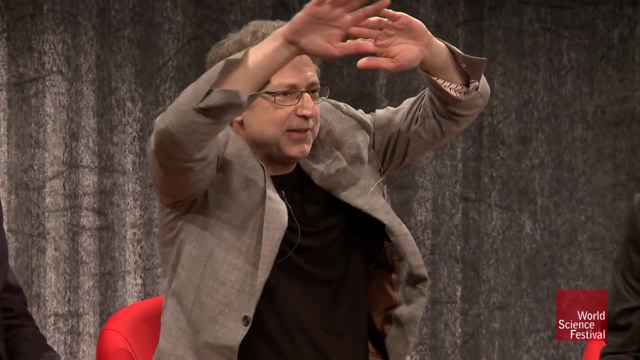 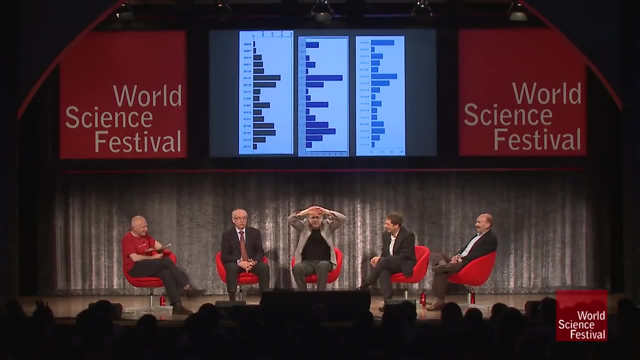 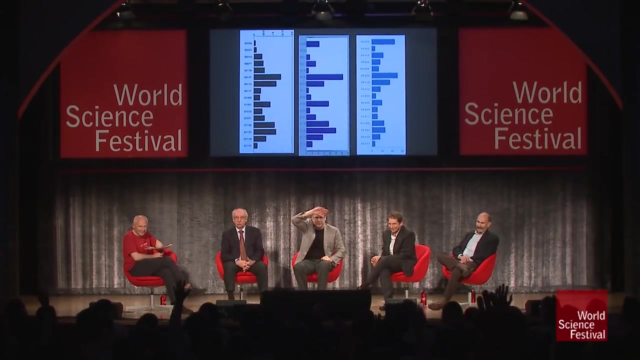 So who in the audience thinks that the head of the brain- heads, heads, heads, heads, heads, heads, heads- is less likely than the one that actually was thrown? You should know that. Who thinks it was more likely, OK. who thinks it was the same? 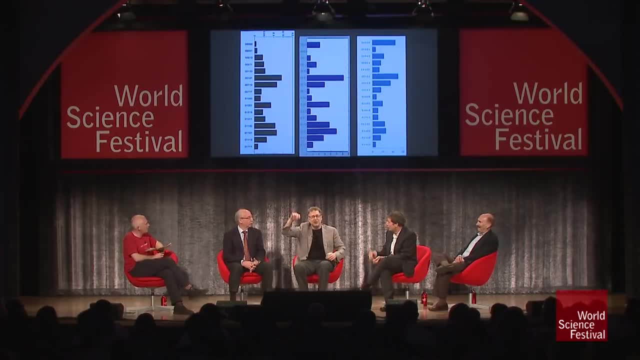 All right, good, They're all the same. So every synchronous has the equal probability. If you're actually flipping a fair coin, right, Well, if you're actually flipping a fair coin, But who cares about that? You see, the mind doesn't. 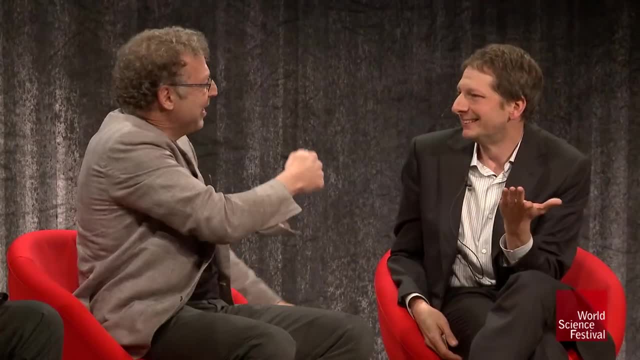 The parts of the world that aren't predictable. Wait a minute, I want to do some betting with you, But, Josh, did you actually what was it exactly? Heads, heads, tails, heads, tails. Or did you just say? 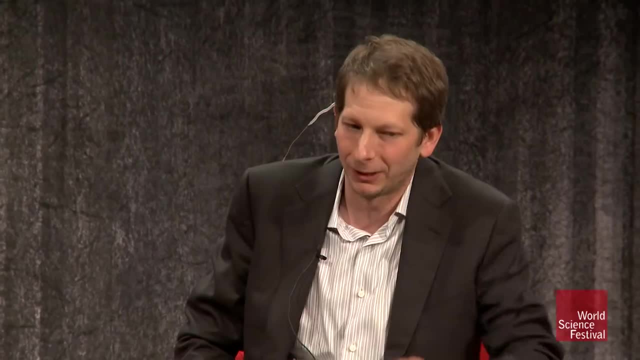 Well, there's something magical about tonight, like the first birthday, Because I would have said that no matter what, because I know how the data are going to look like. But in fact I did actually put that sequence. I swear Really. 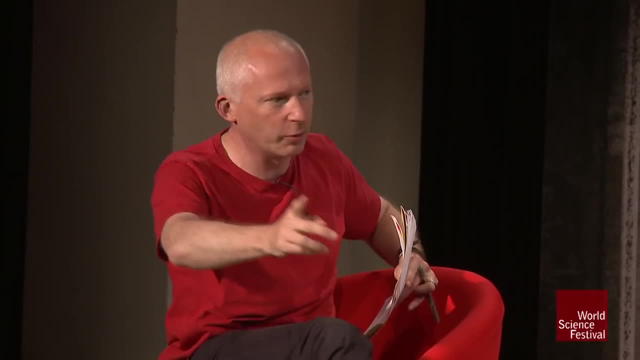 I did. I'm not sure yet Now, Leonard, I want to come to you because we're getting near to the end of our time. All right, we'll go fast, But I'm worried about the 0, 0, 0 with all you smart alecks. 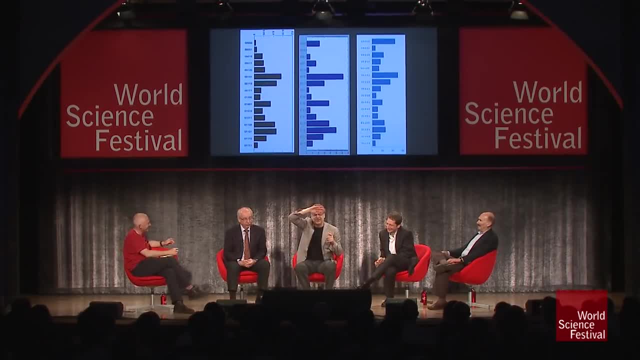 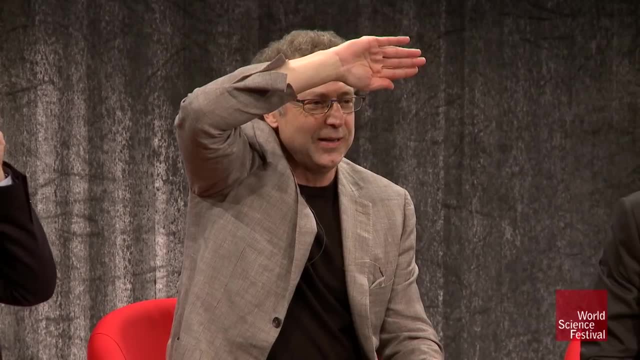 because I normally so. here's something about science that you learn about. You know, taking data is an art, And I didn't talk to whoever was tallying these numbers And, And, And emphasized to throw out the outliers. So if any of you guys said 1,000 countries or 10,000, 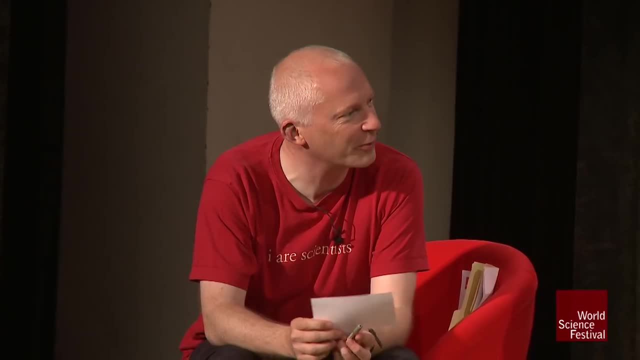 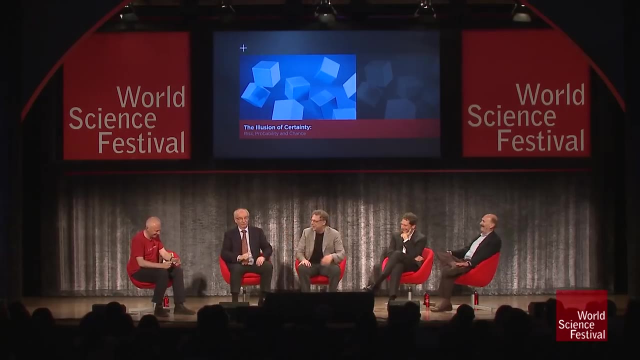 in Africa. this thing is totally screwed. No, no, no, I've had it where people put negative numbers. What about imaginary numbers, Complex numbers, Anyway? so I think there are. Don't give me the answer yet. No, no, I won't do. 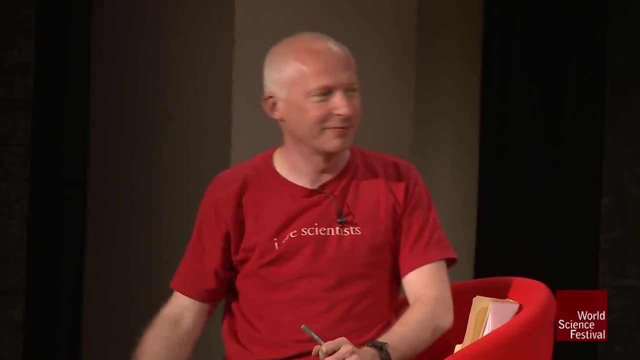 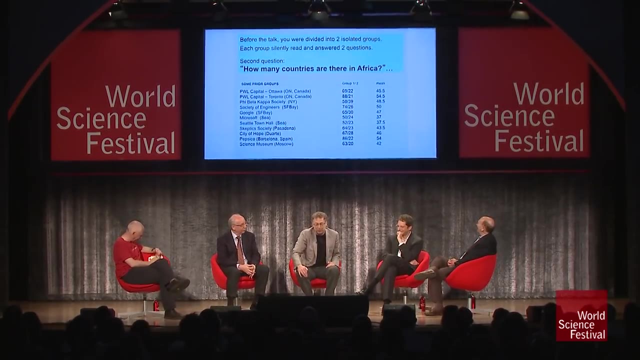 But I think you'll be pleasantly pleased with the outcome. Can I have my first slide here? OK, In Africa, there we go. Here's a few. This is a random selection of other places that I've tried this, Although you know really they all did work as well. 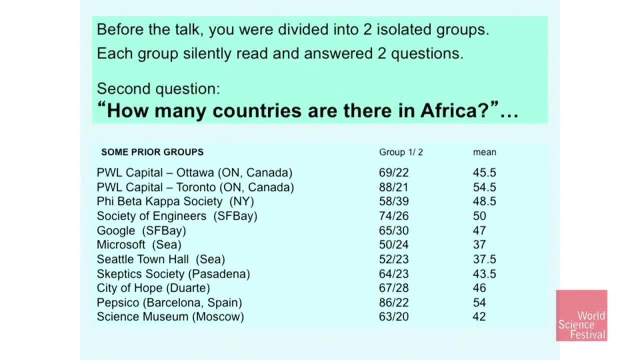 So if you'll notice that group 1 tends to guess around 60 or 70. And group 2 tends to guess around in the 20s. So there's a fifth Group 1, which was you guys, I think, right. 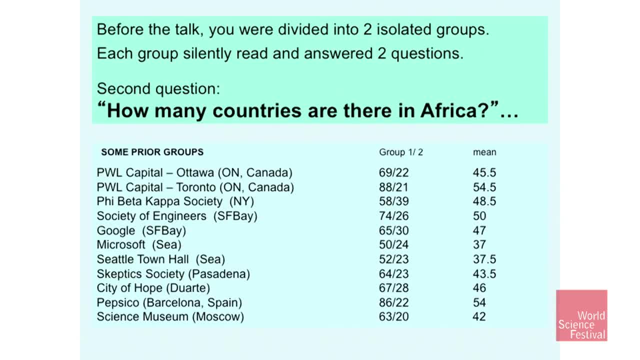 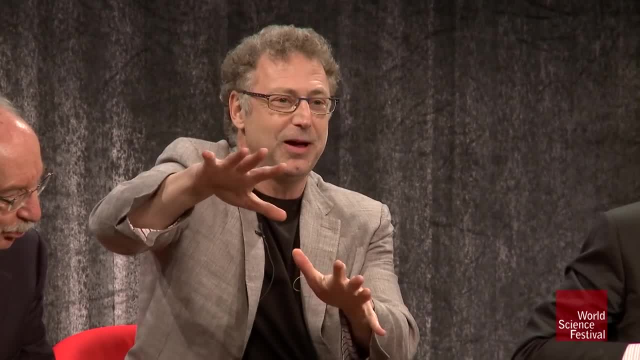 You tended to guess about three times as much as group 2.. So I somehow, using my own psychic powers, I managed to influence you guys to guess much, triple the number as you guys, And so let's see the answer. OK, So there you go. 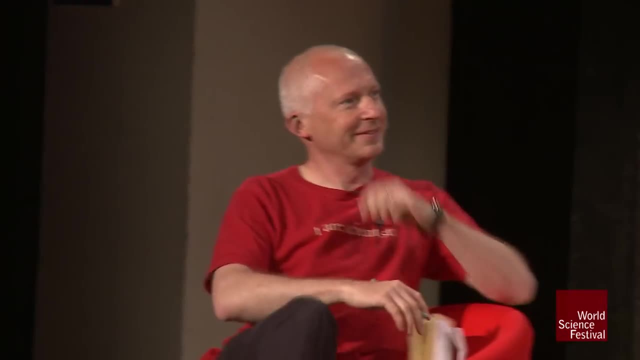 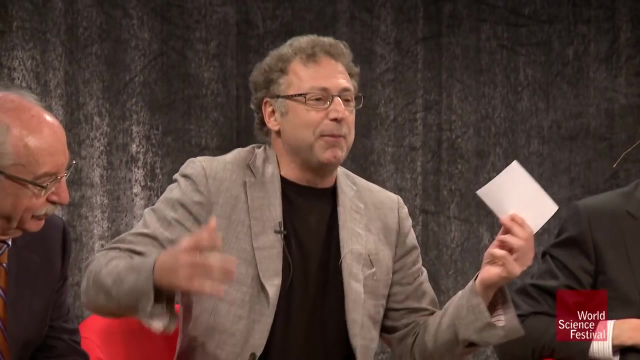 Yeah, I mean, it's absolutely amazing. So group 1, 57, 57.39.. So that falls right in there, And group 2, 28.89.. So how did you influence? So it's about double. 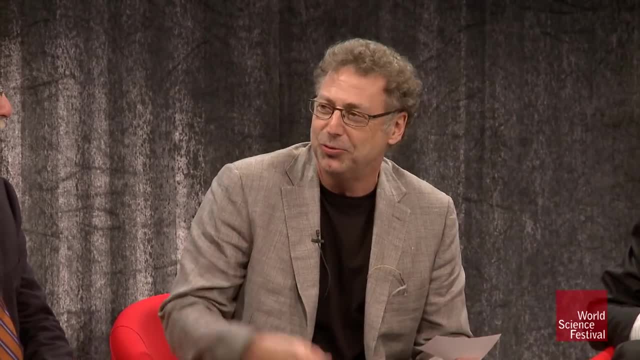 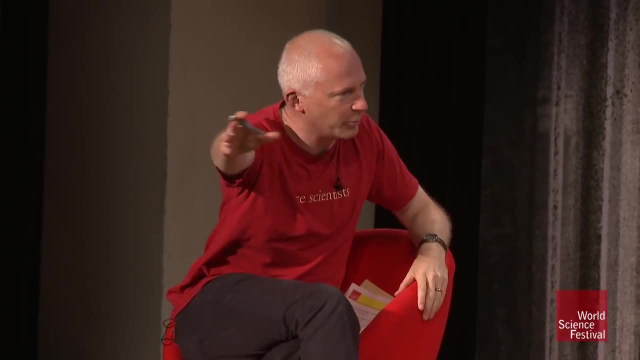 It's about double here And the actual number of: yeah, the last time I counted it, which was a couple of years ago, but I think it's 54.. OK, yeah, And the question is: yeah, So you need to explain how you influence. 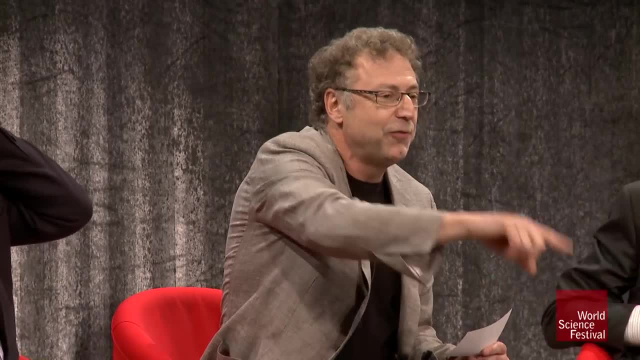 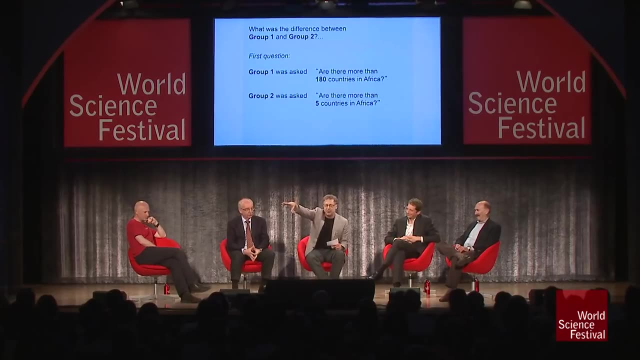 Yes, I'm going to. So here's the punchline: How do I influence you? Well, the first question, The first question was: show me the next slide, You'll see. you get a different first question. OK, You guys were asked: are there more than 180 countries? 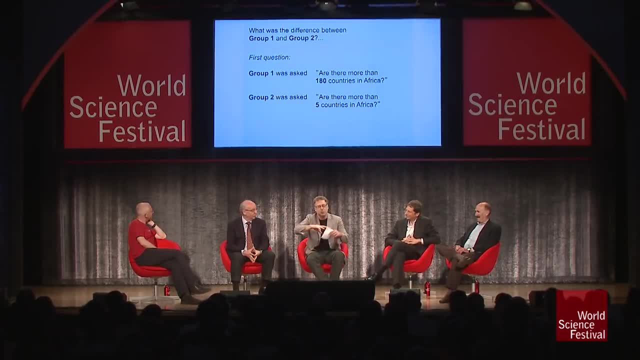 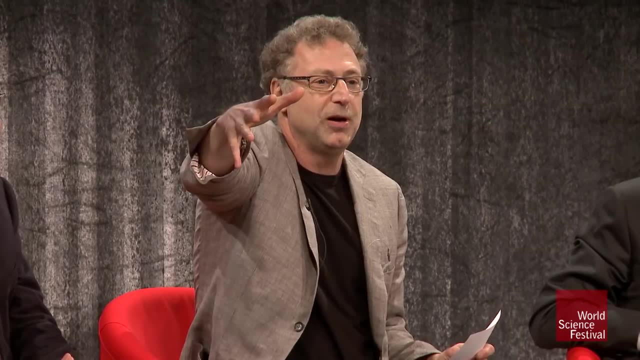 in Africa. You guys were asked: are there more than five countries in Africa? And I'm assuming that you both thought most of you. these are absurd numbers. But just the mentioning of that absurd number skewed your estimate. So this is called anchoring. 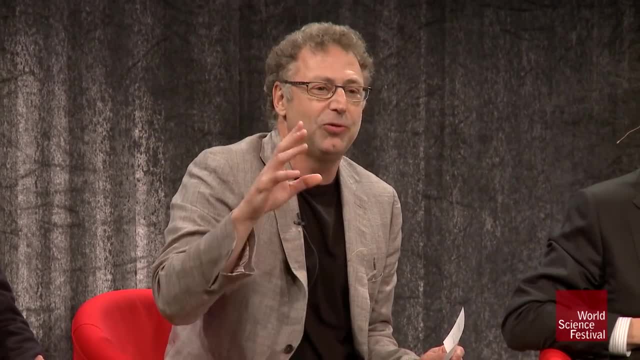 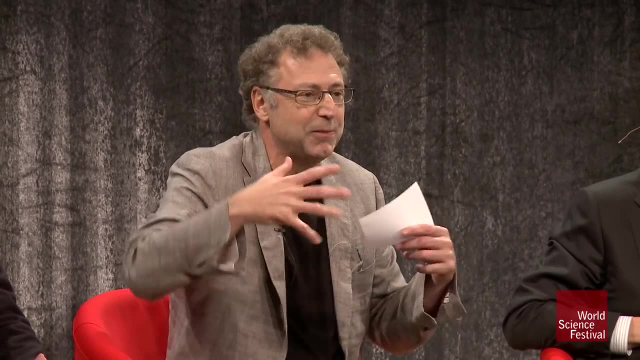 And it's an example of a broader thing called priming And it just shows. the point of this is to show that when you're trying to understand probabilities and statistics and do these sophisticated analyses, a lot depends on also having the right data in your own lives. 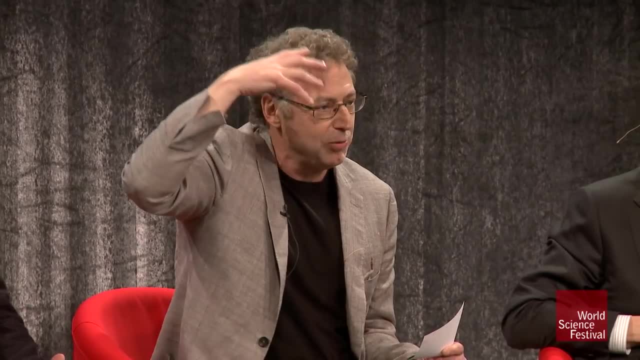 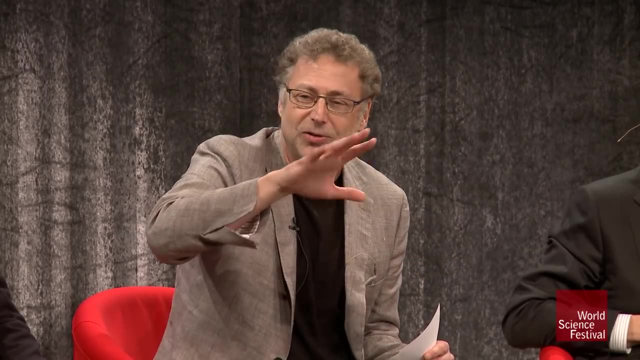 when you're trying to estimate how likely something is or what's going on, to remembering and having the right feeling for what the actual number was, And your estimation abilities. quantitative abilities- are easily influenced by irrelevant factors, And that was the point. 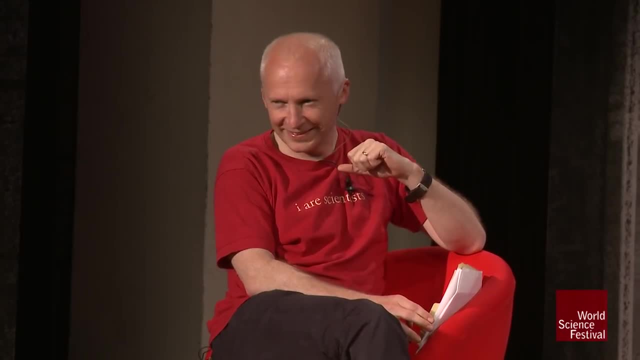 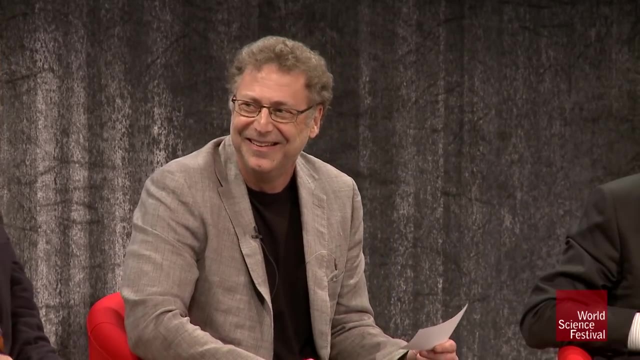 Excellent. 33 countries now 33?? No, 35.. No, Well, we can talk. Well, I thought it was going down by 20 since I heard that. Well, we've just got a few minutes left, So I'd perhaps like you all to just sum up. 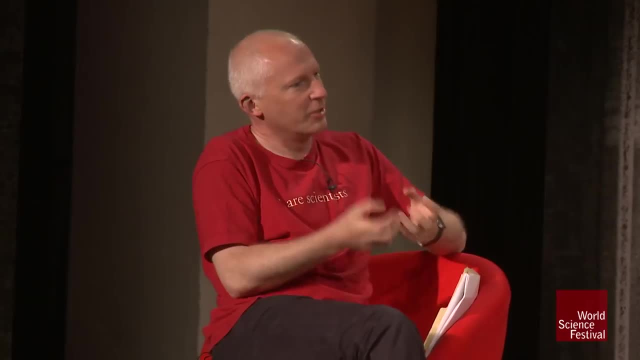 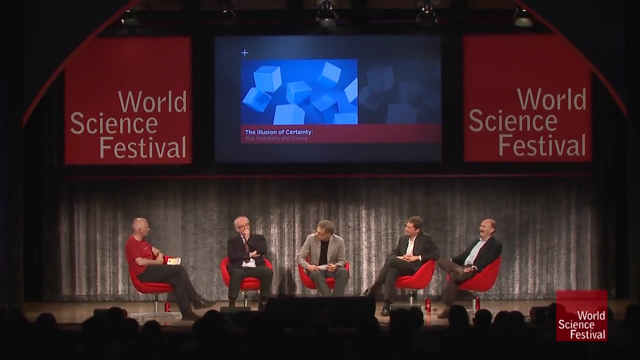 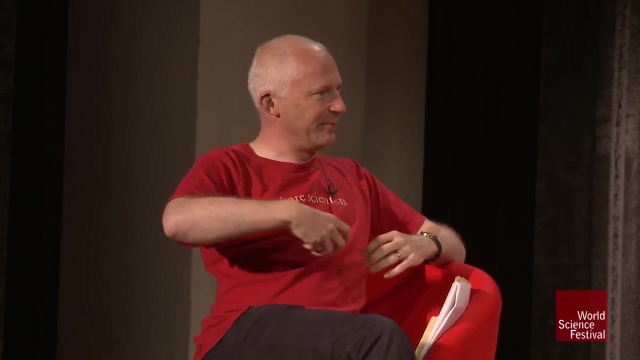 whether you think that, whether we can actually negotiate the huge amount of data that we meet every day. I mean, we seem to be leaving data all over the place. Do you think there is hope for actually tonight? I think we've really helped this audience to change our perception. 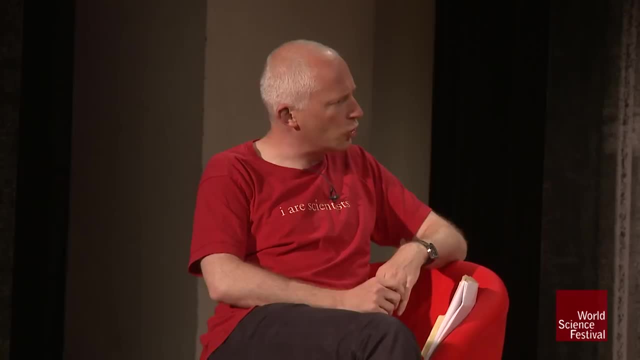 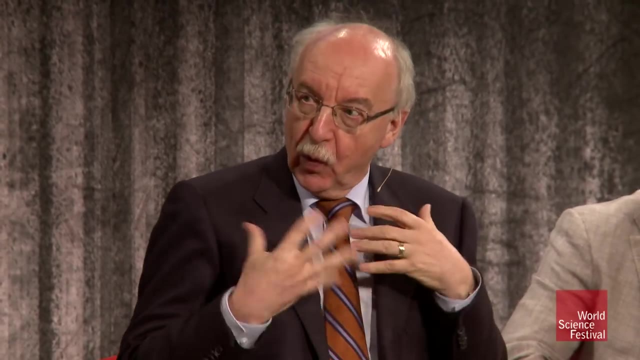 on how we can interpret data and risk and chance. I mean, Gerd, do you think is it natural frequencies which is key to helping us? Natural frequency is just one of the representations that are easy. I think the key is to go beyond the illusion of certainty. 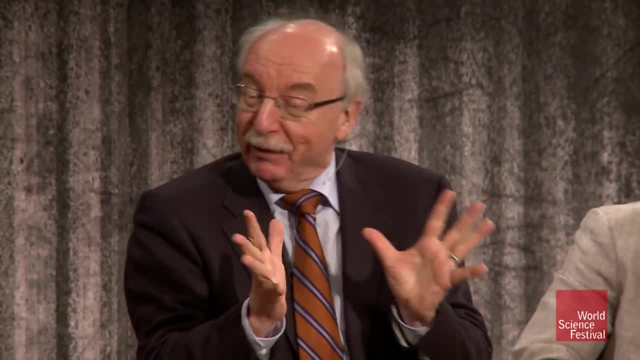 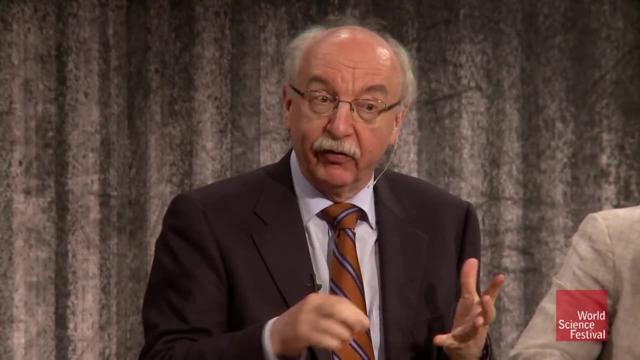 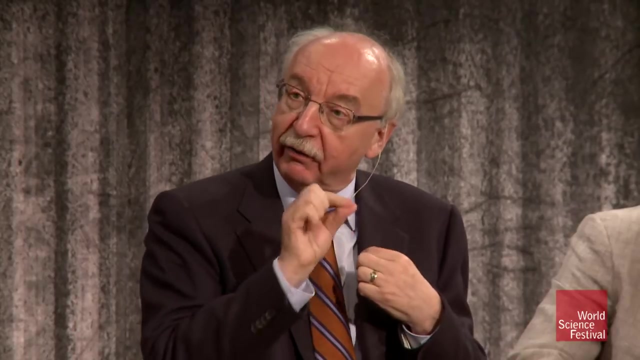 which we didn't talk about today, which basically means seeing certainties where there are none. And in this world, as we know, there's nothing certain except death. and And how do we get to what I call a risk literate society? 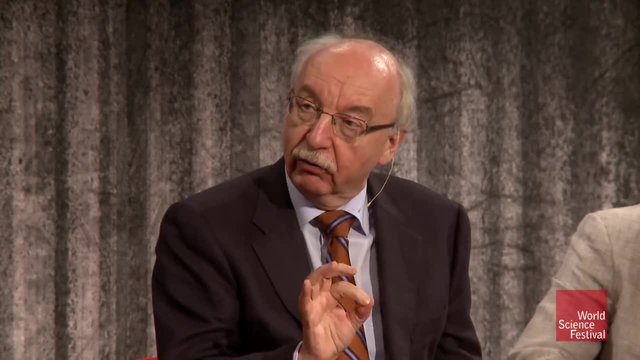 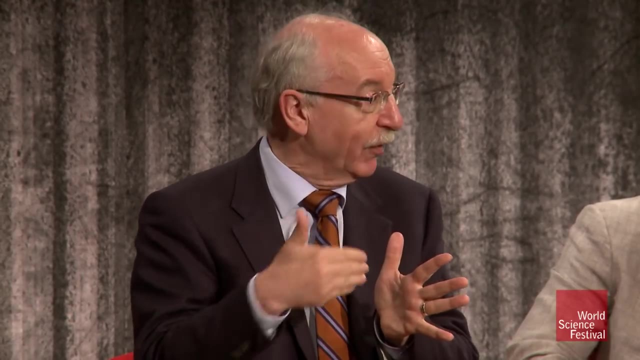 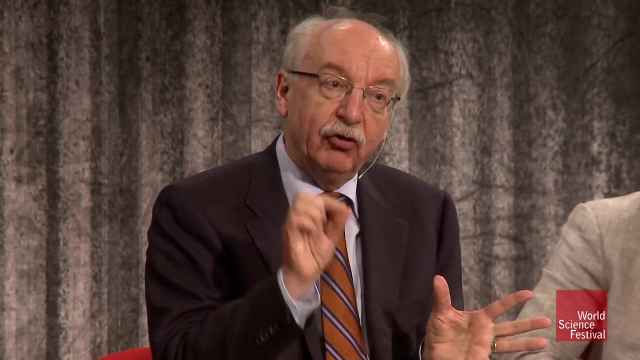 How do we get there? We need to change the schools- elementary school, high school- and teach statistical thinking, not statistical rituals as in psychology. And we are still teaching the next generation the mathematics of certainty. We need to change that. And instead of trigonometry and geometry, 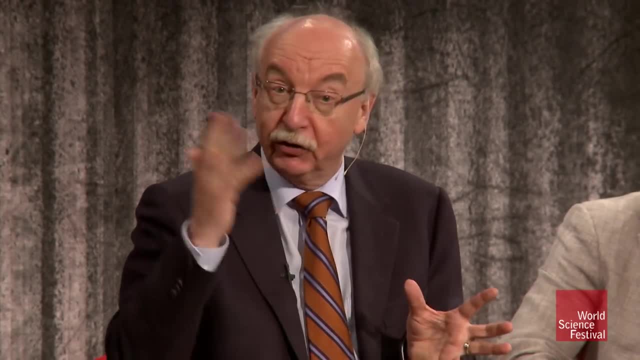 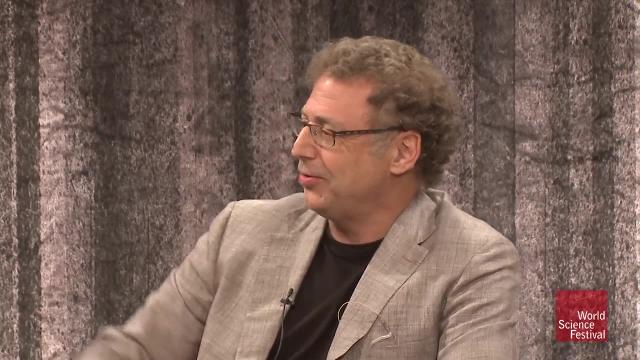 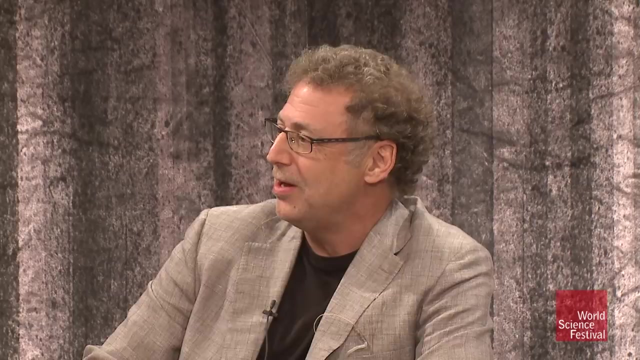 focus On the things that are really relevant later for doctors, for judges. Leonard, would you agree with that? Yeah, I think that we can learn Like after Gerd's explanation. hopefully, when people go for medical testing, they'll understand how it works. 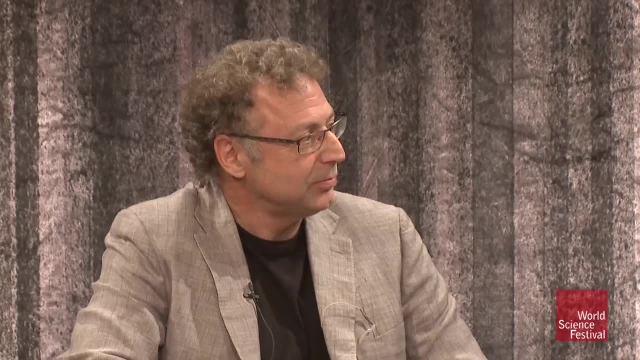 And Joshua, do you think we should be tapping in more to our natural abilities? Well, I would say yeah, I mean it's in common with these guys. It's all about understanding how the brain works and how the mind works. understanding. 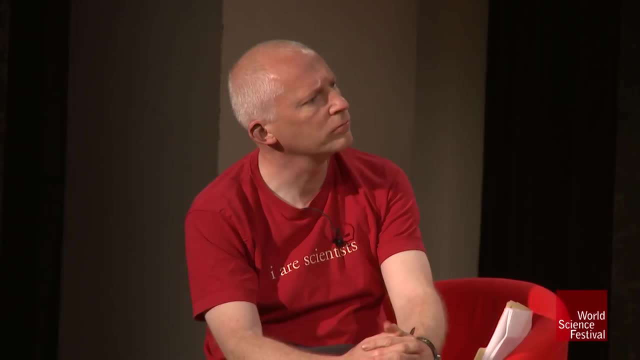 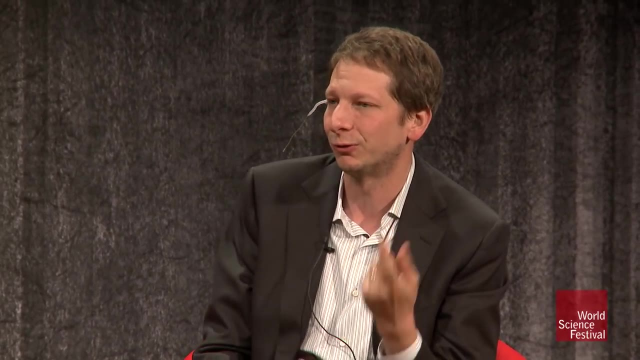 the kinds of representations that our minds are designed to work with, Understanding the kinds of inferences that we're good at, the ones we're bad at, And I would say, particularly in the computer age, what are the different ways we can use computers, rather, 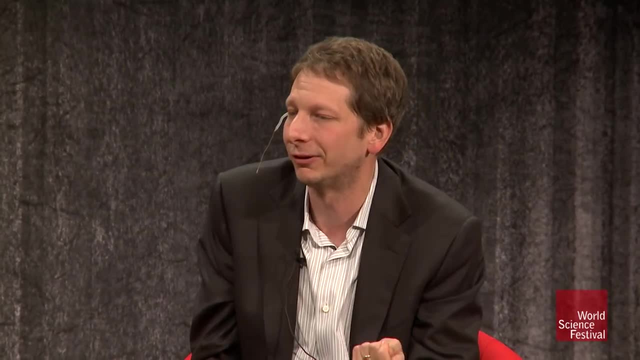 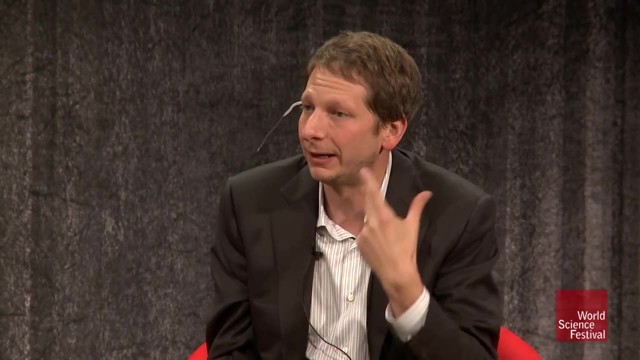 to make diagrams or visualizations that show the patterns that we wouldn't otherwise see in the ways we wouldn't see it. Or to say, make machine learning algorithms that are able to find patterns in data the way our brains do, but scaled up to much bigger data sets and worlds of data.